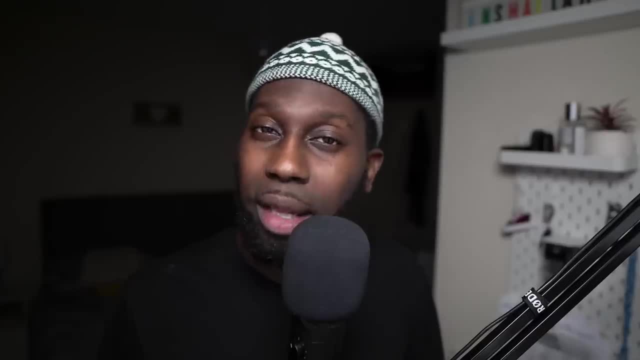 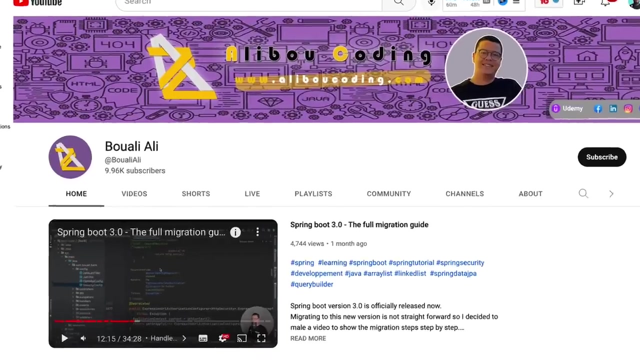 crash course on Spring Security and there was a lag with JWT section, So we decided to rerecord the entire section and actually make it so extensive. This crash course right here is brought to you by Aliboo and is the one that led the Spring Security, So go ahead and subscribe to this channel. 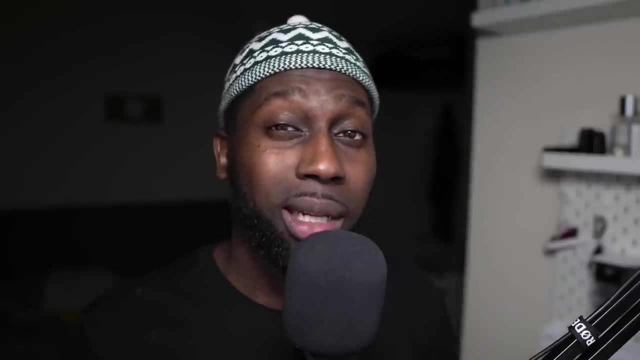 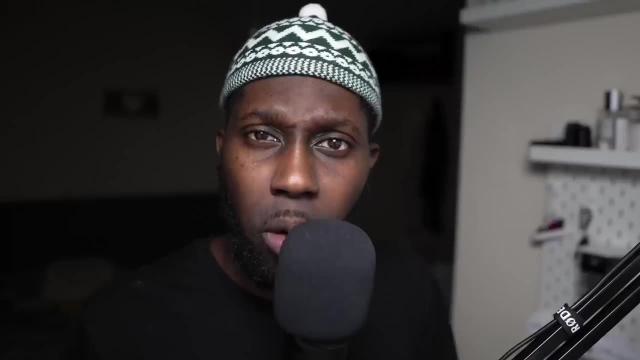 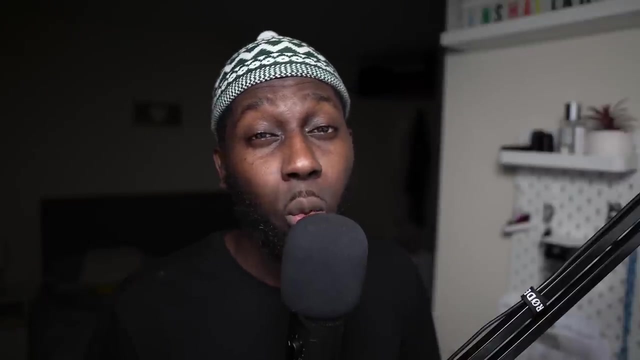 Show some love, because it's going to be bringing you awesome content like this from time to time. Security is a must when designing and building APIs, and it's really important that you understand JWT so that you can secure your APIs. Before we crack on, literally just take one second and smash. 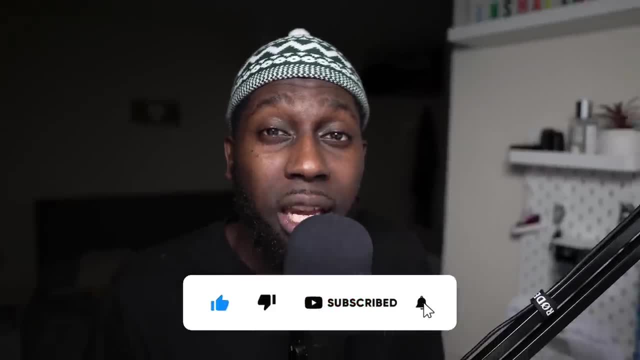 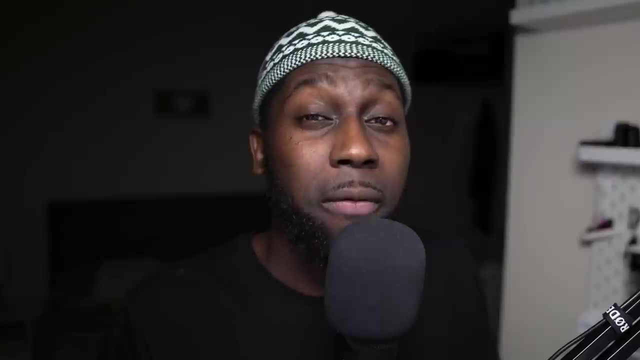 the like button. Also, if you're new to the channel, subscribe, And if you haven't joined the private Facebook group as well as Discord, go ahead and join, Because the community is growing and we're waiting for you. So, without further ado, let's kick off. 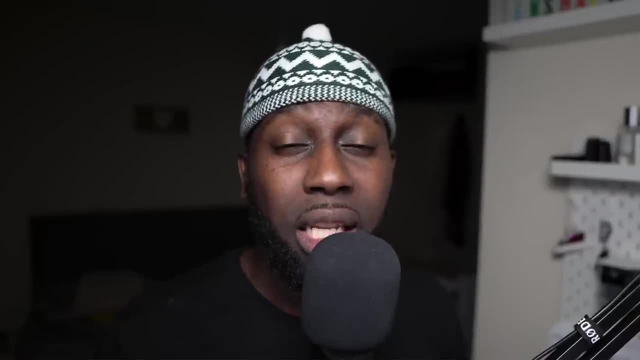 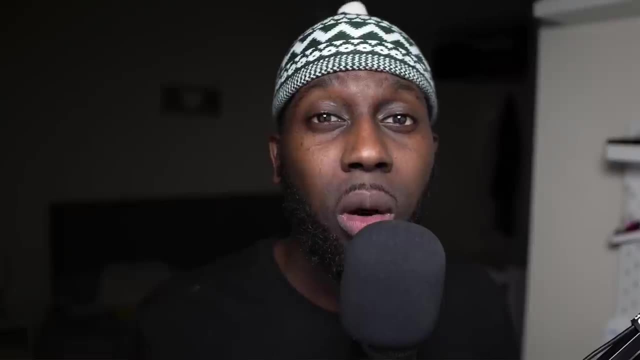 I just want to say that you can grab the entire source code and the description of this video so that, if you have any issues or you want to take what you learn from this course and then apply it within your own API, you can do so. feel free to clone the. 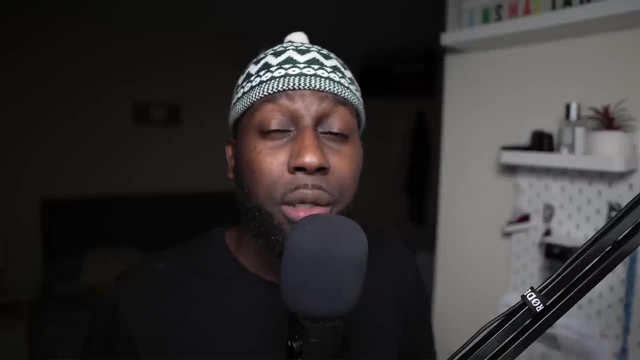 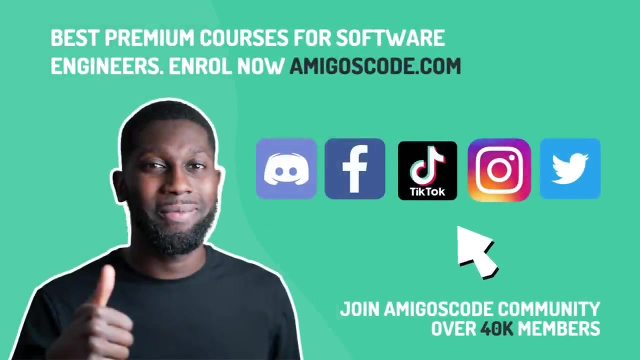 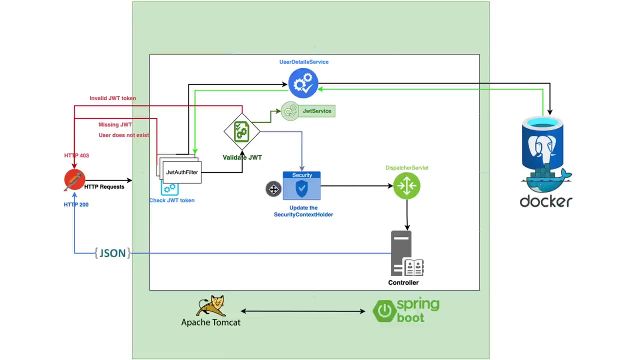 repo and, yeah, just use the code as you intend. And if you have questions regarding JWT, literally just ask on the community and someone within the community will be able to help you. Before we start the implementation process, let me first explain to you how this JWT validation mechanism works. The whole story starts when a 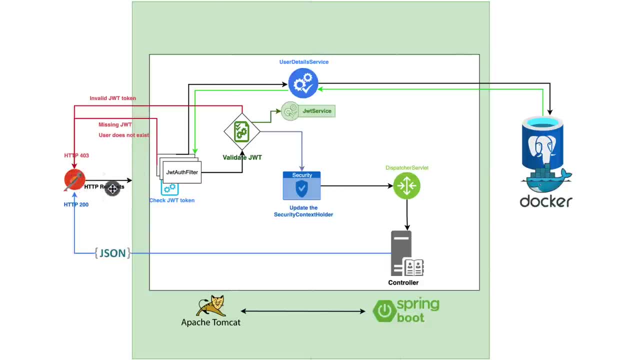 customer and a client send an HTTP request to our back-end system, which is running using spring wood container run running on an Apache Tomcat embedded server. So just a reminder for you: the first thing that gets executed within a spring application ease the filter. 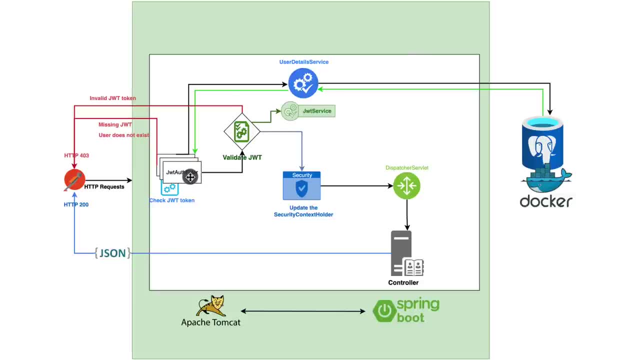 So anytime and each time you create a filter, just notice and remember that it will be the first thing that gets executed within our application. so in this case, the first thing that will be executed is our jwt authentication filter, and this is only a once per request filter. 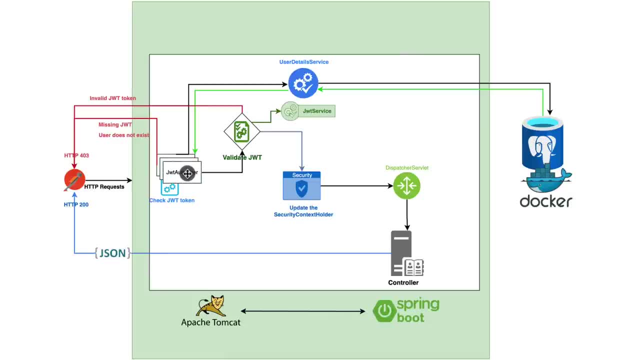 and has the role to validate and check everything regarding the token, or the jwt token, that we have. so now let's start the process. the first thing that will happen, we will have here an internal check to check if we have the jwt token or not. so if the token is missing, 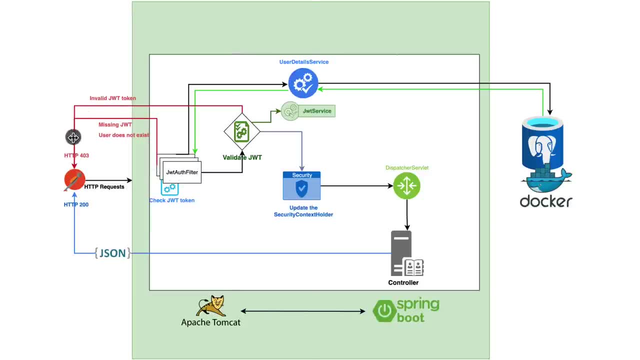 as we can see here, we will send a 403 response to the client. so, and the reason is this: missing jwt. all right, so now we have our jwt token and then after that we will start the process, or the validation process. So this validation process will start in this way. 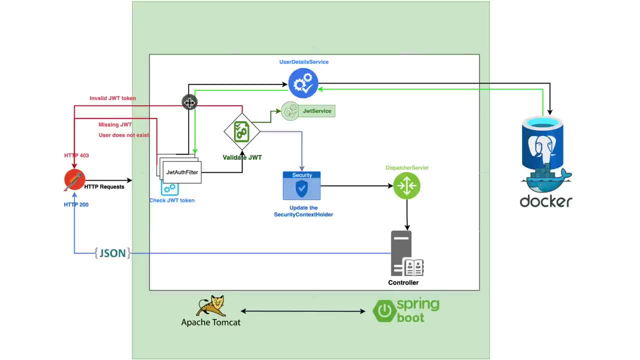 So the filter, like the internal execution, will first make a call using the user details service to try to fetch the user information from the database And this we will base on the user email that we will set as a claim or a token subject that we will extract within this JWT authentication filter. 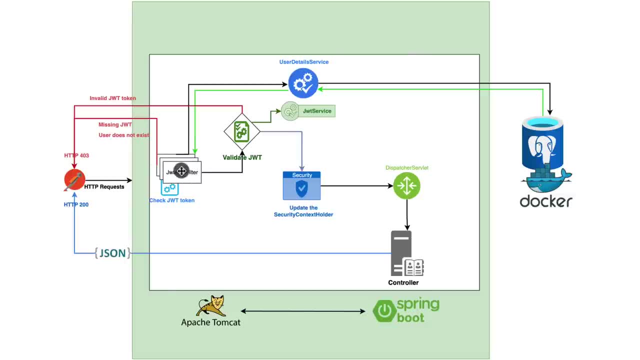 So I repeat again, this JWT authentication filter will check the JWT token, extract the username or the email- or we call it the subject when we talk about JWT tokens- and it will use that email to fetch the user details information from our database. okay, 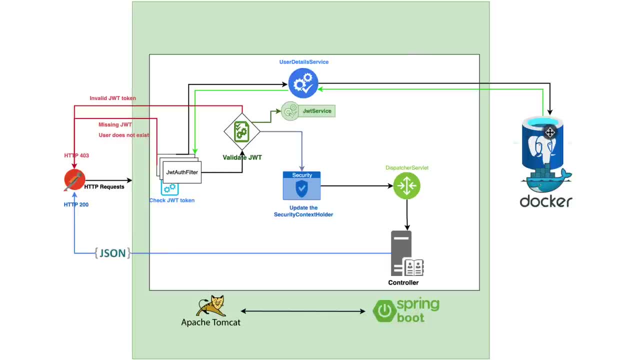 So this is the first goal. Then, once the user is fetched, we have the response from our database and the response can be either way: Can be existing user or non-existing user. okay, So once we get the response to our JWT authentication filter, 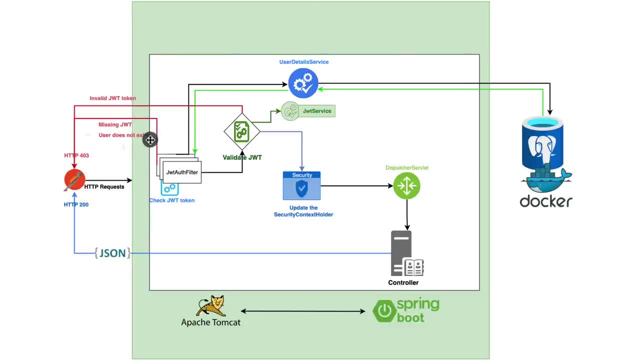 here we will make a few checks, which is, if the user does not exist, we will also send a 403 to our customer. In case everything is fine and we get our user from the database, we will start then a validation process. So this validation process. 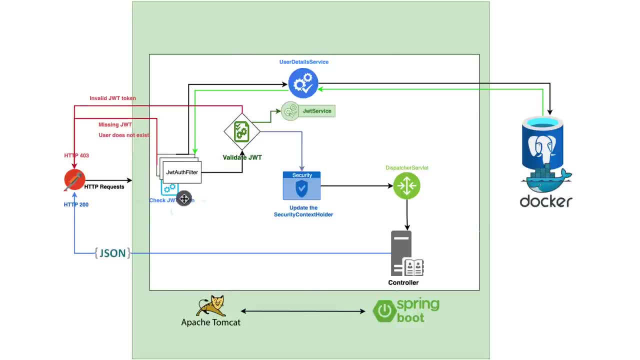 because this JWT token was generated for specific user. So we want to validate this token based on the user. And here we have this validate JWT process or mechanism, which we'll try to call a JWT service, And this JWT service will take the parameter: the user itself. 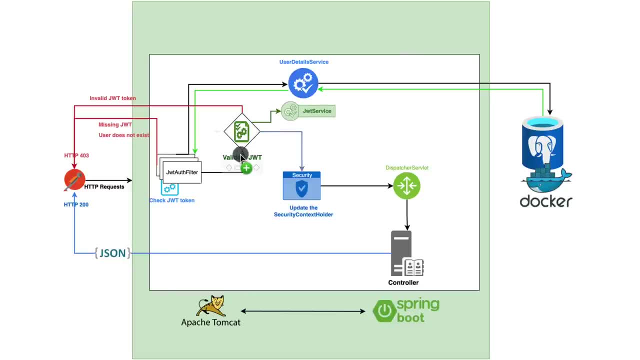 and also the token, or the string token, or the JWT token, call it whatever you want- After the execution of this validation process. here we have two case scenario. So the first one: the token is not valid, So it's not so, for example, the token is expired. 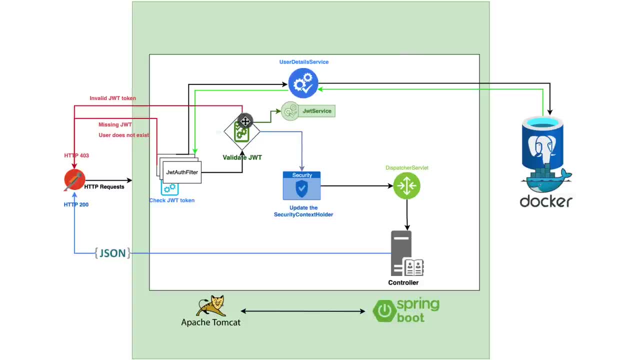 or the token is not for that specific user. So what we do, we will send also a 403 back to our customer. So, and the reason will be this: invalid JWT token. Otherwise, what will happen? we will call or we will update the security context. holder. 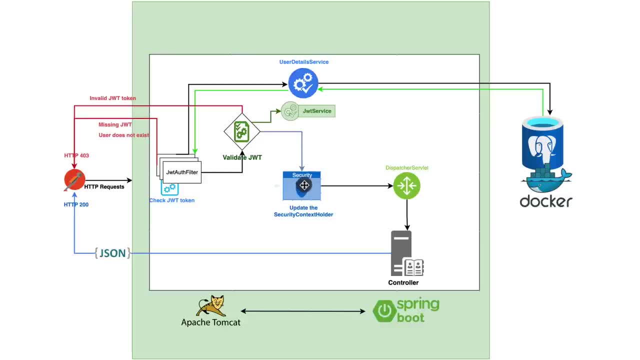 and set this connected user, Because when we fetch the user details information from the database, we will be able to set this security context holder. So we will tell Spring or we will tell the set or the rest of our filter chain that this user is now authenticated. 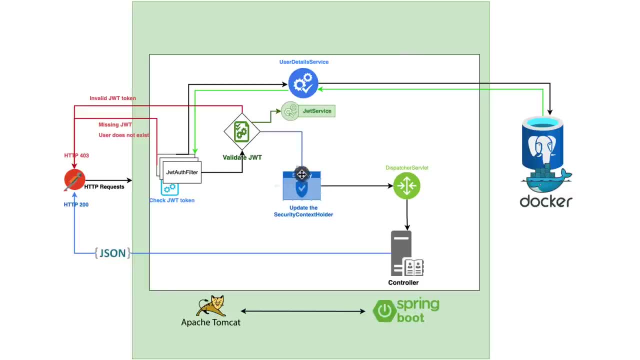 and we will update the authentication manager. So every time we check if this user is authenticated for this request, the answer will be yes. Once the security context holder will be updated, it will automatically dispatch the request and it will be sent to the dispatcher servlet. 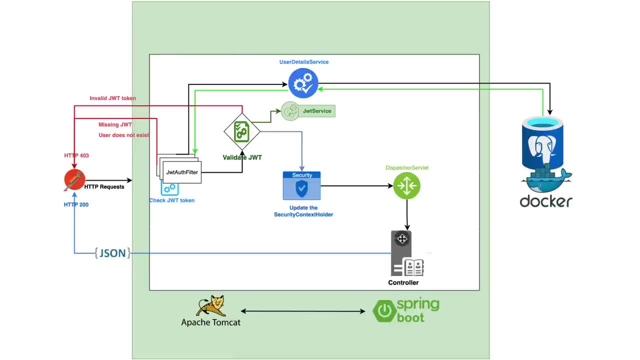 And from the dispatcher servlet it will be sent directly to the controller. We will do all the execution that we need to do, For example, calling the service, going to the database and so on and so forth, And then we will send back a response. 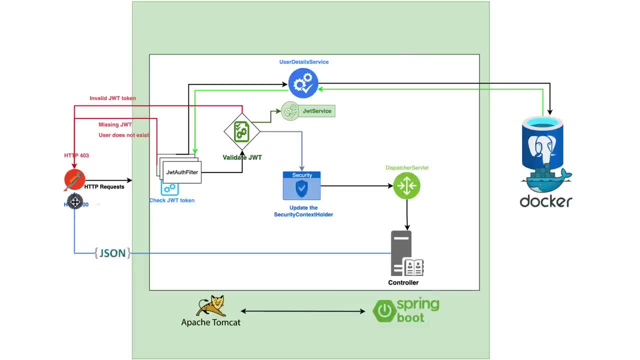 For example, it can be a JWT and it will be HTTP 200 or whatever any process that will get executed within this controller. So this is how JWT authentication mechanism works. Now let me show you how to implement this and how to realize these steps. 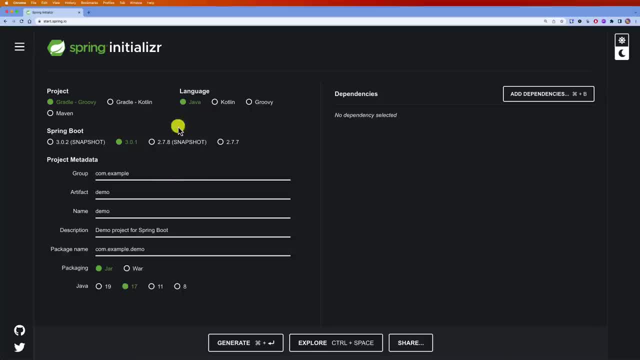 Let's first start by creating a new Spring Boot project. To do so, the recommended way and the way I also recommend is: Goi is going to startspringau, which is the Spring initializer, and create a new project from that. So first of all, make sure you want. 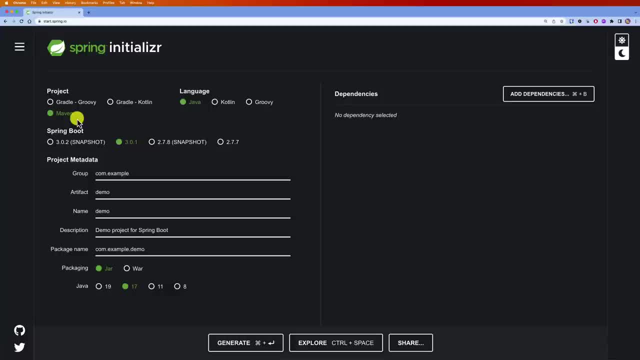 you use Maven. This is what I will be using in this video and tutorial. Then we want to use the recent version of Spring Boot, which is now 3.0.1,. okay, And also here, make sure you select Java 17. 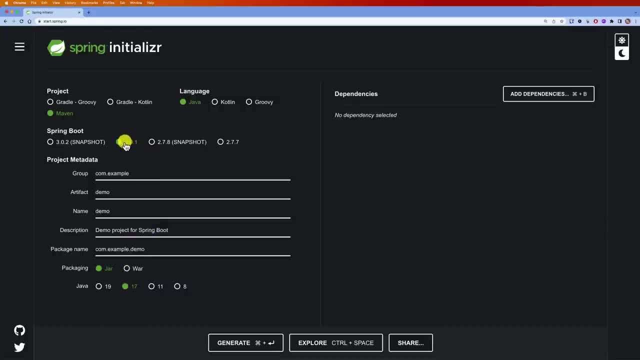 because the minimum required version which is compatible with Spring 3 is Java 17.. Next, select the jar packaging and now let's fill this, this project, metadata. So for the group ID, I will call it comalibu and the artifact, I will call it security. okay, 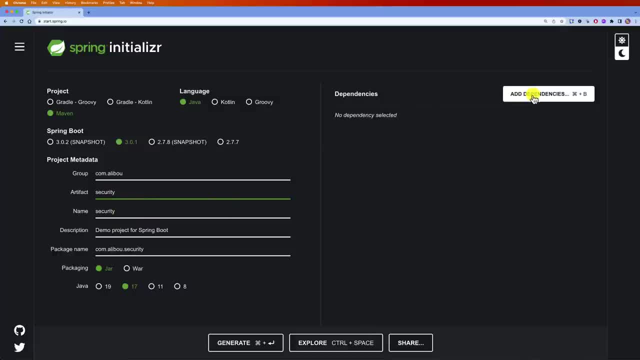 So I will leave the rest as it is, And now I will move on and add some dependencies. So, first of all, we need the Spring web because we want to expose few endpoints. We need also the security, and this is the main object of this video. 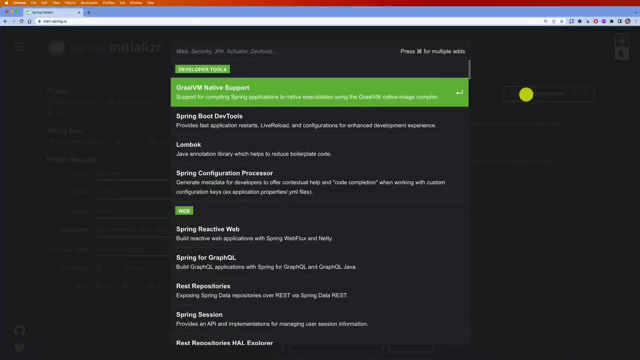 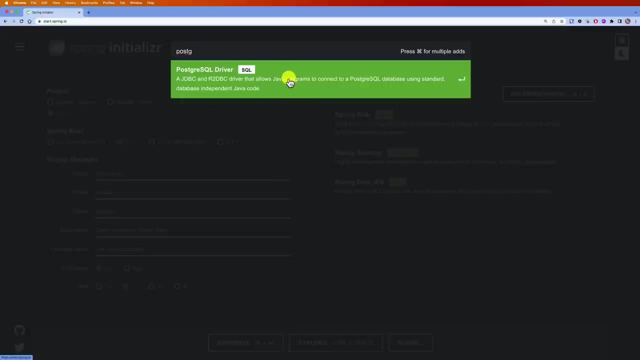 And then we will need JPA or Spring Data. JPA because we need to manipulate and interact with the database. Then we need a PostDegree SQL driver to connect to PostDegree SQL. You can also use any other SQL database like MySQL or Oracle or whatever. 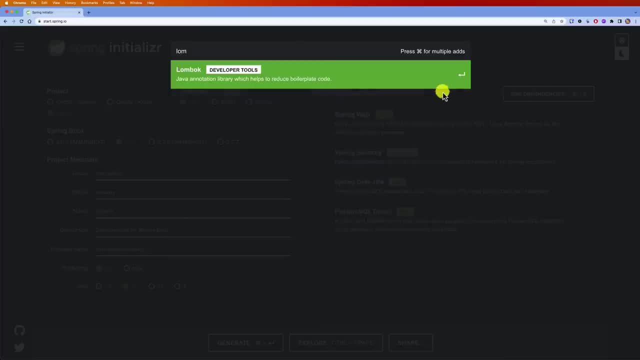 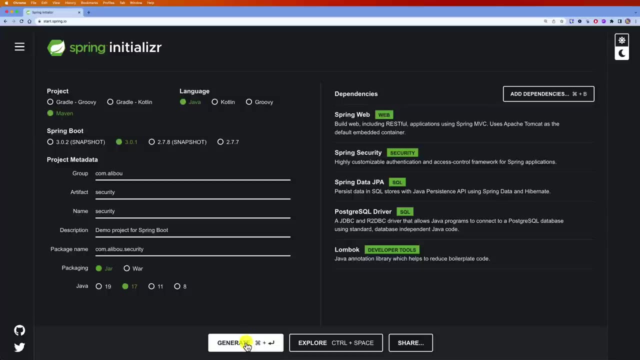 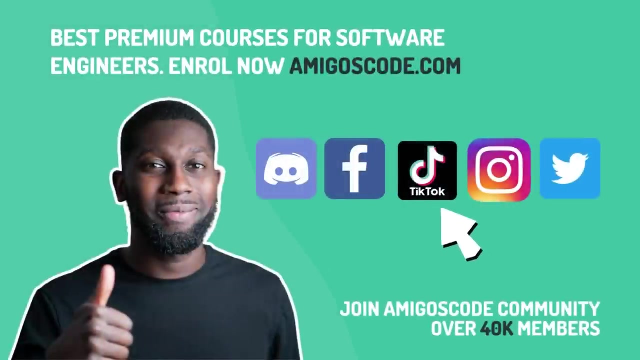 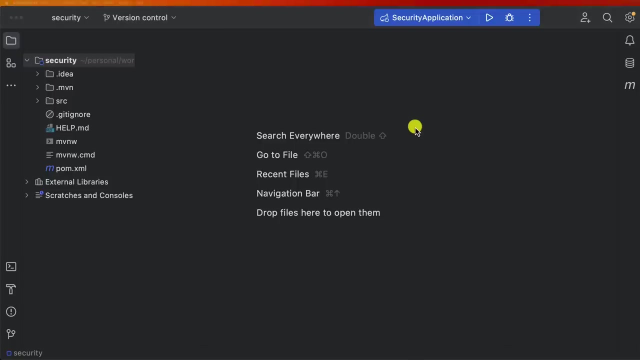 Finally, we want to use Lombok to reduce the boilerplate code. So now we have our project ready, We can just go ahead, click on generate and start coding. As I mentioned before, we will be using PostDegree SQL as a database for this application. 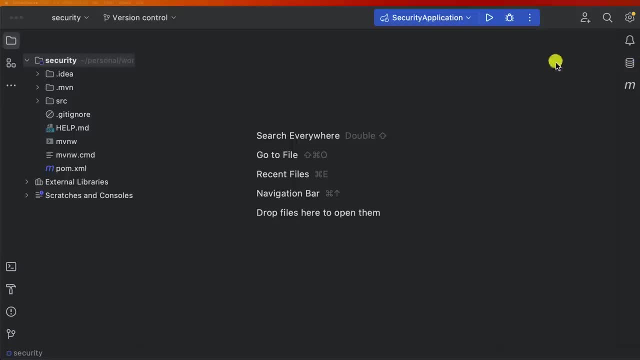 So let's first start by configuring our data source. For that I will be using NTDJ and I will use PostDegree SQL And I will use this database tool. So this one is available only with the ultimate version. Otherwise, if you don't have the ultimate version, 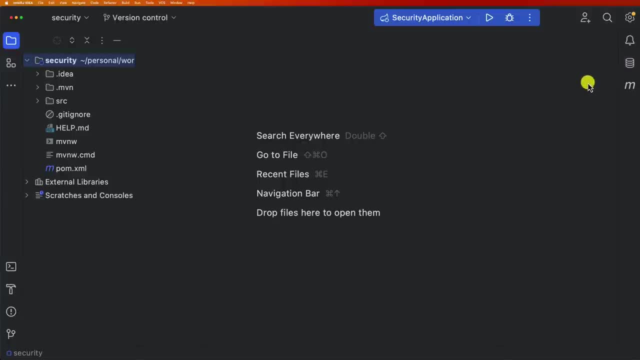 just make sure you install PostDegree SQL, and you can use the pgAdmin or you can use the dBeaver tool to connect to any data source. Okay, So let's start with that. Click on here and then we have this plus icon. 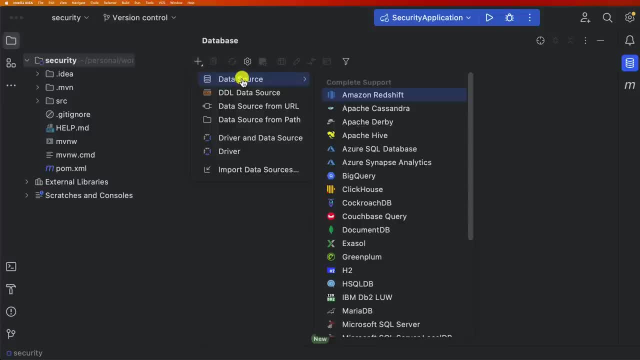 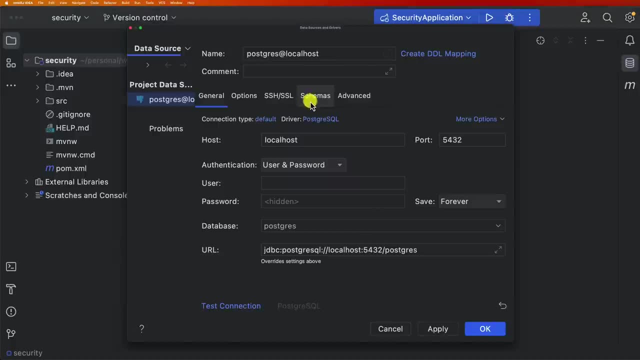 So click on this plus icon And then we want a data source and then filter for PostDegree SQL. Click on that And to be able to connect, so make sure here, if this is the first time you will have, instead of driver, PostDegree SQL. 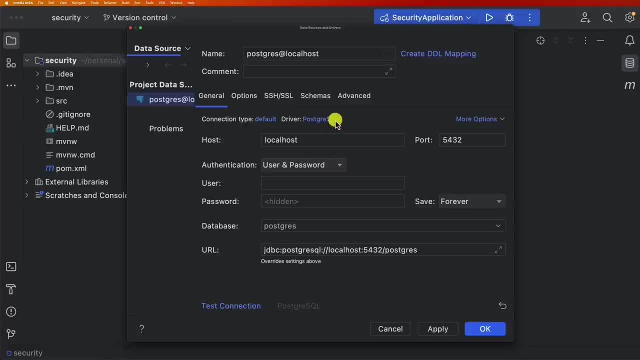 you will have a link or you will have a button here to download the driver. So just go ahead and click on it and download the driver. Next, the host is localhost because it's the local one And the default port for PostDegree SQL. 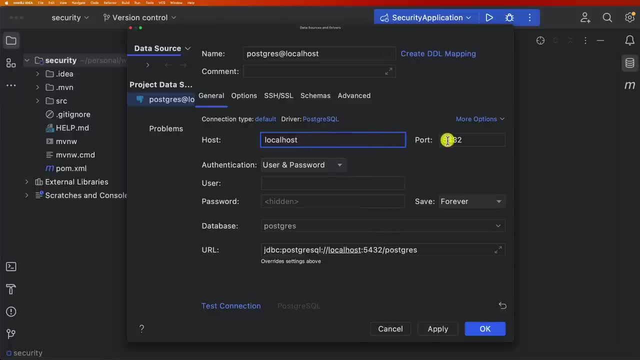 is the host. PostDegree SQL is 5432.. Then, if you create, when you created your PostDegree SQL, did you mate or did you choose a username and password? If yes, so just go ahead and specify them here. So for me, for the purpose of this tutorial, 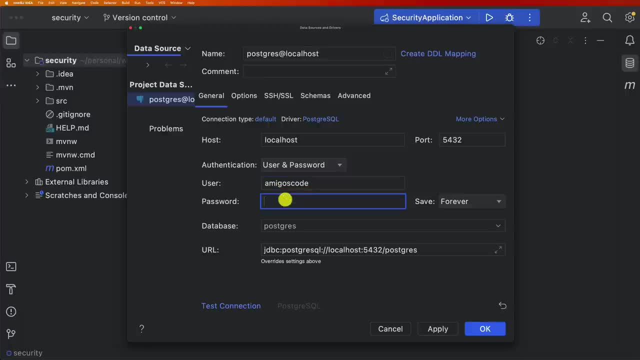 I made it Amigos code And for the password, it's just password. Okay, And then, once you fill all this, I will give you the information, just to check if everything is working fine. Click on this test connection and make sure you get this succeeded. 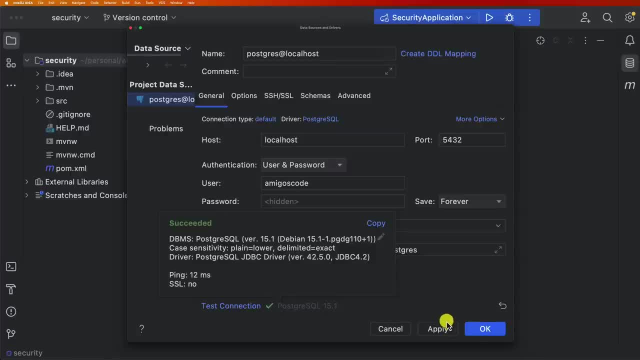 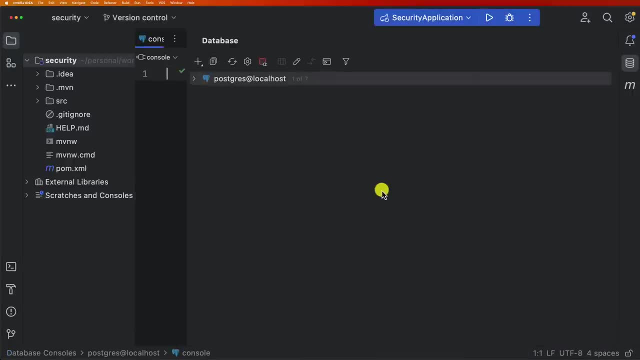 Otherwise, just check your configuration. All right, So now everything is done, I will go ahead and click on okay, And the first thing that I will do is I will create a new database. So right click on this data source new and then database. 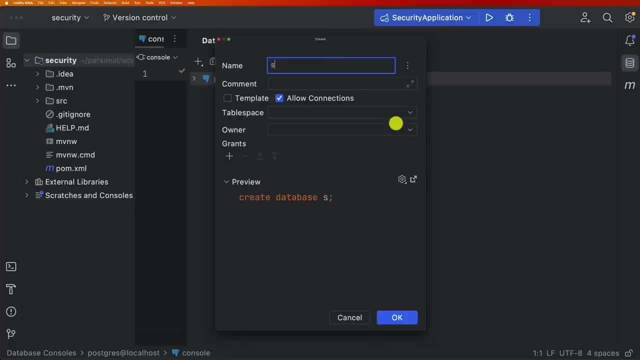 So I will call it JWT security And then hit okay. So the first time it will not be automatically shown, So just click here on this two of eight. the numbers might change from one laptop to another, And here I want this JWT security. 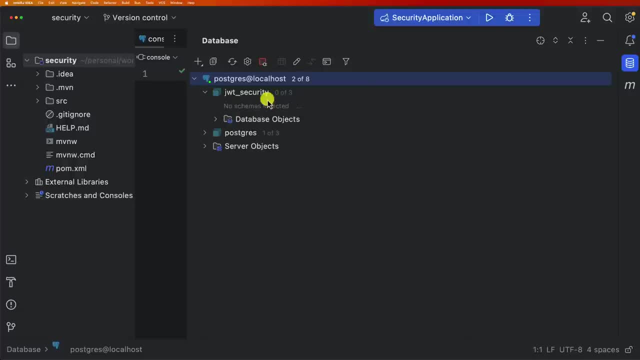 Okay, So open it in here and here we can see that. Okay, We have zero of three schemas. Just select the public one, because this is the one we need And this is where we will find all our tables once we create them. 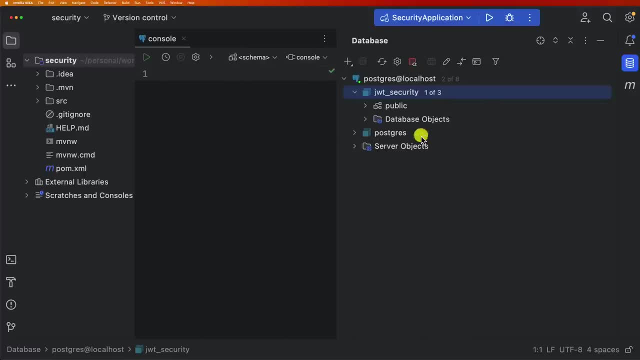 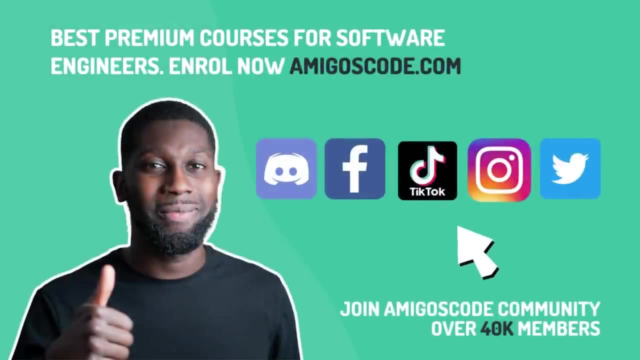 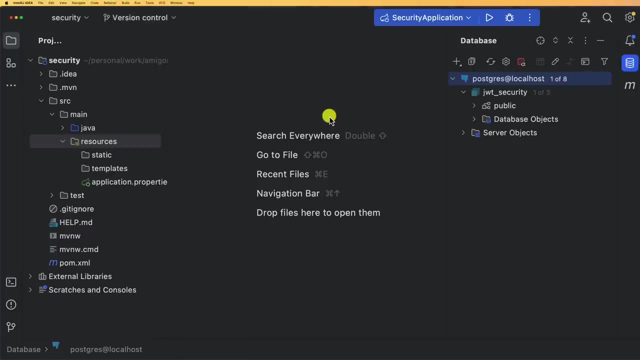 So now we have our data source available, Let's move on to the next step. Now let's establish a connection between our application and the database we just created. So the first thing to do is go here to this application properties and rename it and use the representation YAML. 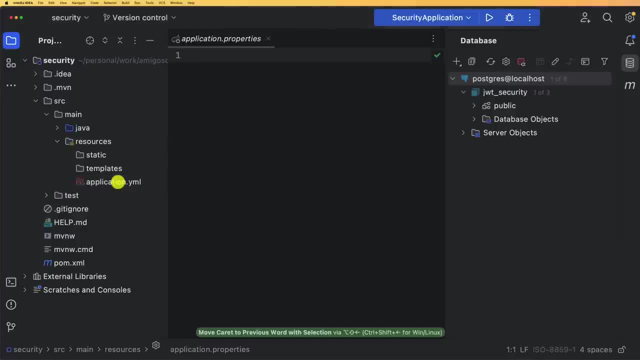 Okay, So this is what I prefer personally, and you can keep properties if you want to. but to better follow this tutorial, it's better to transform it to YAML. So in order to connect to a database, we need to provide a bunch of properties right here. 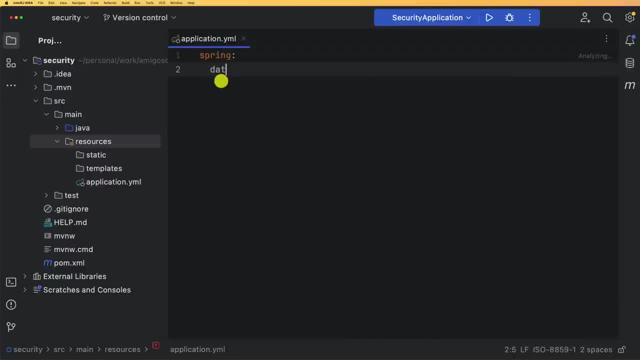 So we will start with spring And then data source, And one of the things that we need to provide at first is the URL, And this one is the URL, or the connection string to our database. If you don't know it, just go here to this database, click on it. 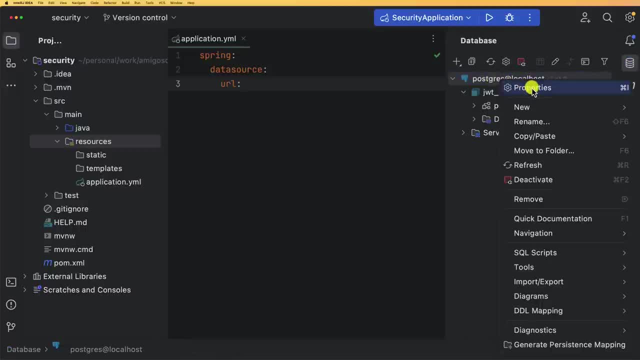 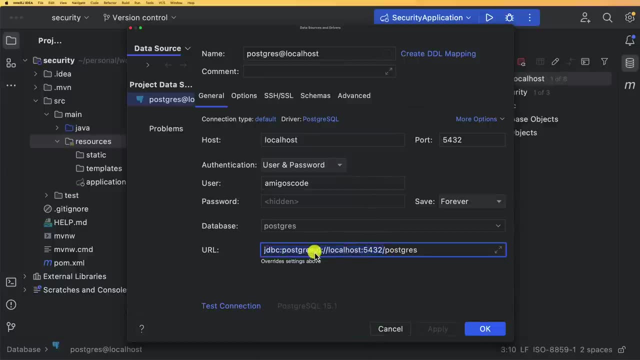 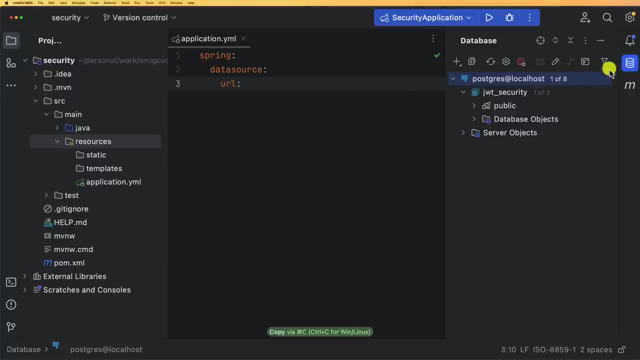 right click on the connection you just created properties and you copy this one. You copy this part right here, It's gdbc//sql, and then the address port, slash the database. So let me close this. I will paste this one and make sure here. 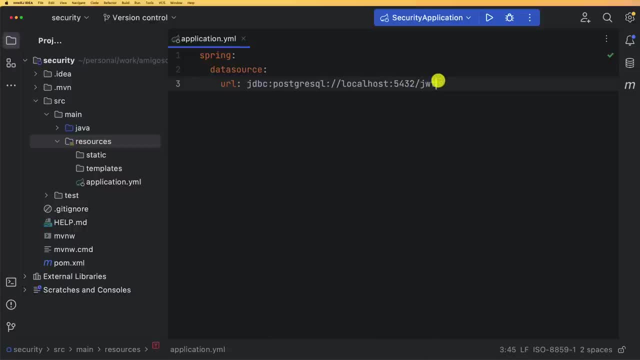 you write the correct database name, So for us we call it JWT security. Now we need to provide the username and password. Okay, So for my case it's empty. Make sure you provide the correct one, And here it's password. 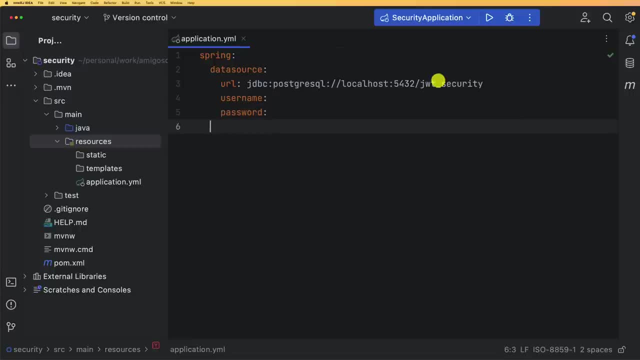 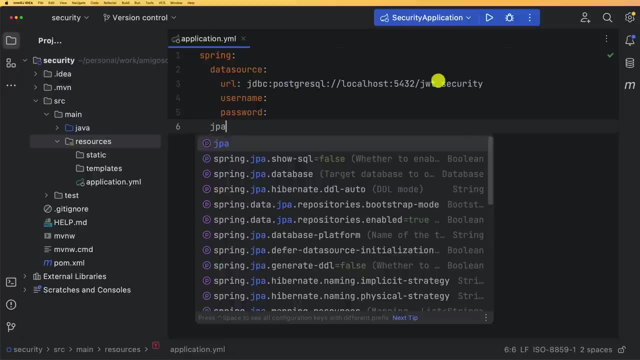 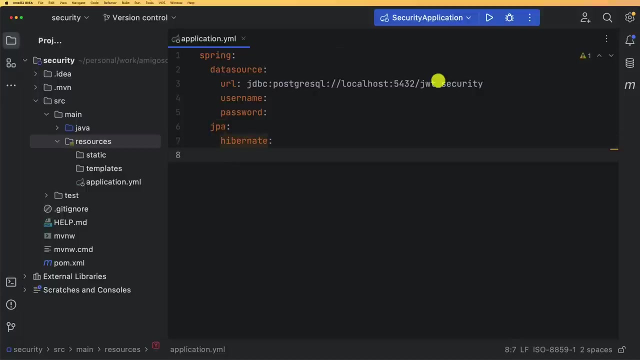 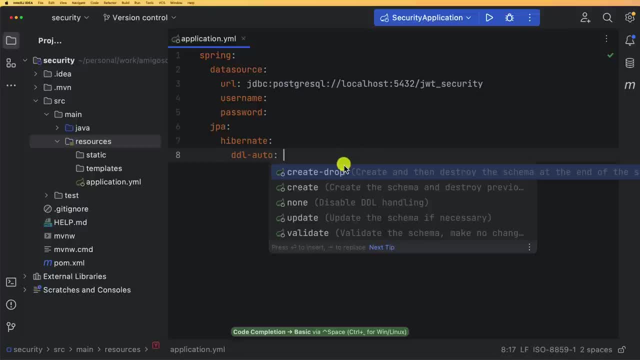 Oh, I have DDL auto And here we have a bench of Options. So we have create, drop, create non update and validate. So I will be using the first one, because every time I want to start the application, I want to create a new database, a new schema. 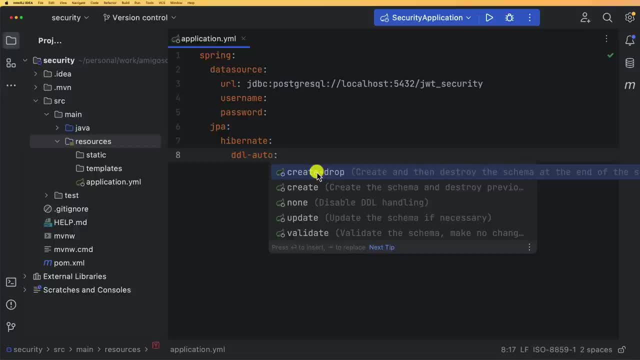 And when I stopped the application, I want to destroy it. Okay, So I always want to start with empty database, Alright. So the next one within JP uh, within JPS, or understands jpacom, like you see, now you need to really pay attention about the indentation right here, because this one 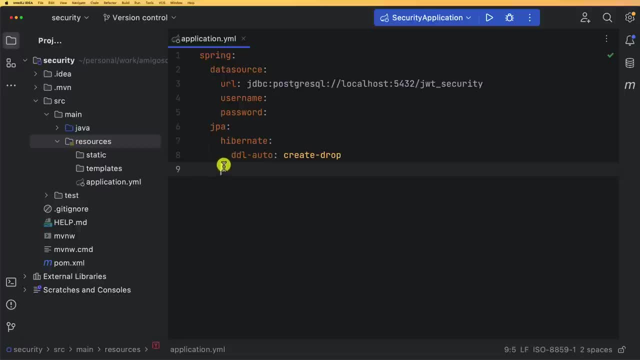 this tdl auto is part of the hibernate and the one i will write right now is part of jpa, so it's spring jpa and then show sql. i want to show sql when. when we perform, or when spring data jpa performs a query, i want to see that query. okay, i want also to add some other properties, so here: 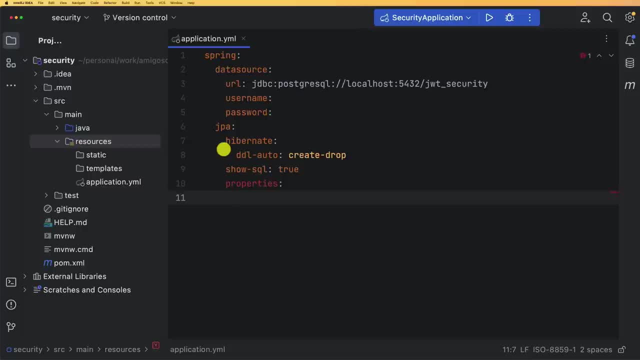 i will type properties and one of these properties, and here i have hibernate, and within this hibernate i want also to format the sql. so format sql- true, i want my queries to be formatted now, go back to the same level as properties and provide some information about the database. so 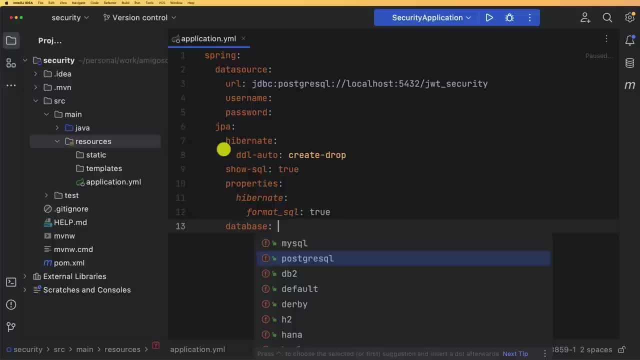 here we want to tell jpa which database we are using, and for this case we are using postgre sql- and then we can also provide the database platform that we are using and this will help spring performing and writing the better queries to to suit our postgre sql database. so for this one it's 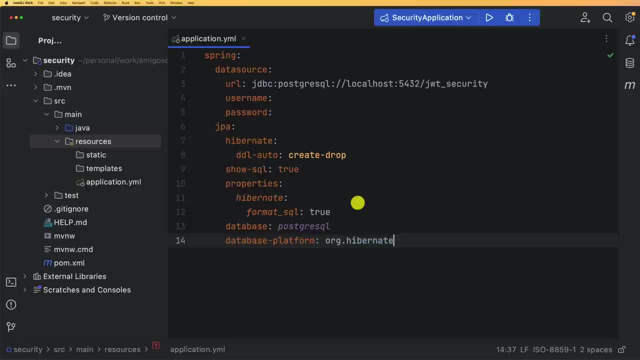 orghibernatejpg. Alright, and here we just forgot one property right here, which is the driver class name. So this will help Spring to detect or use the best driver class name, And here we are using PostgreSQL, so IntelliJ will automatically propose it to you. otherwise, 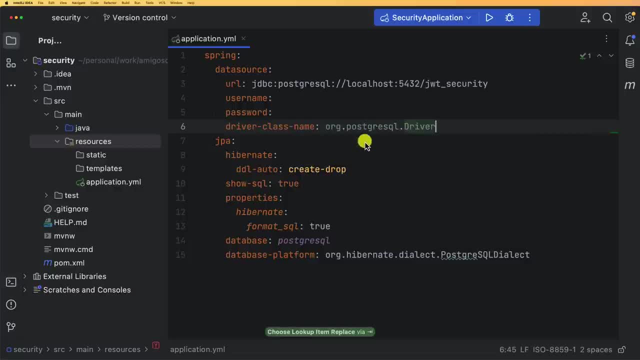 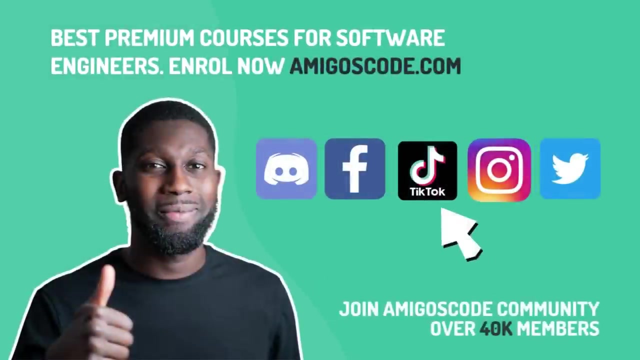 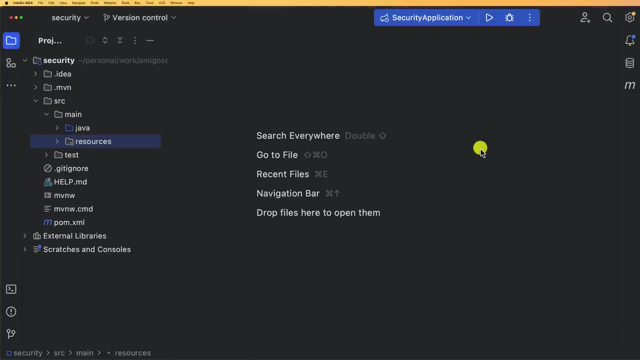 it's the orgpostgreSQLdriver and this is the one that we got from the PostgreSQL driver dependency. All right, so that's it about this configuration. Let's move on and start implementing our security. When we talk about authorization and authentication, we mainly talk about users. 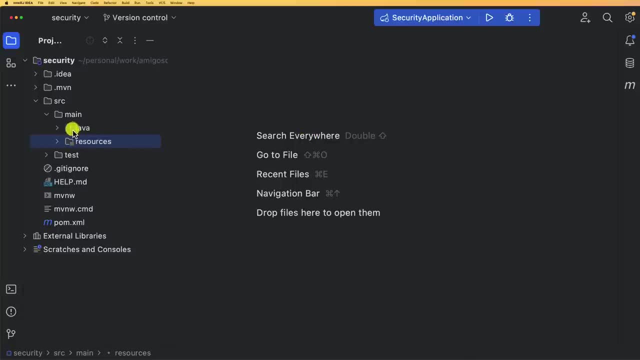 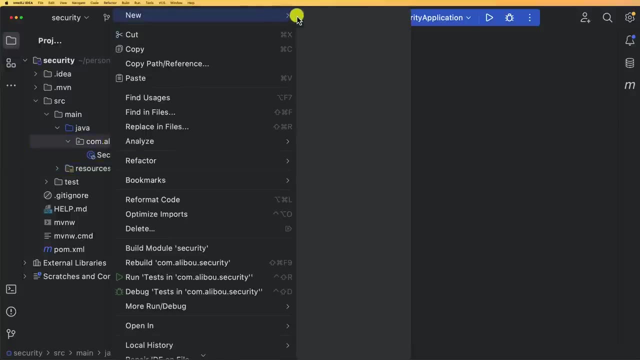 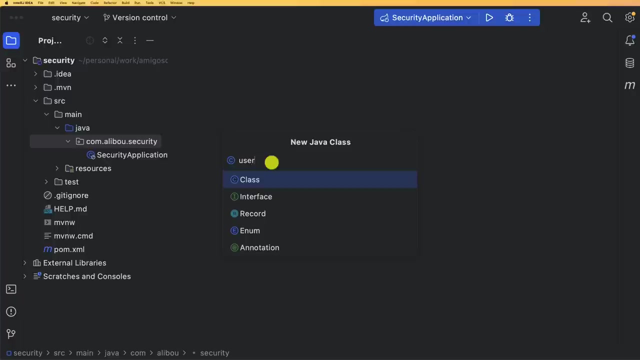 So let's go ahead and create our user class. So within the Java package and within the main package that we have right here, right click and new class, and here we can create a package and a class at the same time. So the package I will call it user and here I will just call the class user. 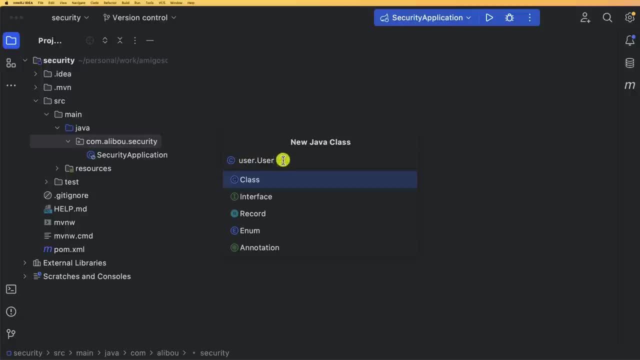 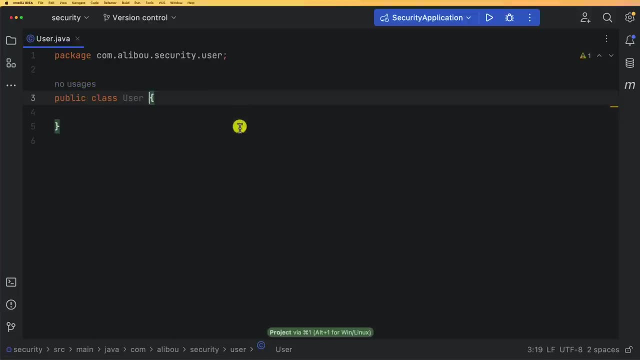 So useruser will create a package user and inside of it it will create a class user. All right, So this is our user, The user class. let me make this one full screen, And now I want to write a bunch of properties within this class. okay, 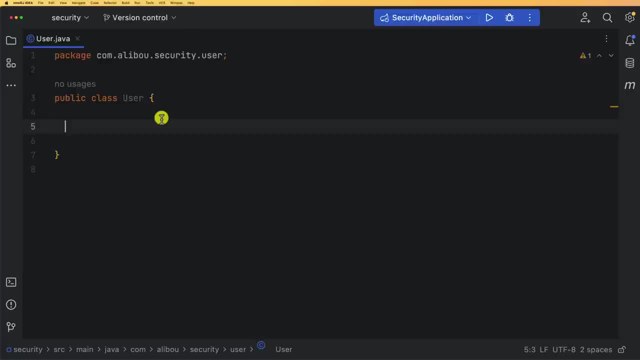 So my user has the following characteristics or the following fields: So first of all I want to have an integer ID and then I want to have a string- first name, and private string, last name, And also, of course, we need an email and password for this user to be able to authenticate. 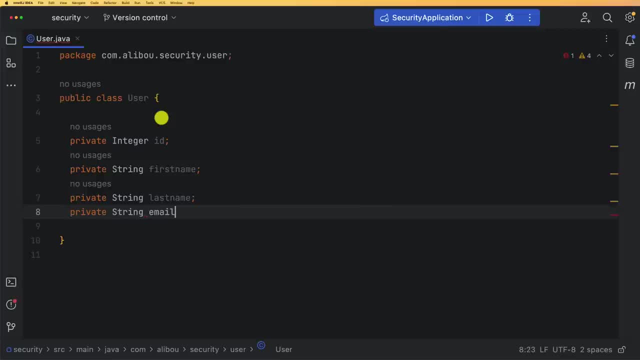 and connect to our application. So here I will add email and also private string password. So these are the information about our user. Now I will add a bunch of Lombok annotations in order to reduce the boilerplate, because you know, When we create a class we need getters and setters. 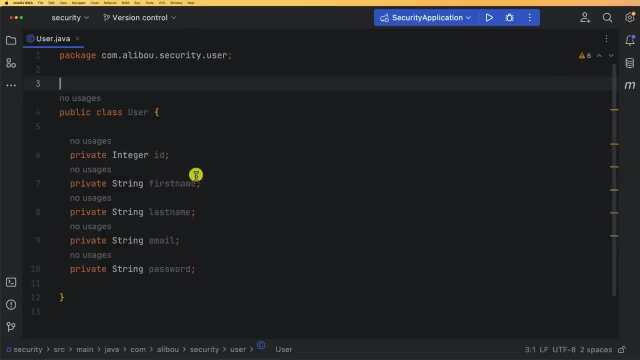 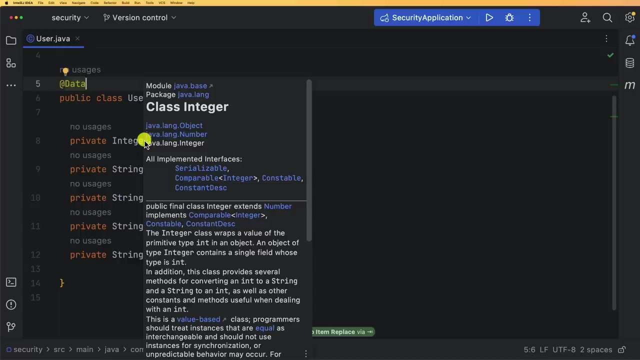 We need constructors, We need also the design pattern builder to build, to be able to easily build our object, and so on and so forth. So let's start with that. So we will need the date annotation and this annotation will provide us with the equivalent. 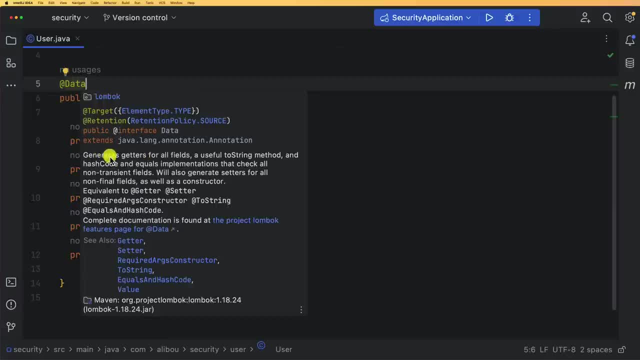 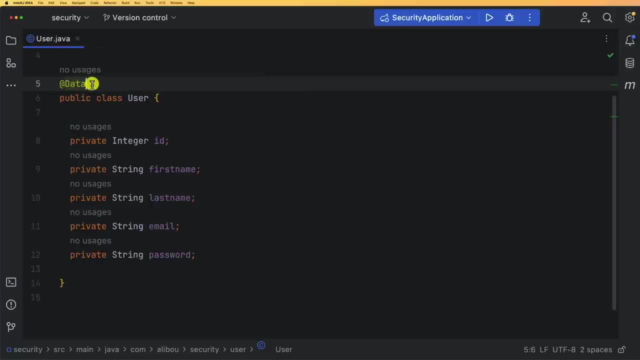 of getter setter, as you can see here. So it generates getters for all fields for useful method methods. So it's the equivalent to the getter setter required as constructor to string and equals and hash code. Okay, Also, I want to use the builder annotation. 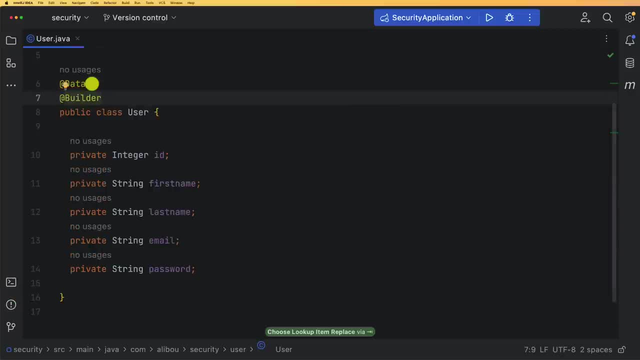 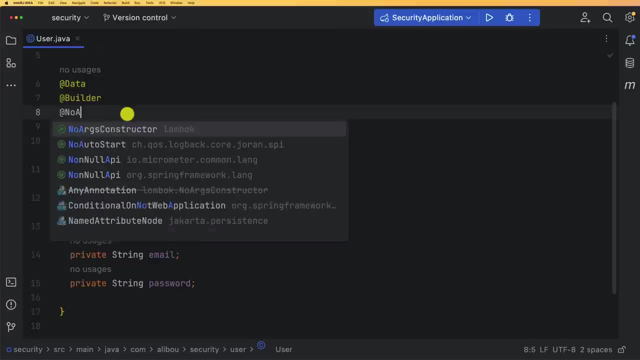 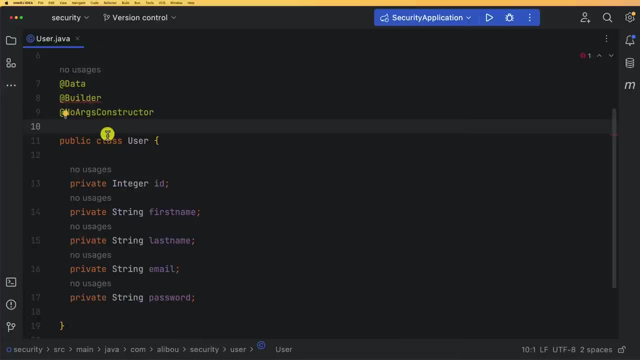 So this builder annotation will help me build my object in an easy way using the design pattern builder. Okay, And also I will need the no args constructor and, of course, when we talk about design pattern builder, We need always the all construct, the args constructor. 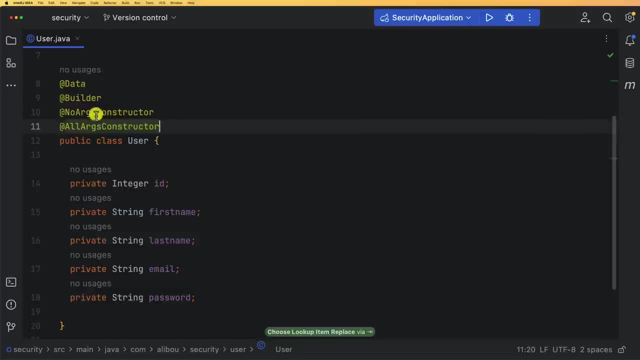 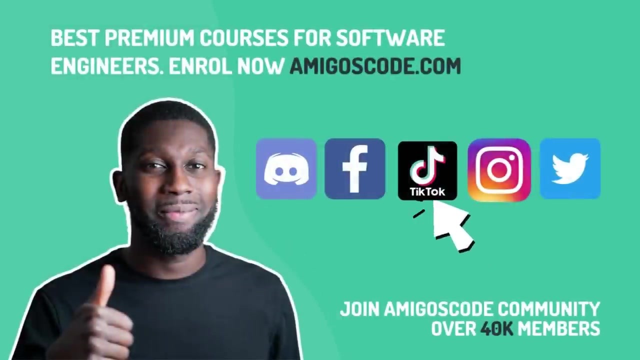 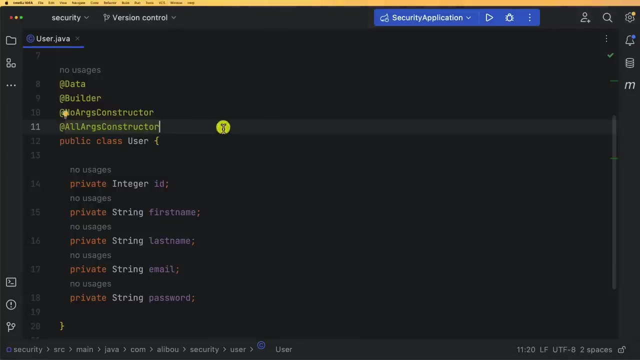 Okay, So let's add this one and, like this, we have our, we have our user class. Now let's make this user class an entity. To make this user class an entity, So the first thing We need to add is this entity annotation. 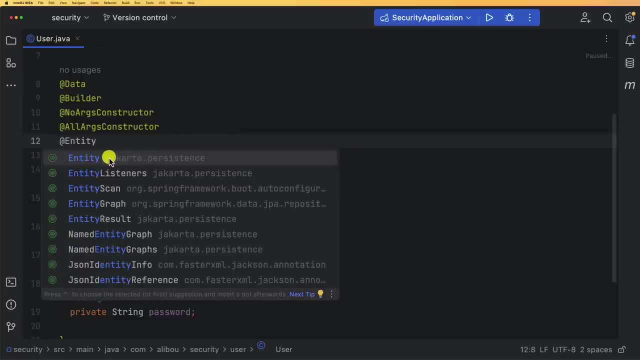 And since we are using the spring boot three dot zero here, make sure that the package is Jakarta dot persistence and it's no longer Java X dot persistence. So this also will help you tell if you are using the correct version of spring boot. Okay, 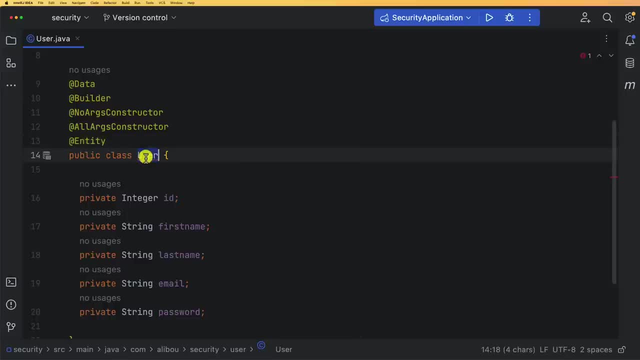 So here we need the entity annotation and because this user name, this user class is already reserved for post degree SQL, Because post degree SQL already has a table called user, So we cannot create a second table called user, I will use the table annotation right here, because you know the table annotation. 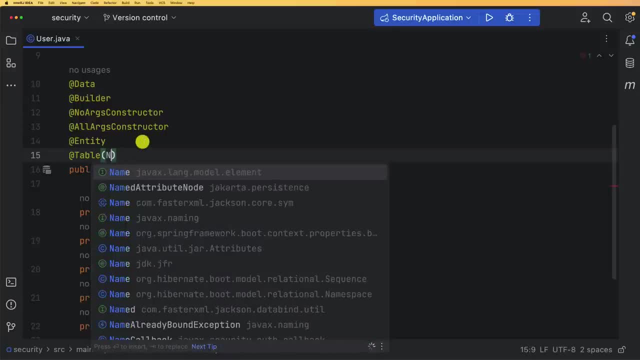 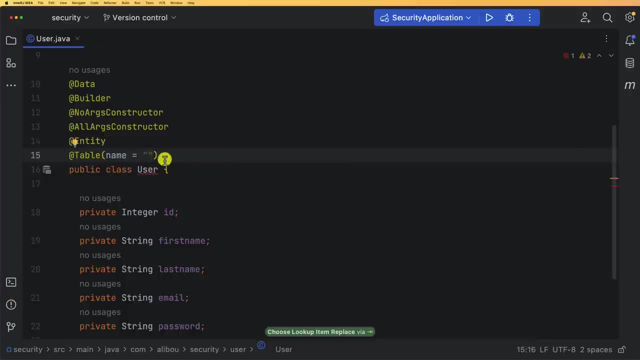 If I do not provide, if I don't provide any name right here, it will take the entity or the class name as a default name for the table. Okay, But here I want just to call it underscore user to avoid this. Okay, So let's call it underscore user. 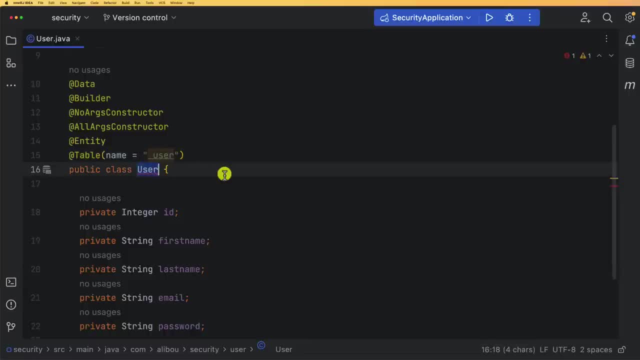 So let's call it underscore user to avoid this ambiguity between this user class and the one with um and the one with post degree SQL. So now this is kind of sufficient to tell that this user class now is an entity. but we still need to provide one small information. 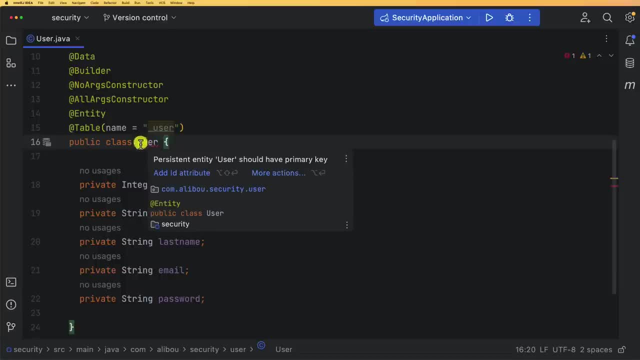 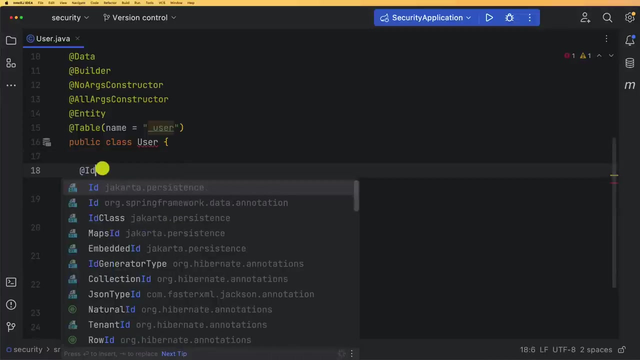 Okay, So here we have this error. right here We see that this persistence entity user should have a primary key. Okay, So we need to add an add An ID attribute, which we already have right here, but we still missing this ID annotation. 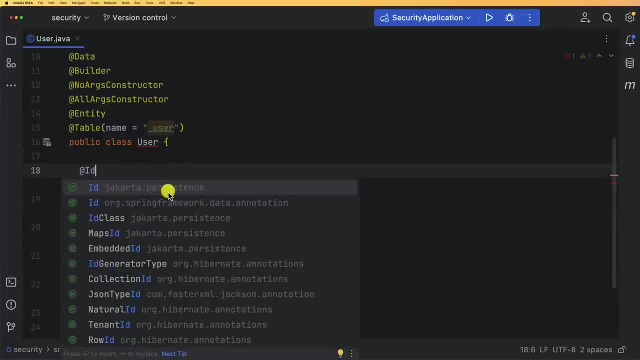 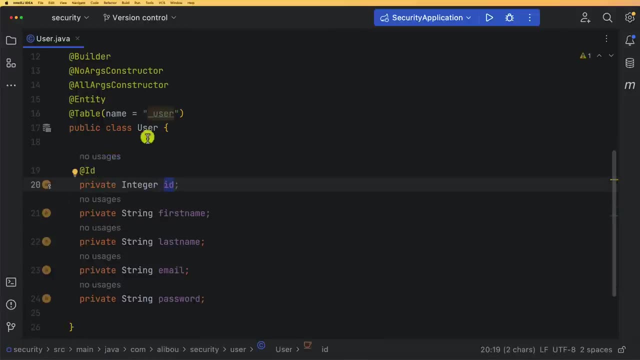 So this ID annotation: it's coming from the Jakarta dot persistence and it's telling that this ID is the unique identifier of this user class. Now I want also this ID to be auto incremented or auto generated, So every time I want to create user, I don't need to provide this ID. 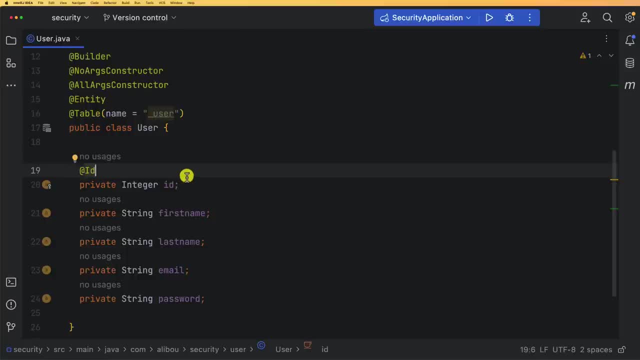 And every time this ID is null, I want it to be auto incremented by the system or by spring data JPA itself. So to do so and to make it in an easy way, I will use the annotation generated value. Okay, So this generated value, it will make this ID or this object auto generated, using whether. 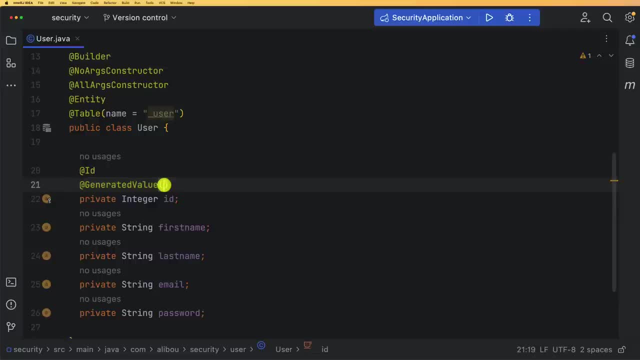 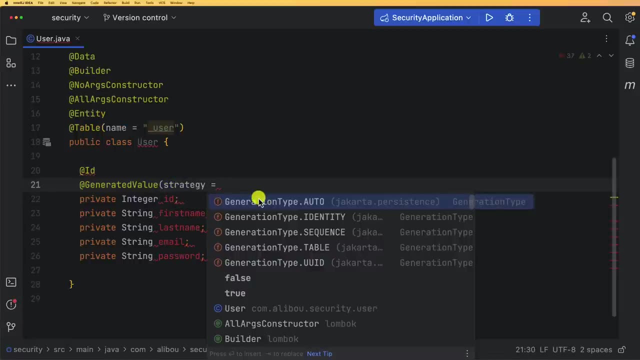 a sequence, a table and so on and so forth, And we call this a strategy. Okay, So for this strategy we have, we have several options. Okay, We have auto identity sequence table and you UI ID, So the auto is the default value. identity means that it will use an identity number. 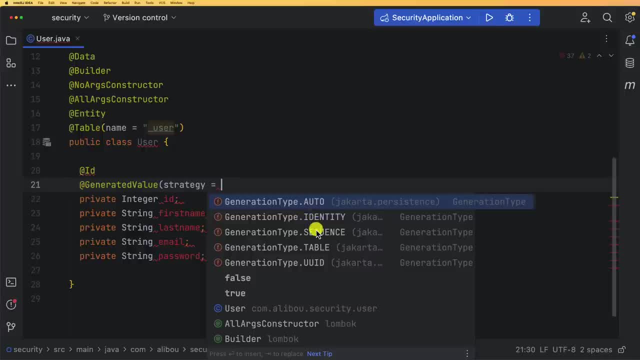 like an auto increment sequence means that we will create a sequence within our database and use this sequence to increment each time the value of the ID. Okay, So the table: this means that we will create a table and the database and we will call. 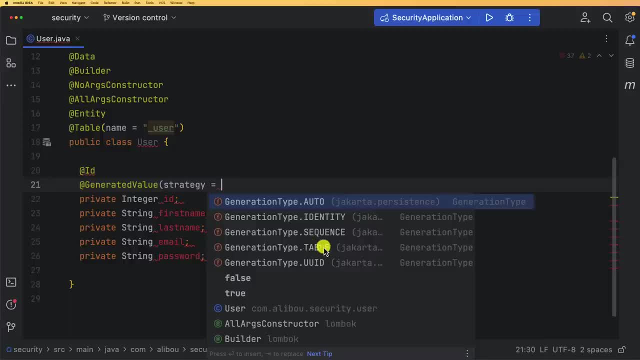 it by default. it's called hibernate sequence And this table will always be requested and queried by a spring data JPA to get the last value and incremented for the last one, The UU ID is using this one. I think you know it from uh, from the Java, Java utilities. but uh, if you leave it to. 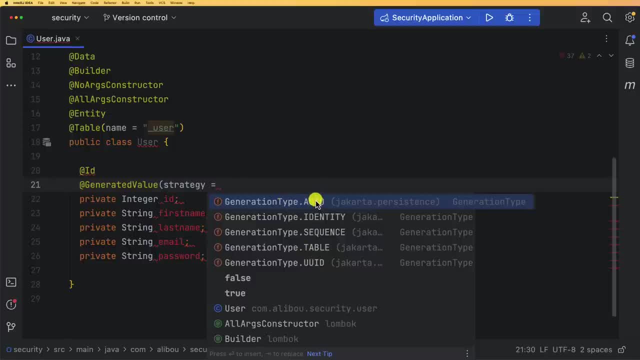 auto. If you leave the generation type to auto hibernate, we'll try to detect the best suitable option for you. For example, if we are using post-degree SQL, it will pick by default sequence. If you are using my SQL, for example, it will pick table, because my SQL does not work with. 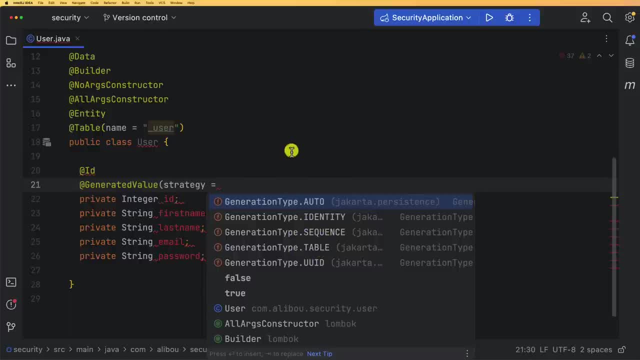 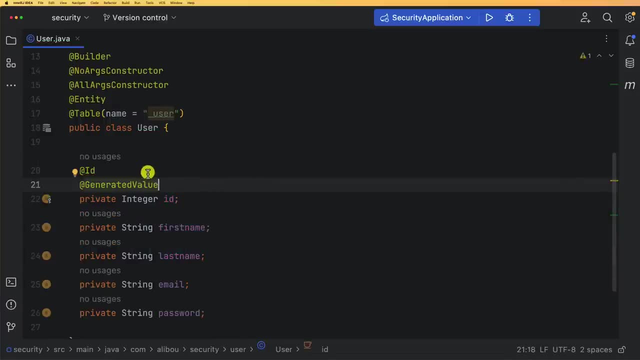 sequences. So it will. it will pick table for that. So for the moment I will just keep it empty like this, because, as I mentioned, the default value is auto, So it will be automatically detected. Okay, So now we have our entity. 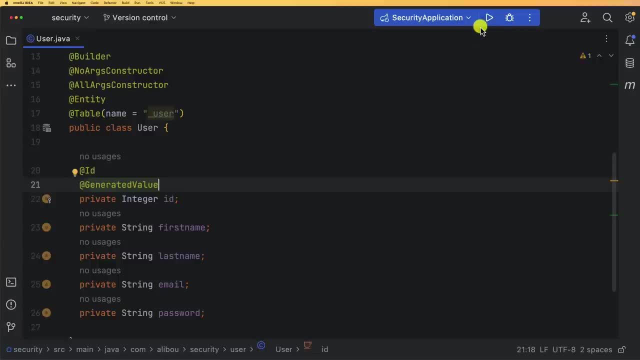 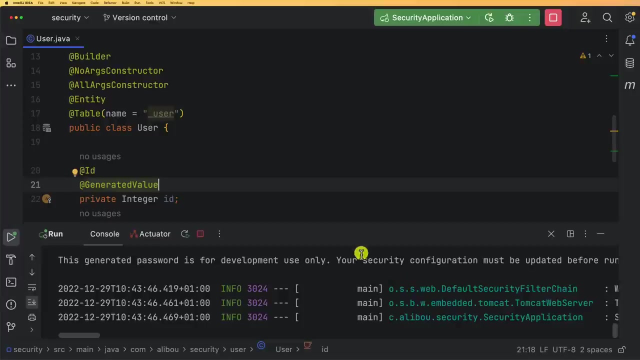 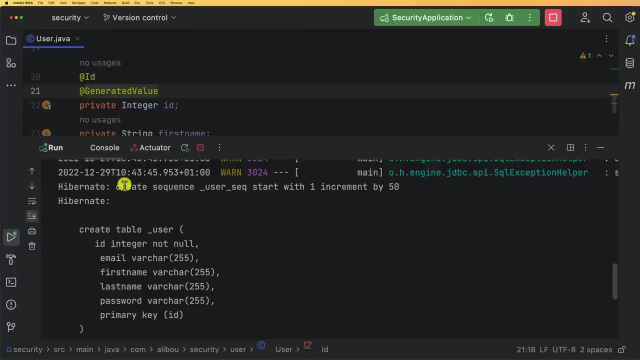 Let's try to start the application and make sure that we have our table created within the database Here enable the annotation processing for Lombok. And now we have our application started, Let's have a look quickly on the logs And here I will just show you how to create sequence. 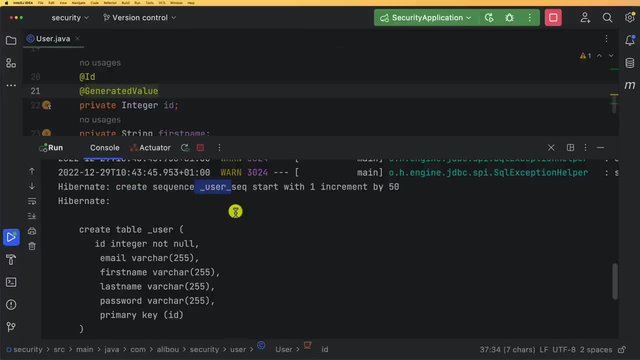 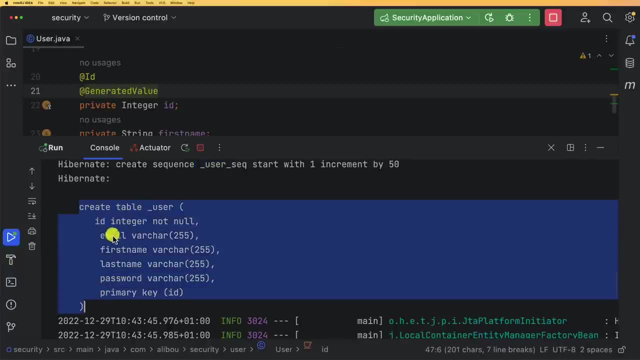 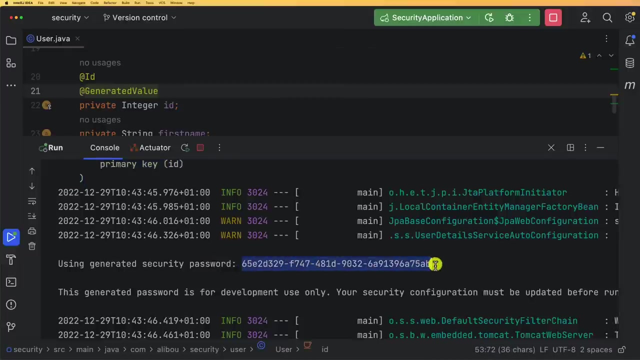 User sequence start with one increment by 50.. This is automatically generated, as I've mentioned, And here we see the SQL that we have: create table user with an ID, email and so on and so forth. Okay, And here we have spring. security is auto generating a security password, and this one we will see. 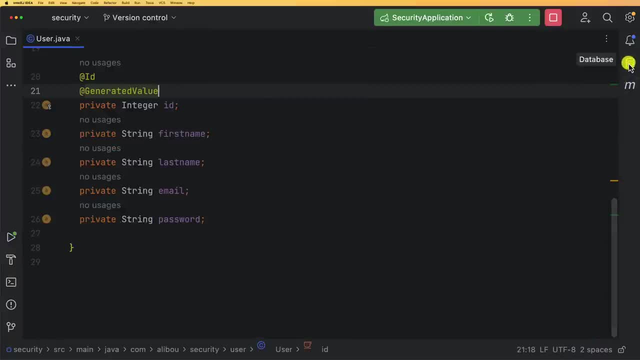 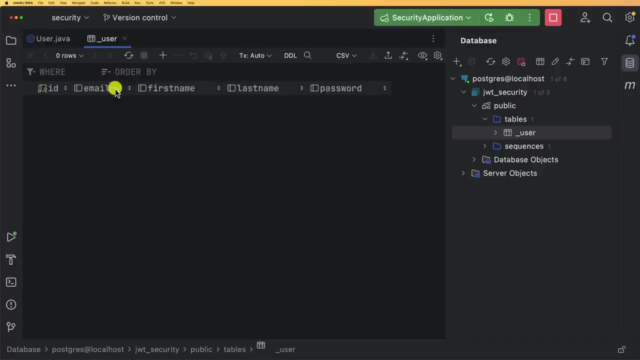 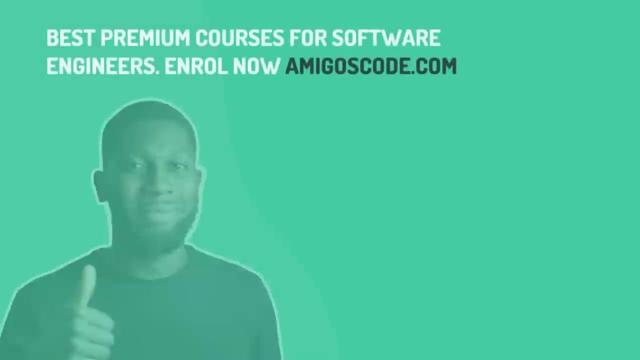 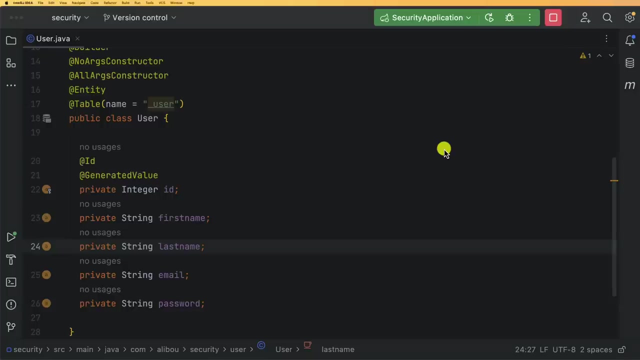 later on. Okay, So also, if you want to check, you can open your database right here. click on this one refresh And within the public schema, we see that we have this user table right here and if we open it we will see the ID or the attributes that we already provided. 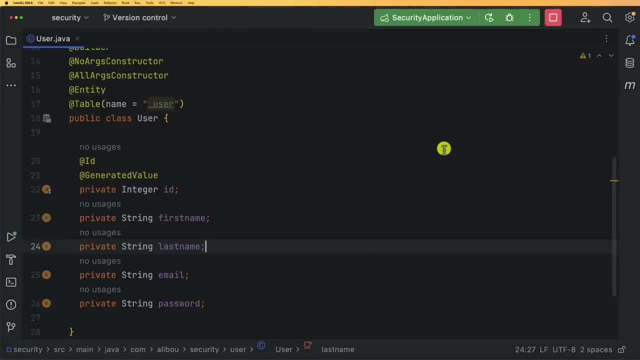 When Spring Security starts and set up the application, it will use an object called user details, and this user details is an interface that contains a bunch of methods, And each time you want to work with Spring Security, you need to ensure that you are providing this user details object in order to make Spring Security life easy to use. 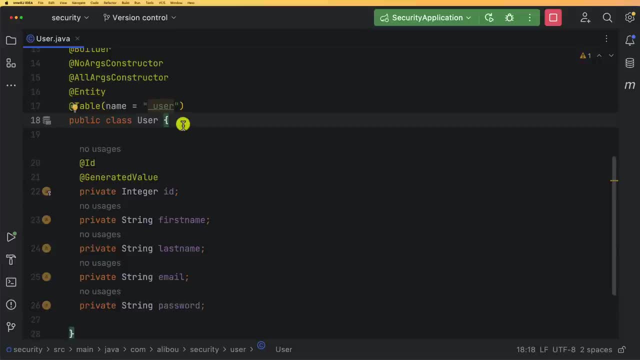 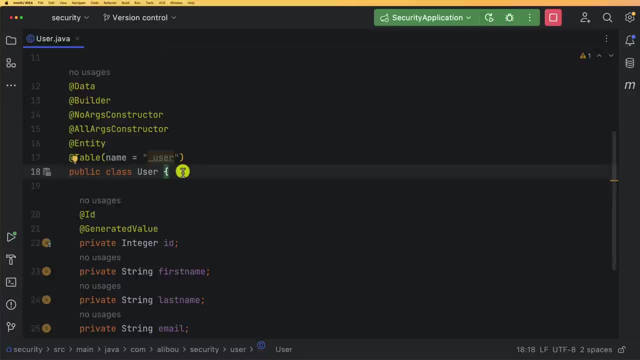 So to do this For us, for our user, I recommend this way. So every time you have a user, think always to make it or to implement the user details interface, So, like that, your user or your application user is already a Spring user, if we may say. 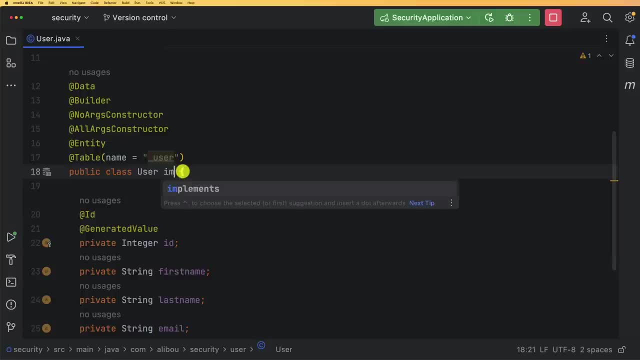 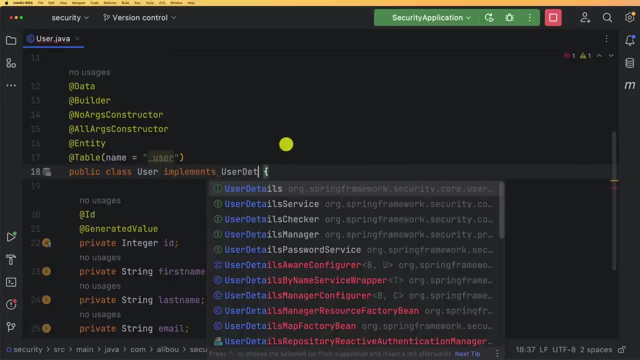 so. So to do that, just go ahead to this user class that we created and implement an interface called user details And this user details. It's from the package orgSpringFrameworkSecurityCoreUserDetails. OK, click here and now it will ask us to implement. 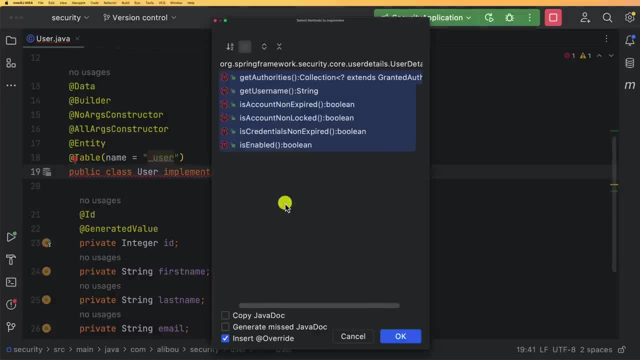 a bunch of method. So click on this one implement method and we see right here that these are the methods that we want or that we need to auto generate. OK, not auto generate, but we need to implement. So it's: get authorities username And we have this Boolean. 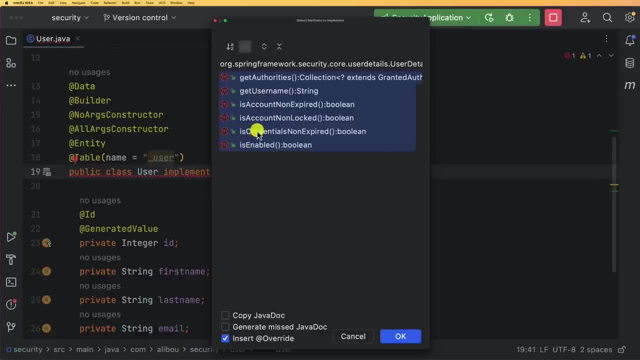 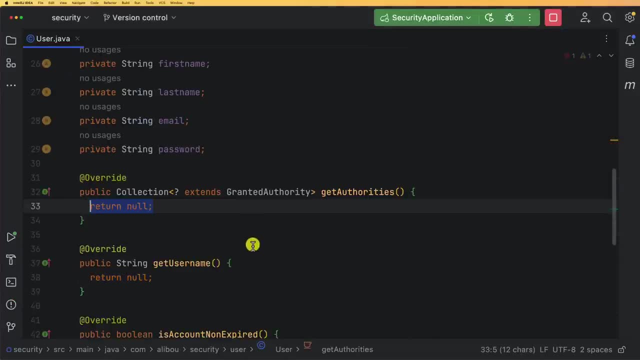 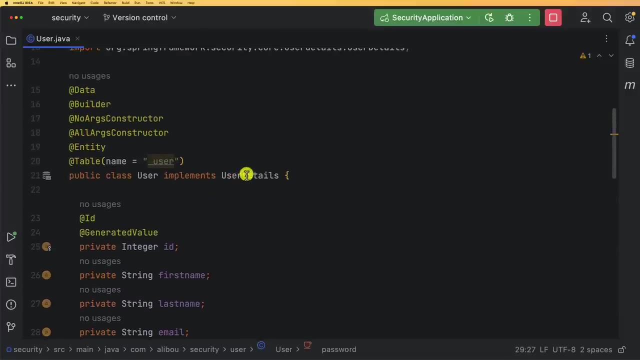 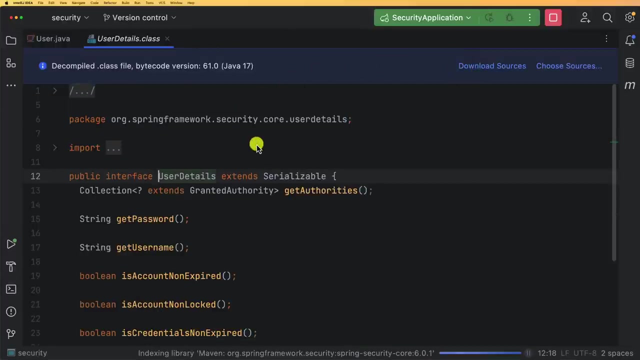 Methods: account expired, locked, and so on and so forth. OK, so just go ahead, click OK and we will see how to override. But before that I want to go a bit a bit more into details about this user details interface, So I will open the definition, download the source so we can easily see it. 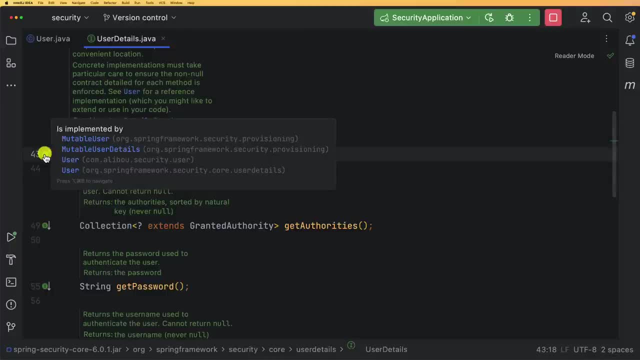 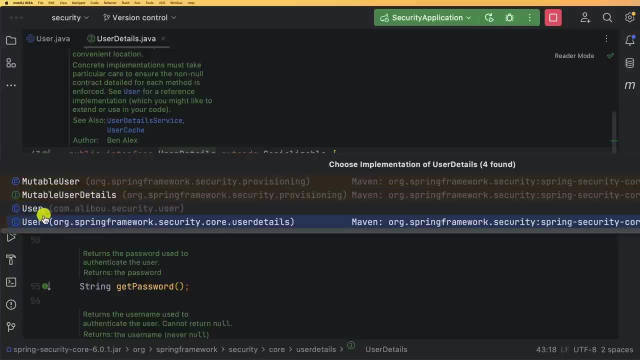 So here, if I click on this icon right here to see all the implementation Of this interface, we have this mutable user, mutable user details and so on and so forth, And also we have our user class, the one that we created, And we can see also that we have this user from Spring FrameworkSecurityCoreUserDetails. 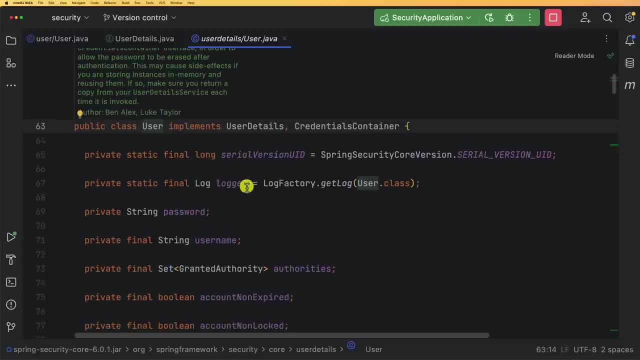 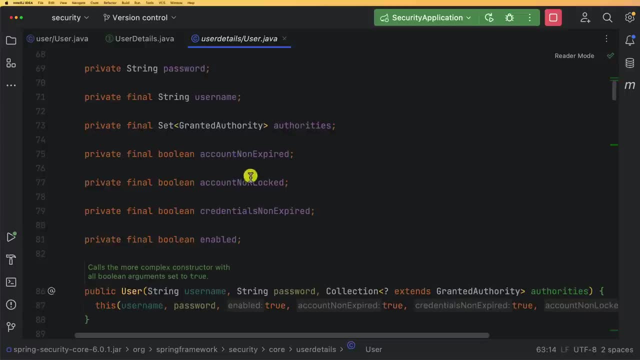 and let's have a look on this one. OK, So this user detail contains the user name, password authorities and the bench of Booleans. the account expired, locked, non-expert And in this case, We will see that we have this user account expired and we have the user address in this. 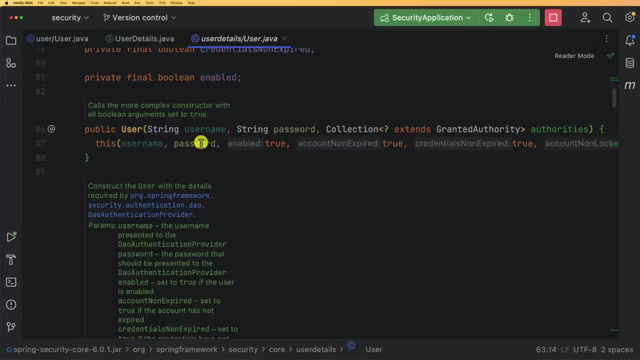 case, And we have the user data And then we have the user address in the account. So we have the user data. The user data here is the user name password, So we can see this user account expired or not, And this information or these: 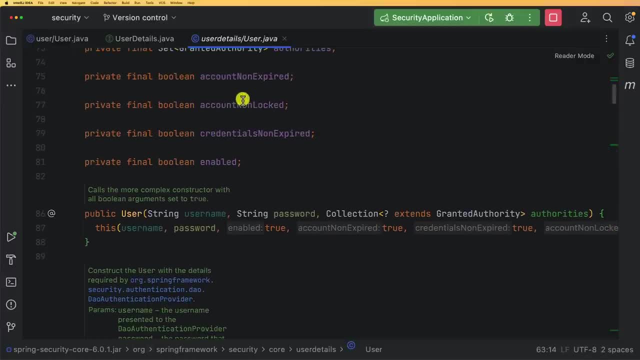 These attributes spring will use automatically To Play with authorization and authentication and, for example, if we can rely on this account non expired, If we want to have some expiring dates or use, the user can expire. and also if we want to lock and unlock the user. 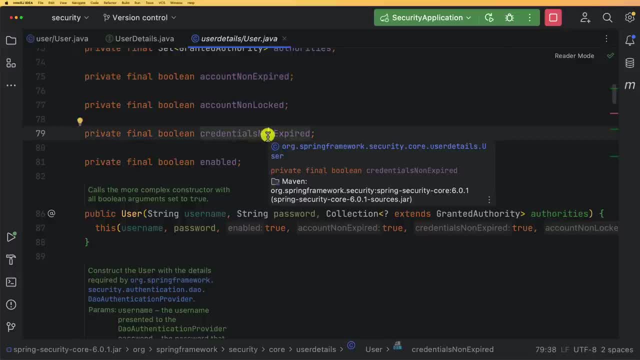 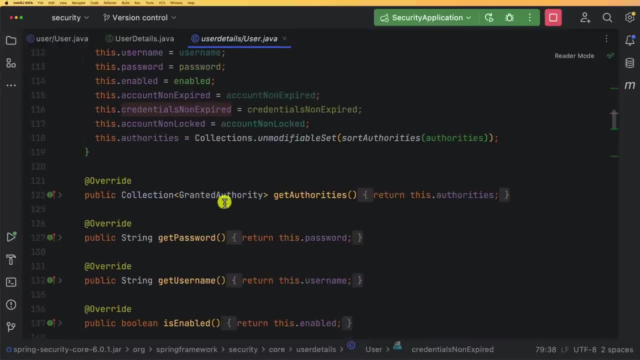 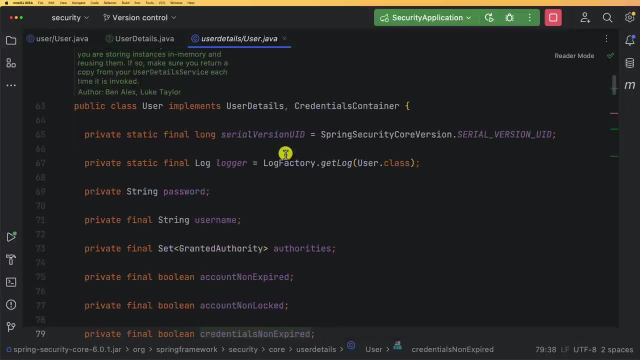 or the same, if we want to work with credentials and so and so forth. okay, so i will. i will give you the time to play and check this and here we see that we have a bunch of constructor and we have these methods that they need to be overridden right here. okay, so here we see that this user 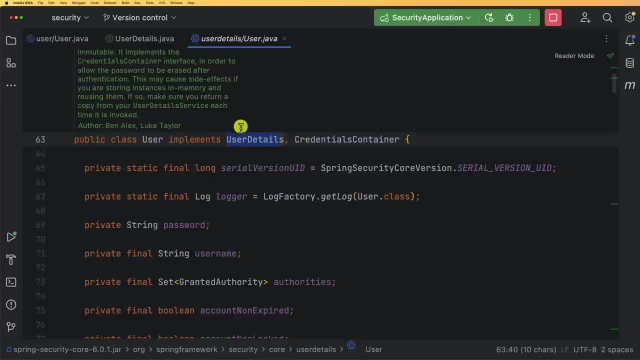 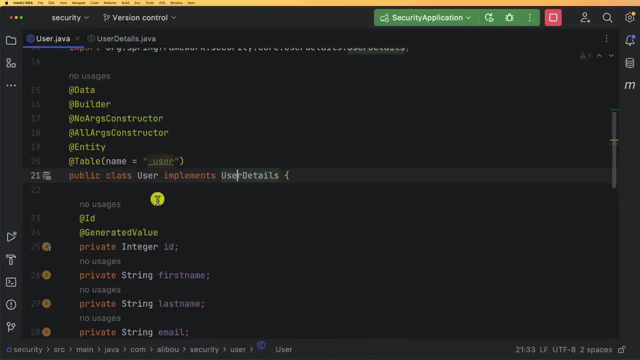 already implements user details. so for you you have two options: whether you implement this user details interface within your user class or you can create, for example, a user, you call it app user and then extend the user, the one from spring boot. so it will be the same, but for me i want always to. 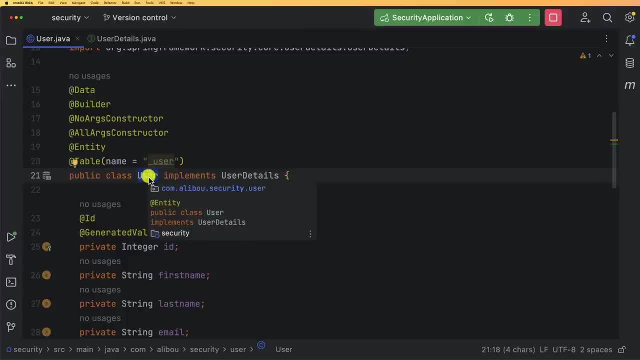 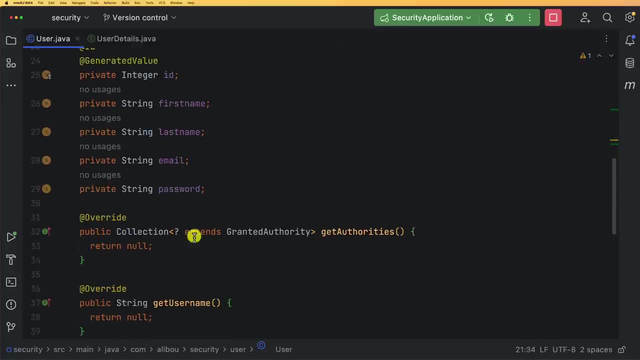 have control over my object, so i create my own user class and implement user details. so now let's go ahead and implement these methods. okay, so here. the first one is we need to provide a call to the user detail to be a user user class. we have this function called user details, and so 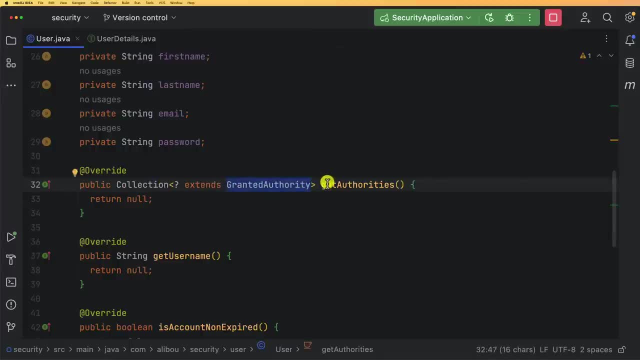 collection of granted authorities, and already the method is called get authorities. so this get authorities will return or should return. a list of roles like. let me explain it like that: when we talk about roles, so here we need to add a role. okay, so i will do, or i will create a role and 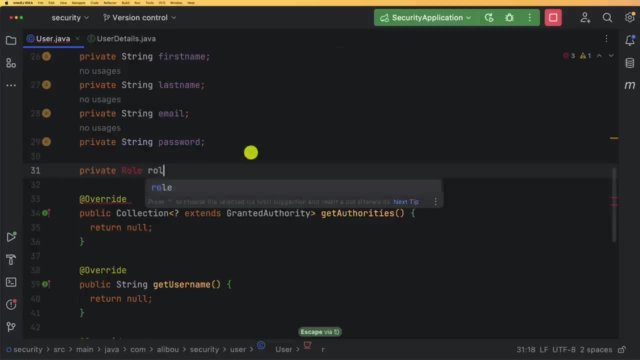 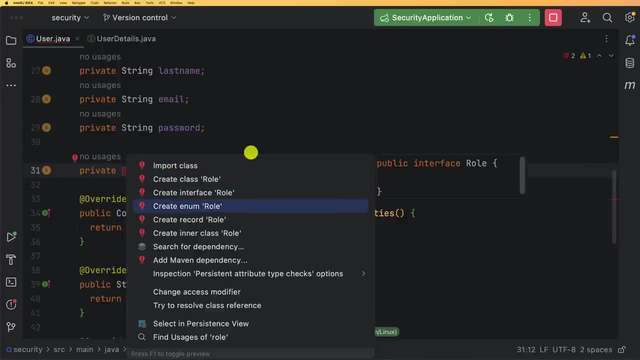 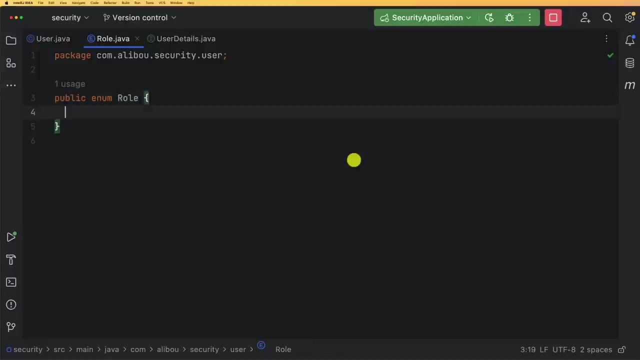 this one. it will. i will create an enum for it and i will call it role and this: let's create this class and here you can choose the option create enum, role, hit, okay, and we want to create it within the same package and within this role. it's so easy, i will just user and admin, okay. so we, we want to. 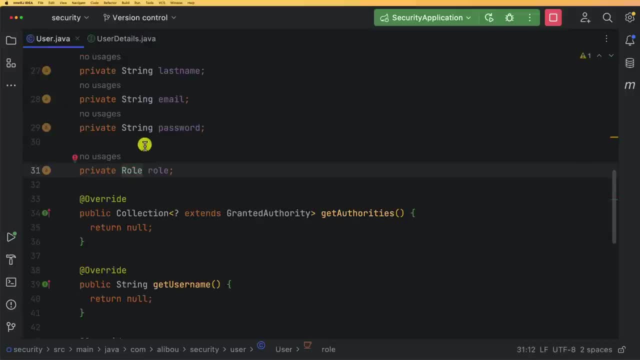 have only two roles within our application. so now we have this role and, because it's an enum, we need to create an enum for it, and we need to create an enum for it, and we need to create an enum for it and we need to add this enumerated annotation, and this enumerated annotation is to: 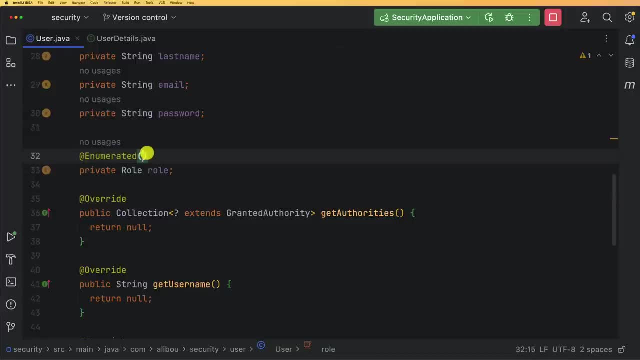 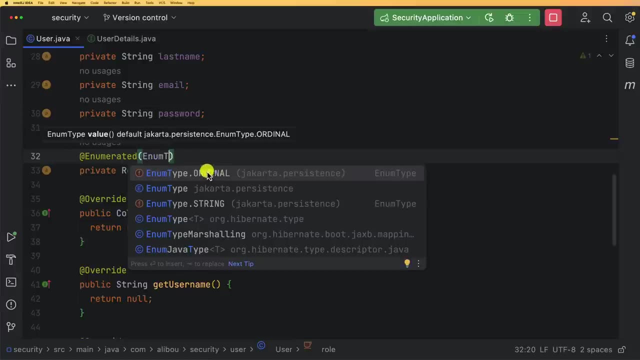 tell spring that this is an enum and we want to use it, whether the enum type: ordinal or string. so, by the way, by by default it's ordinal means it's 0, 1, 2 and so on, so forth. string, it will take the string value of, of the of the enum. okay, so let's go back to this again. 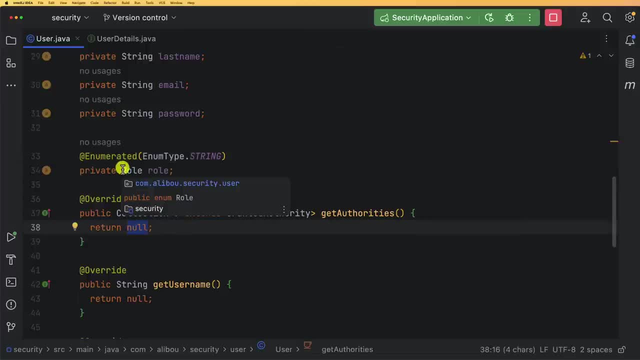 okay, so let's go back to this again. okay, so let's go back to this again: authorities so in here. because authorities so in here, because authorities so in here. because with our design we said or we decided with our design, we said or we decided with our design, we said or we decided that the user can have only 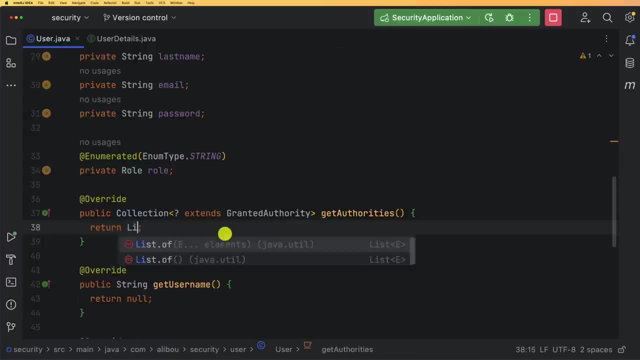 that the user can have, only that. the user can have only one role. so i will just return a list: one role. so i will just return a list, one role. so i will just return a list: dot off, dot off, dot off. and here i want to return a new. 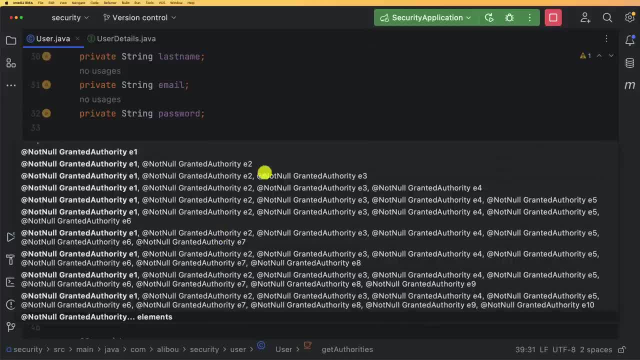 and here i want to return a new, and here i want to return a new: simple, simple, simple, granted authority. granted authority, granted authority, okay, so the object that i want to return, okay, so the object that i want to return, okay, so the object that i want to return is called simple, granted authority. 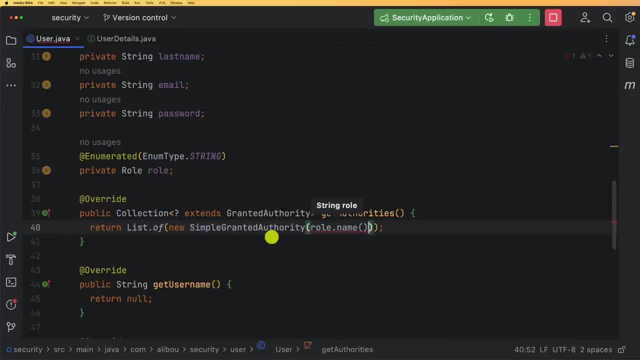 is called simple granted authority is called simple granted authority, and here i want to return the role dot and here i want to return the role dot and here i want to return the role dot. dot name. okay, so the role is referencing dot name. okay, so the role is referencing. 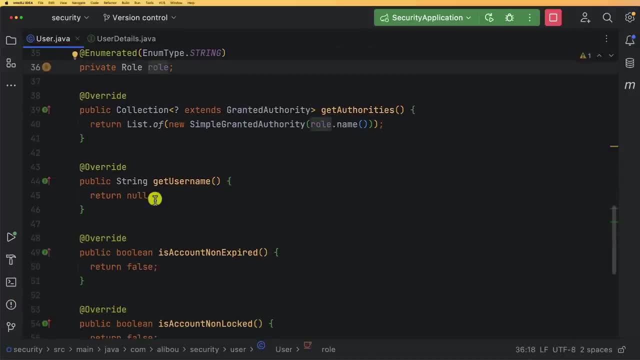 dot name. okay, so the role is referencing this role right here. this role, right here. this role right here. next one is this: get user name. so the next one is this: get user name. so the next one is this: get user name. so the username for us. username for us. 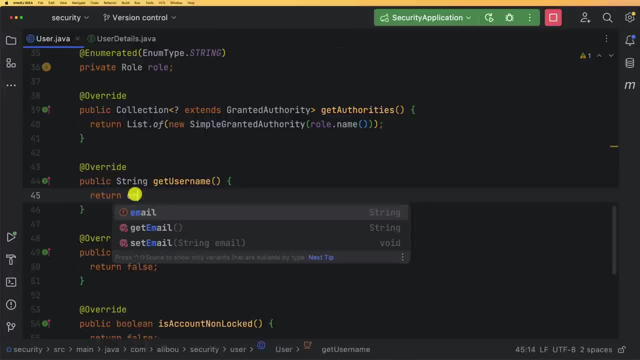 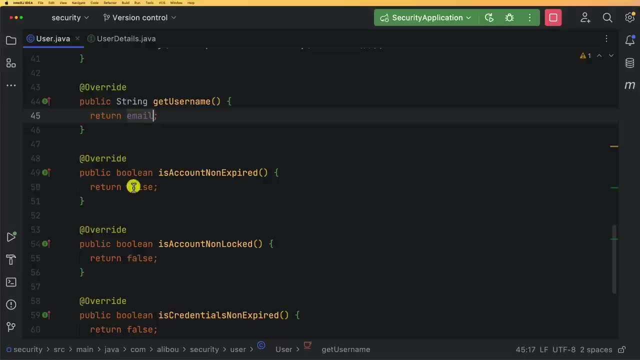 username for us. is our username, so it's the email. okay, is our username, so it's the email. okay, is our username, so it's the email. okay, then we have this account non-expired. then we have this account non-expired. then we have this account non-expired. so here we have. this is account. 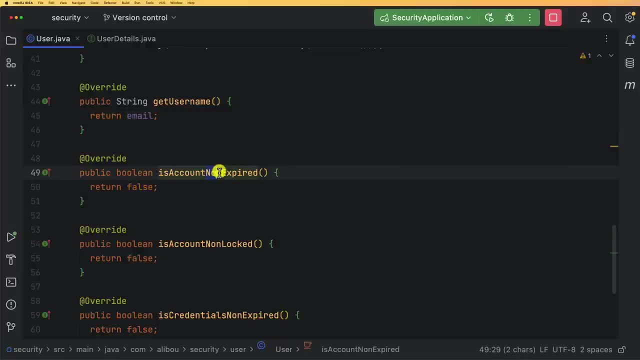 so here we have, this is account. so here we have, this is account, non-expired here, make sure, and be non-expired here, make sure, and be non-expired here, make sure, and be careful. it's non-expired false. this is careful. it's non-expired false. this is. 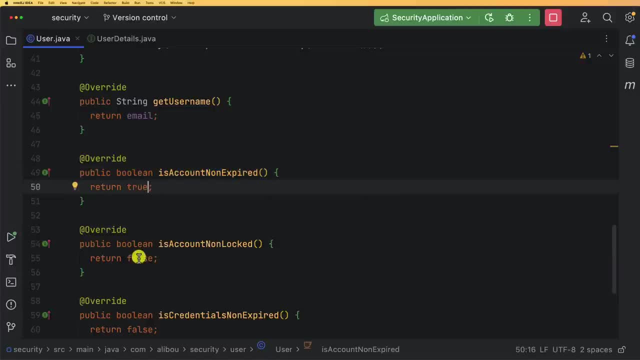 careful. it's non-expired, false. this is the negation. so the negation, so the negation. so non-expired should be true, otherwise we non-expired should be true. otherwise, we non-expired should be true, otherwise we will not be able to, will not be able to. 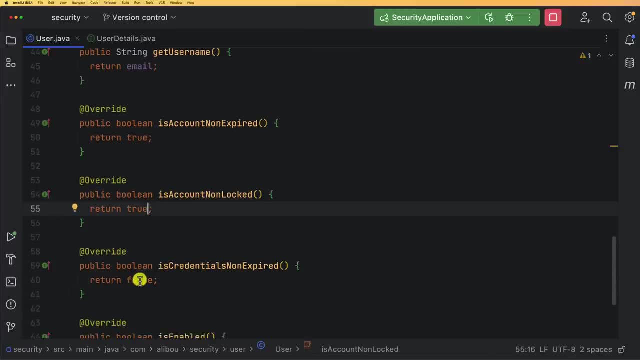 will not be able to connect our users so non expired. connect our users so non expired. connect our users so non expired. unlocked and unlocked and unlocked and non credential on expired and if the non credential on expired and if the non credential on expired and if the user is enabled. 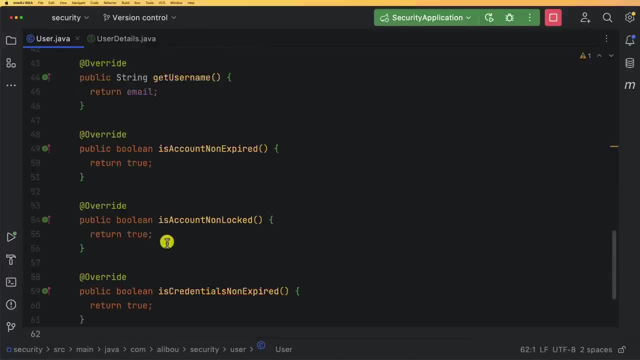 user is enabled. user is enabled: false. and here i want to make it true: false. and here i want to make it true: false. and here i want to make it true. here there is one thing that i need to here, there is one thing that i need to. 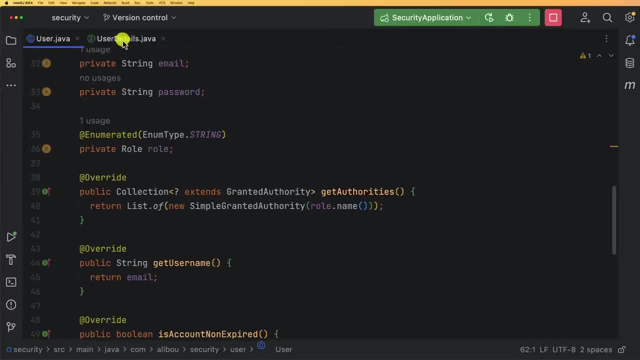 here. there is one thing that i need to mention right here, mention right here, mention right here. so, within this method, let's go back to so. within this method, let's go back to so. within this method, let's go back to this user details, this user details. 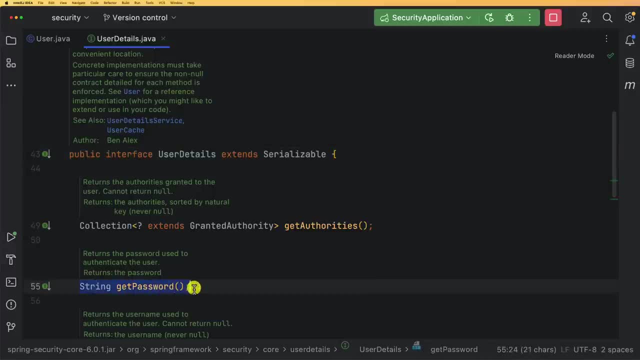 this user details interface. we see that we have this get interface. we see that we have this get interface. we see that we have this get password. okay, but this get password was password. okay, but this get password was password. okay, but this get password was not not. not, uh, was not overridden right here, because 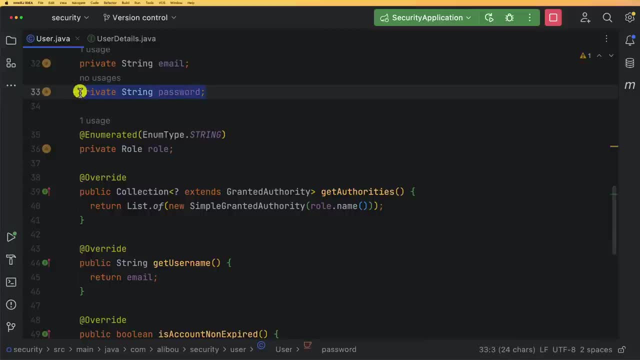 uh was not overridden right here because uh was not overridden right here because we have this string, we have this string, we have this string. password right here, password right here, because we have this string and we have the lombok and we have the lombok and we have the lombok annotation. so we have already a method. 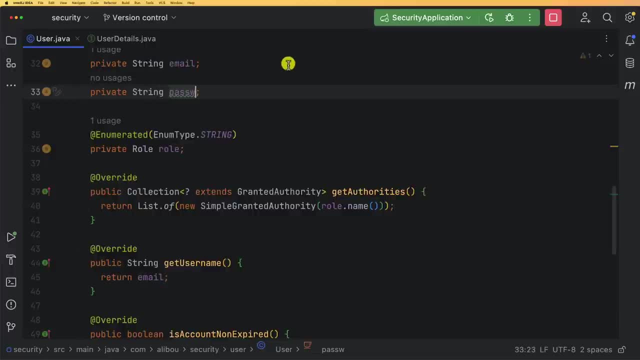 annotation. so we have already a method annotation. so we have already a method called get password. but here if i just called get password, but here if i just called get password, but here if i just name this one, we see that we will see. name this one, we see that we will see. 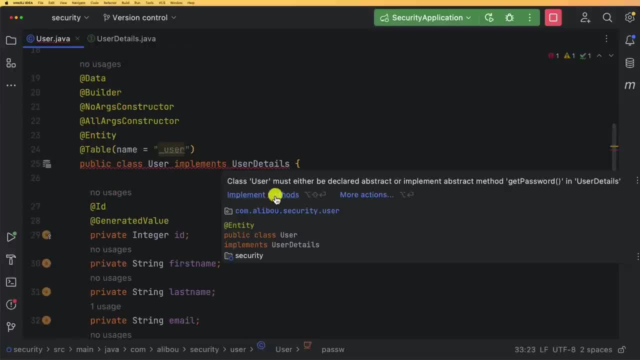 name this one. we see that, we will see that here. we will that here. we will that here. we will automatically tell that. we want to automatically tell that. we want to automatically tell that we want to override this method. okay, so let's override this method. okay, so let's. 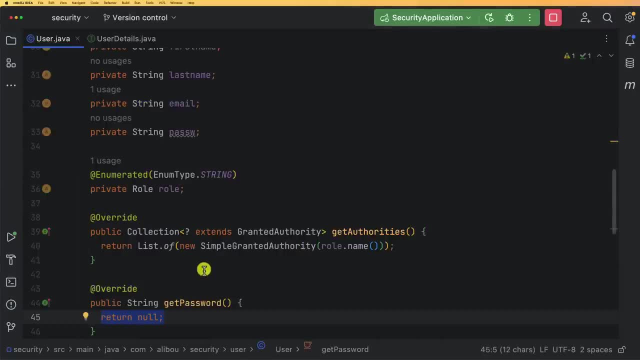 override this method. okay, so let's override it just to be. override it just to be. override it just to be to be more visible, or like better to be more visible, or like better to be more visible, or like better visible for you. i will rename this one. 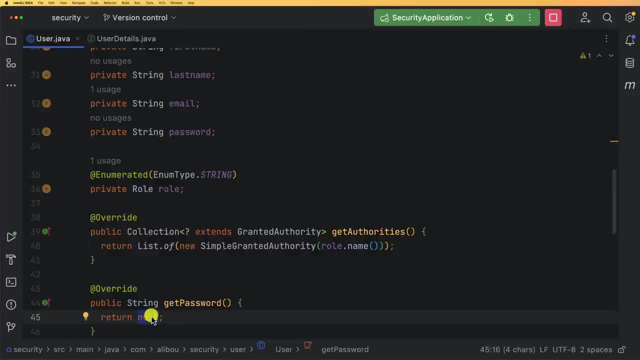 visible for you. i will rename this one visible for you. i will rename this one to password. and here for this password, i to password. and here for this password, i to password. and here for this password. i will just return my my password, okay, so will just return my my password, okay so. 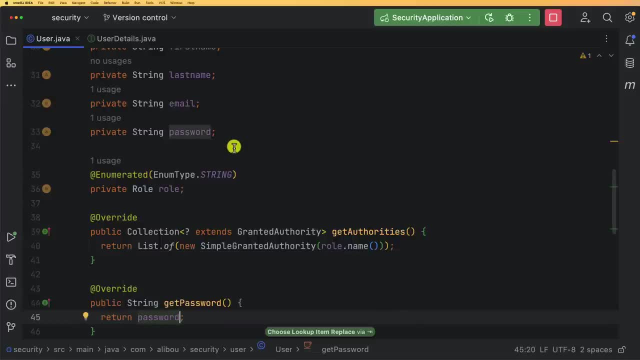 will just return my, my password, okay. so i just wanted to mention this one. so in i just wanted to mention this one. so in, i just wanted to mention this one. so in the next time, or like when you have a, the next time, or like when you have a, 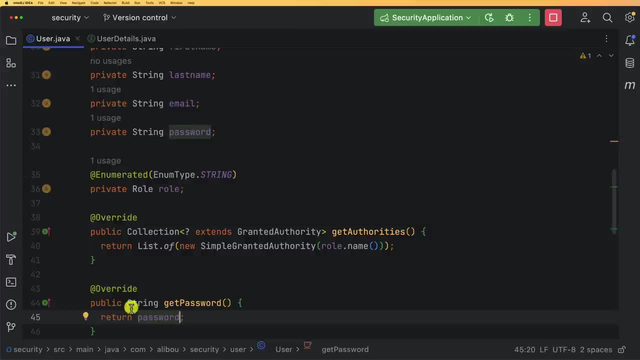 the next time, or like when you have a different name for this password field, different name for this password field, different name for this password field, you don't get surprised when you see. you don't get surprised when you see. you don't get surprised when you see this get password or when you have this. 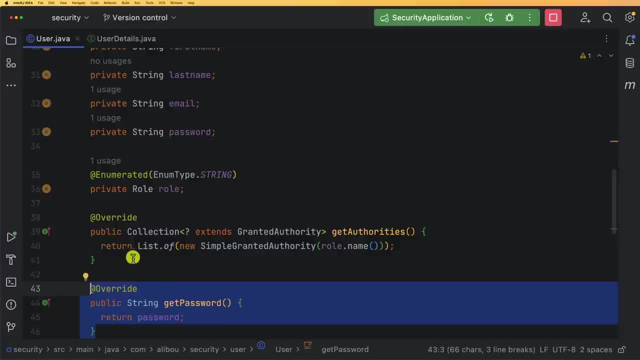 this get password, or when you have this, this get password, or when you have this password, exactly like that, and you don't password exactly like that and you don't password exactly like that and you don't see it. so now you know the reason why see it. so now you know the reason why. 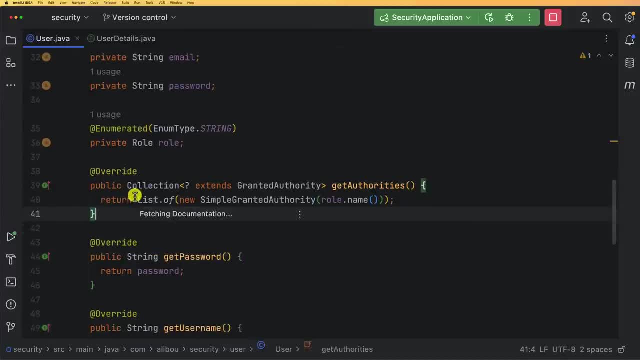 see it. so now you know the reason why. okay, so now we have everything we need. okay, so now we have everything we need. okay, so now we have everything we need within, within, within our user details. so we created a new: our user details. so we created a new. 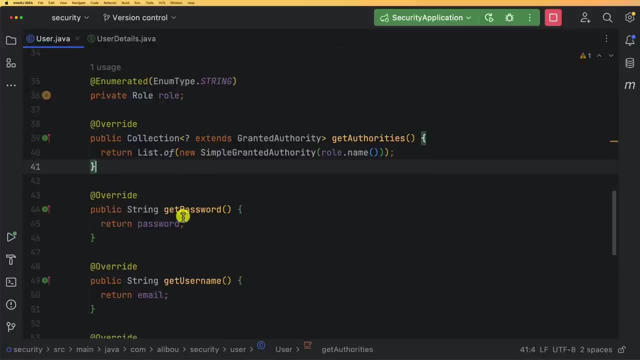 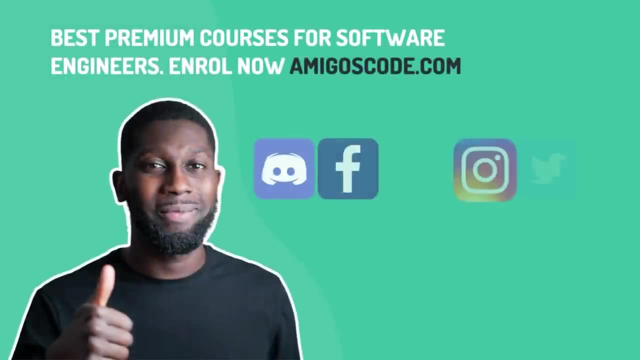 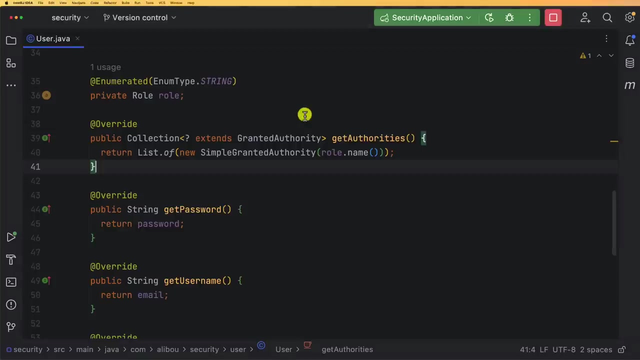 our user details. so we created a new role and we overridden or we defined all role and we overridden or we defined all role and we overridden or we defined all the methods that are required by spring, the methods that are required by spring, the methods that are required by spring: security. 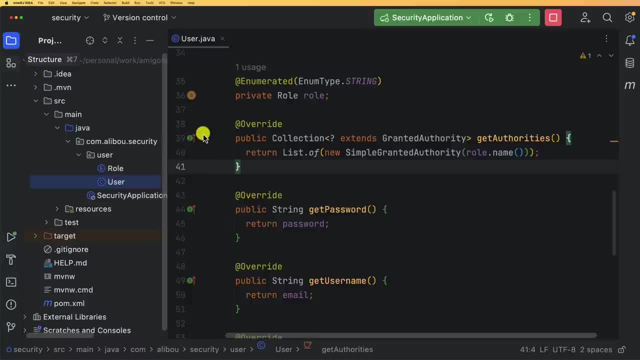 now our user is ready. so now our user is ready. so now our user is ready. so let's move on and create a repository. let's move on and create a repository. let's move on and create a repository for that user class. so the repository for that user class. so the repository. 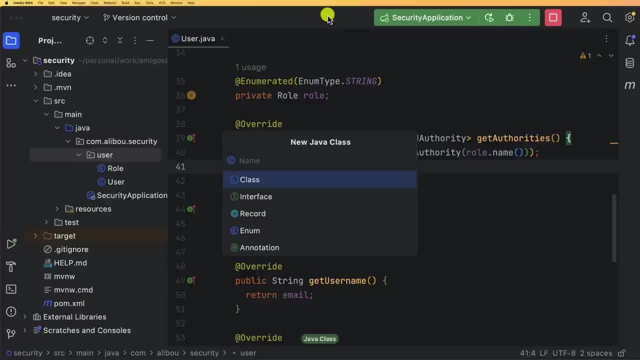 for that user class. so the repository is the class which is responsible to, is the class which is responsible to, is the class which is responsible to communicate with the database. communicate with the database, communicate with the database. so, when working with spring data, jpa we. so when working with spring data, jpa we. 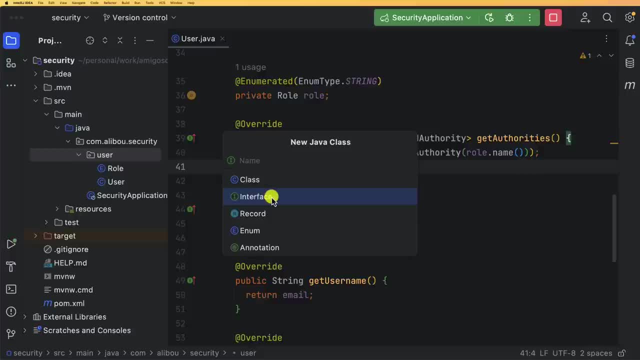 so, when working with spring data jpa, we don't need to create a class. all we need don't need to create a class. all we need don't need to create a class. all we need to do is create an interface, and let's to do is create an interface, and let's 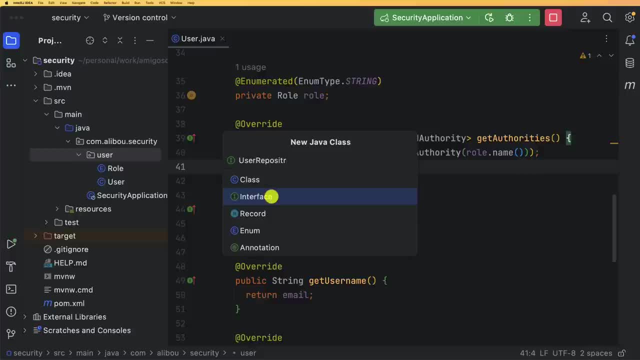 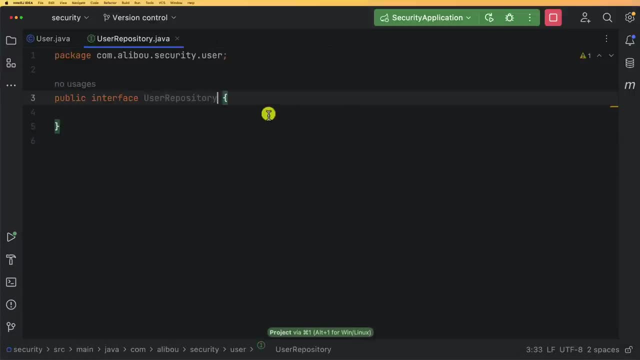 to do is create an interface and let's call it user repository. and this user repository to make it a and this user repository to make it a and this user repository to make it a. interface called jpa repository- okay, and interface called jpa repository- okay, and. 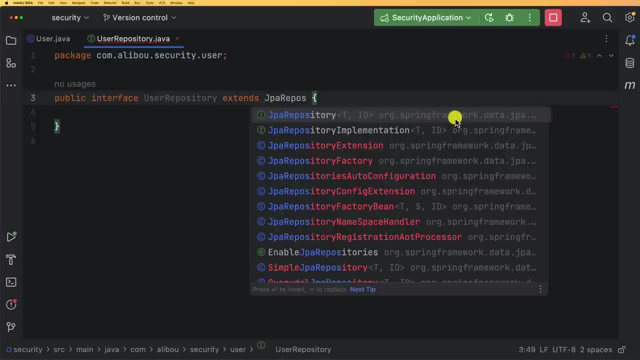 interface called jpa repository. okay, and as you can see here, this jpa repository, as you can see here, this jpa repository, as you can see here, this jpa repository is from spring framework data jpa, and so is from spring framework data jpa, and so 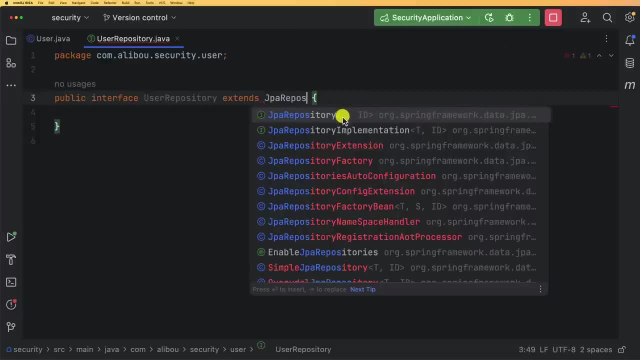 is from spring framework data, jpa, and so on, so forth, and it's a generic on so forth, and it's a generic on so forth, and it's a generic interface that takes a t. so which is the interface that takes a t? so which is the? 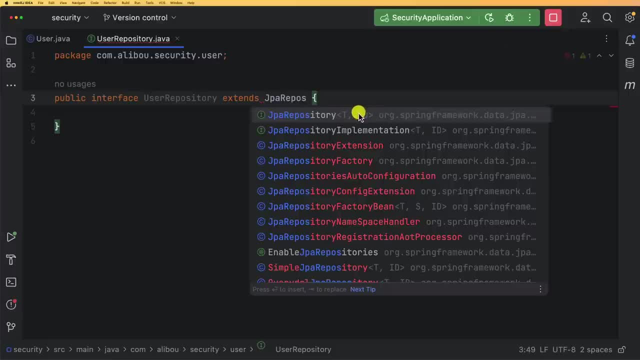 interface that takes a t, so which is the class, and an id which should be the id of class, and an id which should be the id of class, and an id which should be the id of our user class. so let's use this one, our user class. so let's use this one. 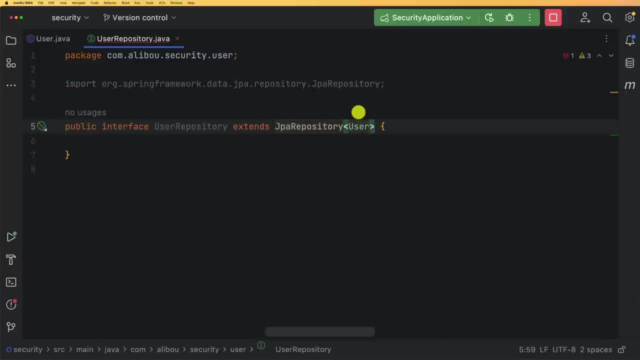 our user class, so let's use this one and pass these types. so this the user and pass these types. so this the user and pass these types. so this the user. and we used integer as an id, so let's. and we used integer as an id, so let's. 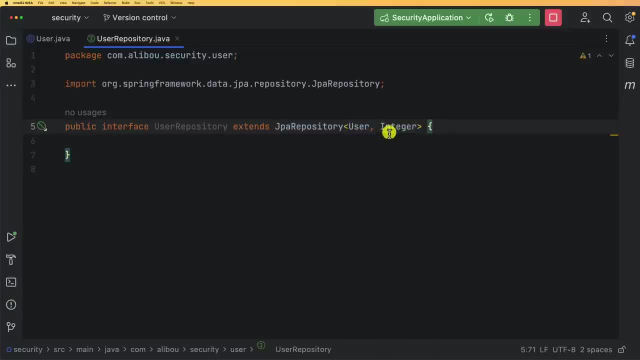 and we used integer as an id. so let's pass, pass, pass integer right here. okay. so now our integer right here. okay. so now our integer right here, okay. so now our repository is ready and, as you know, the repository is ready and, as you know, the repository is ready and, as you know, the spring data jpa has. 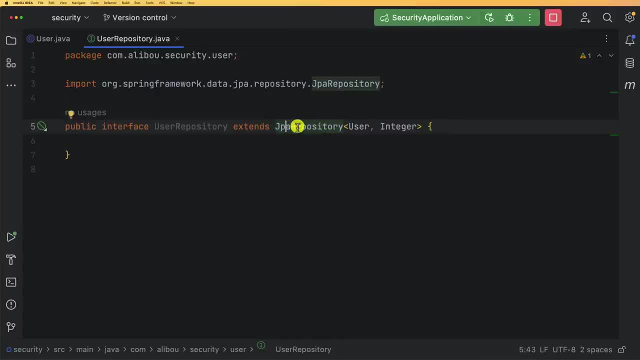 spring data. jpa has spring data. jpa has also a bunch of methods, or ready to use also a bunch of methods, or ready to use also a bunch of methods or ready to use methods. methods, methods like save find all, find by id and so on. like save find all, find by id and so on. 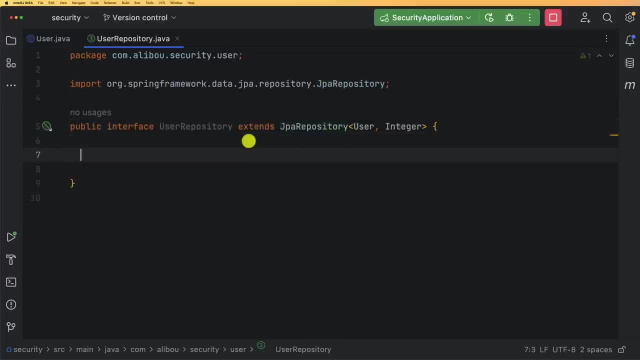 like save, find all, find by id, and so on and so forth. okay, now i will create one, and so forth. okay, now i will create one, and so forth. okay, now i will create one method that we will need later on, method that we will need later on. 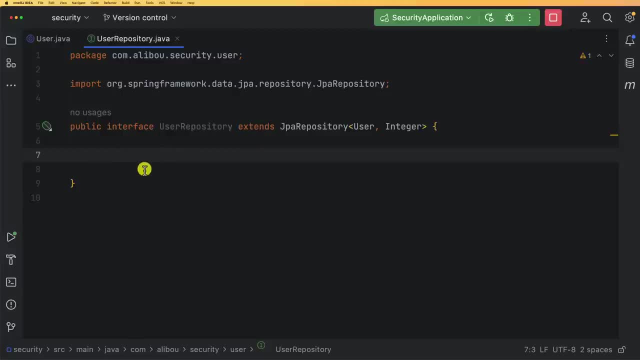 method that we will need later on and this method will, and this method will, and this method will will try to retrieve or find a user by. will try to retrieve or find a user by. will try to retrieve or find a user by email, because email is unique, so we need. 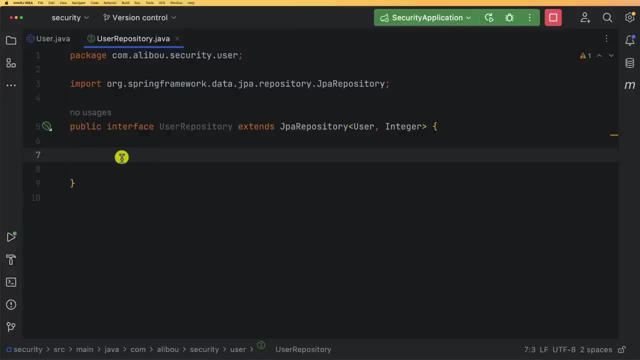 email because email is unique, so we need email. because email is unique, so we need to find, or we need to fetch a user by to find, or we need to fetch a user by to find, or we need to fetch a user by its email. all right, so i'm gonna create. 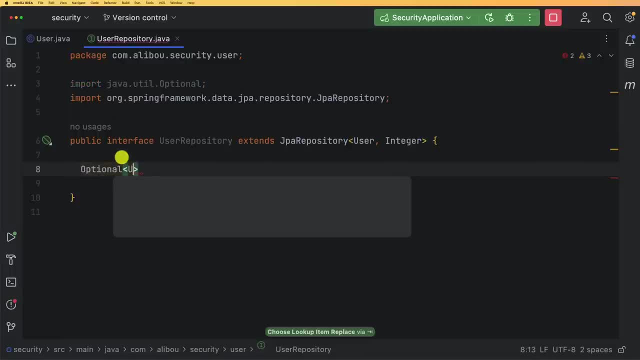 its email, all right, so i'm gonna create its email, all right. so i'm gonna create this optional, this optional, this optional user, and like optional is a generic type user and like optional is a generic type user and like optional is a generic type, so it's an optional of user. and here i 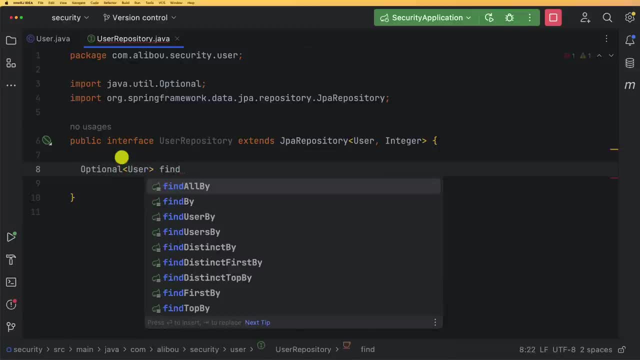 so it's an optional of user, and here i so it's an optional of user and here i will use the query method, will use the query method, will use the query method provided by spring and i will use the provided by spring and i will use the. 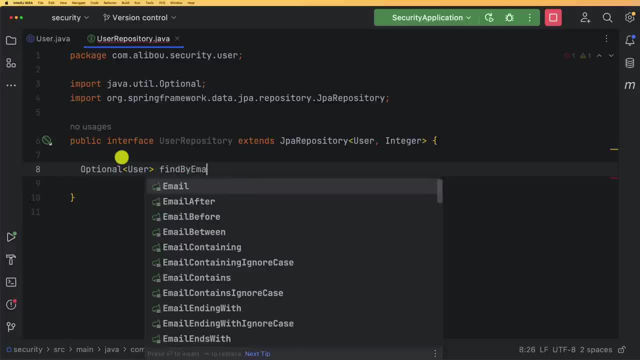 provided by spring, and i will use the method find by method, find by method, find by: and here all you need to do is providing: and here, all you need to do is providing: and here, all you need to do is providing the attribute or the field name that you 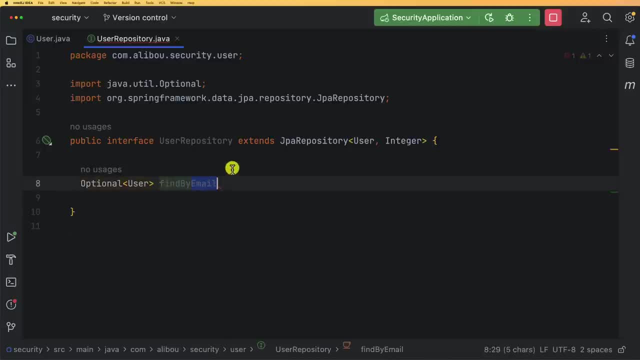 the attribute or the field name that you, the attribute or the field name that you have within your class, have within your class, have within your class. so for our case, it's email, for example. if so, for our case it's email, for example. if so, for our case it's email. for example, if you use username, just find by username. 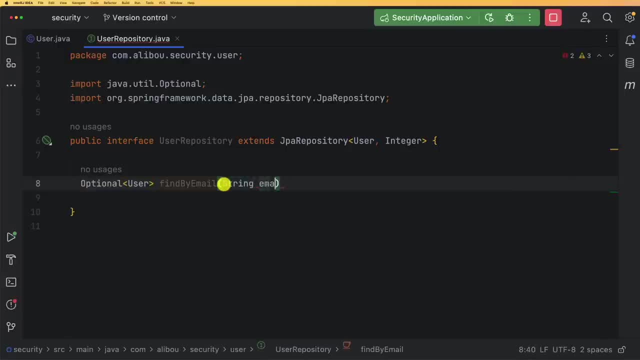 you use username, just find by username. you use username, just find by username. and here all i need to do is to pass. and here all i need to do is to pass, and here all i need to do is to pass: string email, string email, string email, all right, so 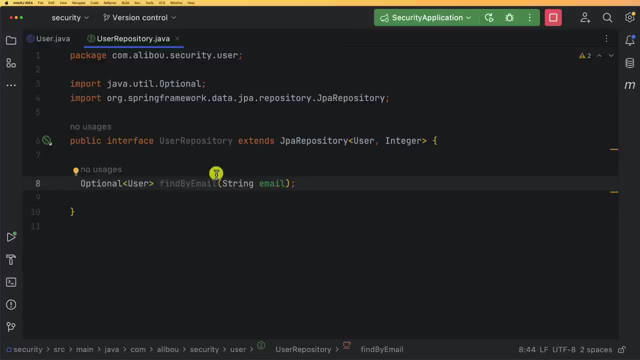 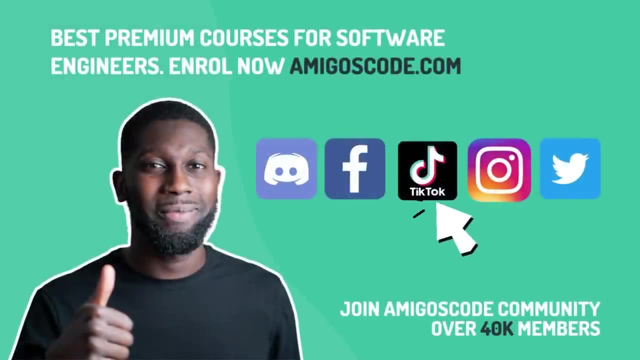 all right, so all right. so this is it now we have our repository. this is it now we have our repository. this is it now we have our repository ready to use. let's move on to the next ready to use. let's move on to the next ready to use. let's move on to the next steps. 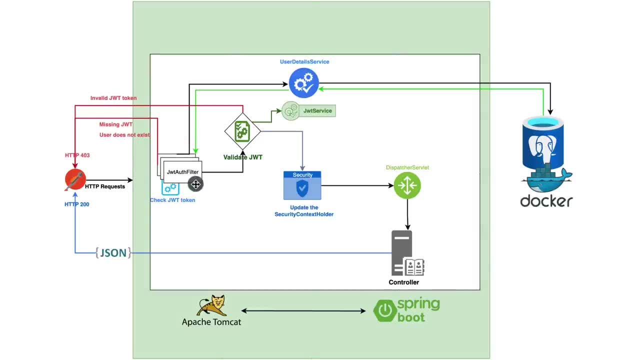 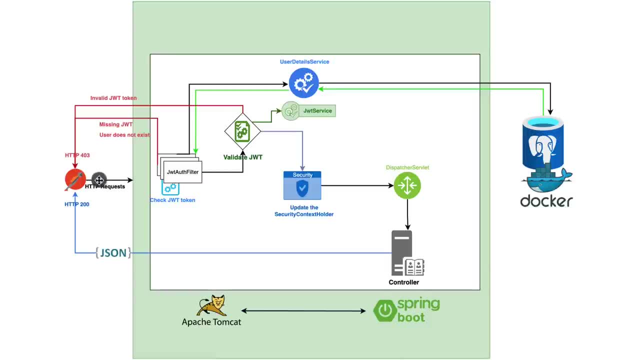 here. so we see that the first thing that here. so we see that the first thing that we will get, or the first thing that we will get, or the first thing that we will get, or the first thing that will intercept our http request is the will intercept our http request is the. 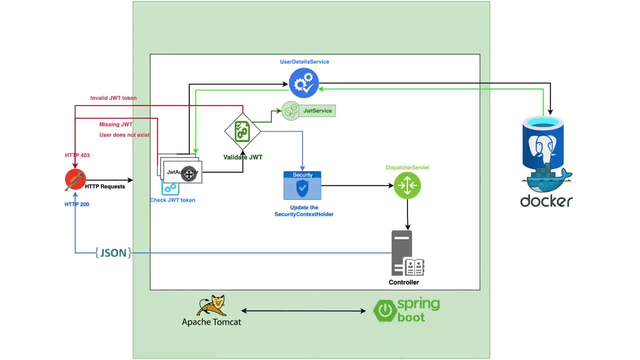 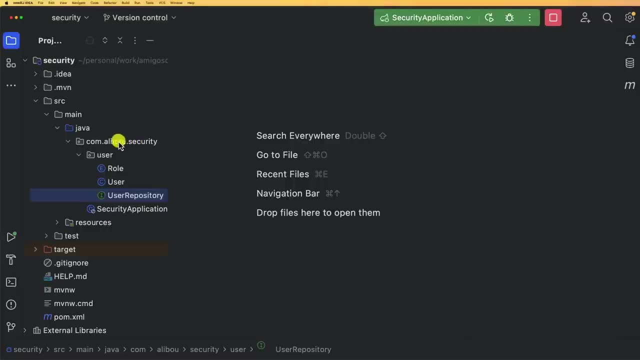 will intercept our http request is the jwt authentication filter. jwt authentication filter, jwt authentication filter. so let's go ahead and create this. so let's go ahead and create this. so let's go ahead and create this filter. so here within our base package, right? so here within our base package, right. 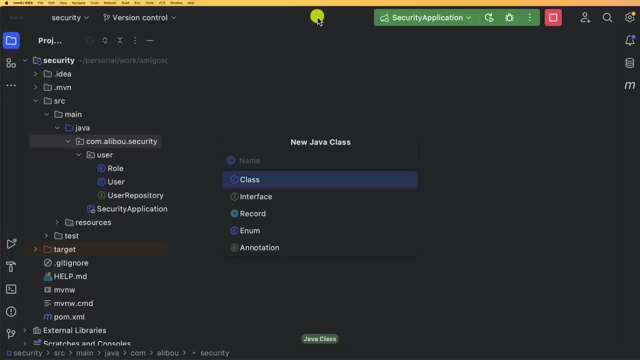 so here within our base package, right click right here. click right here. click right here. new, new, new, and i will create a new package. i will and i will create a new package. i will and i will create a new package. i will call it config. call it config. 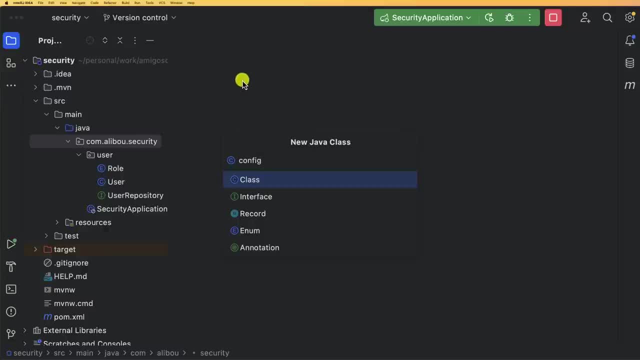 call it config. so i want all this to be part of my, so i want all this to be part of my, so i want all this to be part of my configuration package, configuration package, configuration package: and i will create, and i will create, and i will create a jwt authentication filter. 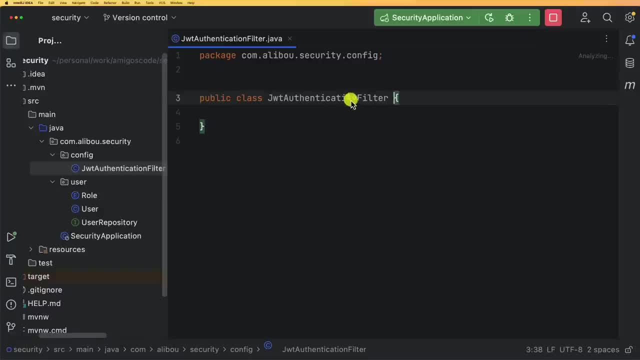 a jwt authentication filter, a jwt authentication filter. i will call it like that. i will call it like that. i will call it like that. so this is our authentication filter, so this is our authentication filter, so this is our authentication filter class. and now, in order to make it a, 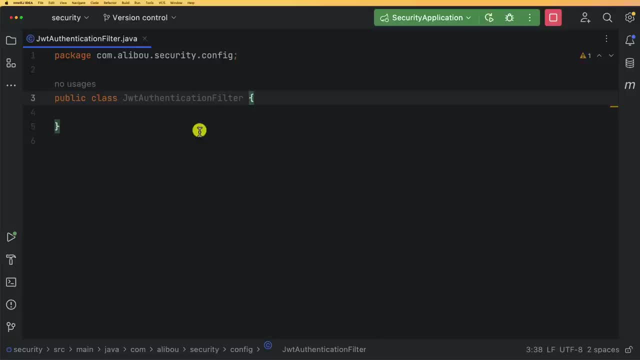 class. and now, in order to make it a class, and now in order to make it a filter, we have multiple options. okay, filter, we have multiple options. okay, filter, we have multiple options. okay, but here, as we can see in the schema, but here, as we can see in the schema, 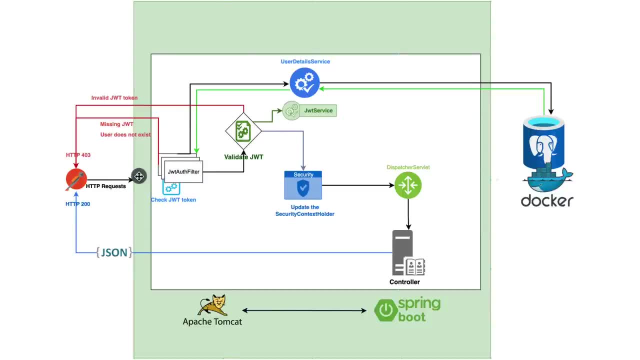 but here, as we can see in the schema, right here we have the. we want this. right here we have the. we want this. right here we have the. we want this filter to be active every time we get a filter, to be active every time we get a. 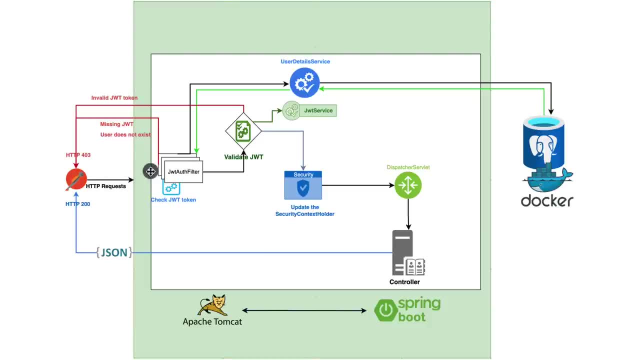 filter to be active every time we get a request. so every time the user sends a request. so every time the user sends a request. so every time the user sends a request, we want our filter to get fired. request. we want our filter to get fired. request. we want our filter to get fired and do all the job that we want that we. 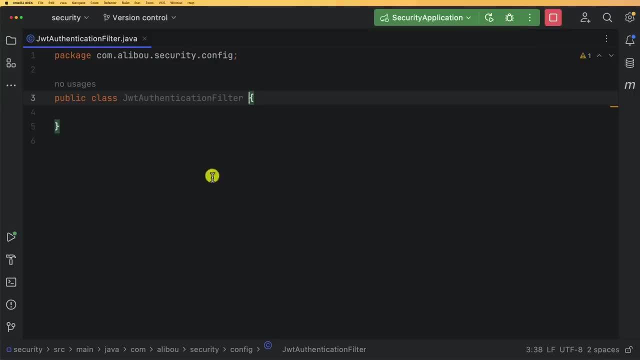 and do all the job that we want, that we and do all the job that we want. that we wanted to do okay, wanted to do okay, wanted to do okay. so this one we need to extend. so this one we need to extend. so this one we need to extend a class called once per request filter. 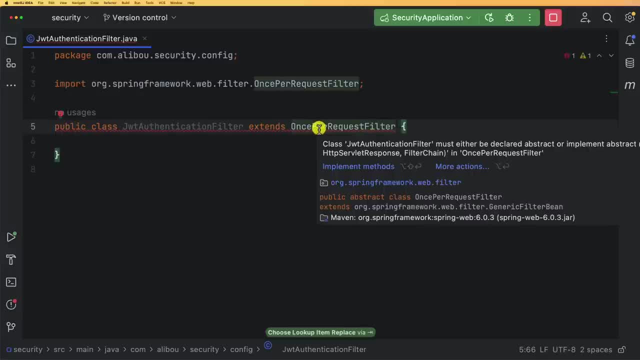 a class called once per request filter. a class called once per request filter and, as the name indicates it's, it will and as the name indicates it's, it will and as the name indicates it's it will be a filter by one every request, so be a filter by one every request. so. 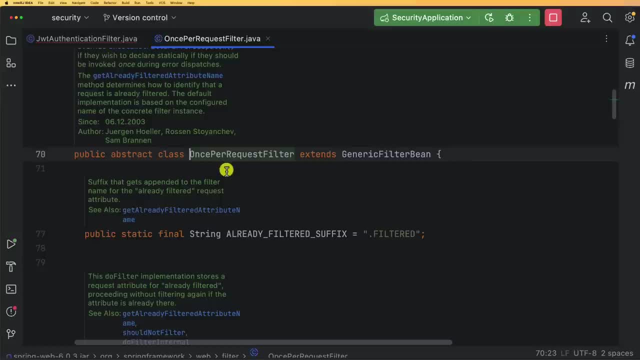 be a filter by one, every request. so let me download the data source and you let me download the data source and you let me download the data source and you can see here, can see here, can see here. once per request filter extends already. once per request filter extends already. 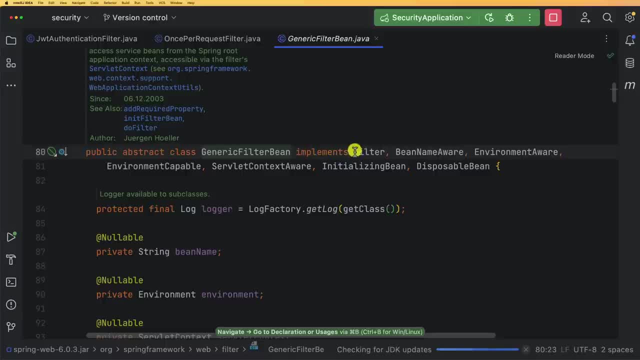 once per request. filter extends already generic filter bean and this generic generic filter bean and this generic generic filter bean and this generic filter bean already implements the filter bean, already implements the filter bean, already implements the interface called filter. so for us we had interface called filter, so for us we had 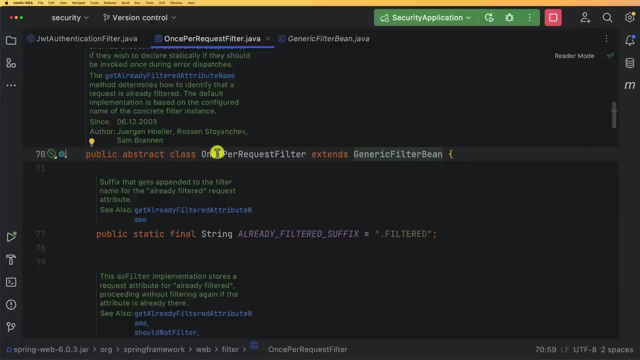 interface called filter. so for us, we had two options: whether using or extending two options. whether using or extending two options, whether using or extending this once per request filter or this once per request filter or this once per request filter. or implementing the filter interface right. implementing the filter interface right. 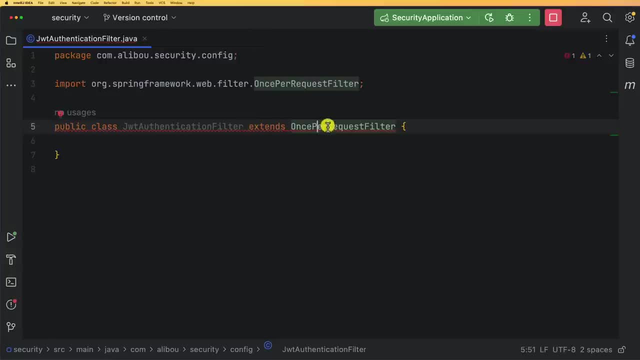 implementing the filter interface: right here, so it will be the same, but here, so it will be the same, but here, so it will be the same. but let's use something already provided by. let's use something already provided by, let's use something already provided by spring, so it's better to use the ones. 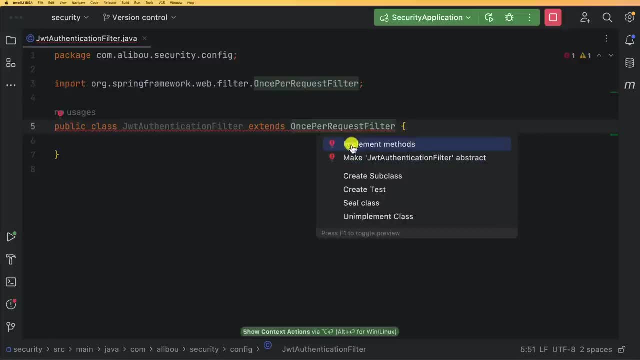 spring, so it's better to use the ones spring, so it's better to use the ones per request filter, so per request filter, so per request filter. so now let's implement the methods. now let's implement the methods. now let's implement the methods and we see here that we have a method. 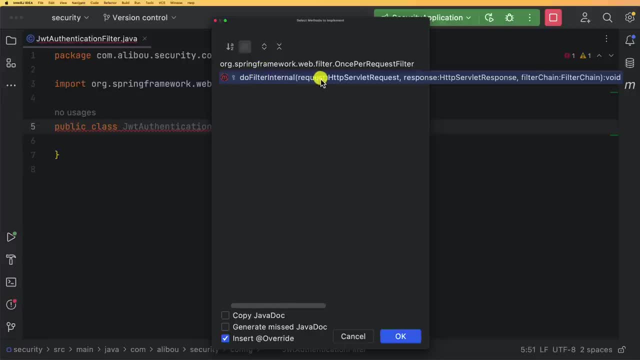 and we see here that we have a method and we see here that we have a method called do and filter internal and we called do and filter internal and we called do and filter internal. and we have three parameters: the request, the have three parameters: the request, the. 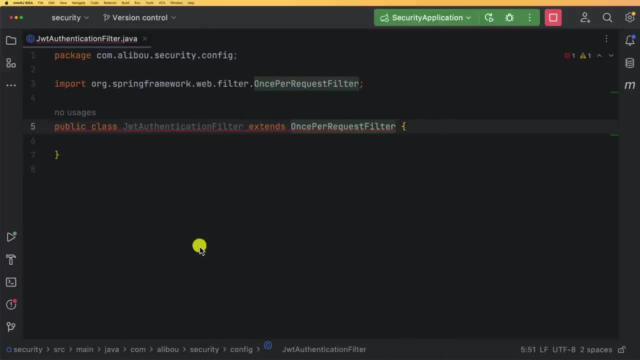 have three parameters: the request, the response and the filter chain. let me response. and the filter chain- let me response. and the filter chain. let me explain each part of it. explain each part of it. explain each part of it. i will just inline these parameters. i will just inline these parameters. 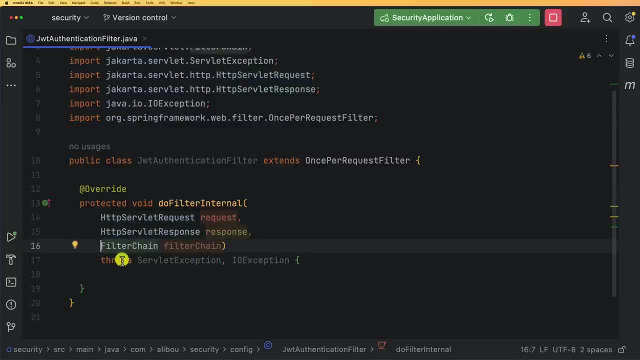 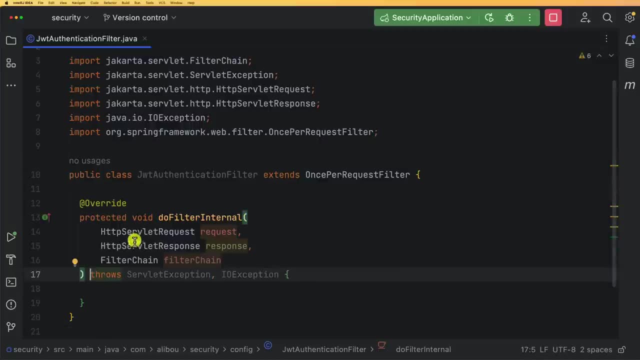 i will just inline these parameters right here so you can see all of it. so these are our, so these are our, so these are our parameters. so here what we have: we have parameters. so here what we have, we have parameters. so here what we have, we have this http: 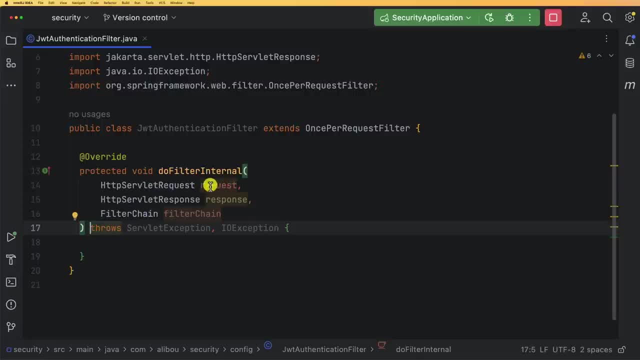 this http, this http servlet request: the response and the servlet request. the response and the servlet request: the response and the filter chain. so the request is our filter chain, so the request is our filter chain. so the request is our request and the response is also our request and the response is also our. 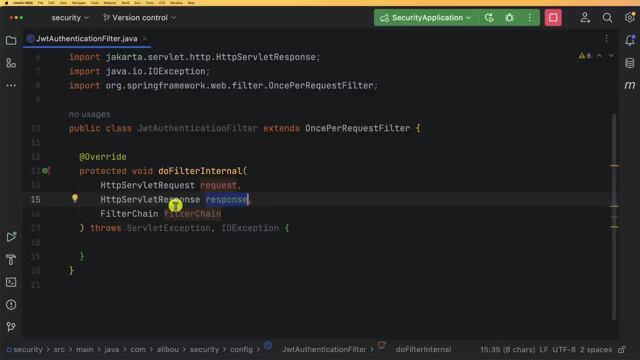 request and the response is also our response. so we can intercept every response. so we can intercept every response. so we can intercept every request and make and extract data from request. and make and extract data from request. and make and extract data from, for example, from the request and. 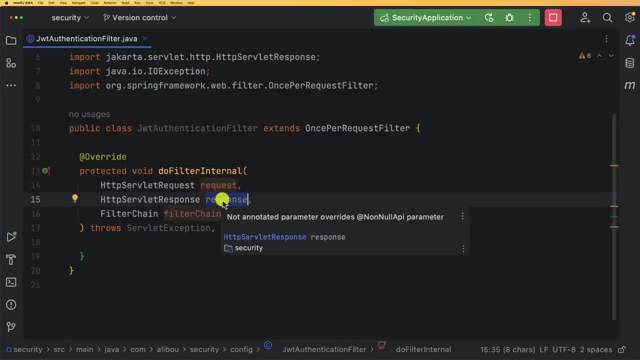 for example, from the request and for example, from the request, and provide new data within the response. so provide new data within the response. so provide new data within the response. so, for example, if i want to add a header, for example, if i want to add a header. 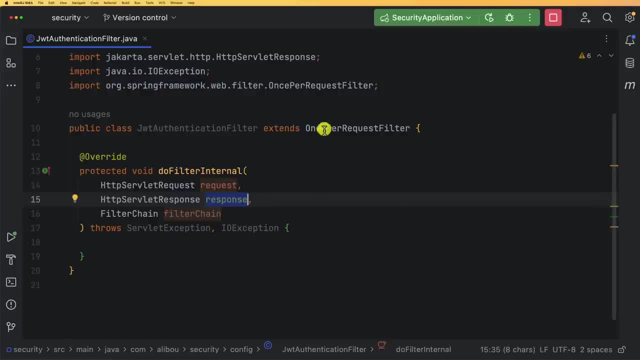 for example, if i want to add a header to my response, we can do it using this to my response. we can do it using this to my response. we can do it using this once per request filter: okay, and the once per request filter okay, and the once per request filter okay, and the filter chain is the chain of 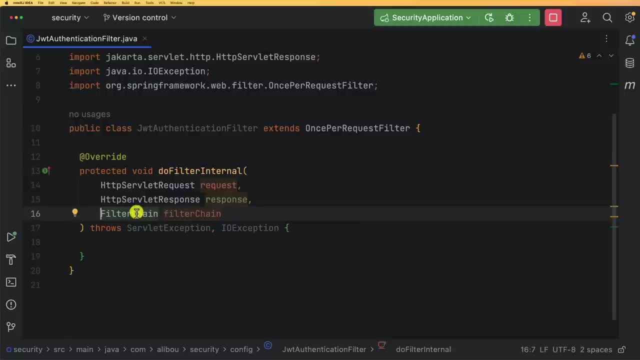 filter chain is the chain of filter chain is the chain of responsibility design pattern. so it responsibility design pattern. so it responsibility design pattern. so it will it contains the list of the other will. it contains the list of the other will. it contains the list of the other filters that we need. 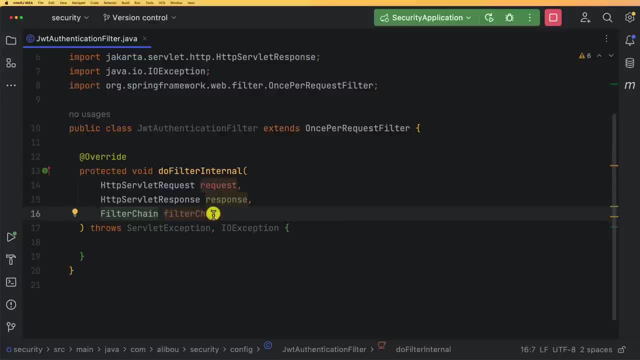 filters that we need, filters that we need, we need to execute. so when we call this, we need to execute. so when we call this, we need to execute. so when we call this filter chain dot- do internal filter or filter chain dot. do internal filter or filter chain dot- do internal filter or do filter, it will call the next filter. 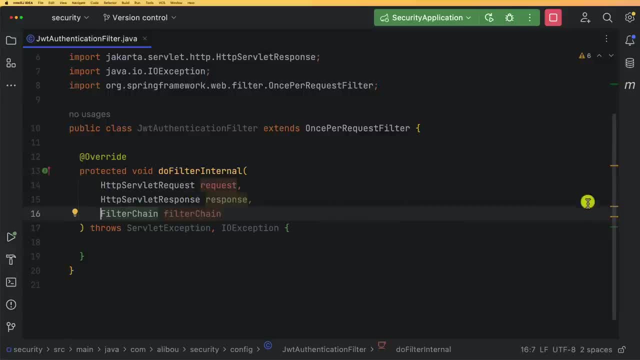 do filter, it will call the next filter. do filter, it will call the next filter within the chain. so here i want uh just within the chain. so here i want uh just within the chain. so here i want uh. just remove this, remove this, remove this, this warnings. so because this, uh, these. 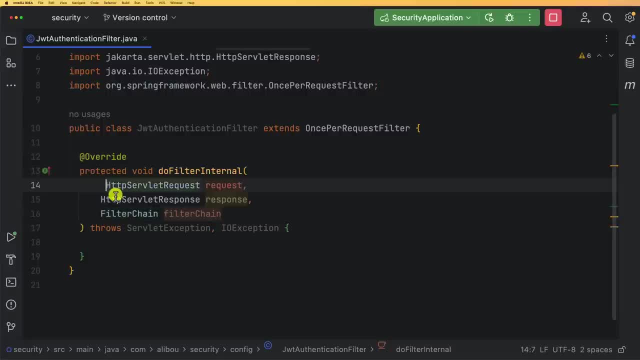 this warnings. so because this, uh, these, this warnings, so because this, uh, these three parameters, they should not be null. three parameters, they should not be null. three parameters, they should not be null. and to do so, i will just add this. and to do so, i will just add this. 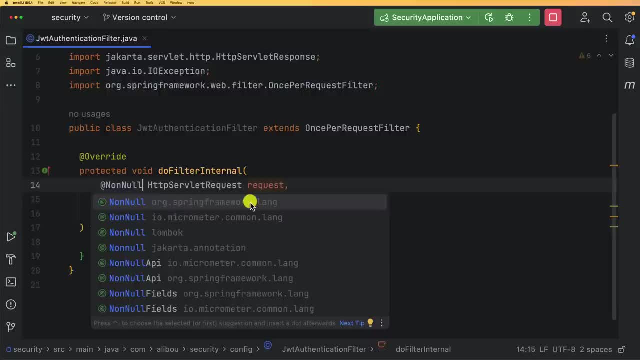 and to do so, i will just add this non null annotation, the one from spring, non null annotation, the one from spring, non null annotation, the one from spring frameworklang, frameworklang, frameworklang, and i'm gonna copy paste it and move it. and i'm gonna copy paste it and move it. 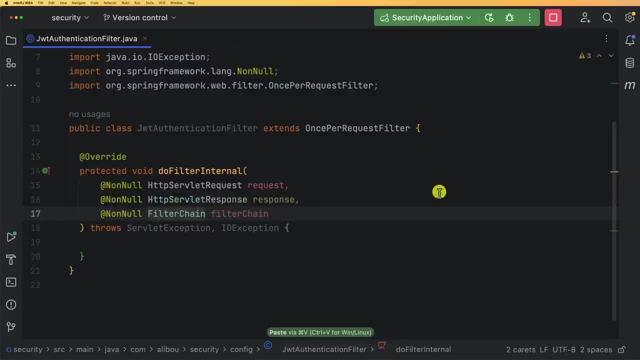 and i'm gonna copy paste it and move it and put it and put it, and put it in here. okay, so like this: we no longer in here. okay, so like this: we no longer in here. okay, so like this, we no longer have this warning. have this warning. 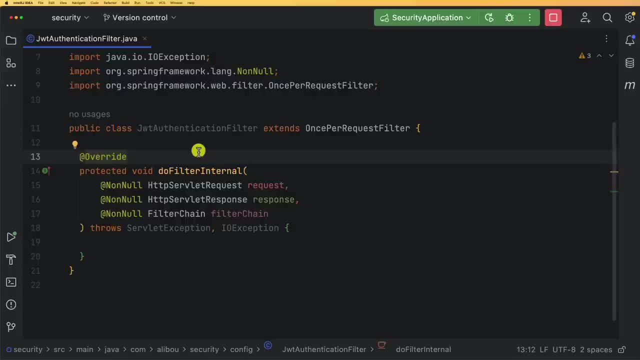 have this warning and now, the last thing to do before and now, the last thing to do before and now, the last thing to do before moving on and start implementing this, moving on and start implementing this, moving on and start implementing this. the last thing to do is we need to tell. 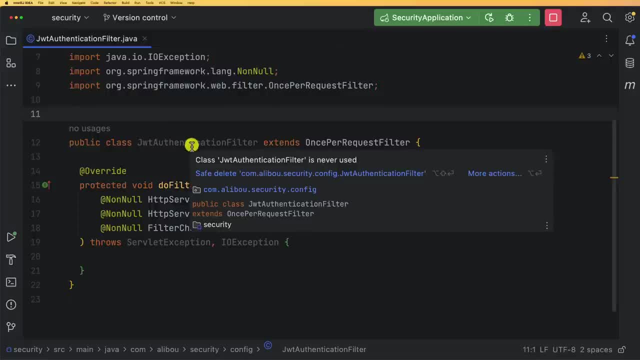 the last thing to do is we need to tell. the last thing to do is we need to tell spring that we want spring, that we want spring, that we want this class to be managed bin okay, or to this class to be managed bin okay, or to this class to be managed bin okay, or to become a spring pin. 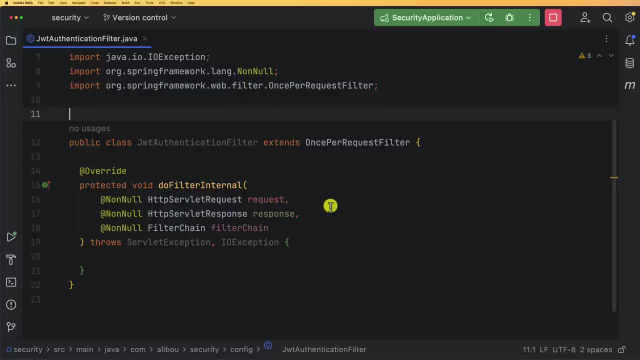 become a spring pin. become a spring pin, and to do so, we need to annotate whether and to do so, we need to annotate whether and to do so, we need to annotate whether: with service annotation or component with service annotation or component with service annotation or component annotation. 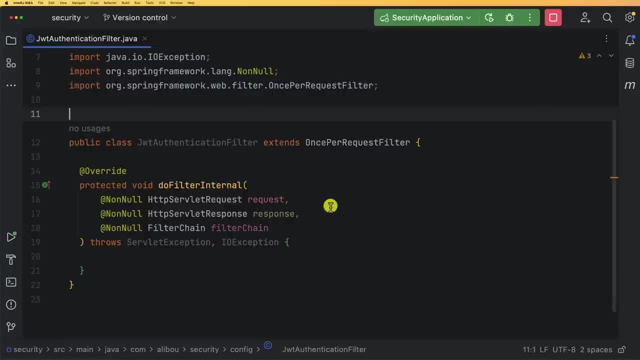 annotation. annotation or also repository, it works because three. or also repository, it works because three. or also repository, it works because three of them are the same. annotation of them are the same. annotation of them are the same. annotation, the repository and the service, they both. the repository and the service, they both. 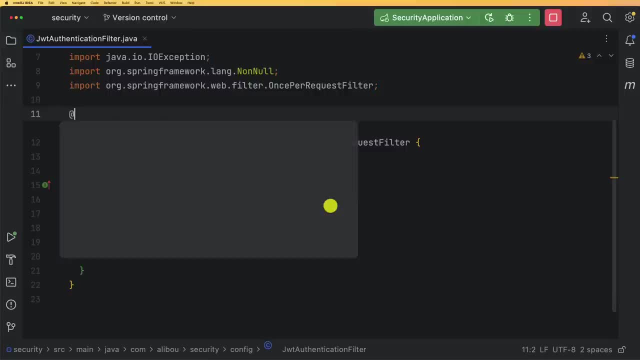 the repository and the service. they both extend the component, extend the component, extend the component. but i will just make it a component, but i will just make it a component, but i will just make it a component right here, right here, right here. and also i will use another lombok. 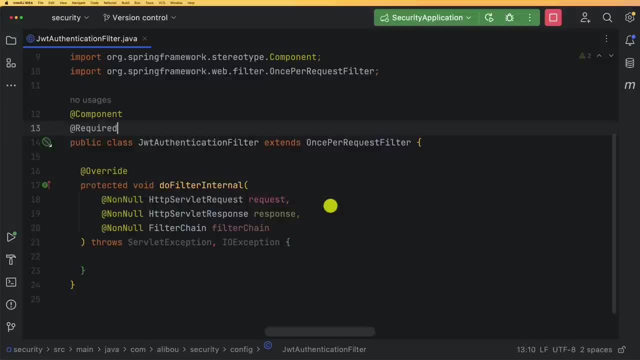 and also i will use another lombok, and also i will use another lombok, annotation, which is annotation, which is annotation, which is the required arcs constructor and this the required arcs constructor and this the required arcs constructor and this required arcs constructor, it will create. required arcs constructor. it will create. 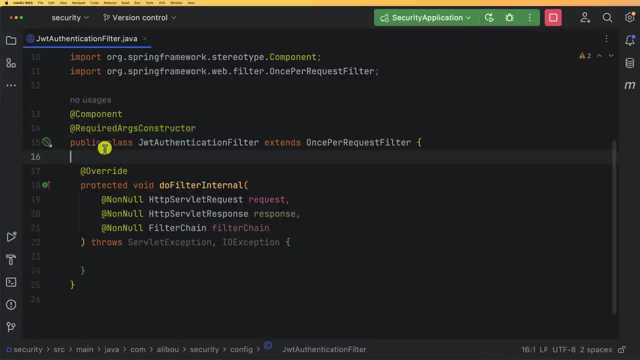 required arcs constructor. it will create a constructor using any final field, that a constructor using any final field, that a constructor using any final field that we declare, we declare. we declare right here. so, for example, if i use, if i right here. so, for example, if i use, if i. 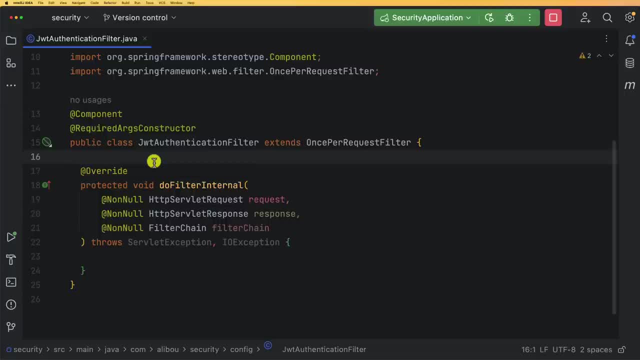 right here. so, for example, if i use, if i do private, do private, do private final string, my string, this annotation, final string, my string, this annotation, final string, my string, this annotation, it will create a constructor using it, will create a constructor using it, will create a constructor using this private final field. okay, so, 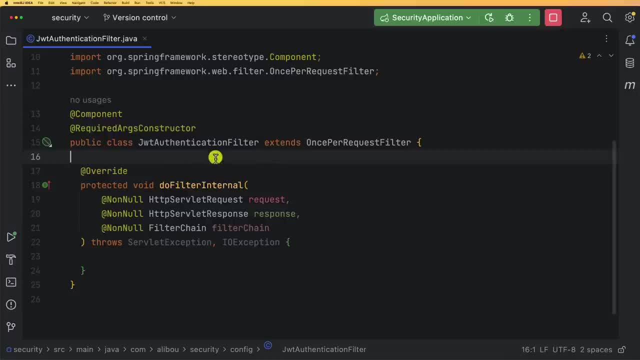 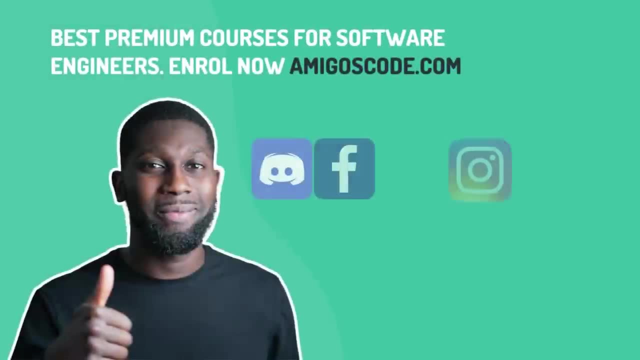 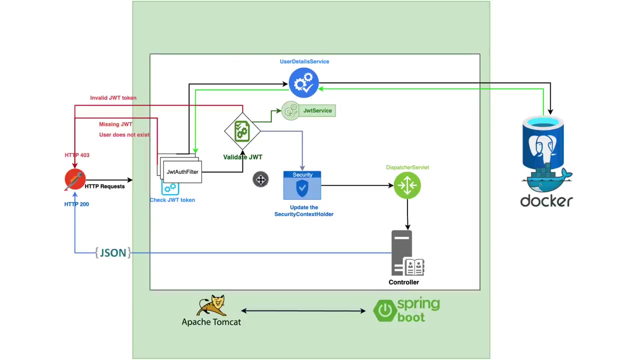 this private final field. okay, so this private final field, okay. so now we have our. now we have our. now we have our filter ready to use. let's now start filter ready to use. let's now start filter ready to use. let's now start implementing it part by part. 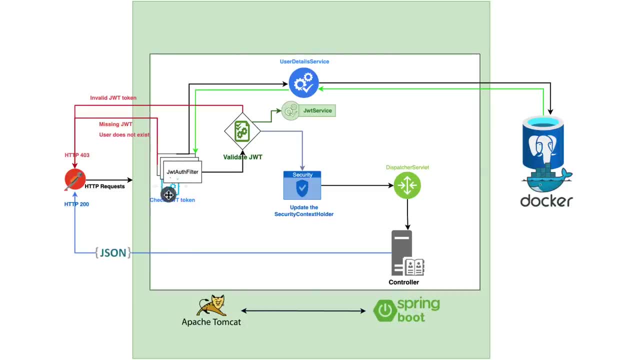 from this diagram right here, we see that. from this diagram right here, we see that. from this diagram right here, we see that the first thing, that the first thing, that the first thing that gets executed, or the first thing we do gets executed, or the first thing we do. 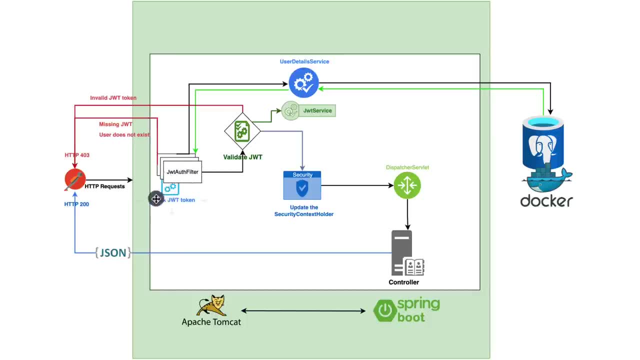 gets executed. or the first thing we do within this jwt authentication filter, within this jwt authentication filter, within this jwt authentication filter, is checking if we have the jwt token, is checking if we have the jwt token, is checking if we have the jwt token. okay, so let's move on and implement. 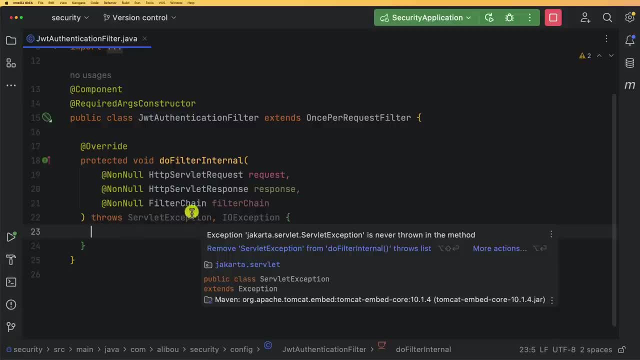 okay, so let's move on and implement. okay, so let's move on and implement this, this, this, this. all right to do so within our method. all right to do so within our method. all right to do so within our method. do internal filter, let's try to perform. 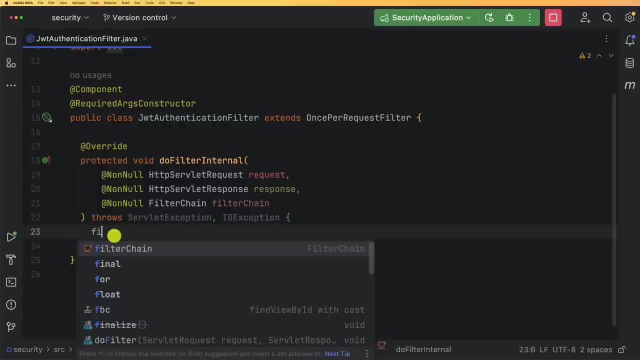 do internal filter, let's try to perform. do internal filter, let's try to perform some operations. okay, so first of all, i some operations. okay, so first of all i some operations. okay. so first of all, i will create, will create, will create a string, i will call it authentication. 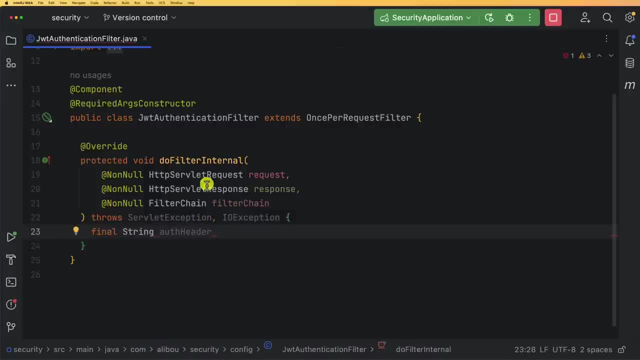 a string. i will call it authentication. a string. i will call it authentication: header, header, header. right. why? because, when we make a call, right. why? because, when we make a call, right. why? because when we make a call, we need to pass the jwt authentication. we need to pass the jwt authentication. 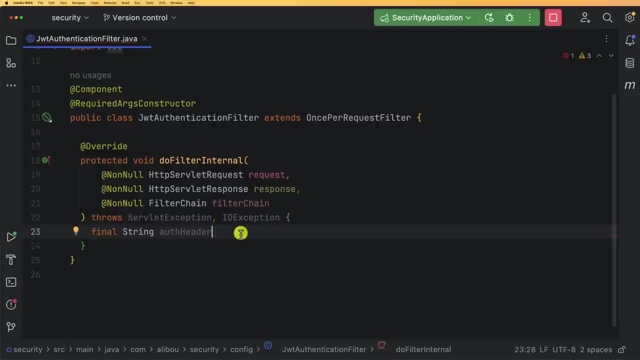 we need to pass the jwt authentication token within the header. so it should be token within the header. so it should be token within the header. so it should be within a header called authorization, so within a header called authorization, so within a header called authorization. so what we need to do here is create is. 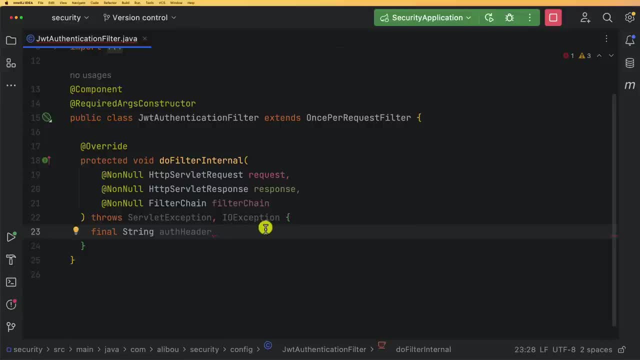 what we need to do here is create is. what we need to do here is create is try to extract this header. okay, try to extract this header. okay, try to extract this header. okay, so this authentication header is part. so this authentication header is part. so this authentication header is part of our request. 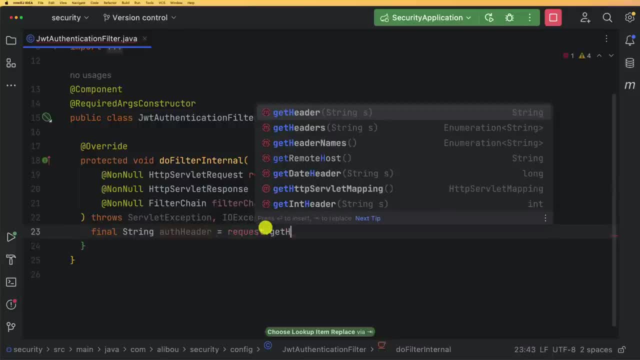 of our request. of our request and from the request, we can call a, and from the request, we can call a, and from the request, we can call a method called get header and within the method called get header. and within the method called get header and within the header. 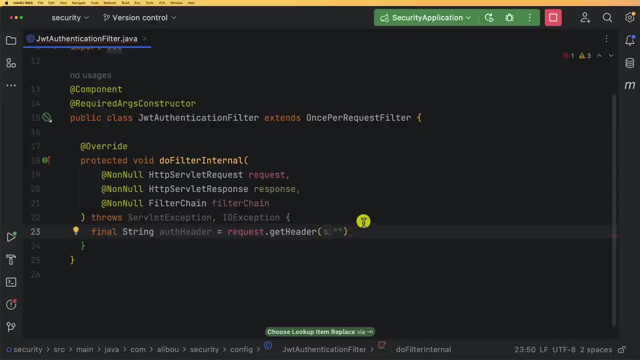 header header. we can. all we need to do is to pass we can. all we need to do is to pass we can. all we need to do is to pass the header name. the header name. the header name contains the jwt token or the viewer contains the jwt token or the viewer. 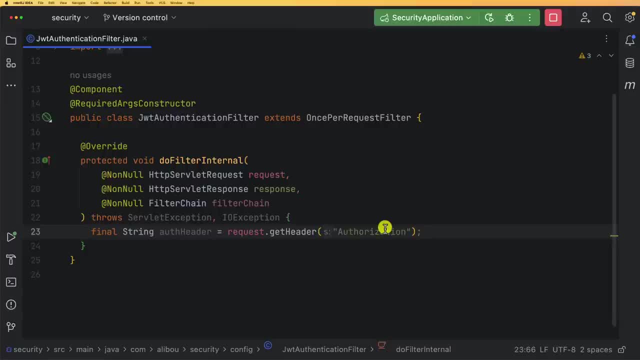 contains the jwt token or the viewer token. we call it also viewer token. okay token. we call it also viewer token. okay token. we call it also viewer token. okay, all right. so, all right. so, all right. so now i will create another variable. let's. now i will create another variable. let's. 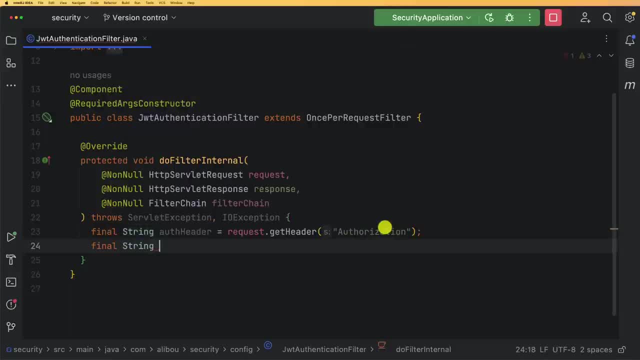 now i will create another variable. let's also make it final string. also make it final string. also make it final string. i will call it jwt or jwt token, call it. i will call it jwt or jwt token call it. i will call it jwt or jwt token, call it whatever you want. 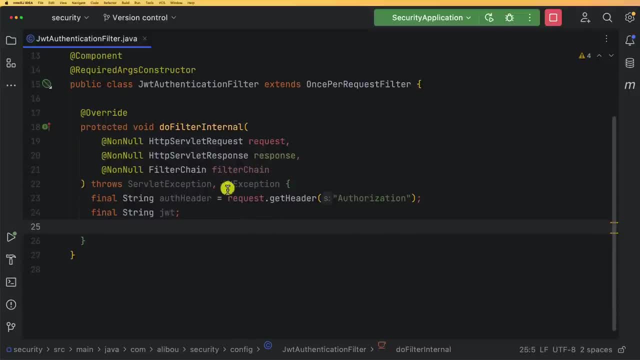 whatever you want, whatever you want. so here i want to implement this check. so here i want to implement this check. so here i want to implement this check that we did before, so we we talk about that we did before, so we we talk about. here we talk about this check. jwt token. 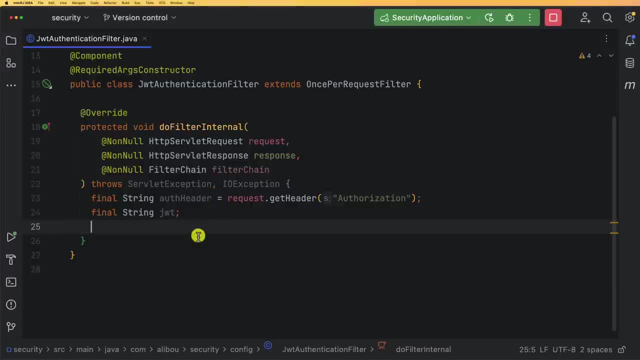 here we talk about this check jwt token. here we talk about this check jwt token. so let's go, let's implement this. so let's go, let's implement this. so let's go, let's implement this. so here the test that i want to do is. so here the test that i want to do is. 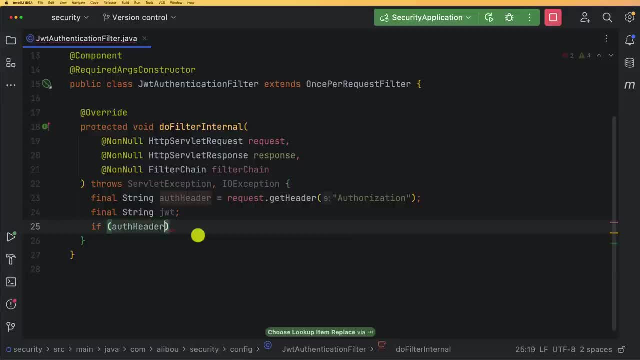 so here the test that i want to do is: if the author authorization header, if the author authorization header, if the author authorization header is null, so i want to do an early return- is null, so i want to do an early return- is null, so i want to do an early return, or 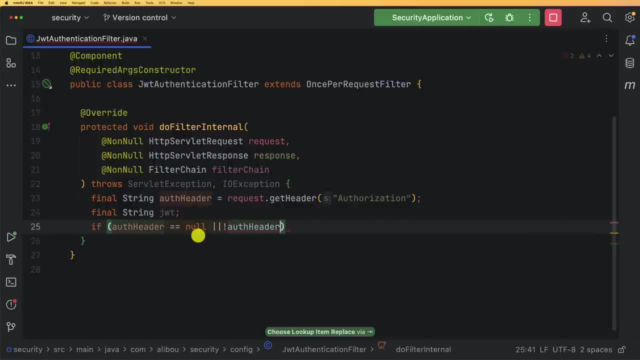 or, or. if not, my authorization header dot. if not, my authorization header dot. if not, my authorization header dot. starts with: because, as i told you the starts with, because, as i told you the starts with, because, as i told you, the beer token, beer token should be always or should start always. 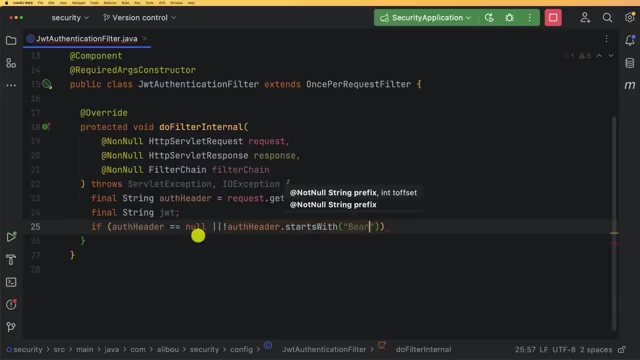 should be always, or should start always. should be always, or should start always with the keyword, with the keyword, with the keyword bitter, okay, and it should be exactly bitter, okay, and it should be exactly bitter, okay, and it should be exactly like that, and then we have a space. so if 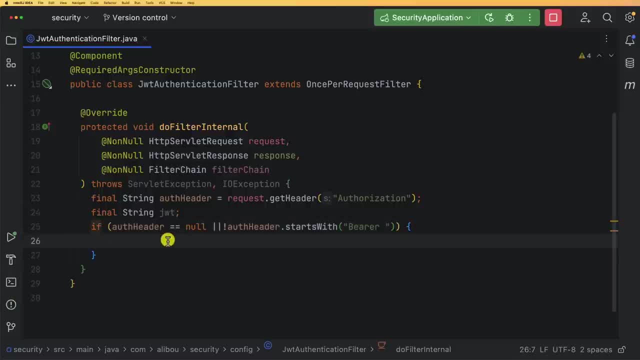 like that, and then we have a space. so if like that, and then we have a space. so if we don't have these two conditions, we don't have these two conditions. we don't have these two conditions. all i need to do is call the filter. all i need to do is call the filter. 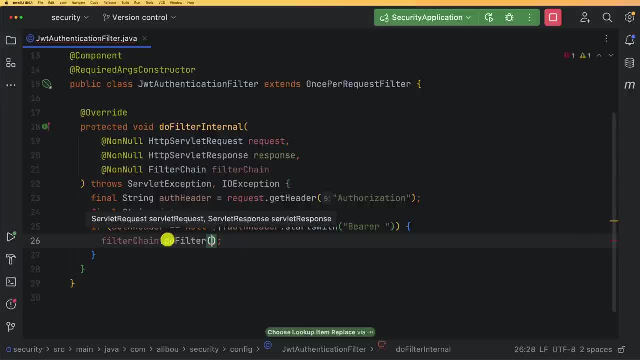 all i need to do is call the filter: chain dot do chain dot do chain dot do filter. and i need to pass the request filter and i need to pass the request filter and i need to pass the request and the response to the next filter. okay, and the response to the next filter: okay. 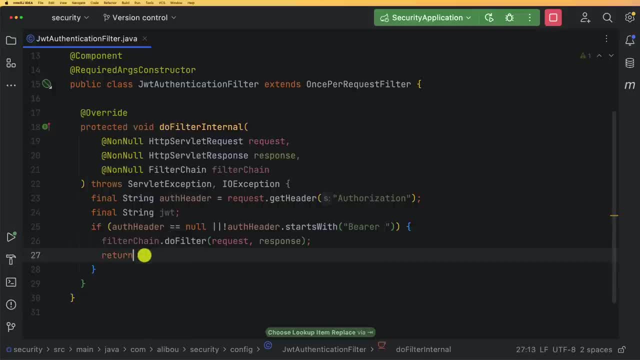 and the response to the next filter. okay, and here don't forget to call the return. and here don't forget to call the return. and here don't forget to call the return. semicolon: so we want, we don't want to. semicolon: so we want, we don't want to. 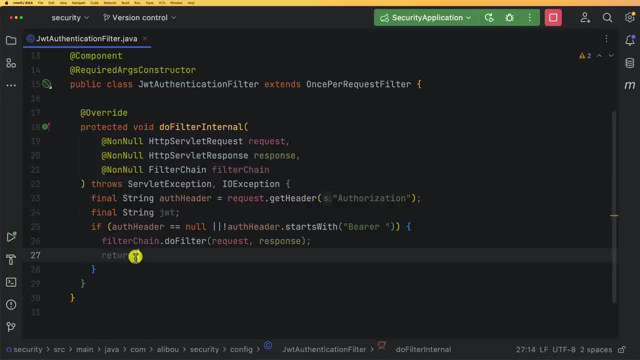 semicolon. so we want, we don't want to continue with the execution of the rest, continue with the execution of the rest, continue with the execution of the rest of that one, okay, of that one, okay of that one, okay. so here, this is the check that we uh. 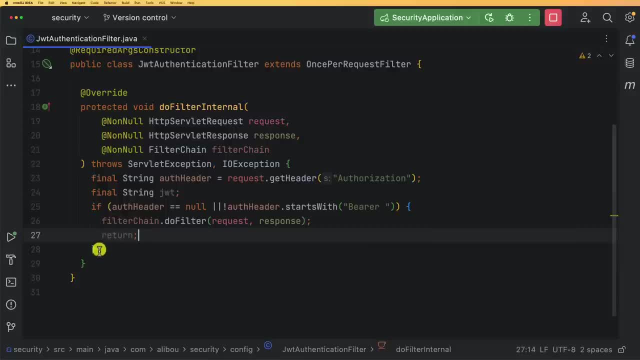 so here, this is the check that we uh. so here, this is the check that we uh that we implemented now. let's try to that we implemented now. let's try to that we implemented now. let's try to extract the token from this header. okay, extract the token from this header, okay. 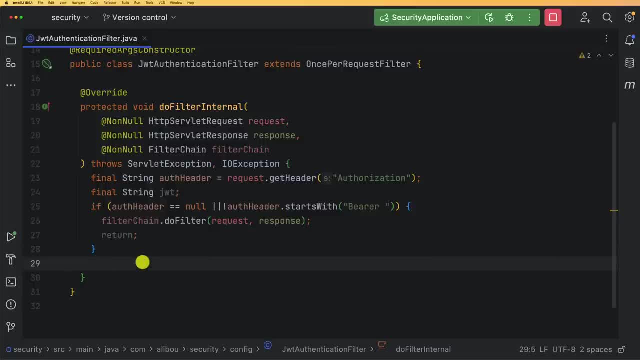 extract the token from this header, okay, from this authentication header, from this authentication header, from this authentication header. the next step is: we created already a jwt. the next step is: we created already a jwt. the next step is: we created already a jwt variable. now i want to extract. 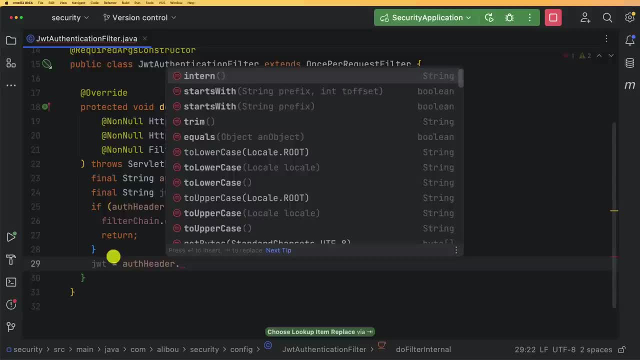 variable. now. i want to extract variable. now i want to extract this token from this token from this token from my authentication header, or from my- my authentication header, or from my- my authentication header, or from my authorization header, and i want to do a authorization header and i want to do a. 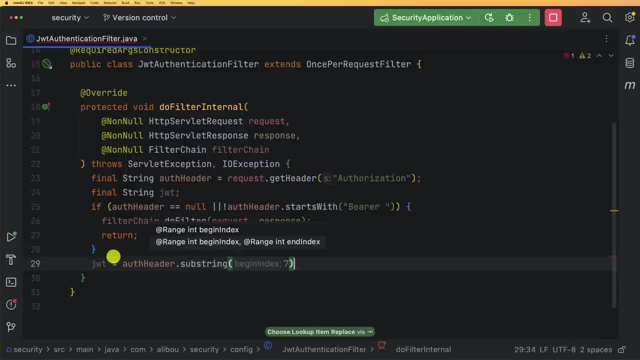 authorization header and i want to do a substring, starting from the position substring, starting from the position substring, starting from the position number seven. and why position number number seven? and why position number number seven? and why position number seven? because if we count this beer with seven, because if we count this beer with 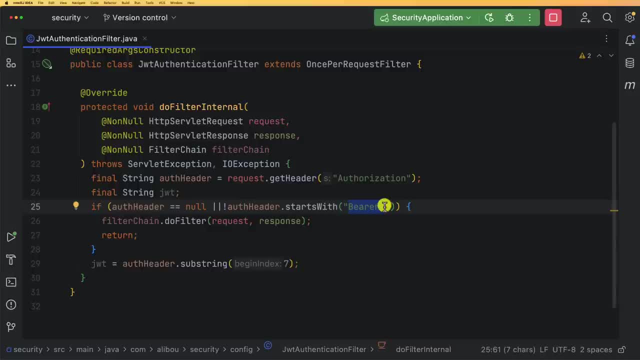 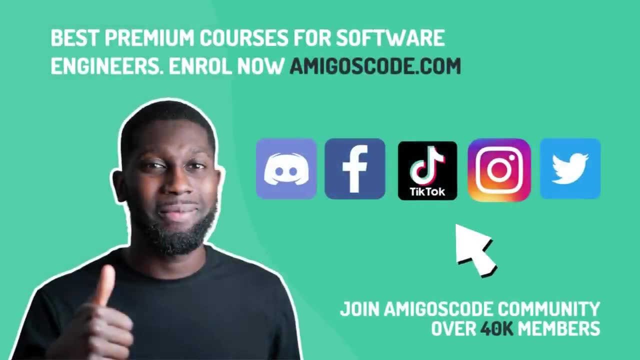 seven, because if we count this beer with this space, this space, this space, the count is seven. okay, so let's move on. the count is seven okay, so let's move on. the count is seven okay. so let's move on and check what we need to do next. 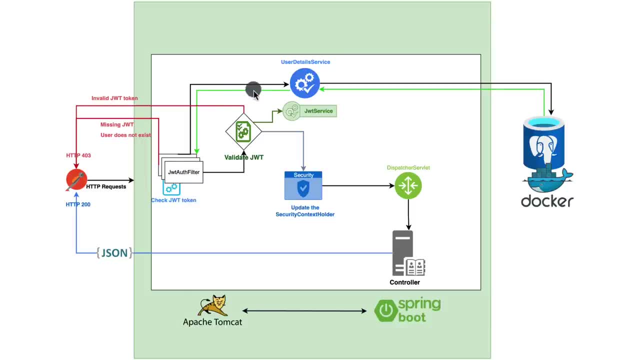 after checking the jwt token. what we, after checking the jwt token, what we, after checking the jwt token, what we need to do, need to do, need to do, is to call this user details service to. is to call this user details service to. is to call this user details service to check if we have. 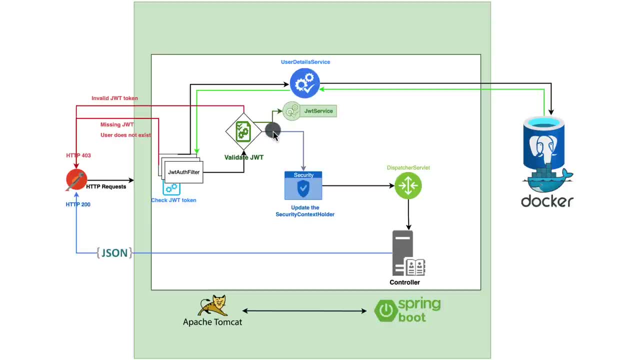 check if we have, check if we have the user already within our database, or the user already within our database, or the user already within our database or not? not? not okay, but to do that we need to call. okay, but to do that we need to call. okay, but to do that we need to call a jwt service here to extract. 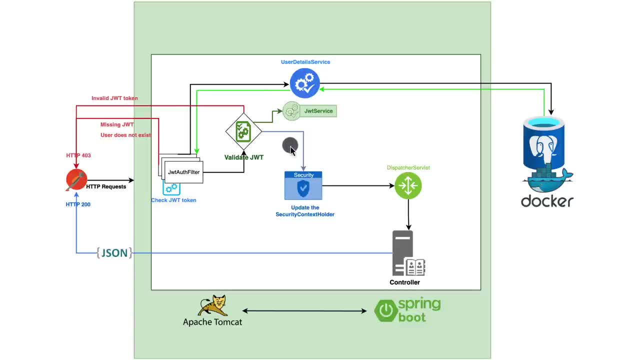 a jwt service here to extract a jwt service here to extract the user, the user, the user name. all right, so let me show you what name. all right, so let me show you what name. all right, so let me show you what we need to do. we need to do. 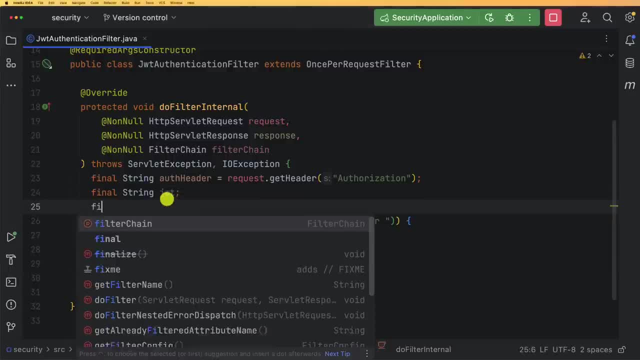 we need to do so. right here, i will just go back. and so, right here, i will just go back. and so, right here, i will just go back and create a final string. create a final string, create a final string. username or email, call it whatever you. username or email, call it whatever you. 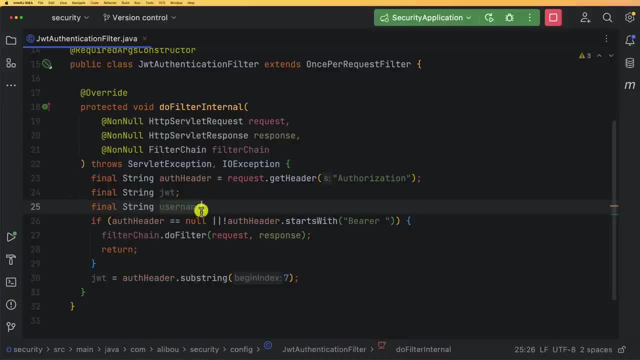 username or email, call it whatever you want, want, want. so i'm just gonna call it user email. so i'm just gonna call it user email. so i'm just gonna call it user email. okay, to be consistent and avoid. okay to be consistent and avoid. okay, to be consistent and avoid confusions, so i will call it user email. 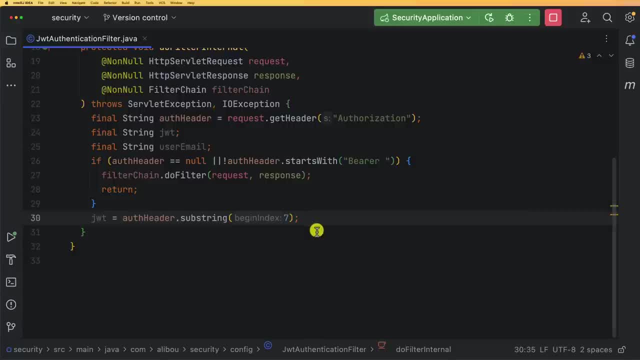 confusions, so i will call it user email confusions, so i will call it user email. so, after extracting the jwt token, so, after extracting the jwt token, so, after extracting the jwt token, what i need to do is: i want to extract. what i need to do is i want to extract. 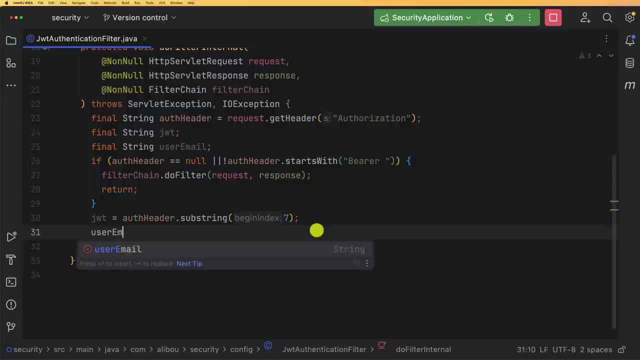 what i need to do is i want to extract also this user email. so this user email equals. so this user email equals. so this user email equals. and here i will add it to do extract and here i will add it to do extract and here i will add it to do extract, the user email. 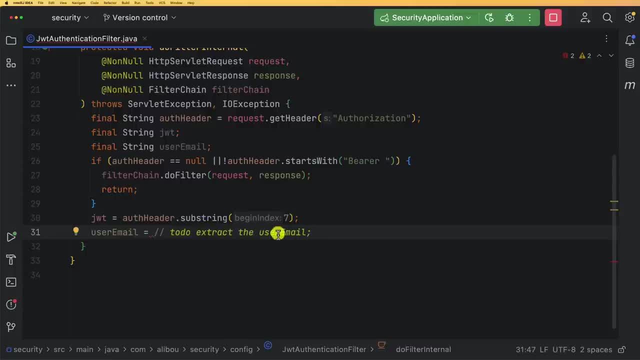 the user email. the user email- okay, but to do so, i need to extract it. okay, but to do so, i need to extract it. okay, but to do so, i need to extract it from: let me add it here from jwt token. from: let me add it here from jwt token. 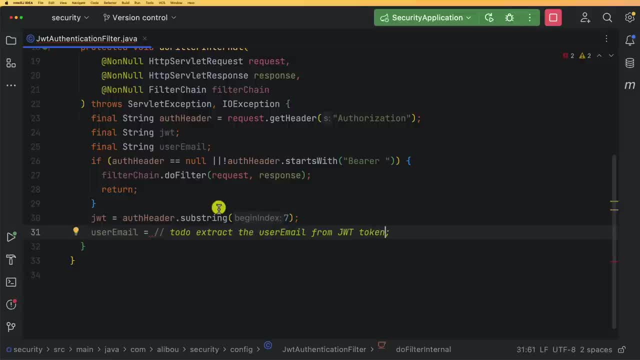 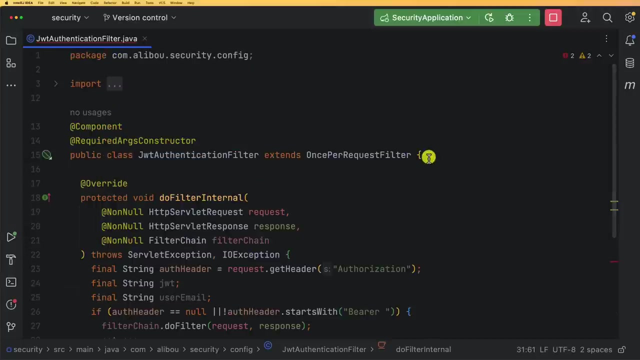 from- let me add it here- from jwt token. so to extract, so to extract for this user email from the token, i need a class that can manipulate this jwt token. okay, so let's try now to implement this class, this class, i will call it here, i will just create my class here. 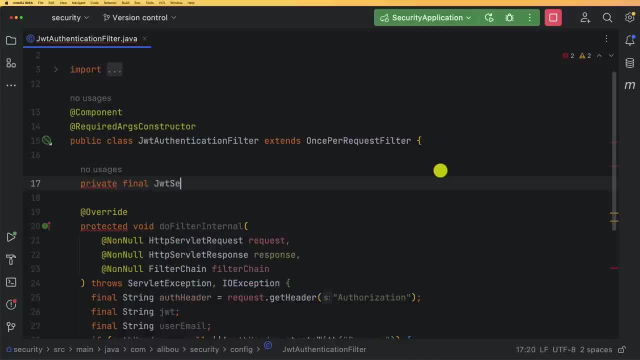 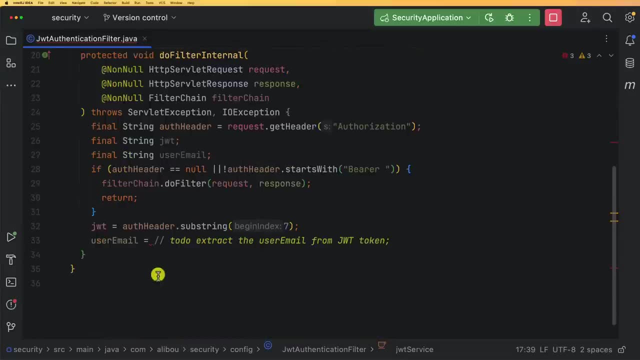 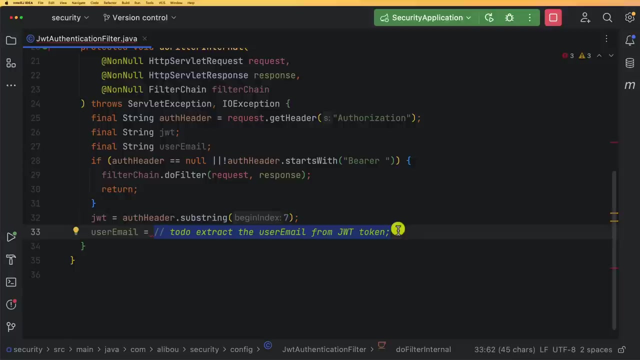 private. final, i will call it jwt service. so i don't have yet this jwt service. but within this jwt service and what i want to do here, i want to use a method that i will call it. for example, jwt dot- extract username. okay, so let me call this jwt service, dot. 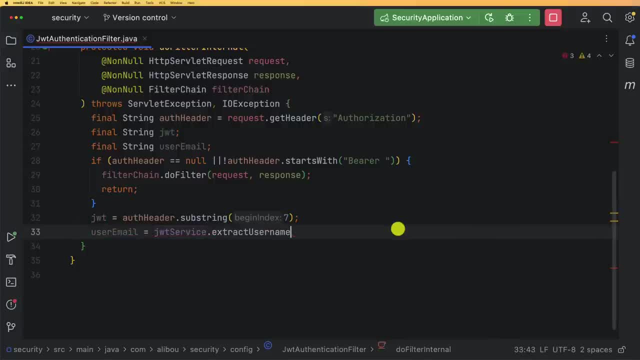 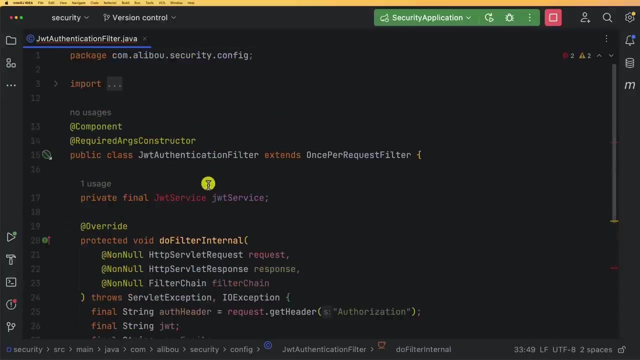 extract user name or user email. okay, let's keep it username within the jwt, because mainly with spring security, we talk about user names and to extract this one i need to pass the jwt as a parameter. okay, so, um, i will create this class. now i will ask uh intelligent to create. 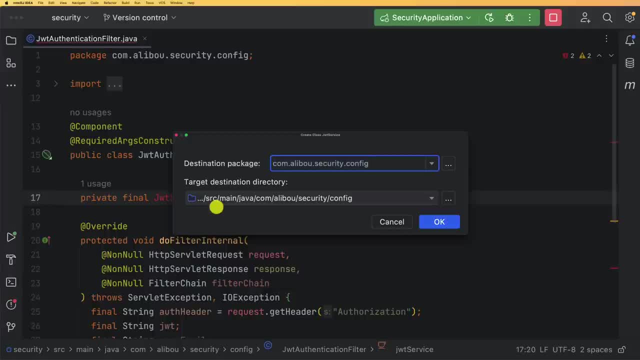 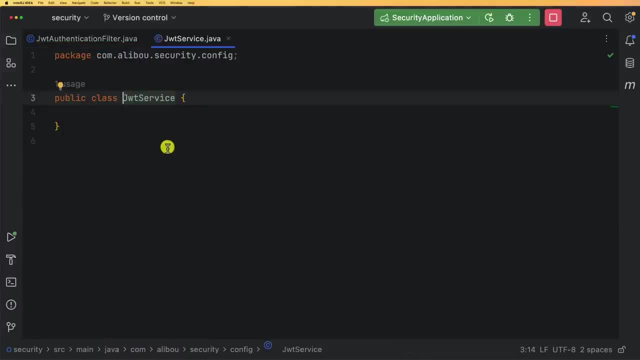 this class jwt service and i will create it. you can keep it, whether with the config, with the config package, or you can move it to a different one. so i will keep it within this package and also, do not forget to add this service annotation to make it or to transform it to a. 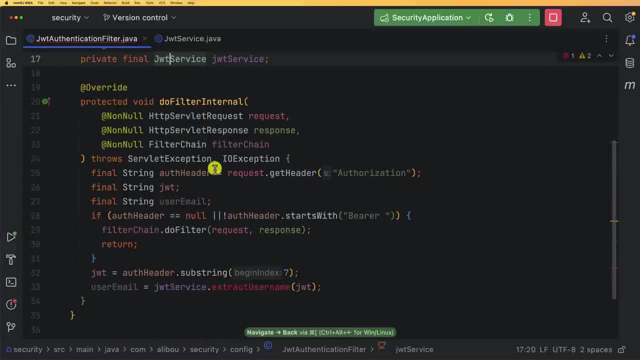 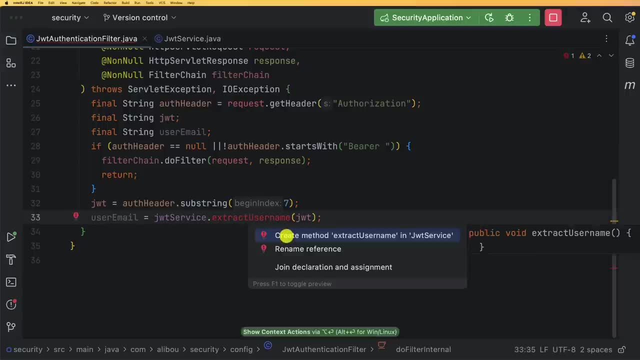 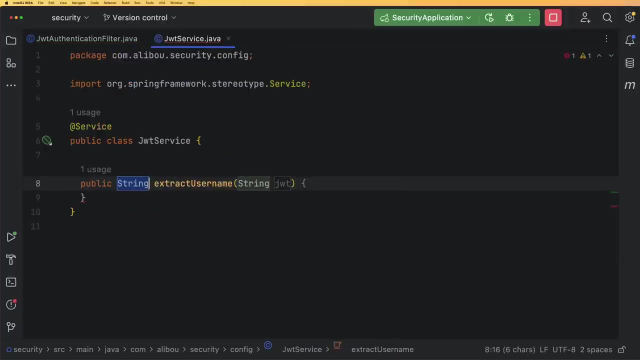 managed bin. all right, so now i will just create this extract username method. so create method: extract username in jwt service. and yes, this is what i want to do. i need a method that will return a string username and it takes as a parameter a string token or string. 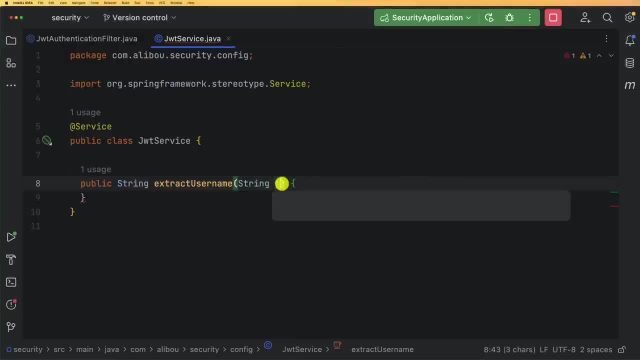 jwt. okay, so let me call this one token- i think it would be better as a name. and yeah, that's it. so i will just return null for the moment and let's move on, and they will show you how we can, how we can implement or how we can extract this information from our jwt service. 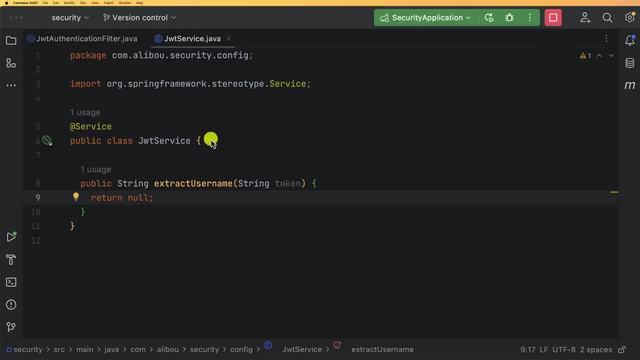 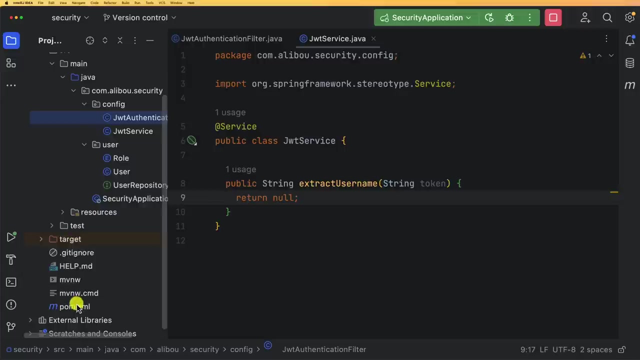 so now, in order to be able to manipulate jwt tokens- generating one, extracting information from the token, validating the token, and so on, so forth- we need to include new dependencies within our application. so let's go open our pomxml file and here, within this pomxml scroll, 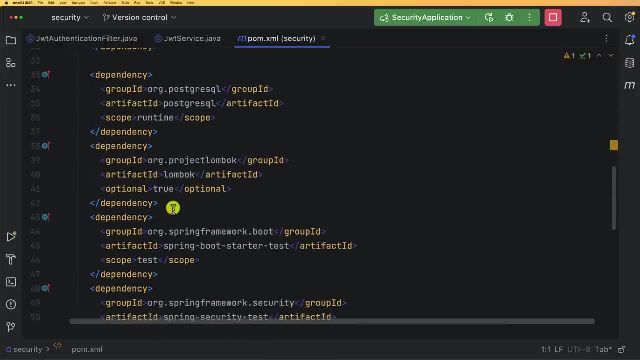 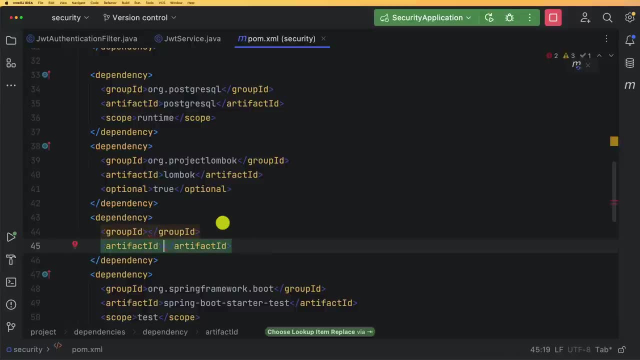 down and go next to the Lombok or PostgreSQL dependency, and here just add a new dependency, and this the first one, called jjwt api, dash api, and it's from a io just dot json web token. okay, and the recent version at this time is the 0.11.5, so let's use this one. we need also to add another. 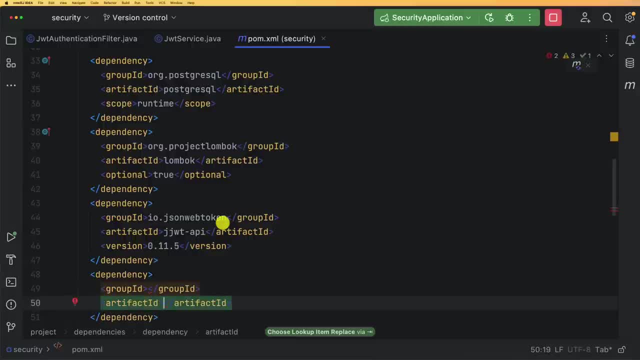 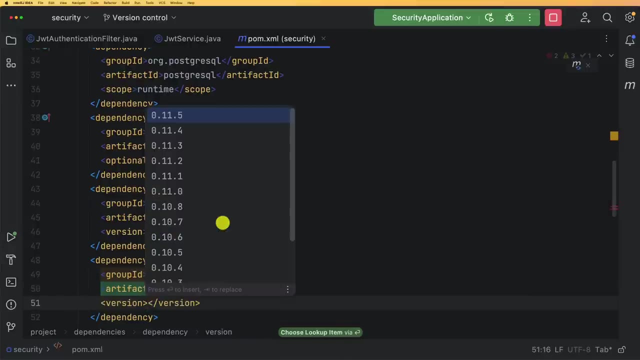 dependency, which is also from the same artifact or from the same group id, but it's a different artifact, so we need a jjwt employee implementation. so it's called jjw wt, amp and from the same group id, also the same version. you can extract this version to uh, to a property and use it from there and 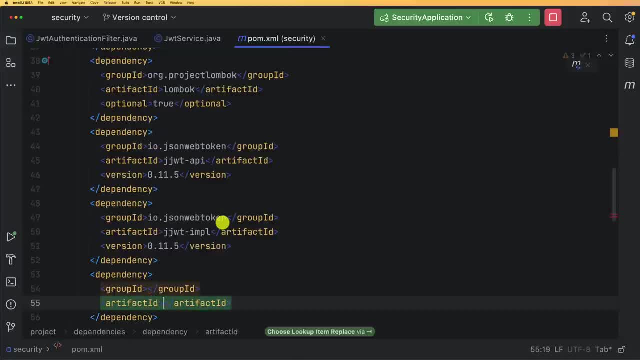 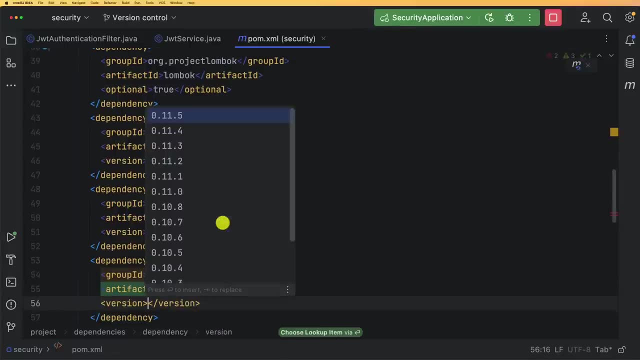 next we need a final dependency, which is the jjwt jackson. okay, so also from the same group id and the same version too. now, once we add uh, or once you add this dependencies or nuke to the jjwt worldjson, we can show that jjwt is already the same json right now, and so if we 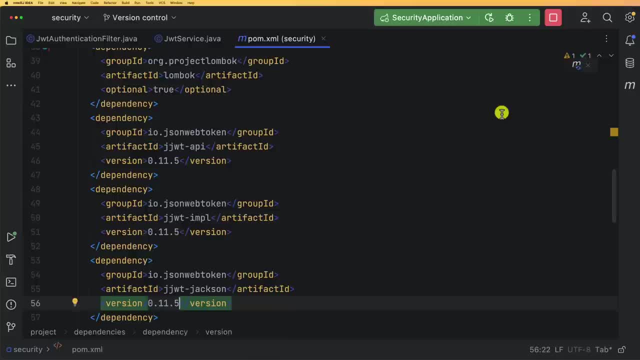 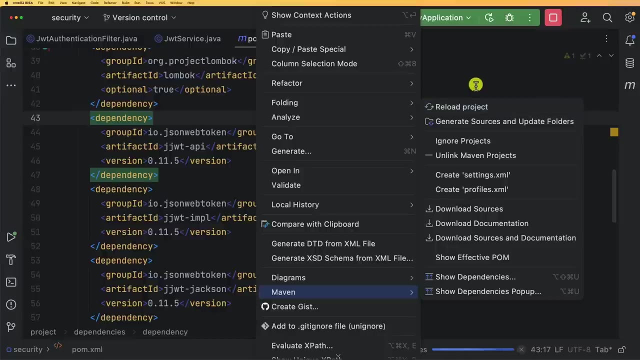 dependency to your pomxml or if you make any updates to your pomxml, make sure you click this button load maven project. but also, if you don't see this button, just right click inside the pomxml file, maven, and then you have the option reload project. okay, so until ej will download all the 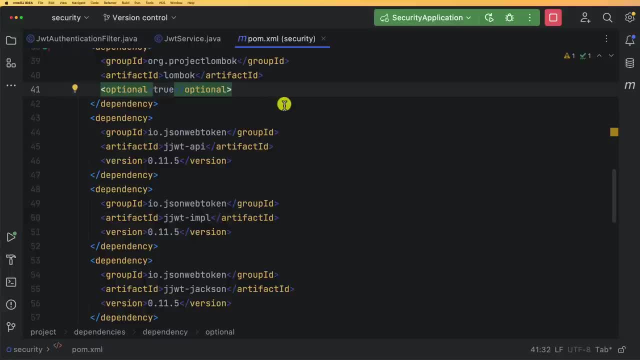 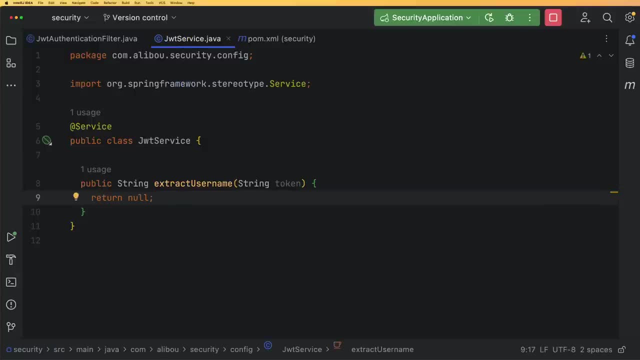 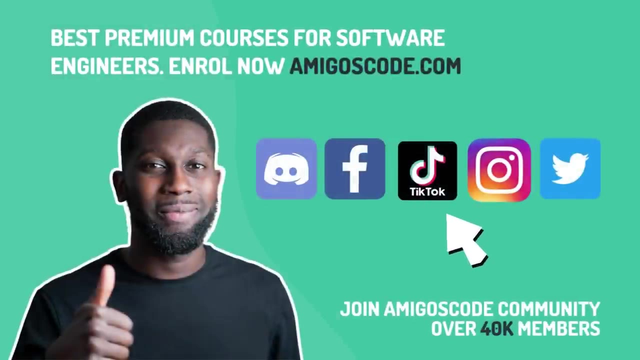 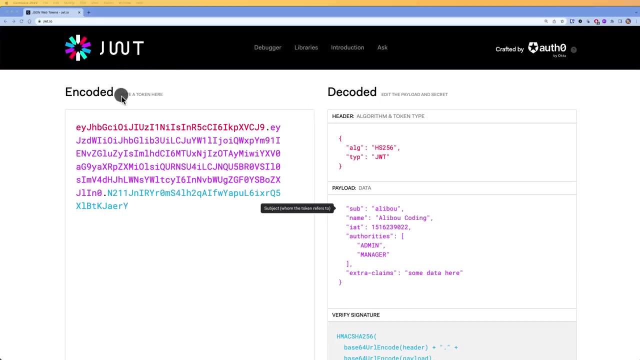 dependencies and add them to the to the class path. all right, so our dependencies are ready to use. now we will go back and implement this jwt service. so before we go and implement all the services and dive too much into the code, let's first try to understand what is a jwt token. so a jwt token stands for a json web token, which is a compact. 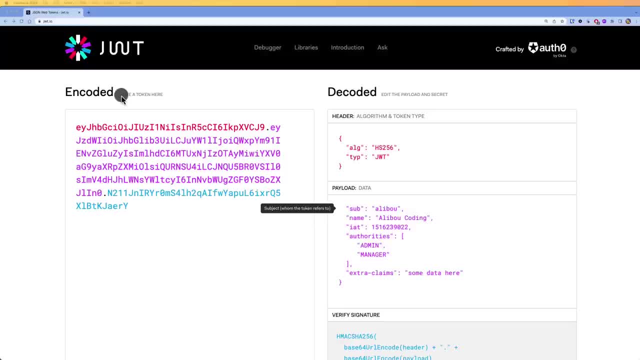 url, save means of representation, of representing claims to be transferred between two parties. the claims in jwt are encoded as json object, that is, digitally signed using a json web signature. okay, so the jwt consists of three parts. so here we have the header, we have the payload and also 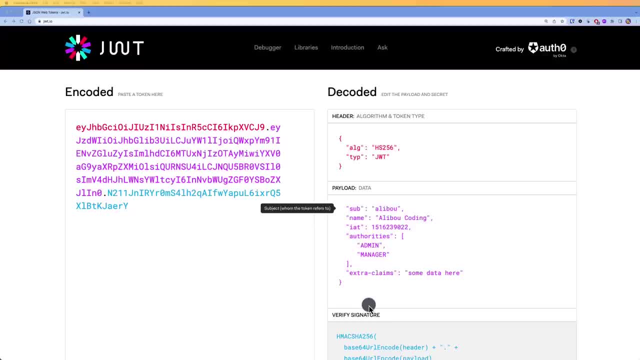 we have the signature, so the header typically consists of two parts which contain the situation. so, as we can see, here we have the subject, we have the name, we have this, i iit, we have. we can have also extra information like authorities or extra claims right here. okay, so there are three types of 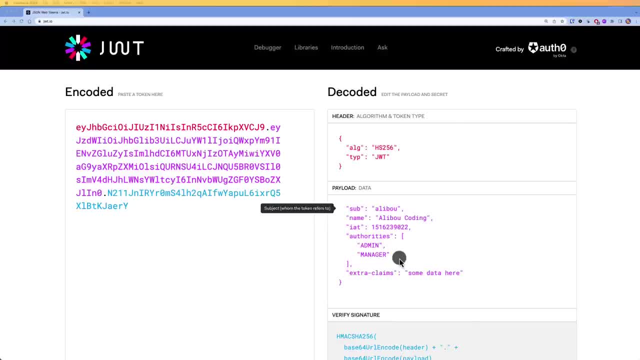 claims: registered public and private claims. the registered claim claims are a set of predefined claims which are not mandatory but recommended to provide a set of useful and repeatable claims. some of the registered claims are: is, are, iss or the issuer. we also have the subject, the, the odd, the x, exp, like the expiration time, and so on, so forth. this we will see when we 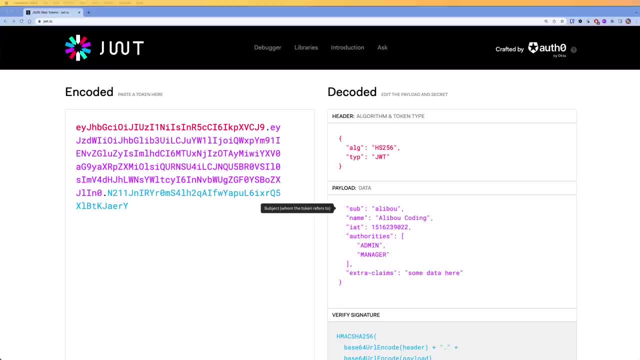 will implement the token generations. okay, we have also the public claims, which are the claims that are the public claims, and the copyrighted claims, which are the claims that are the public claims are defined within the IANA JSON Web Token Registry or public by nature. Private claims are custom claims created. 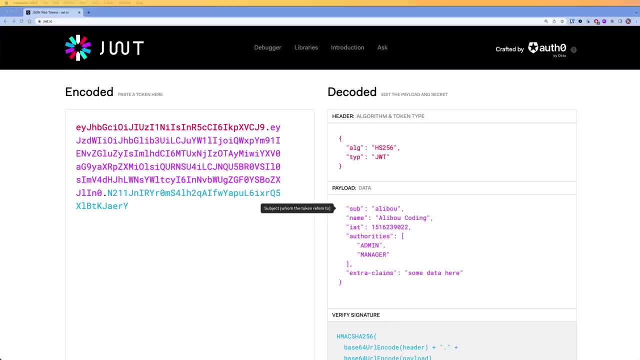 to share information between parties that agree using them. okay, The last one, or the third part of the token is the signature, which is used to verify the sender of the JWT is who it claims to be and to ensure that the message wasn't changed along the way. okay, 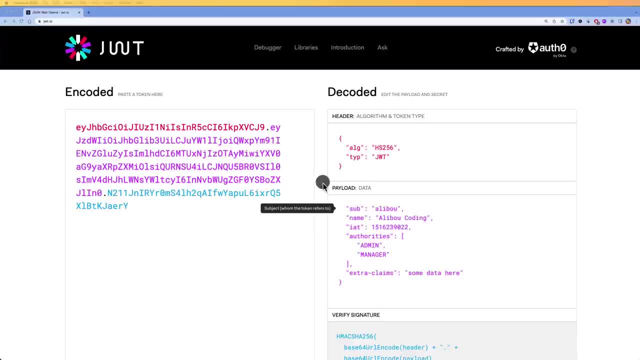 So now let's move on to the code and see how we can generate or how we can extract claims from this JWT token. okay, So also within this jwtio website, you can play with the payload, you can add some information here and, as you can see, every time you add something, 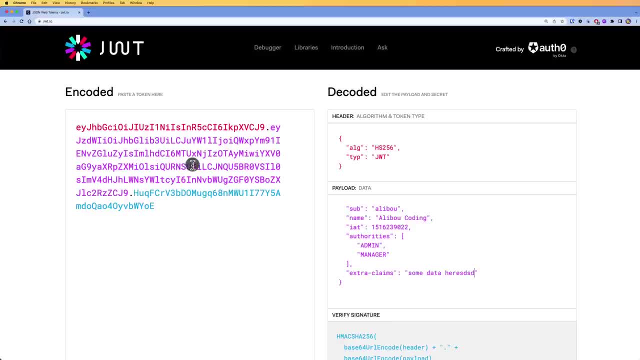 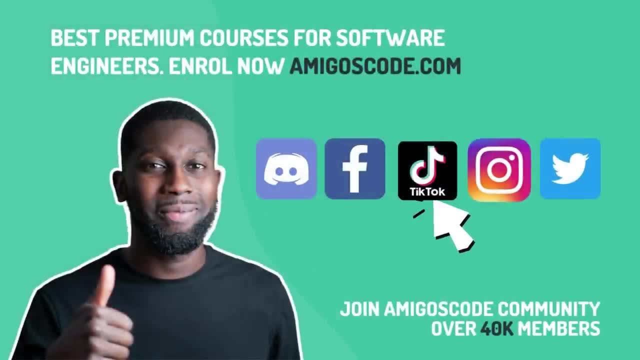 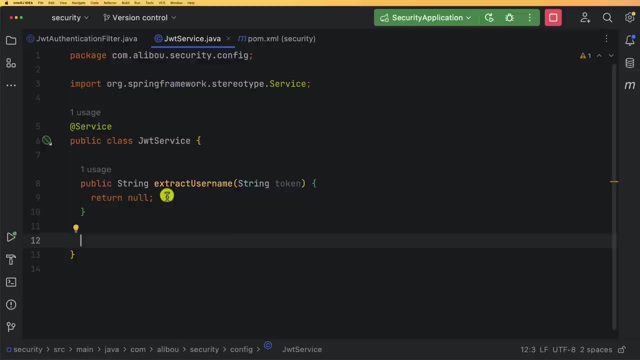 you see that it changes right here. okay, Let's move on and go back to our code. Now, before start implementing this extract username method, I want to implement or write some code to extract all the claims and also another method that allow us. 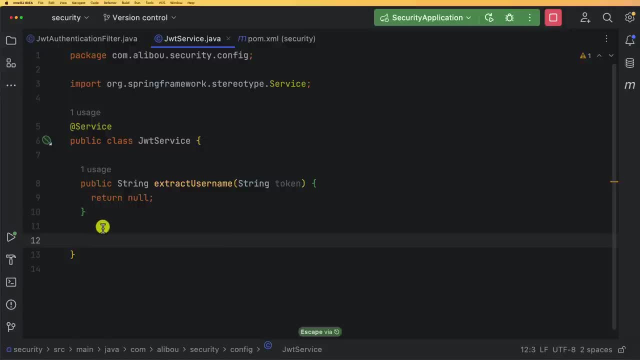 to extract one single claim, okay. So first of all, I want to create this method. I will. it will return a claim And this claims, if you see right here, when you click on import class, it's the one from iojsonwebtokenclaims. 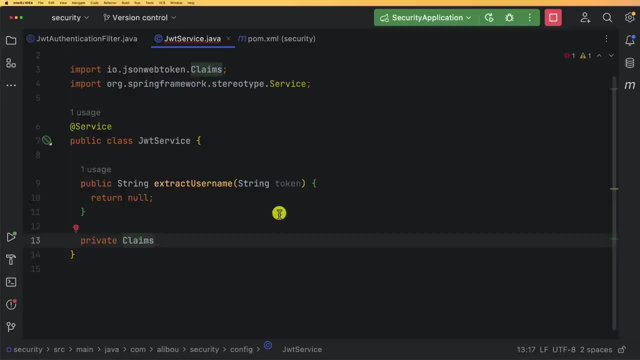 It's the dependency that we just added. So this claims: I will call this method extract all claims. Okay, so this extract all claims, of course it will take a string token as parameter, And now I will show you how to extract this. 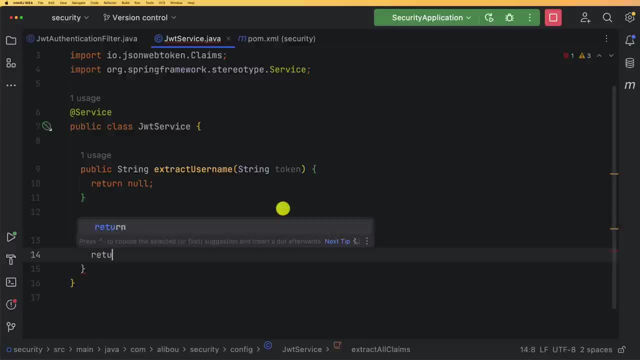 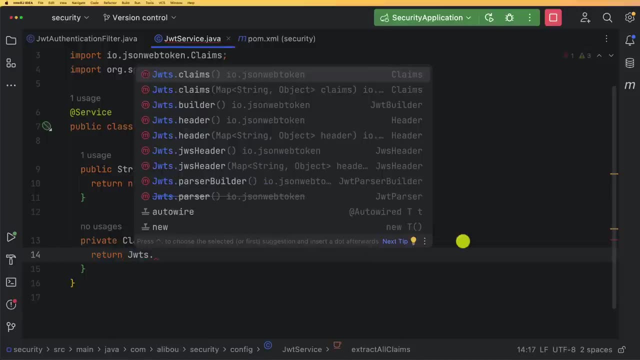 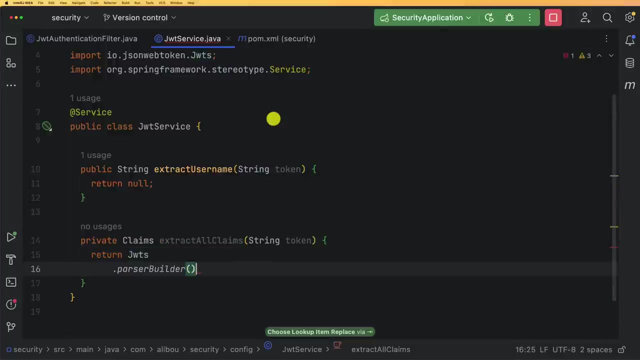 So to do it, we need to return our JWTS, And this JWTS is also from. so this JWTS is also from the iojsonwebtoken And we need this JWTSparseBuilder And in order to parse this builder or to parse the token, 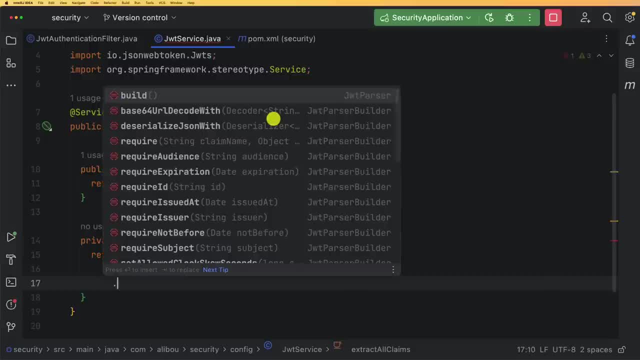 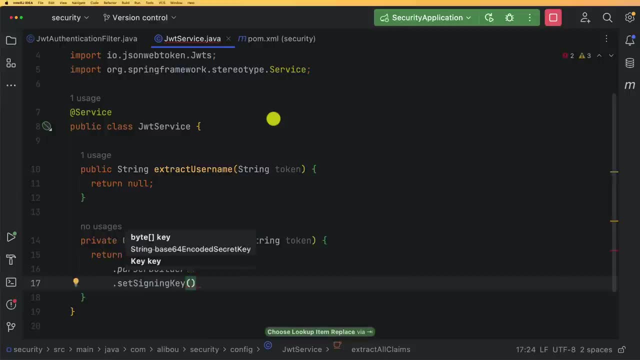 and here we need to set the signing key. okay, Set signing key, because, as we mentioned before, when we try to create, to generate or to decode a token, we need to use the signing key. So I will here just let call this one: get signing key. 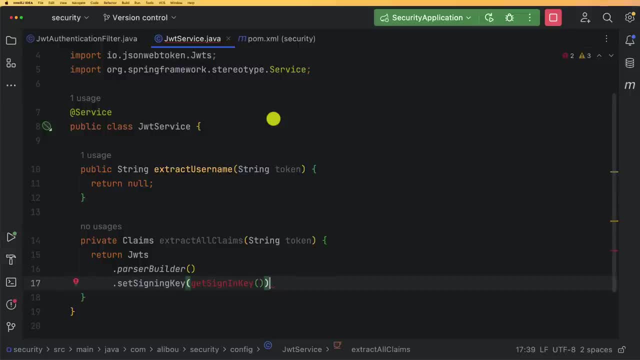 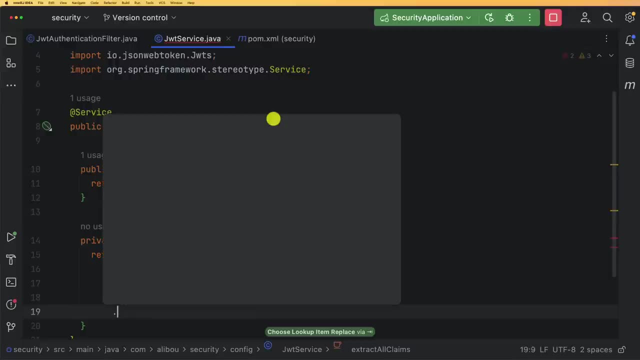 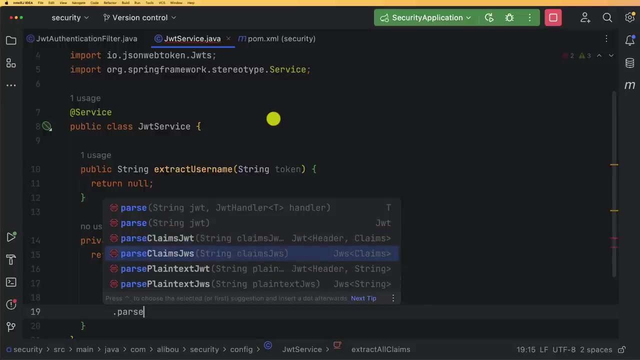 And I will explain it later on. We will implement this method And then we need to build, because it's a builder, And once the object is built, we can call the method: parse claims JW, JWS. Okay, So this one, this method, parse claims JWS. 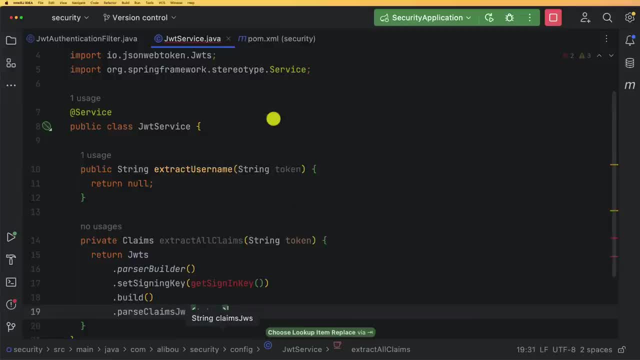 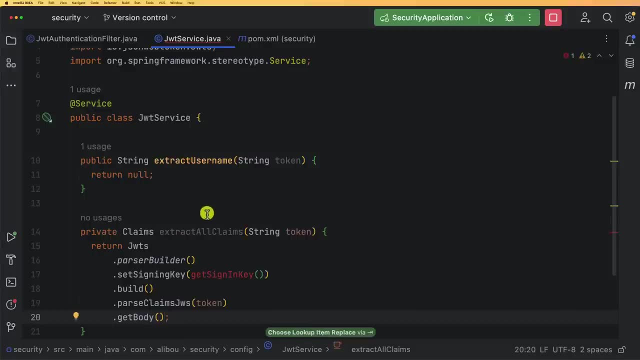 So we want to parse our token And once the token is parsed, we can call the method get body. Okay, So within the get body we can get all the claims that we have within this, this token, right here. All right, 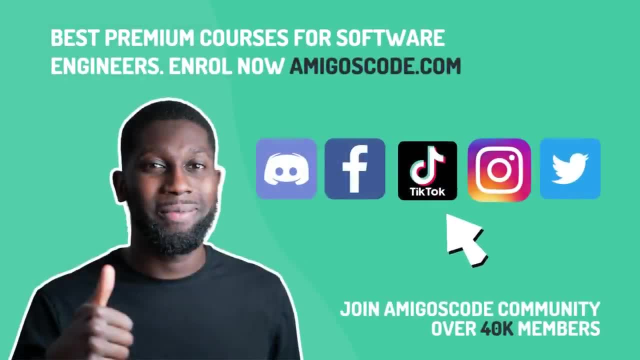 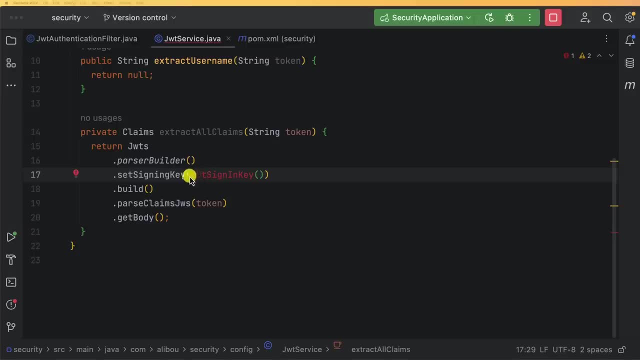 So now I will show you how to do this. We are going to use the sign in key method, So let's start with the sign in key method. So now, before we implement this signing key method, which should return a key, as you can see in the definition here. 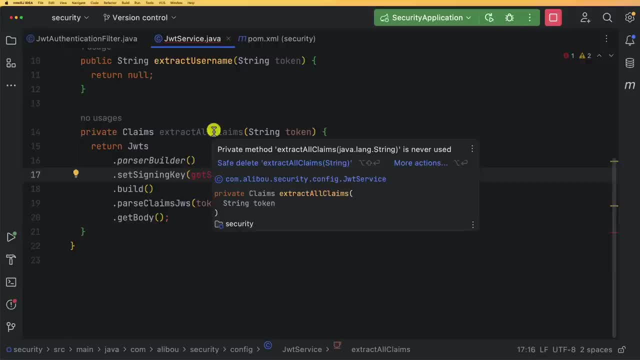 So this one. let's first understand what is a signing key. Okay, So in the context of JSON web tokens, a signing key is a secret that is used to digitally sign the JWT. The signing key is used to verify that the sender of the JWT 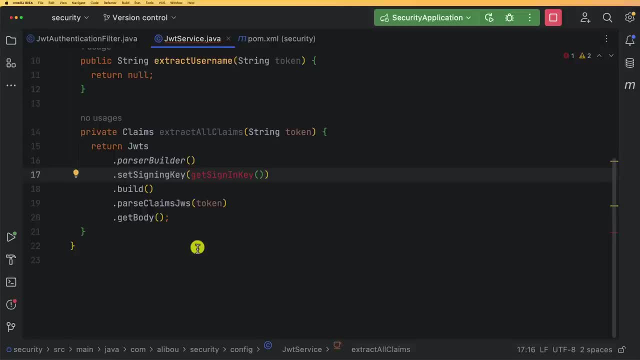 is who it claims to be and ensure that the message wasn't changed along the way. So we want to ensure that the same person or the same client that is sending this JWT key is the one that claims who to be. Okay, So the signing key is used in conjunction. 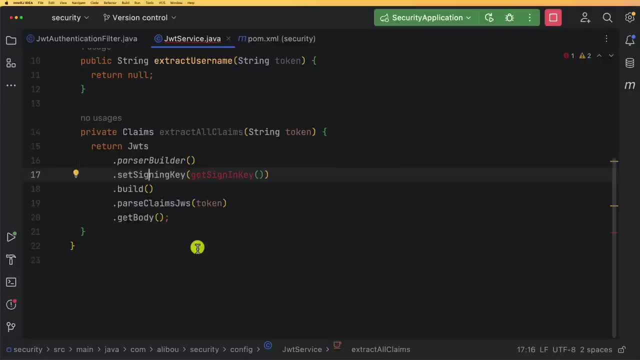 with the sign in algorithm specified in the JWT header to create the signature. The specific sign in algorithm and key size will depend on the security requirement of your application and the level of trust you have in the sign in party. Okay, So here in order to do that. 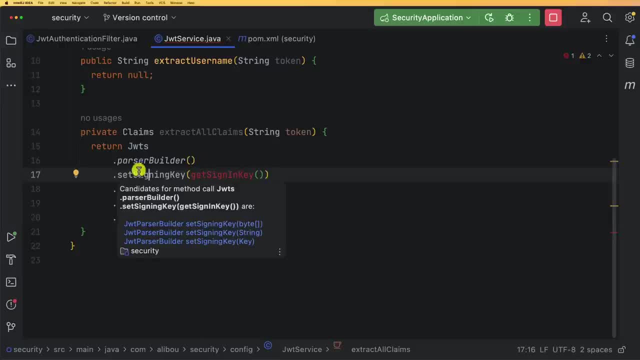 first of all, we need to go ahead and generate a new token or a new signing key or a secret secret key. Okay, So to generate this secret key, we can do it online, because now we like, for security reasons, we need at least, or like, the minimum. 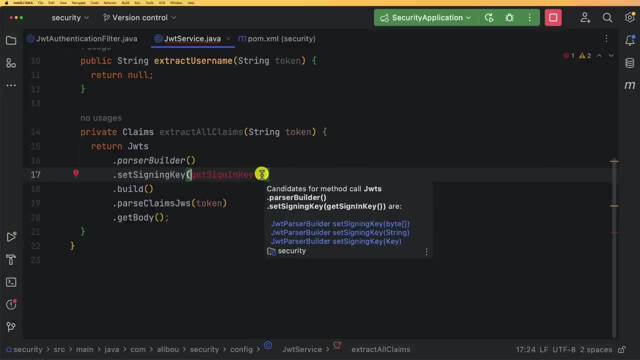 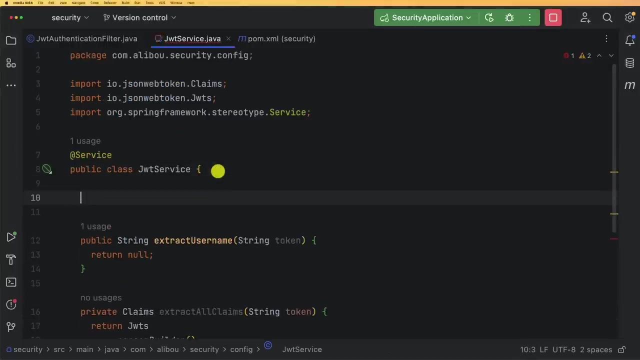 a signing key of size 256.. Okay, So, and in order to generate a key, so you don't need to worry about this, there are so many tools and online tools to do this, So here I will just go ahead and create. 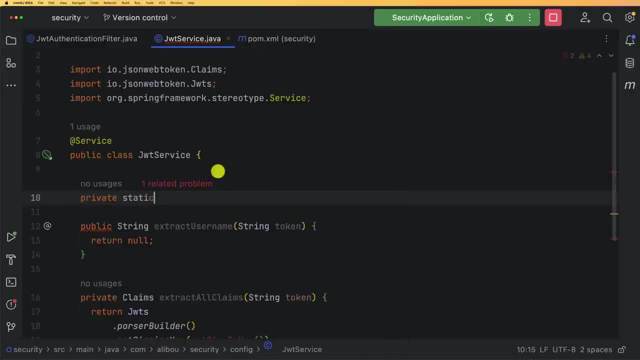 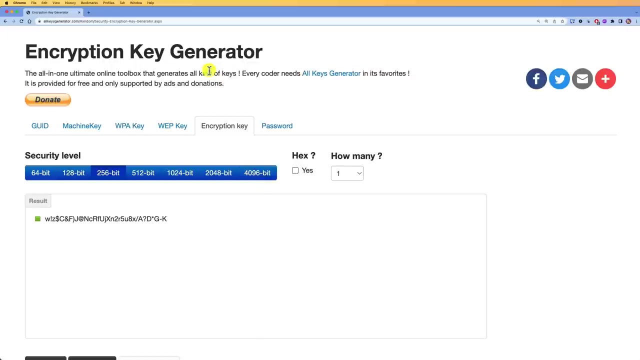 a private static final string. I will call it secret key, And this secret key equals the value that I will generate right now. Okay, So now go to the browser and navigate to this address, which is allkeysgeneratorcom, and then slash random slash security encryption key generator. 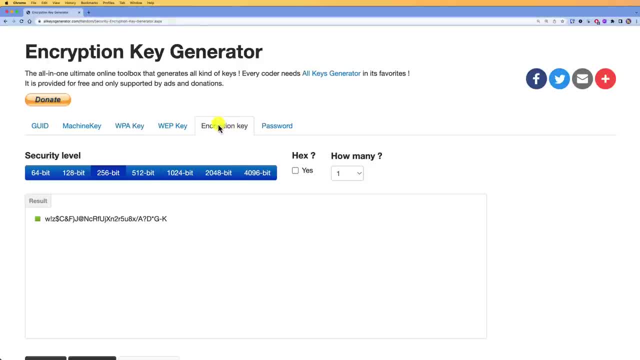 dot aspx. Okay, And we have here encryption keys and here we have also the security level. So, as I mentioned, the minimum required for JWT tokens is 256 bit. Okay, And then click on this checkbox. Yes, The X, make it, check it and make it yes. 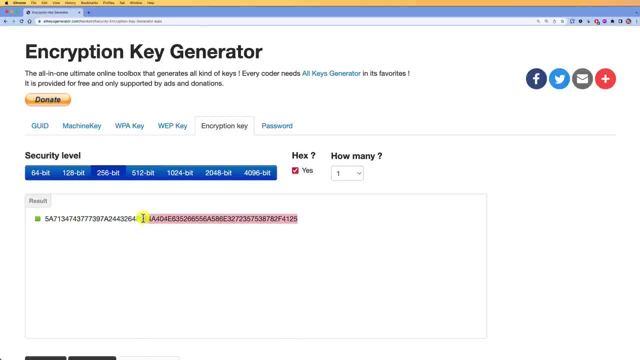 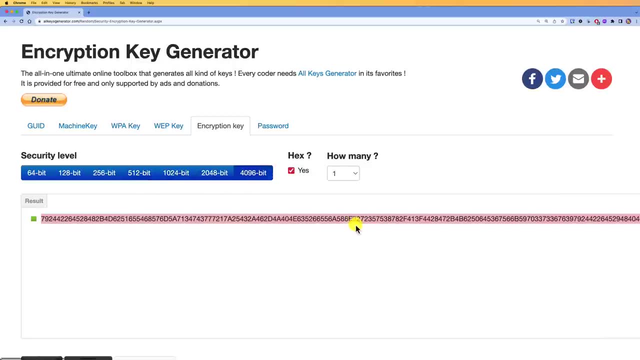 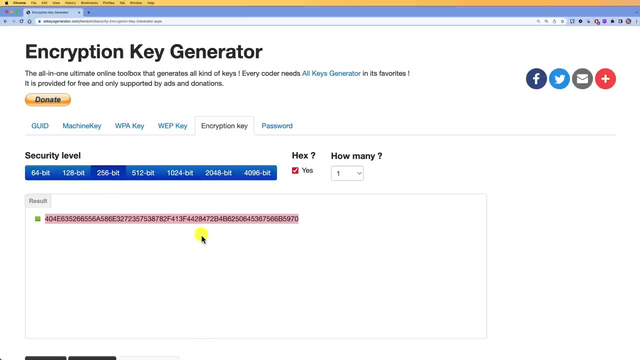 So we can get this X X secret key. Okay, So if you need more security, just go ahead, change it and do like. you can go even up to 4096.. Okay, But for now, for the sake of this tutorial, 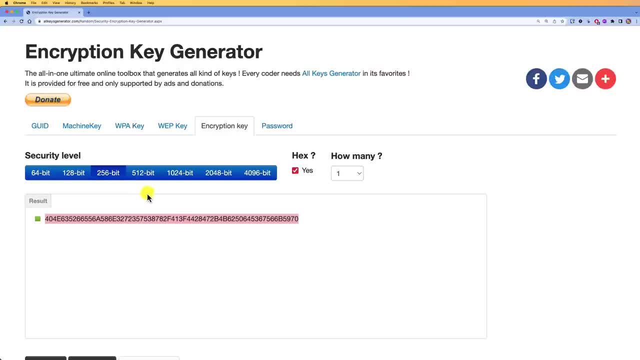 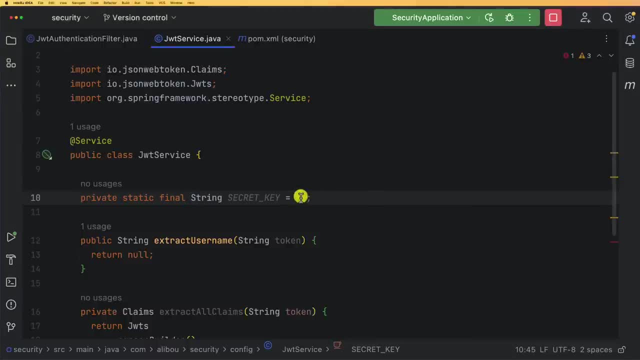 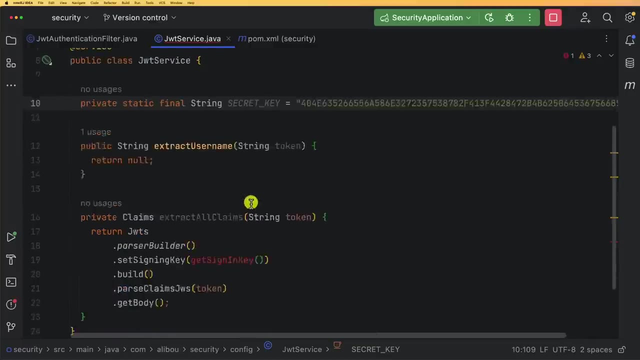 I will just make it or leave it to 256 bits. Okay, Now let's go back to our code and paste this code right here, or this key right here. Also, you can move it to the application properties and use it from there. 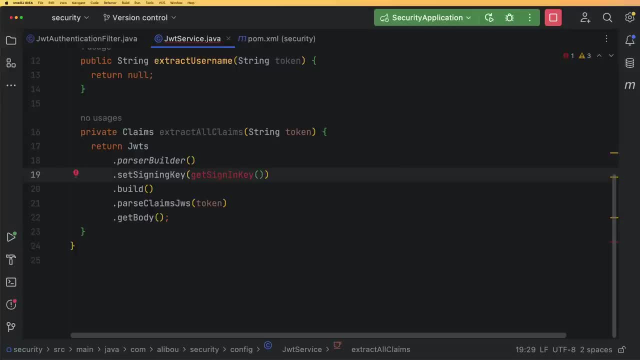 All right, Now let's continue and let's implement this. get signing key. So here I will use IntelliJ to do that. Okay, IntelliJ to auto generate or to create this method. So I will ask him to create this method, and this method should return, not byte. 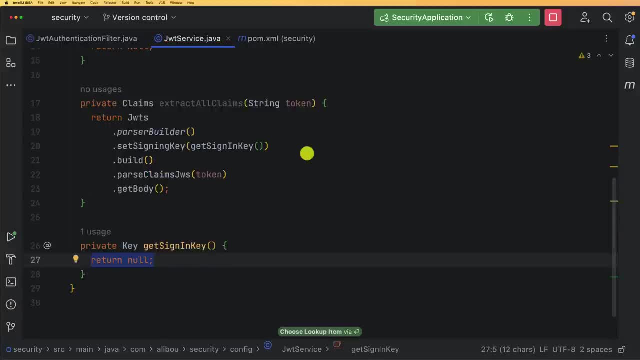 but it should return a key. Okay, So now, to do this, first of all I need to create or to make an object or a variable of type byte. I will call it key bytes, And this one equals decoders and the dot. 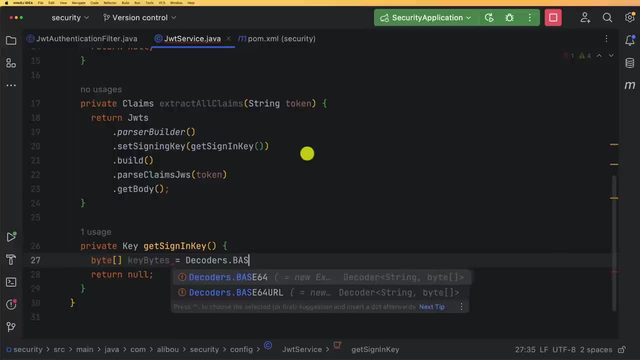 Base 64, because it's a base. we want to decode it on base 64 dot decode And we want to decode our secret key. Okay, So, once the secret key is decoded, now I need to do just to return keys dot, H, M, A, C. 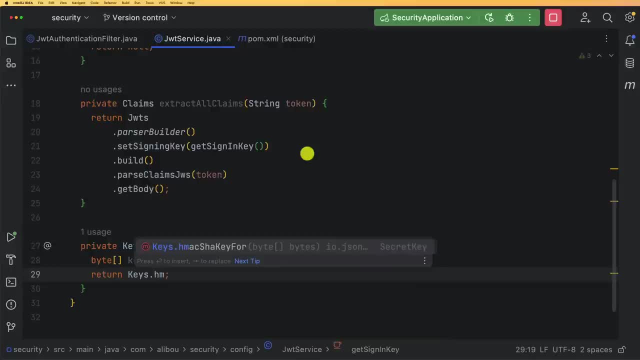 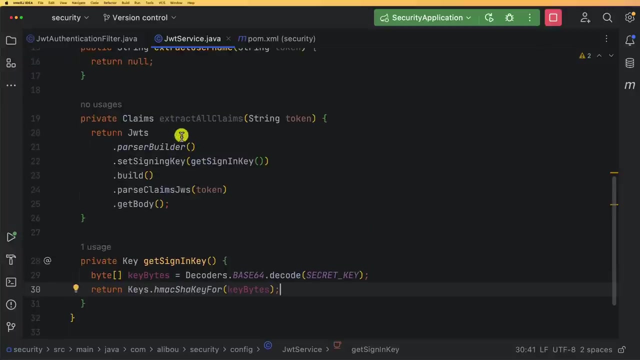 SHA key four. This is one of the algorithms that we mentioned before, And all I need to do is to create this key. Okay, This is to pass this key bytes Right. So now we have our get signing key methods, and we have also this extract all claims method ready to use. 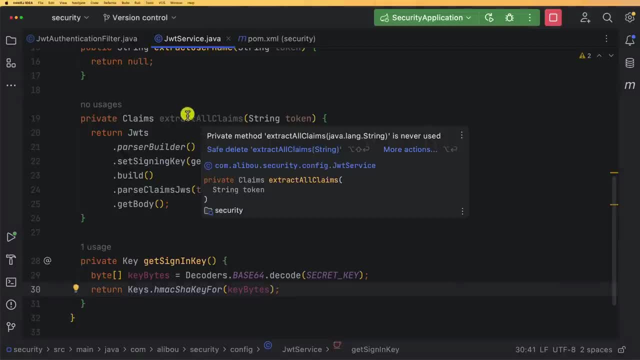 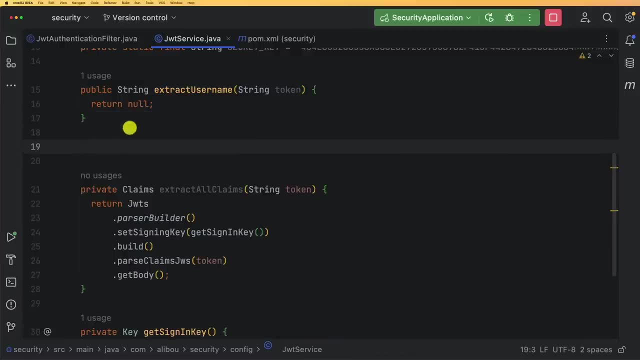 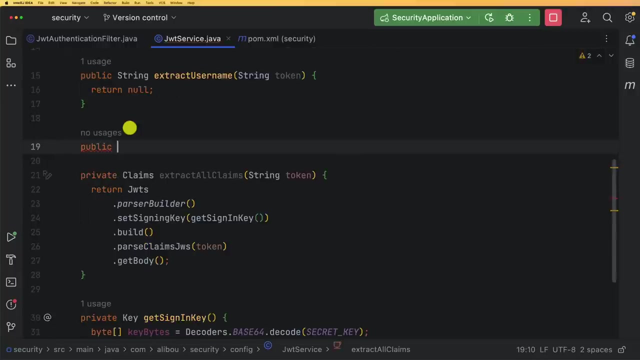 Now we have extract all claims method ready to use. Now we'll go ahead next and implement another method which will allow me or which can extract a single claim that we pass. Okay, So I would use generosity for this, So I will use a public T it. 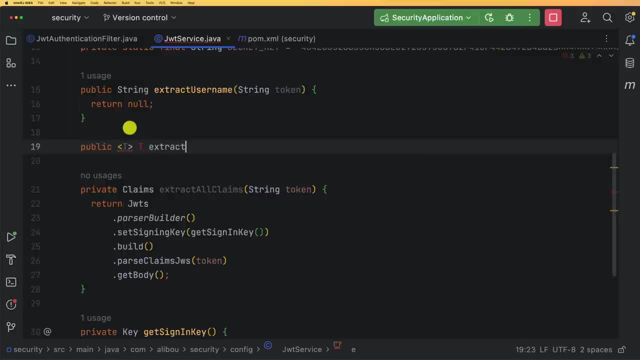 I want it to be a generic method and they will call it extract claim. And for this claim I need of course the token, the key token or string token. And then I want to pass a function, the one from Java utils. 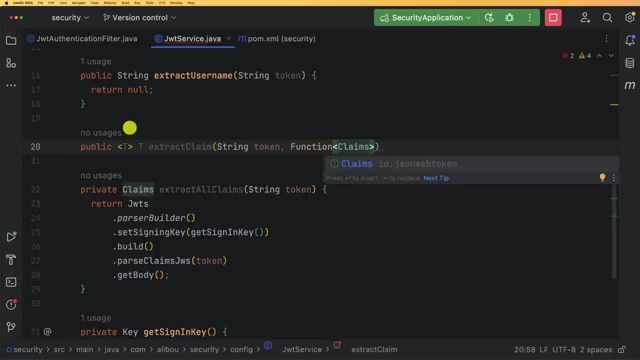 And then I want to pass a function, the one from Java utils, And then I want to pass a function, and this function is of type claims and T, which is the type that I want to return. Okay, I will call it claim resolver or claims resolver or claim, call it. 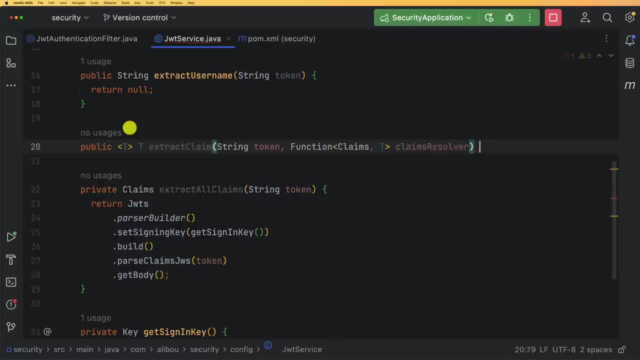 whatever you want resolver, And here it's an. it's a simple. it's a simple method. I will create a final claims object. I will call it claims equals. extract all claims from my token, Okay. So first of all, I want to: 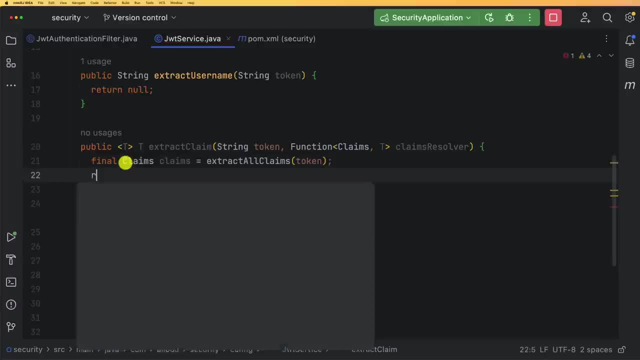 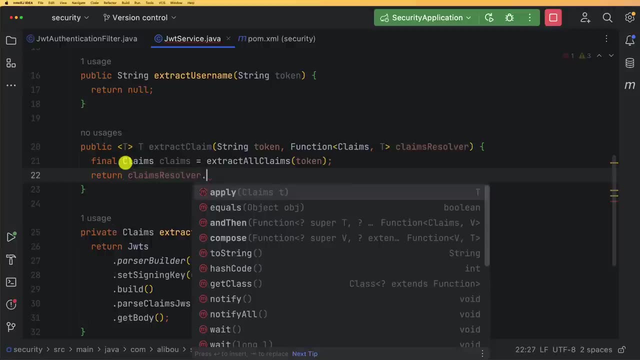 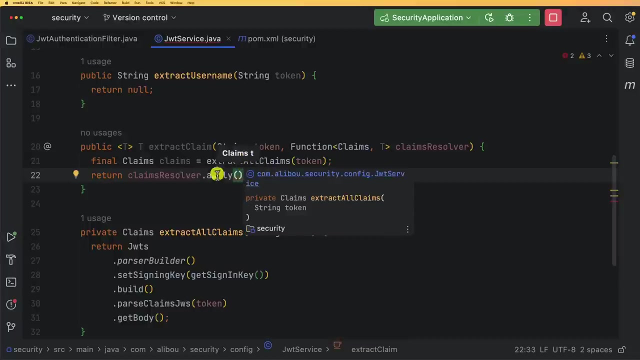 extract all the claims and then I want to do return this claim resolver, the function that I pass as parameter, dot apply, And, as you can see, the apply it will take or it will require a claims T. So the claims is the one of the list of all the claims that we have. 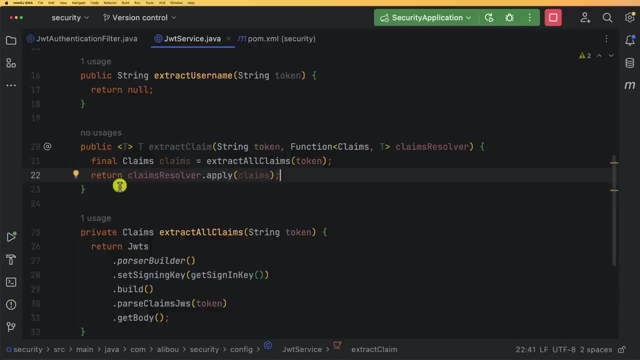 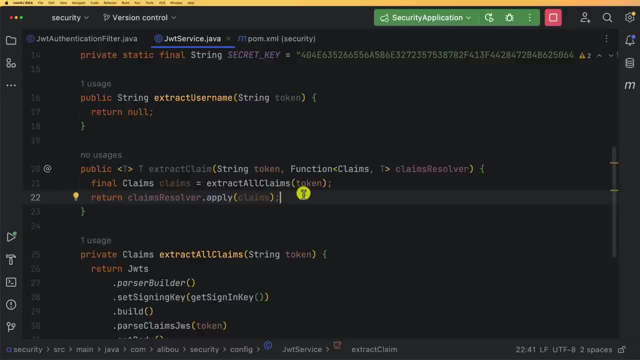 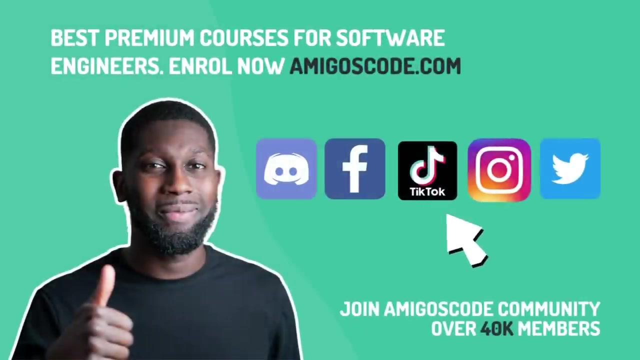 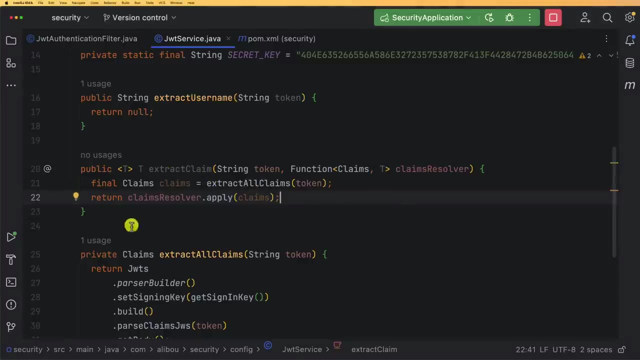 Okay, So this is the extract or claims, all claims method. Now extracting any claim from my token will be an easy peasy task, So I will show you how to do that. So, once I have everything ready, extracting all the claims and also extracting one single claim, 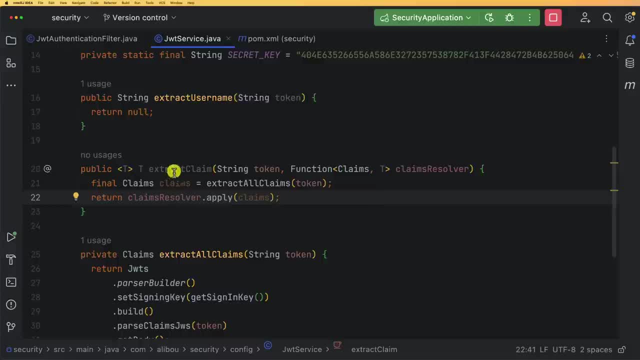 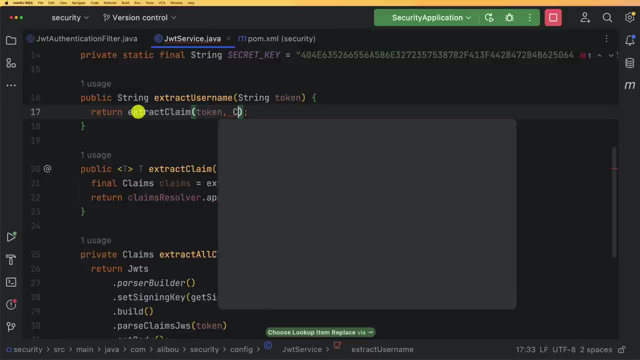 let me show you how we can extract the username out of this token. Okay, So extracting a username is easy peasy, So it will be extract claim and we need to pass the token. And only we need to pass the claims, dot get. subject: 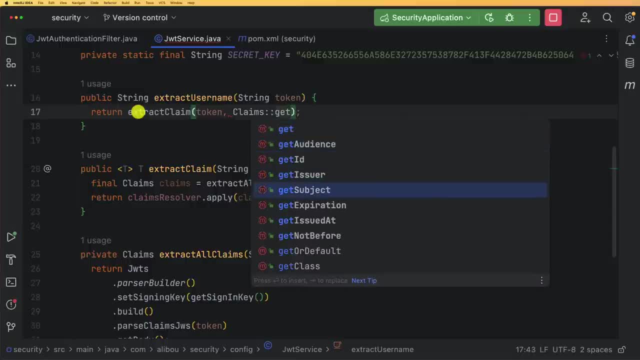 Okay So, because, as I mentioned before, the subject is, or should be, the email or the username of of my user. Okay So, this should be the subject of of the token. So that's it. This is only all about extracting the username. 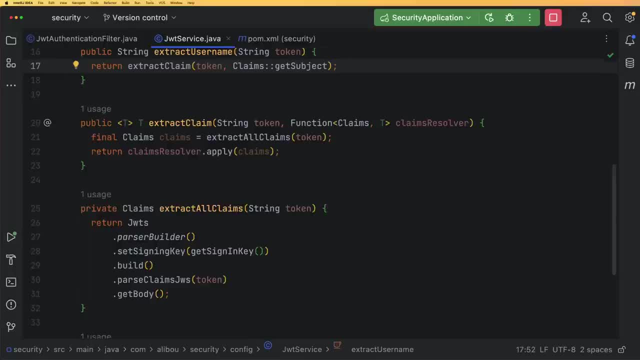 Uh, let's now move on And try to implement other methods that we will need within this JWT service class, like testing If the token is expired, also um extracting the expiration date, generating the token, and so on, so forth. 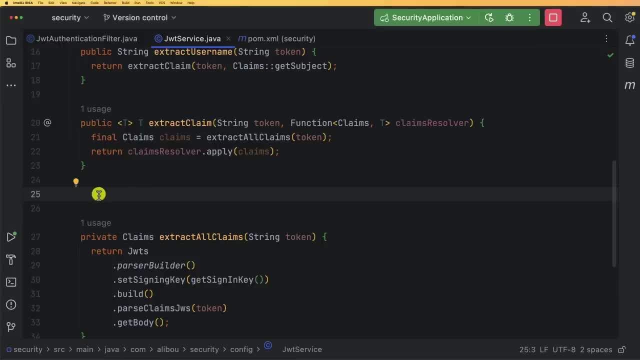 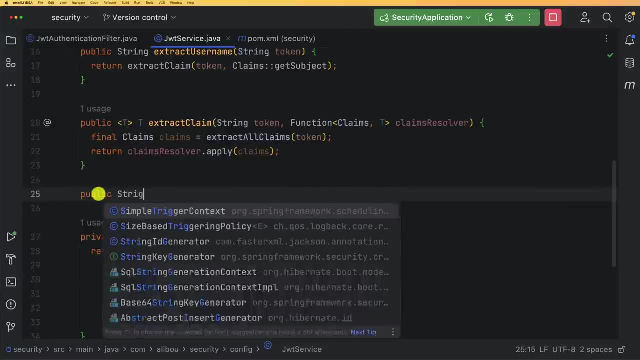 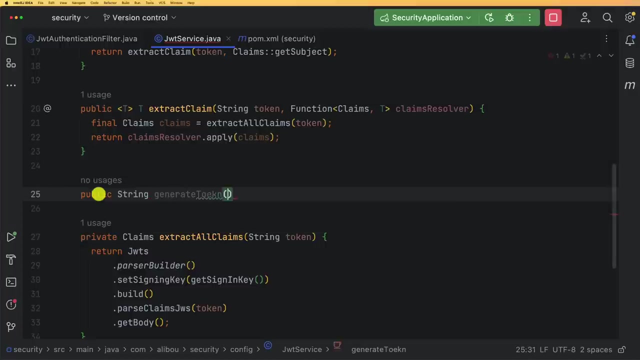 Let's now implement the method that will help us generate a token. So the token, as you know, is a string. So I will create a public string method and I will call it generate token. All right, So this generate token will take as parameter: 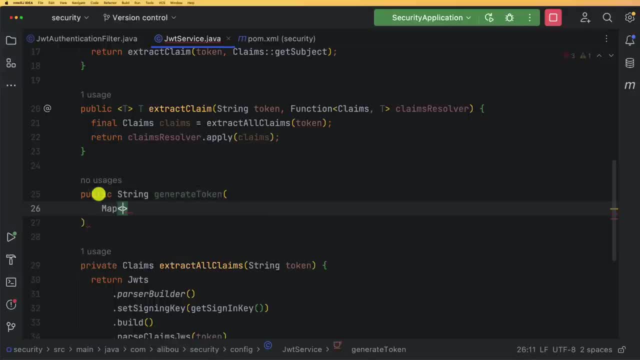 a map, a map of string and object. Okay, And this map of string object will will contain the claims or the extract claims that we want, that we want to add. Okay, I will call it claims or like extract claims. 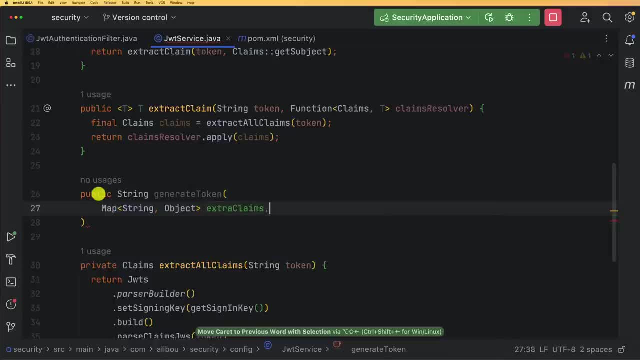 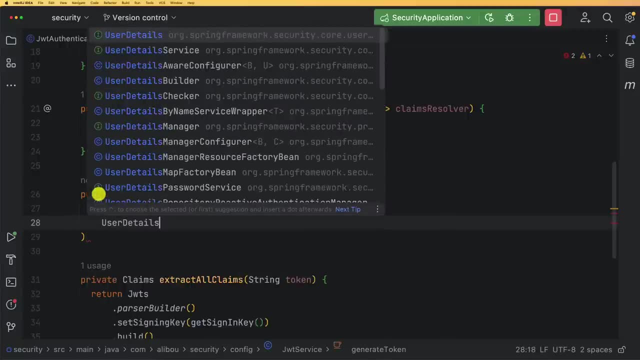 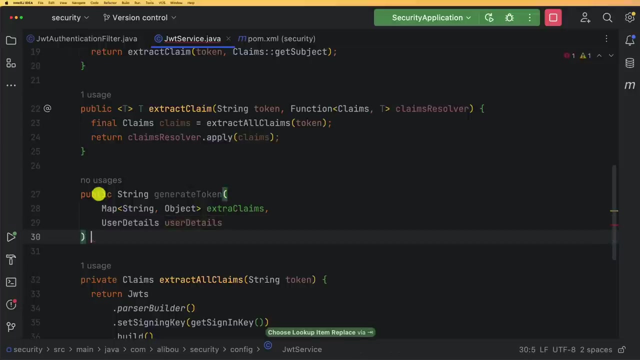 I think it's better to call it extra claims, And also I want to pass my user details. So here, user details, and it's the one from the spring framework. I will just call it user or user details, All right. So this is the method and here this extract claims is the one. 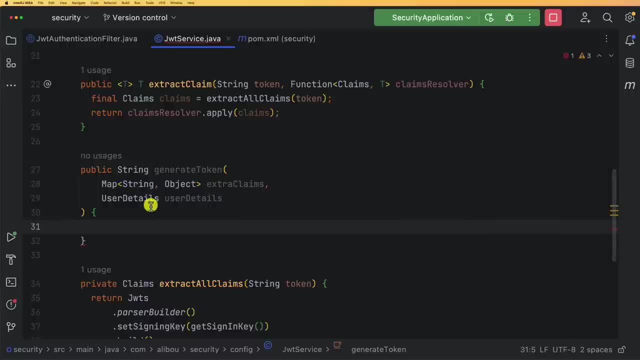 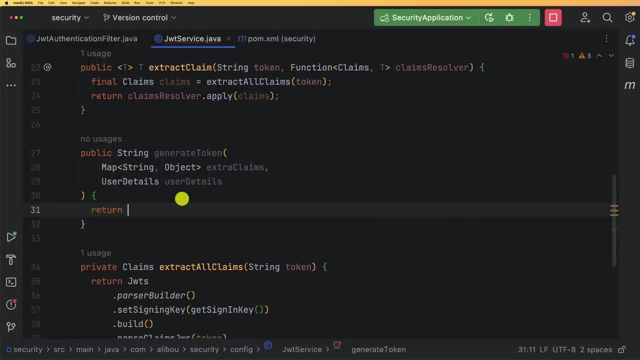 if I want, for example- I don't know- to pass authorities to pass any information that they want to store within my token, All right. So to do this, it's easy peasy, It's just return J W T S dot builder. 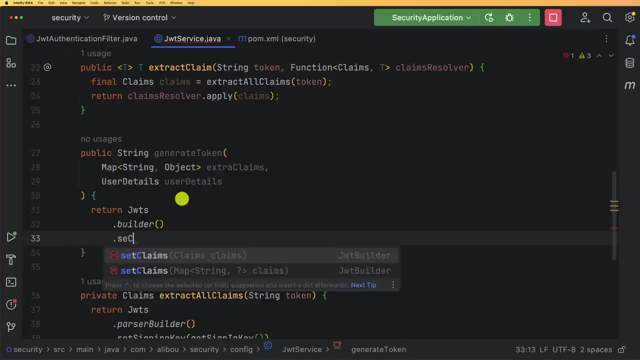 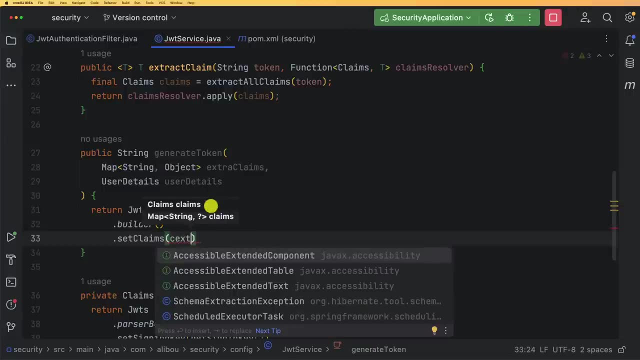 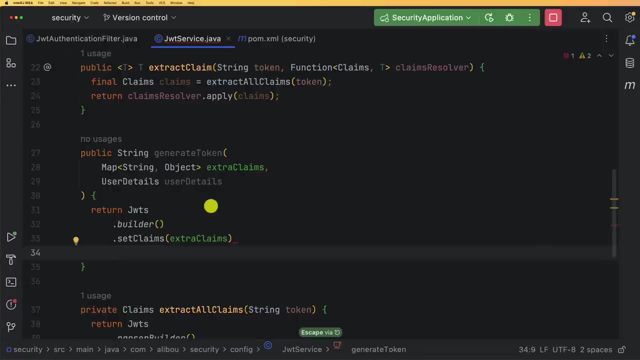 And then I want to set my claims. So these are my claims and those will be the extra claims. Okay, So extra claims And after passing the claims, I need to set my subject. So the subject, as I mentioned before, it should be my username or user email. 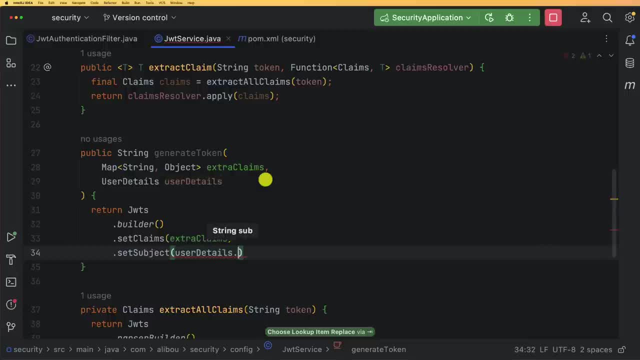 Okay, So I will use the object user details dot. get user name. All right, So because for us the username or the unique part of the user is the email, but for spring it's always called username. That's why we are using username. 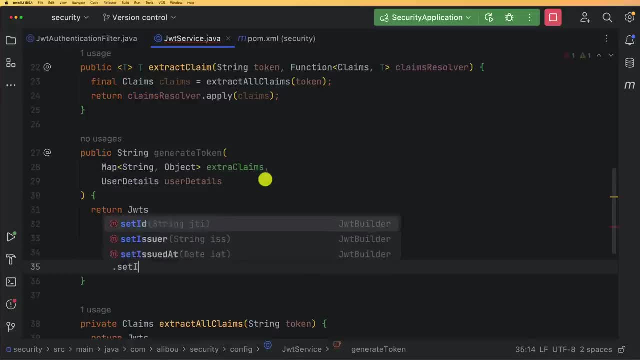 Okay, So, also, we need to set the issued at means, the when this claim was created, and this information will help us to calculate the expiration date or to check if the token is still valid or not. Okay So, uh it. 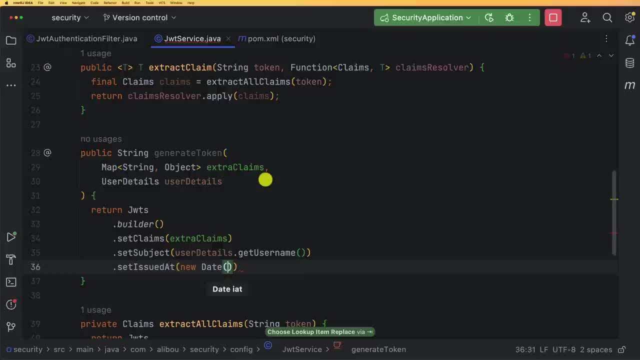 I will use a new date right here and I will pass just the system dot current milliseconds. Okay, So this is the, the issue, the issue date, And I want also to set the expiration date. So the expiration date it will be the same new date and here: 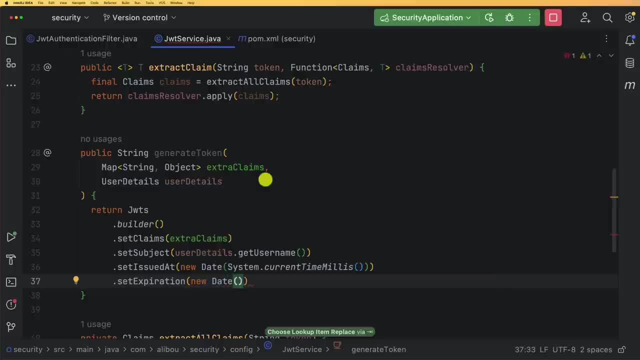 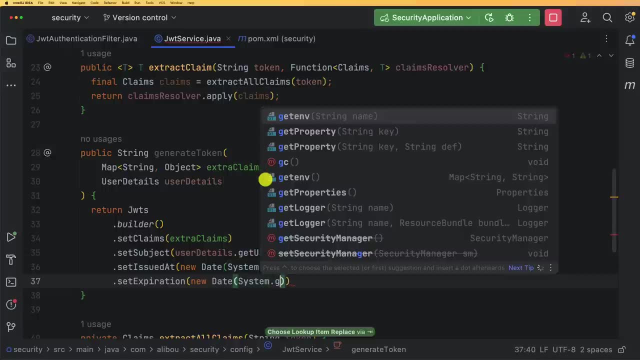 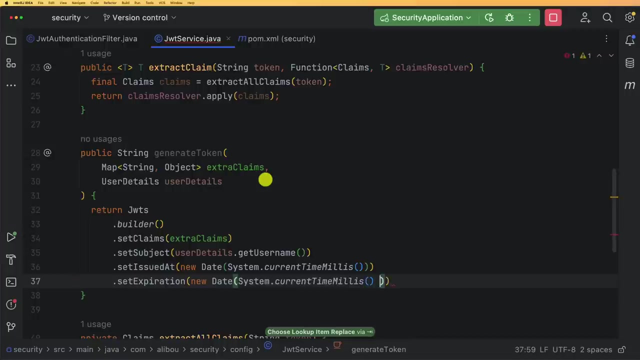 like it's up to you to set how long this token should be valid. Okay, So also system dot, get dot current milliseconds. And then, for example, I want to add um, let's say 1000 times 60,, which is 60 minutes times 24.. 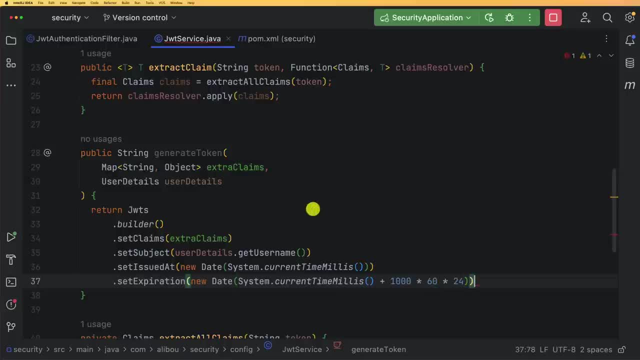 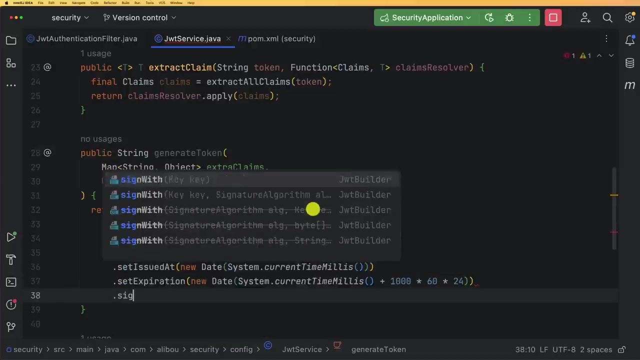 So my token, for example, will be: will be valid for 24 hours plus 1000 milliseconds. Okay, And then you can. you can decide, or you can set any expiration date that suits you. Okay. The final step is to sign with like which key that we want to use to sign. 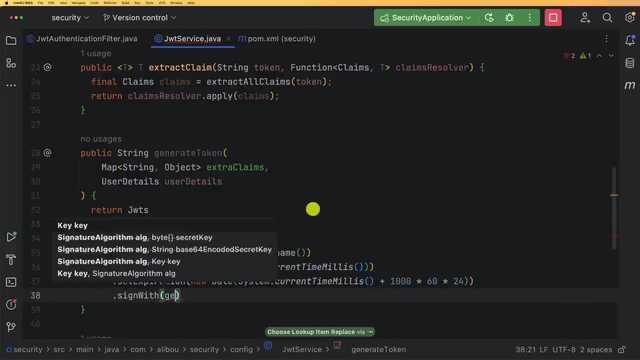 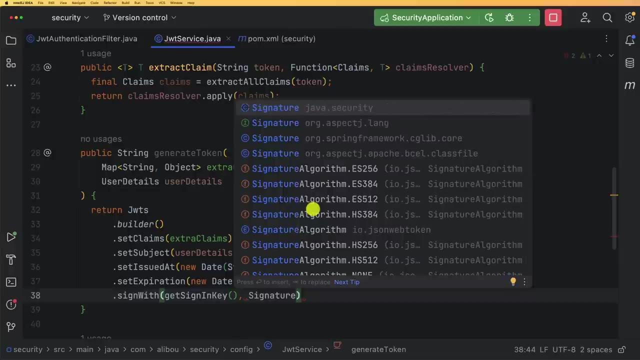 this token, and the signing key is the get signing key method that we already created before. And then we need to pass also the signature algorithm. So signature algorithm. And then we want to use the eight, the H S, two, five, six, Okay, 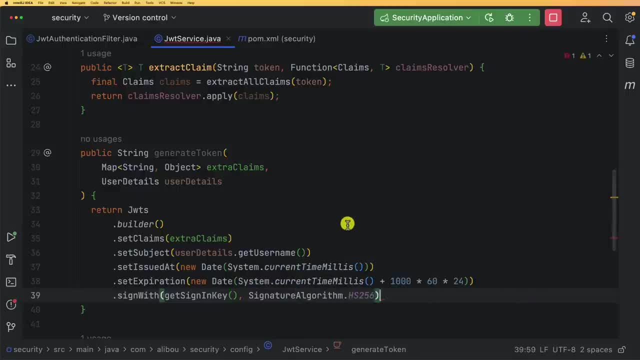 So it's this one, So let's select it and then finally call the method compact. compact is the one that will generate Okay And return the token. So, as you can see, this is how we can generate a token out of extra claims and the user details. 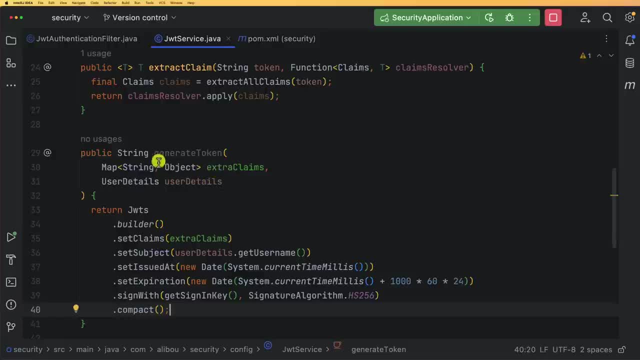 All right. So now this method will um, like we don't have a choice but passing claims and user details. But what if I want to pass, or I want to use um, or I want to generate a token without having? 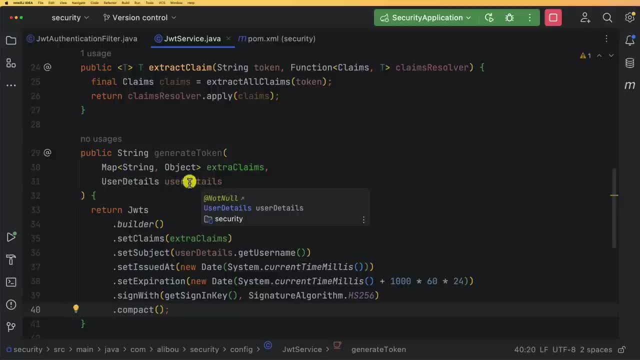 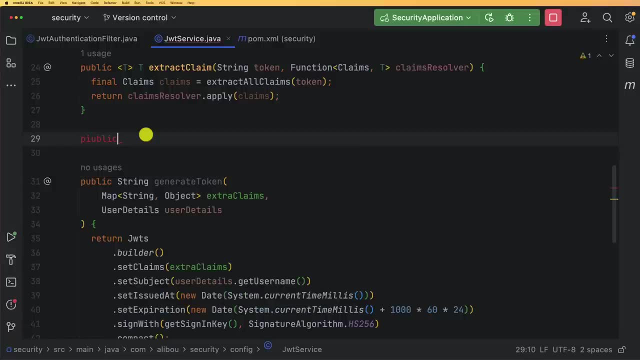 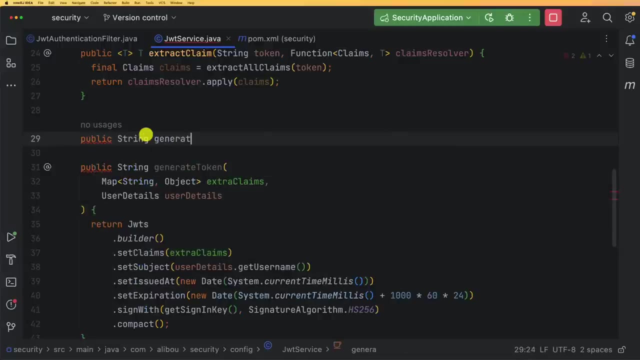 or without extra claims. I only, I only want to generate a token from the, from the user details itself. So it's easy peasy. I will create um another one public string, I will call. I'll give it the same name. 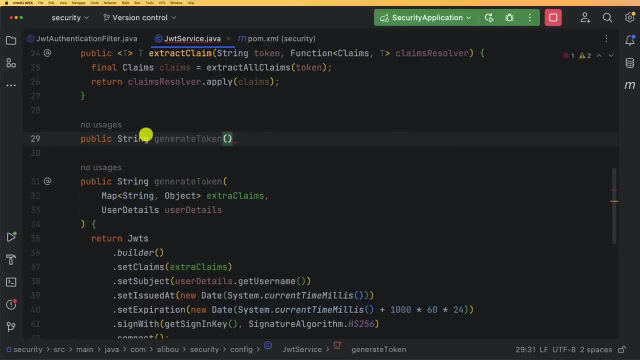 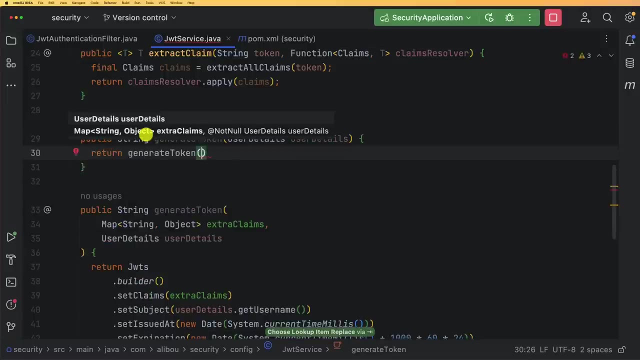 generate token and the generate token It will take it. I will pass only user details as a parameter And here I will just return: generate token out of um null, or let's say a new hash map like an empty one, and then user. 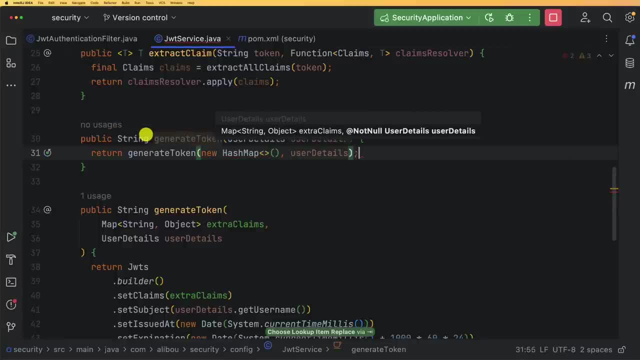 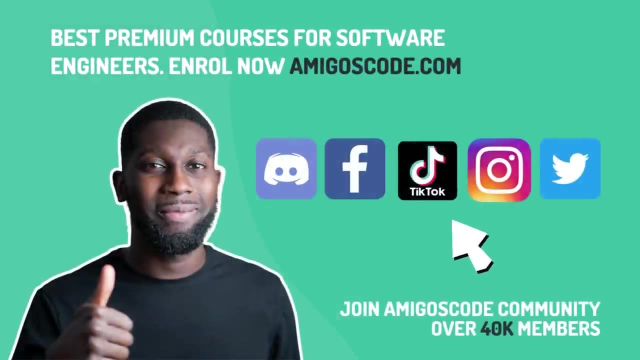 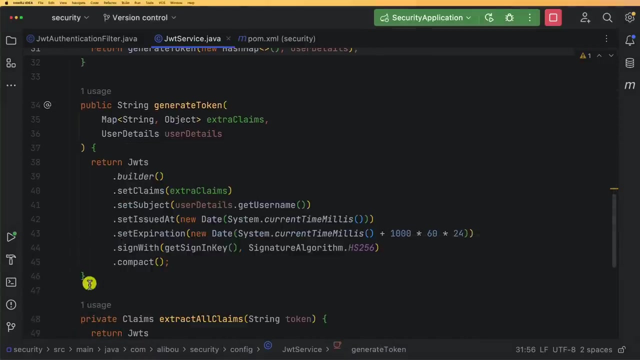 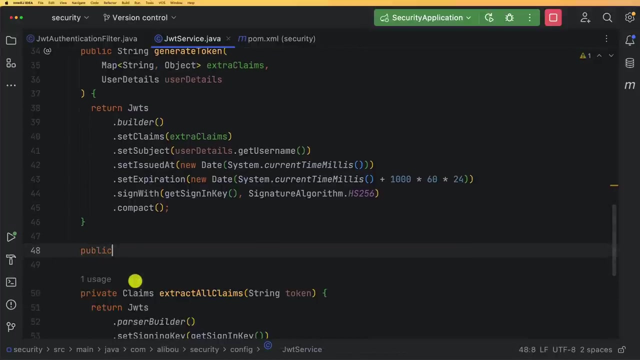 details. Okay, So now I have this generate token method that I can use later on. Okay, As a next step, let's implement a method that will will validate or can validate a token. Okay, So I will create a Boolean and I will call it is: 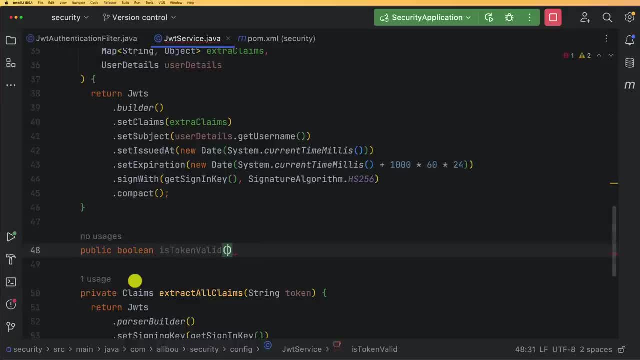 token valid, All right, And this token, this method, is token valid. We'll take two parameters as input, which is the token itself and the user details. Why we need the user details? because we want to validate if this token right here belongs to this user details right here. 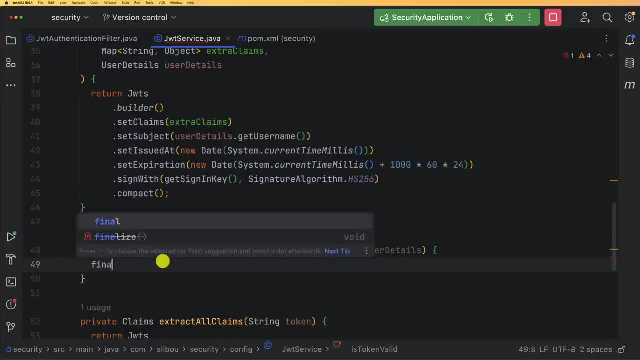 Okay, So first of all I need a final string: username or user email. but within this, within the context of this JWT service, let's stick to username and this one it will be. extract username out of the token. We already have the method for that. 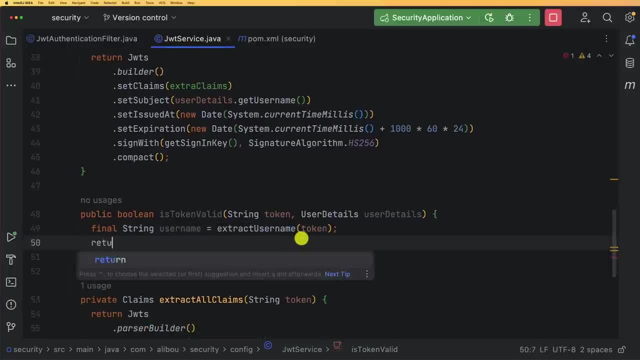 And then then what we want to do is to return if or whether the username that we have right here equals the user details. dot get username, All right. So we want to make sure that username we have within the token is the same as the username we have as input. 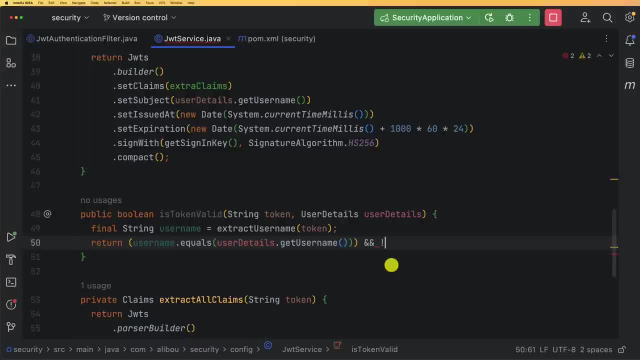 Okay And I want to make sure is is token expired? Like I would need to check that my token is not expired. Okay, And I want to pass my token As parameter. So this is token expired is a method that we need to create. 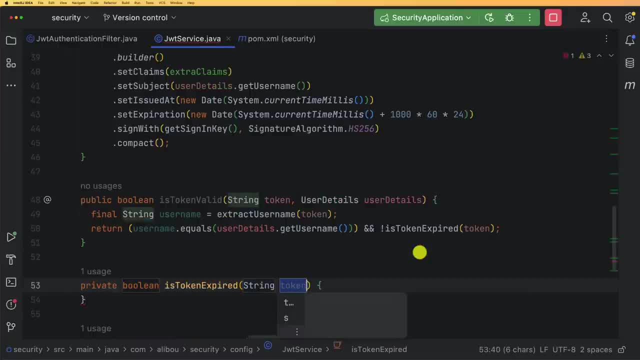 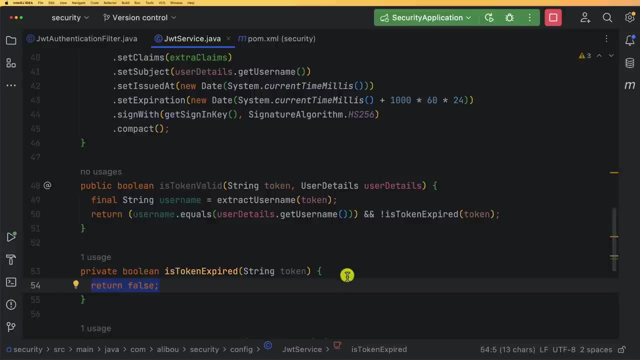 So let me go ahead and create this token expired and let's implement this token, Okay. So I want, for this is token expired. I want, I will create a method. I will call it extract expiration from the token that we have dot before, because it's a date. 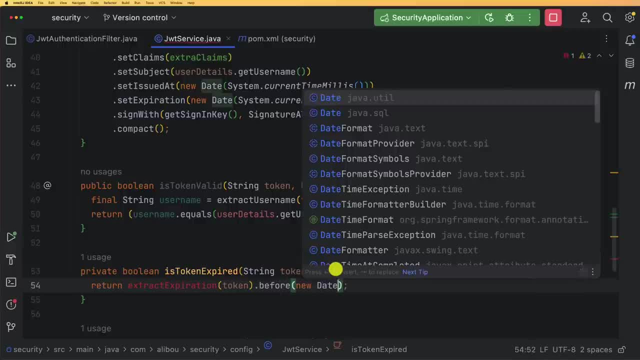 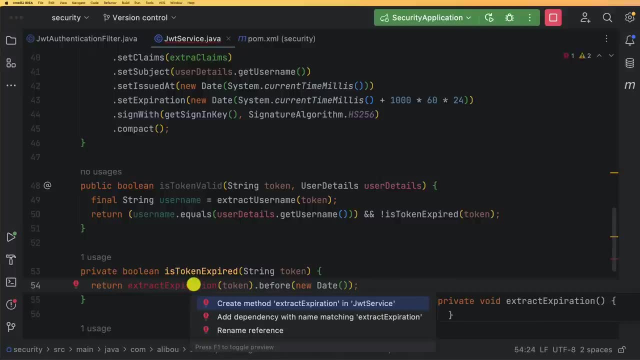 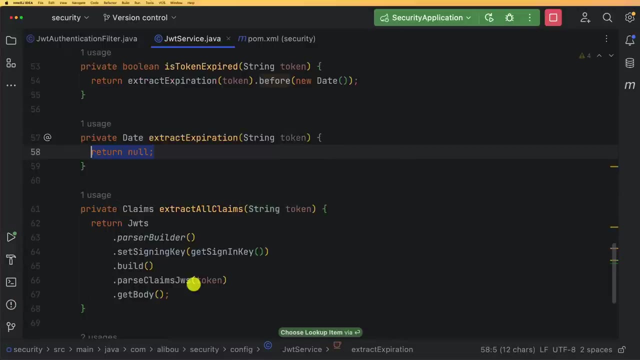 So it I want to make sure that it's before today's date. Okay, Before new date. Now let's create this extract expiration. So this extract expiration should return a date and it has, or it passes as a parameter, the token itself. 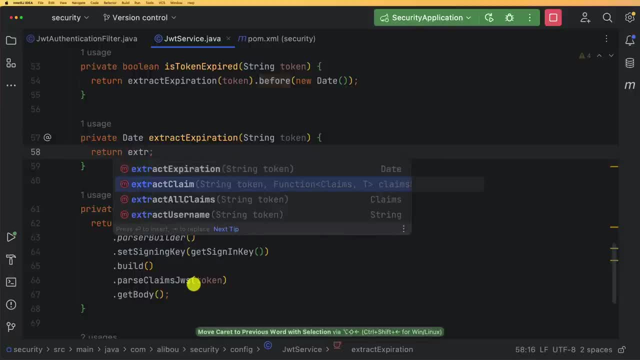 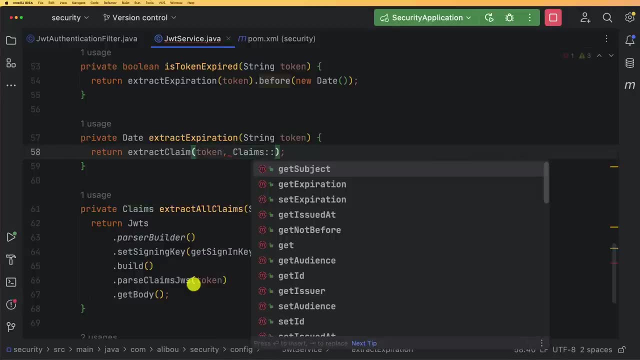 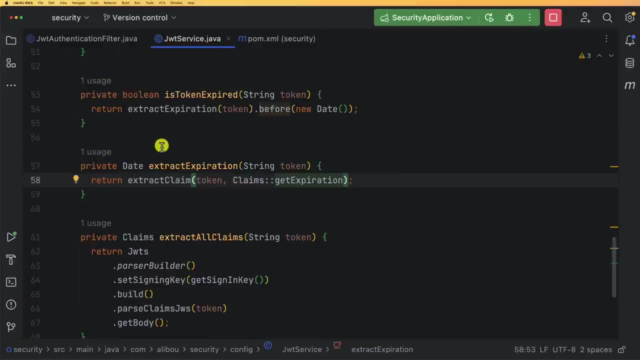 So it's also easy. So it's extract claim from the token And then it's claims dot, dot or colon, colon get expiration. Okay, So this is how we can extract the expiration date. All right, So how we have here if the is token expired. 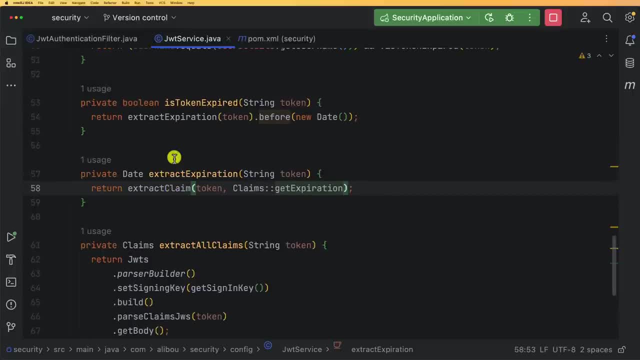 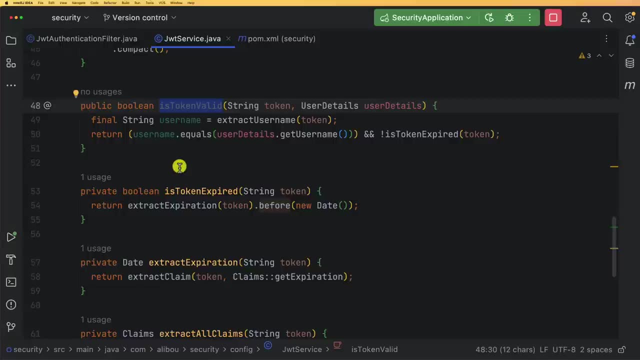 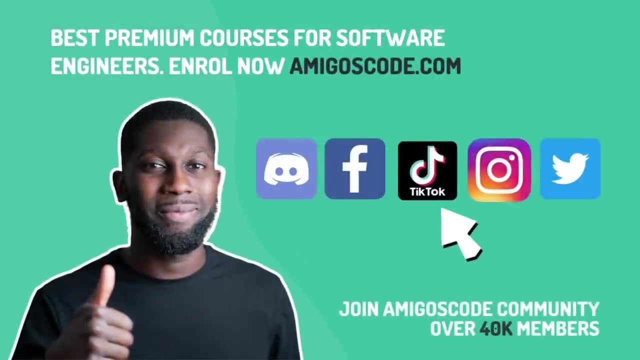 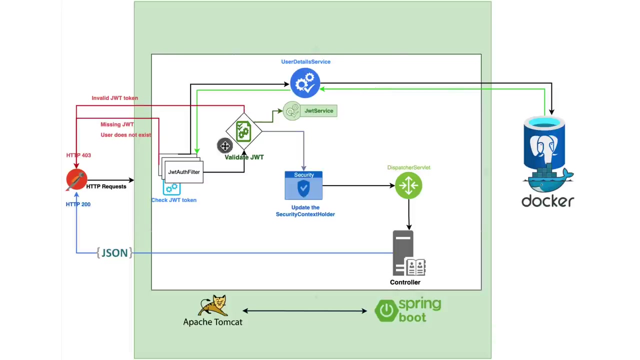 we have the is token valid. We have all the methods that we need, So is token valid. This one, we'll use it later on. So now let's move on and go back. finish implementing this Authentication filter. So here we just finished implementing this JWT validation process, or validation. 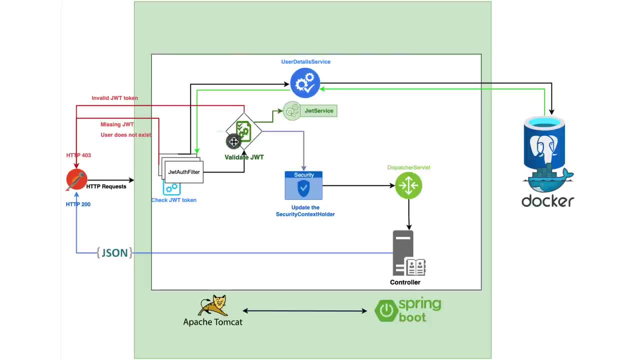 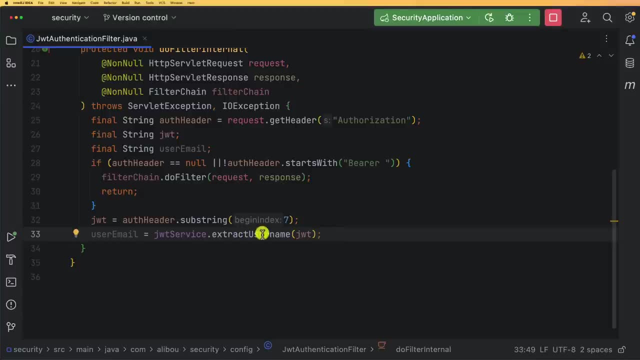 service right here And now we want to go back to this validate JWT process. So, within our code, what we did here, we extracted our user name. so we have now our user name valid. Let's go ahead and perform or finish our validation process. 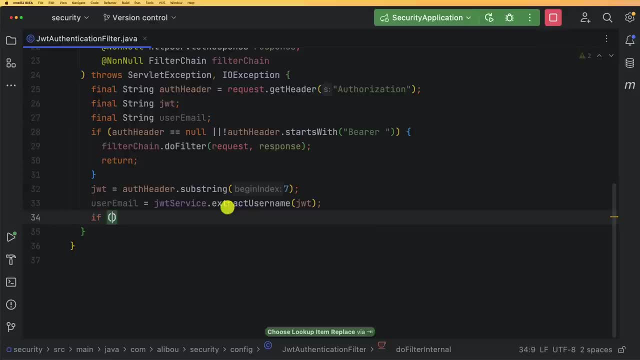 All right. So here I want to check if my user email is not null. So I have a user email or I can extract my user email out of my JWT token. and I want to check something else. I want to check that the user is not authenticated yet, because if the user is not authenticated, 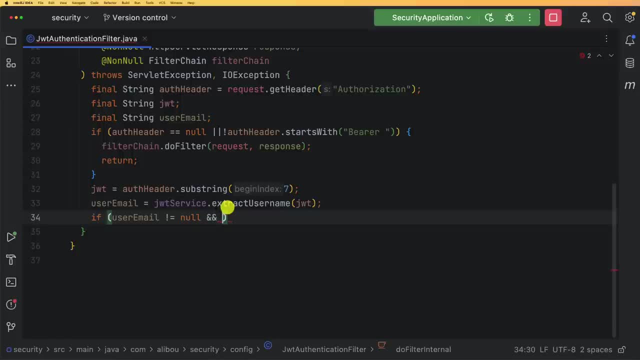 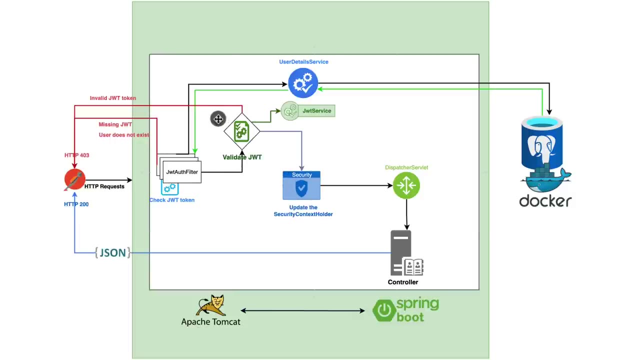 I don't need to perform again all the checks and setting or and updating the security context and so on and so forth. So here I want to check if the user is already authenticated. I don't need to do all this process and so on and so forth. 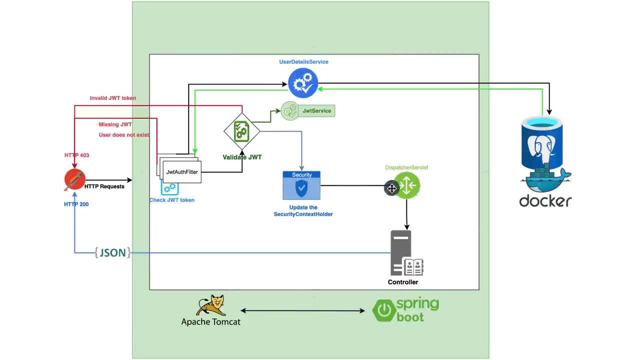 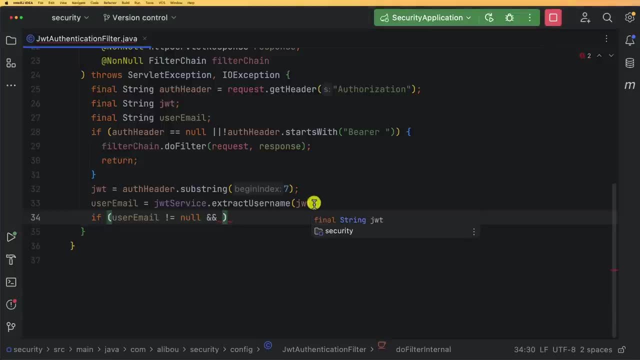 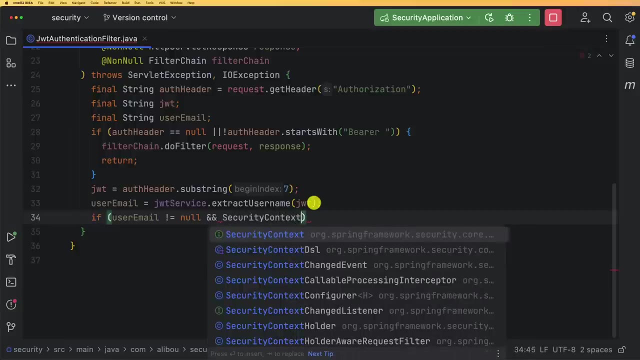 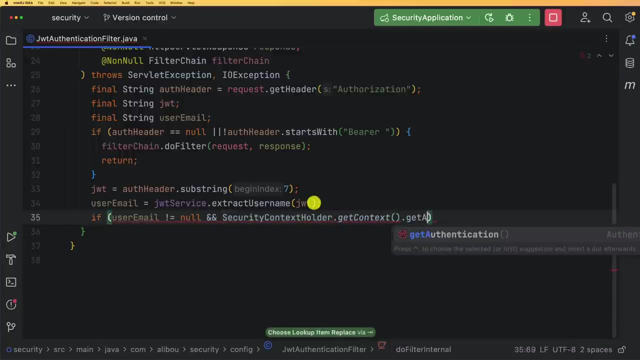 All I need to do is pass here and leave it to the dispatcher servlet, Okay. So to do that, or to check if the user is already connected or is already authenticated or not, we have an object called security context holder and from that we can get the context, and then we have a method called get authentication, and when the authentication is null means that the user is not yet authenticated. 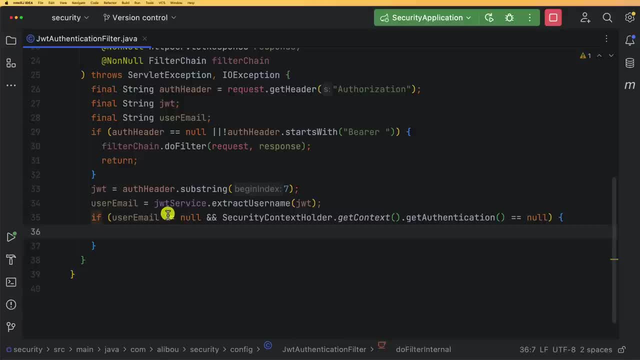 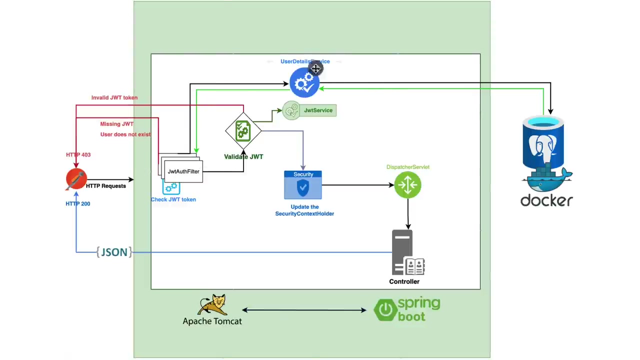 Okay, So this means that the user is not connected yet. All right, So once the user is not connected, what We need To do here, like when we go back to follow this process, we need to perform and to check or get the user from the database. 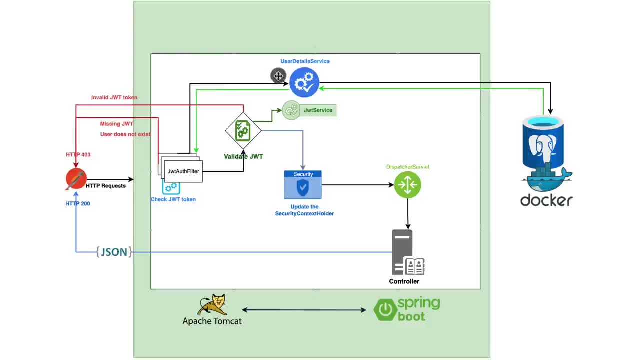 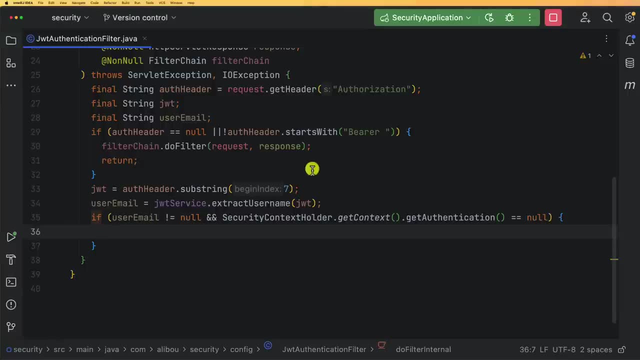 All right. So once we do this validation process, we want also, or we need, to check if we have the user within the database. All right, So to do so, I will create an object called user details, or you can just call it user, because our user already extends or implements. 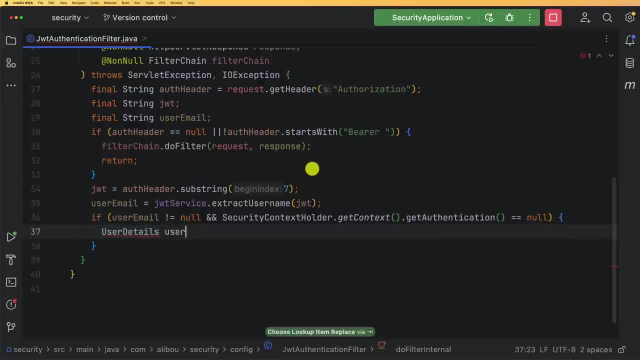 The user details interface, and we call it user details equals, and here I will use this dot user details service, which we don't have yet. And here we have a method load by user username. Okay, And the you and my username in this case is the user email. 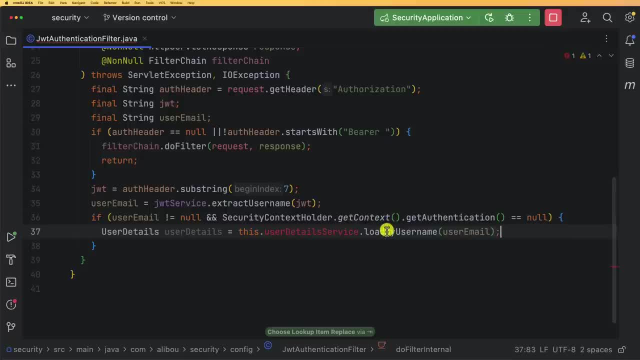 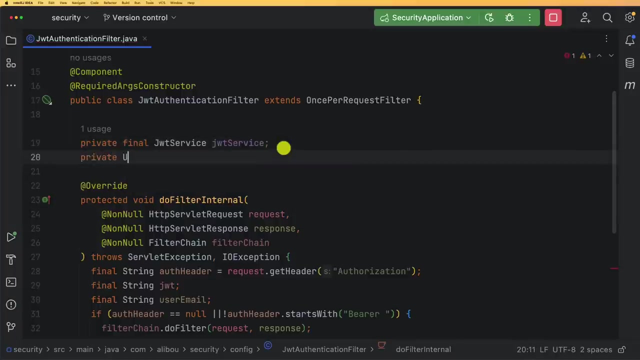 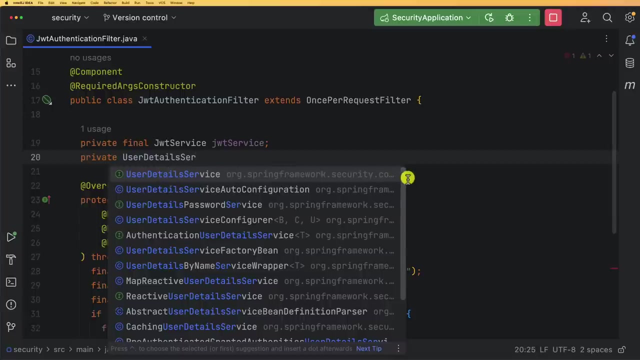 All right. So here the method called Load user by username, and in this case we don't have this user details service, but let's create one here. So this user details service is already an interface within the spring, available within the spring framework, and it's from spring framework security core and so on, so forth, and I will call it user details service. 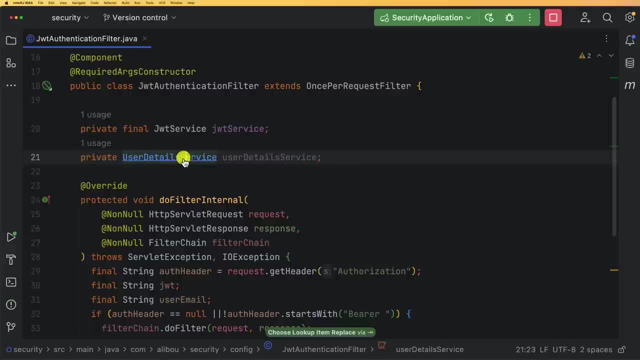 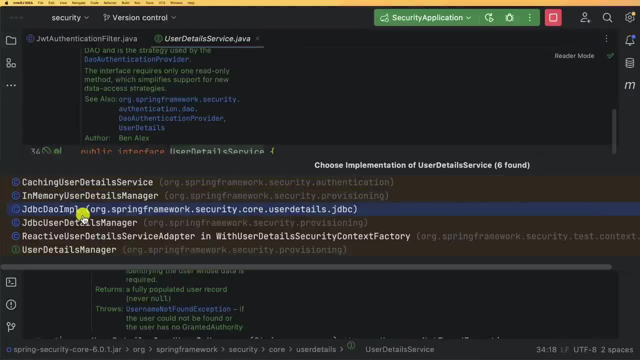 So this user details service is already an interface within the spring framework and it's from spring framework, security core and so on, so forth, and I will call it user details service. So this interface, if we check it right here, So here we have some implementation for it. 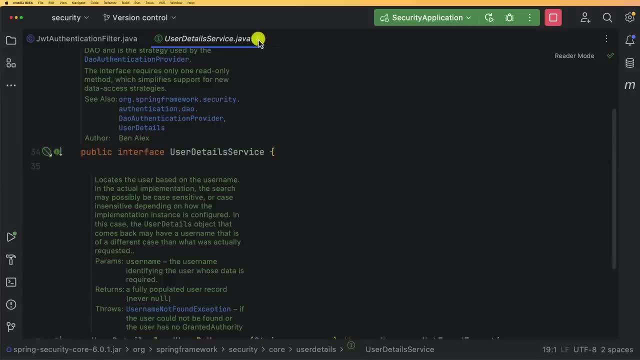 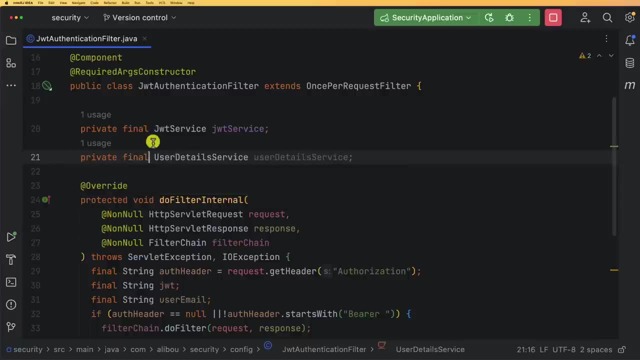 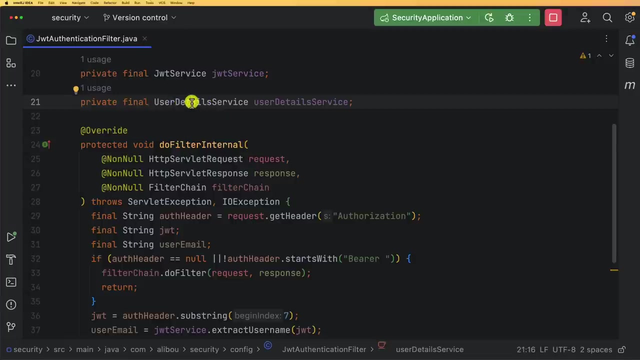 Okay, But we want our own implementation because we want to fetch our user from our database. All right, So make this one final, Don't forget this, And let's move on and implement or provide a bin of type user details service. So that's a bin of type user details service. 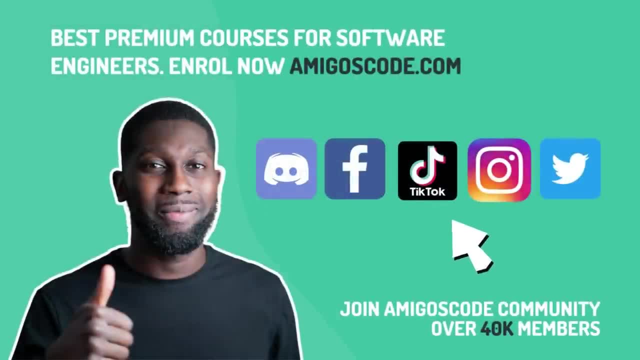 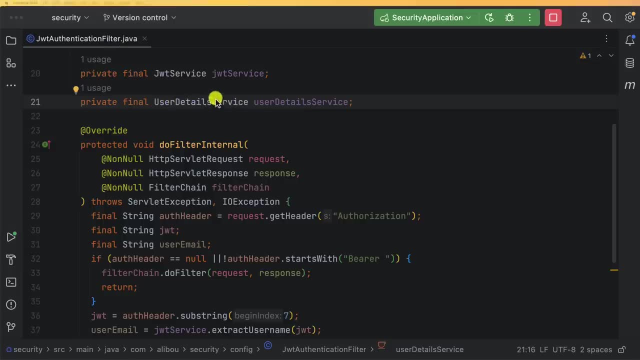 So let's go ahead and create a bin of type user details service At this level, we need to create a bin of type user details service, or we need to create a class that implements this interface So and also give it the service or component annotation, so it becomes a managed bin and spring will be able to inject it. 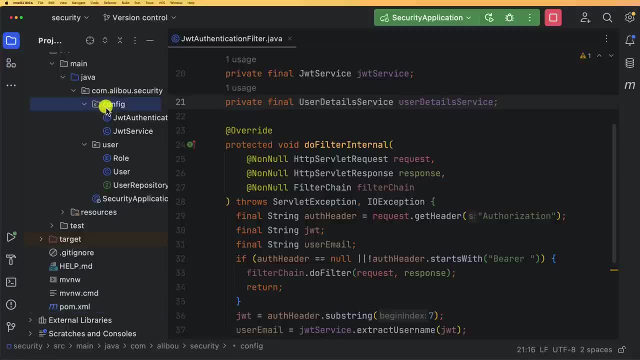 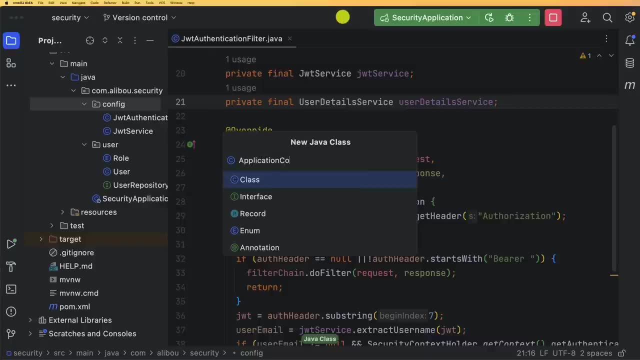 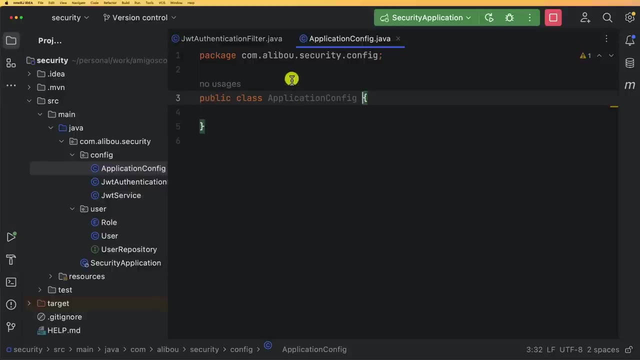 But let's do it in a fancy way. Within This config package, I will create a class. I will call it application config. So this application config will hold all the application configurations, such as bins and so on, so forth. All right, So to make this class a configuration, we need to annotate it with the annotation called configuration. 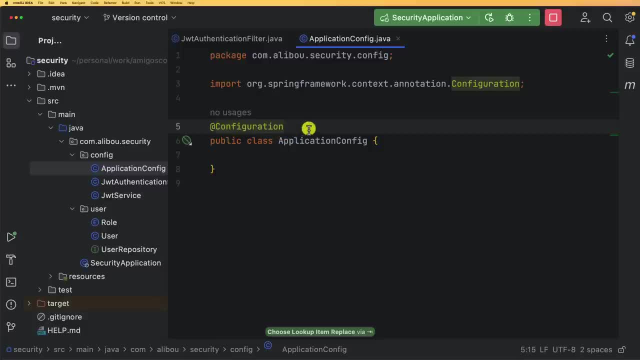 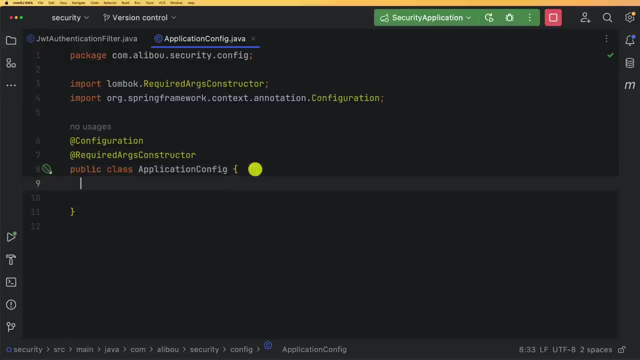 So at the startup, spring will pick up this class and try to implement and inject all the bins that we will declare Within this application config. All right, We also need the required Rx constructor in case we want to inject something. So what we need to do now is to implement or to create a bin of type user details service and to do so. 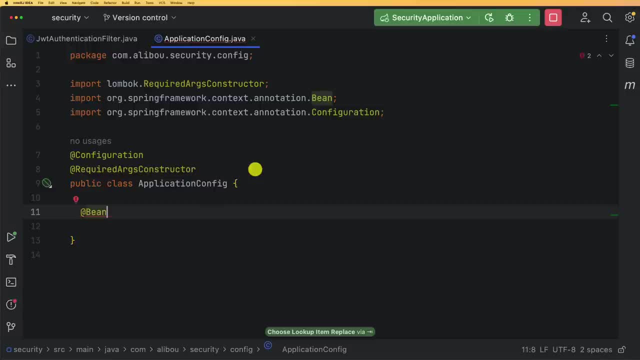 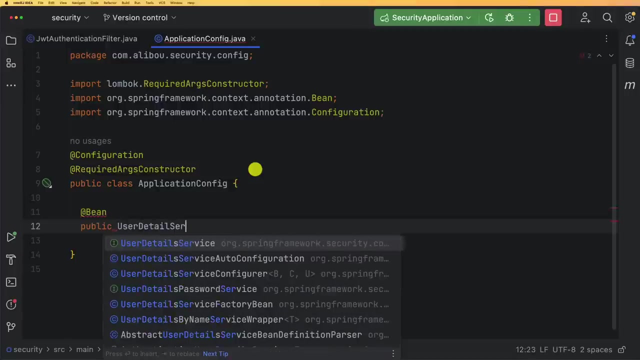 First of all, we need to use the annotation bin, this to indicate, to spring that this method represents a bin, and a bin always should be public, No private bins, And our bin is of type user details service. Okay, So let's call it user details service. as easy as that or as simple as that. 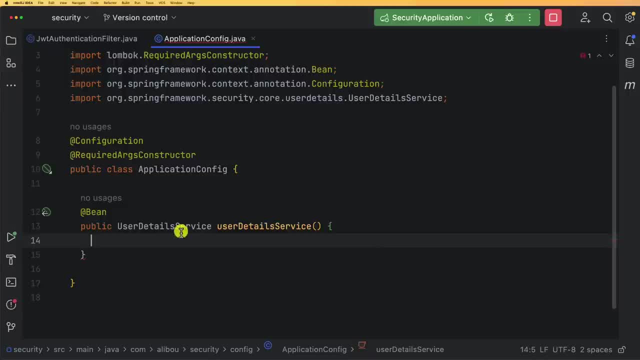 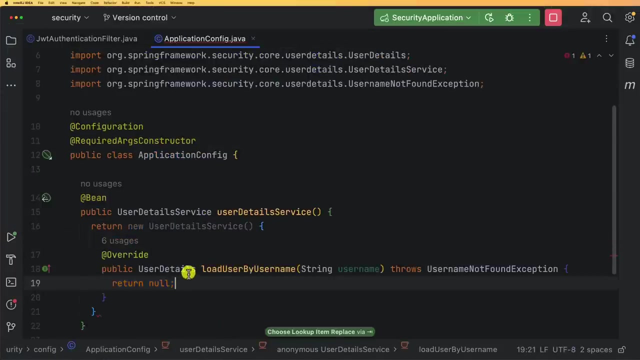 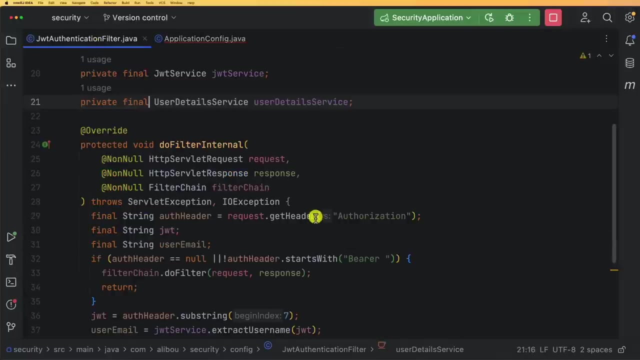 And then we can use a lambda expression so we can use or we can say return a new user details service and we implement the load user by user name. So we can do like that: New user User details service, like this, and automatically you will see here that we have this load user by username method, the one that we want to use in here. 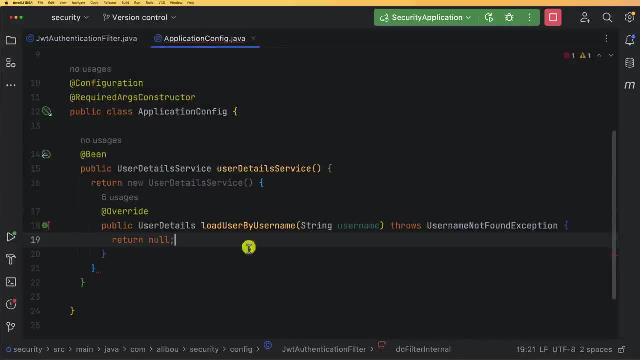 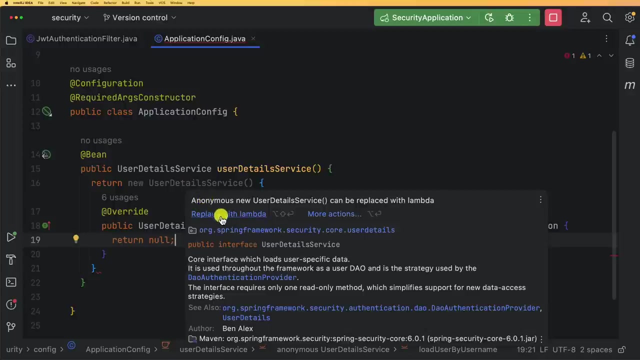 This method right here, Okay, But? but we can make it more simple than that and we can use a lambda expression and the lambda expression It's. it looks like that. So here we already see that, until AJ is proposing to replace this with a lambda. 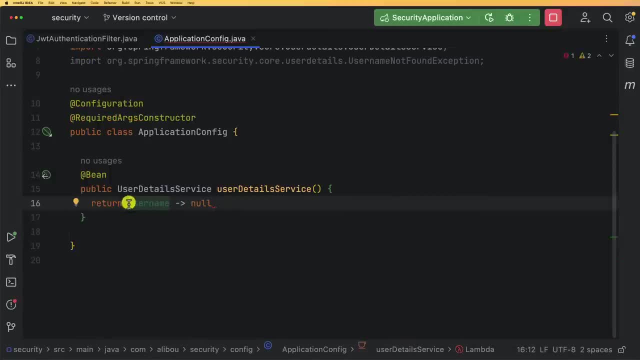 So we'll just go ahead and click on it. So the lambda is the user name. So we provide the user name, the one we have as an input within this method right here, And then we need to provide the implementation. Okay, So in this case, what we want to do is to fetch. 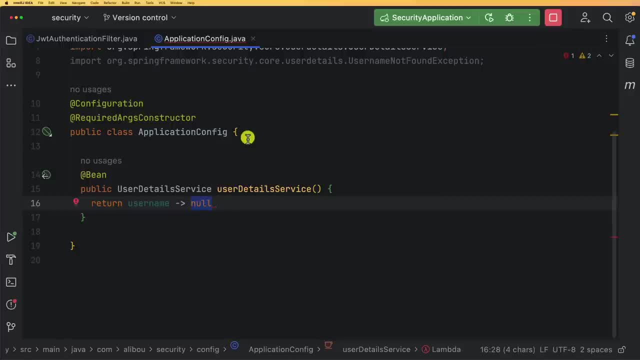 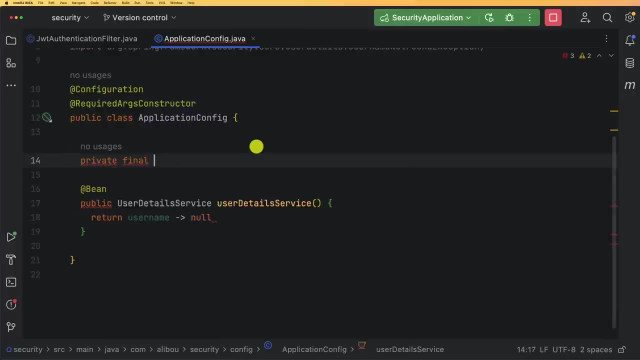 The user or to get the user from the database, and to do that we need to inject our user repository. Okay, So let's create a private final user repository. Let's call it repository or user repository, And here, simply what we need to return is user repository. 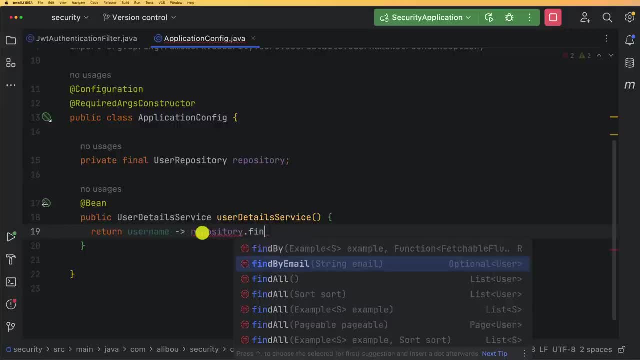 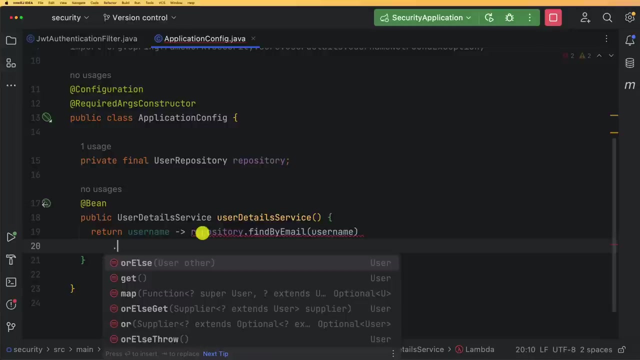 Dot, find by email, the method that we created When we just created the user repository, and find by email. We need to pass the user name. Okay, and since the find by email returns an optional of user, here I want to add an, or else throw so, in case we don't have or we don't find the user name or the user within our database. 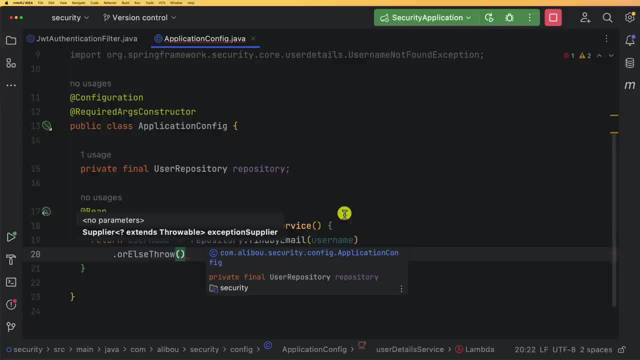 We need to return an exception of type whether entity not found exception, or we can also return The exception user name: not found exception. Okay, so I will use the user name not found exception and I will just provide here. It should be also a lambda. 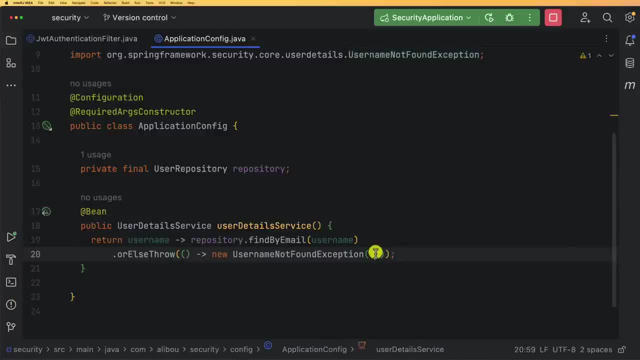 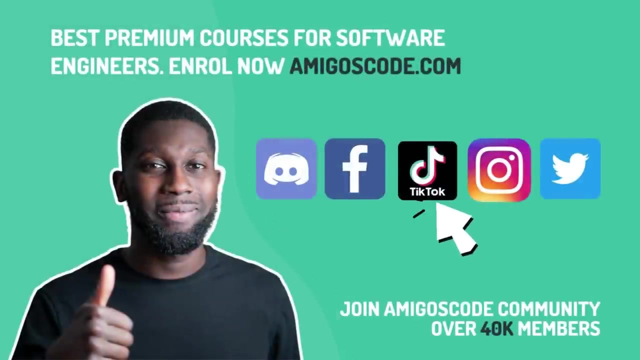 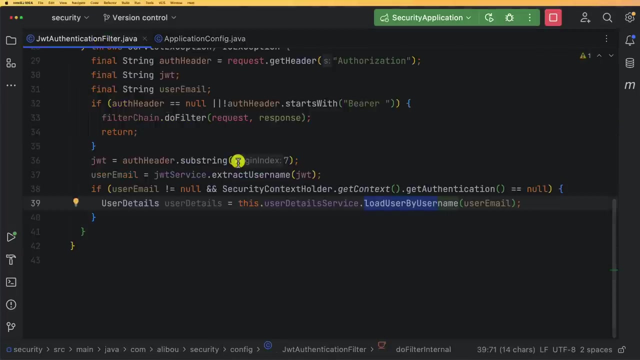 And, for example, as a message we can say: user not found, All right. So here now we have our user details service, So now it's ready to use. Let's continue implementing our JWT authentication Filter. Now we can go back to our filter and finish the implementation. 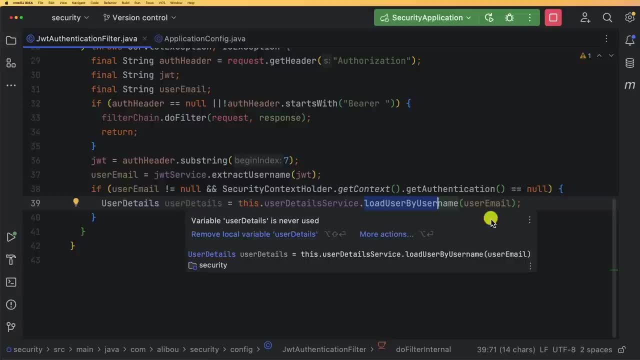 All right. So here we have our user details, or we have our user, and the next step is to validate and check if the token is still valid or not. So here I will add: if JWT service Dot is token valid, Okay. and here I need to pass my JWT and the user details that I just got from the database. 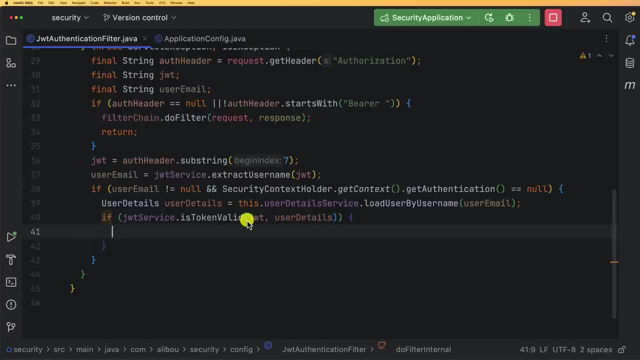 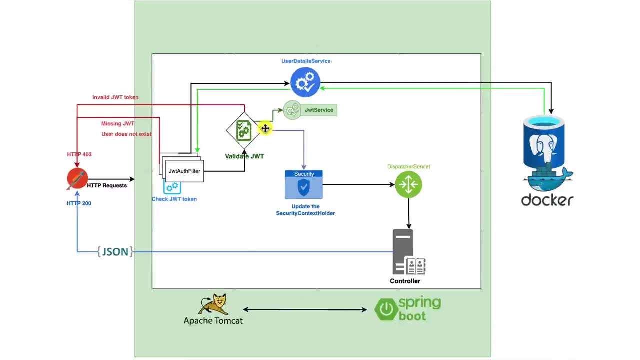 All right. So if the token is valid, then what I need to do, I need, like we have in here we need, if the user is valid, We need to update the security context and send the request to our dispatcher servlet. Okay, Okay, All right. 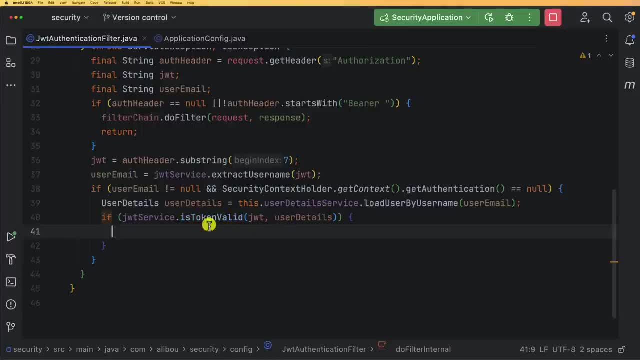 So, once our token is valid, I need to create an object of type username password authentication token, So username password authentication token, I will call it auth token- and this object is needed by by spring and by the security context holder in order to update our security context. 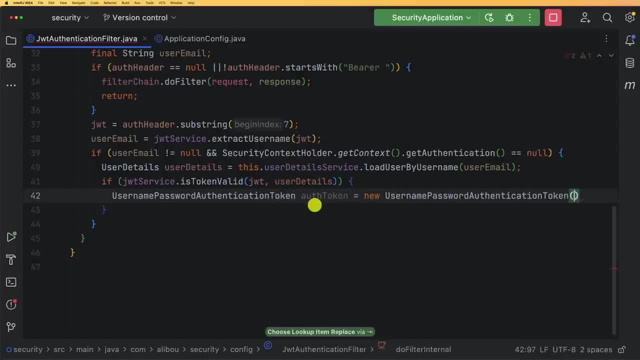 Okay, so equals The new username and password Authentication token and it takes as parameter the user details. and then for the next parameter, for the authorities, I want to pass it as null and then the user details, dot get authorities. So here, because we are, we don't have credentials, as you remember when we created the user. 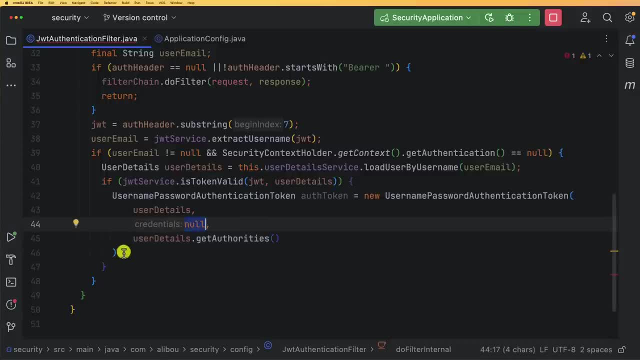 We don't have credentials, So that's why I'm passing these credentials as a null value. So once I finish creating or finish instantiating this user name authentication token, I want also to give it some more details, So I will use the auth token dot set details and these details it takes an object. 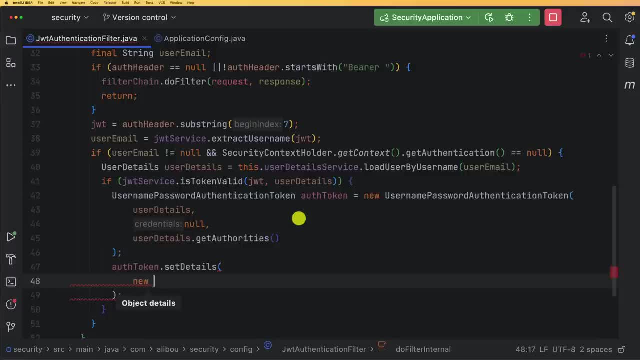 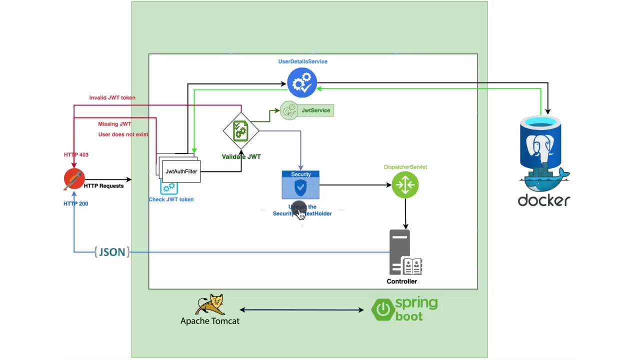 So I will pass a new object of type new web authentication details source, Authentication details source, and here I want to build the details out of our request, out of our HTTP request. All right, Now the final step is, as we mentioned here, The final step is to update the security context holder. 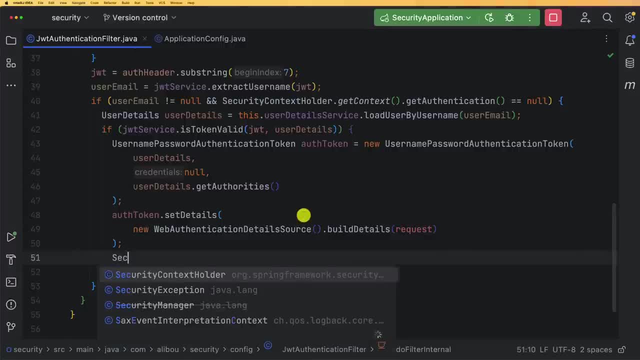 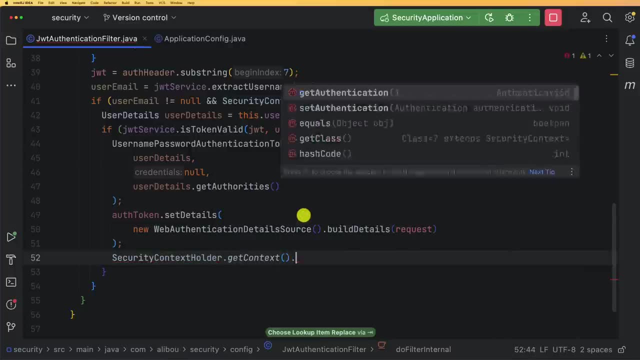 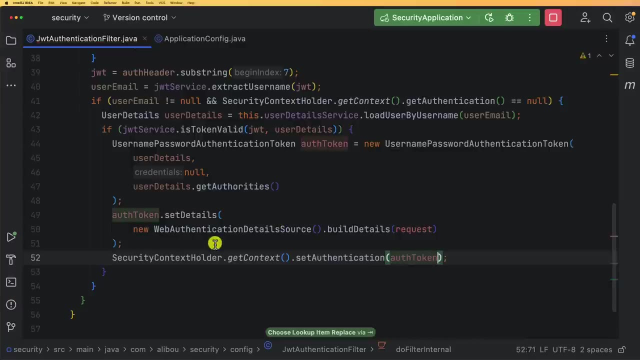 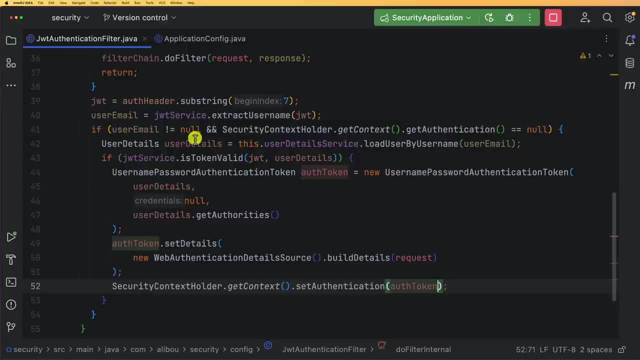 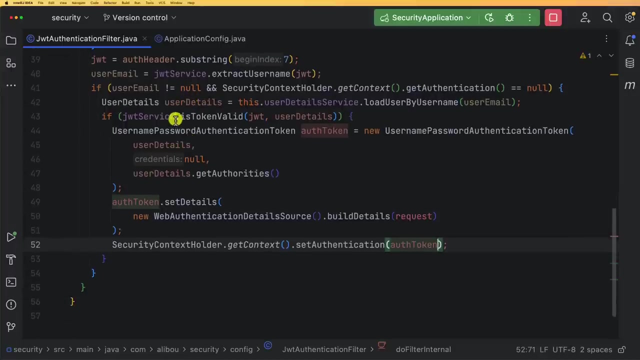 So to update the security context holder. So to update the security context holder: dot get context, dot set authentication with our authentication token. All right, And that's it. Now let's recap this one. So here, when, if we have our user email and the user is not authenticated, we get the user details from the database and then what we need to do 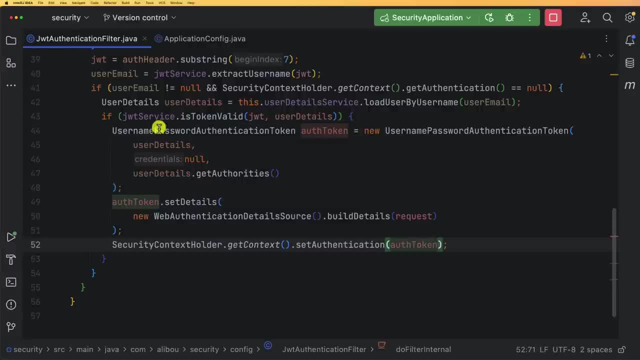 We check if the user is validated Or not. If the user and the token is valid, So we create an object of type user name, password authentication token. We pass user details, credentials and the authorities as parameter, And then we extend or enforce this authentication token with the details of our request. 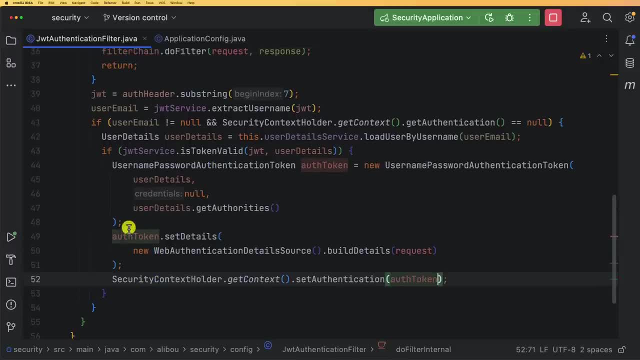 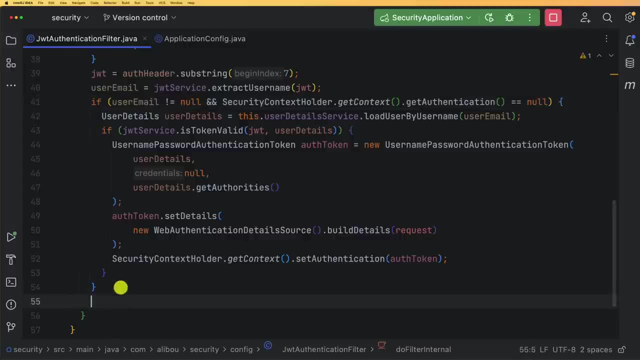 And then we update the authentication token. And don't forget, as a last step, and always do think about after This, if Think about always calling our filter chain, dot do filter, So we need always to pass the hand to the next filters to be executed. 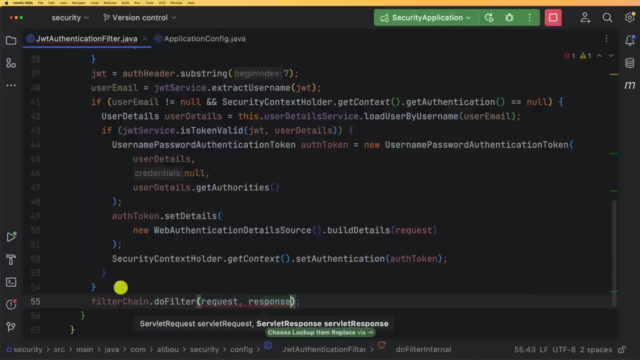 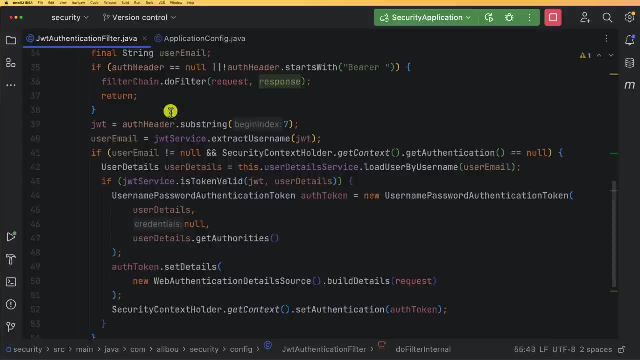 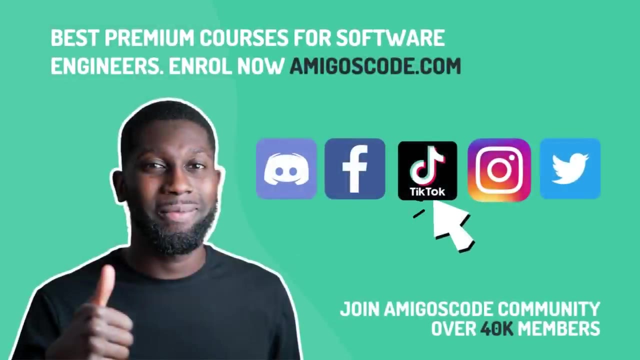 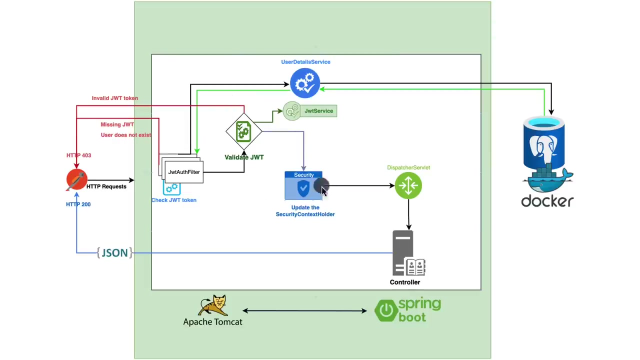 OK, And here we need the request and the response. And that's it about our JWT authentication filter. It is ready to use. Let's move on and see what we need to implement next. This whole process is now implemented, but we still need to do some extra steps. 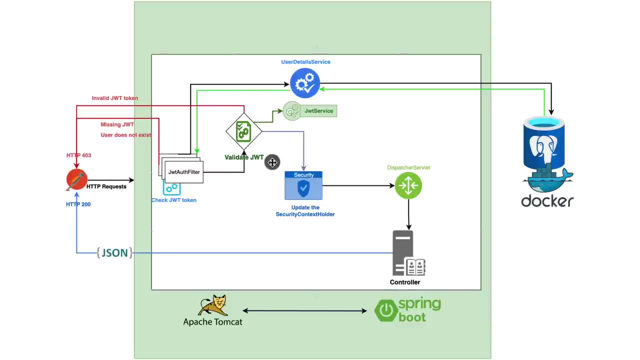 The extra step we need to do is to tell spring which configuration that we want to use in order to make all this works. OK, So we create the filter, We implemented the user details, service validation, updating context, And so And so forth. 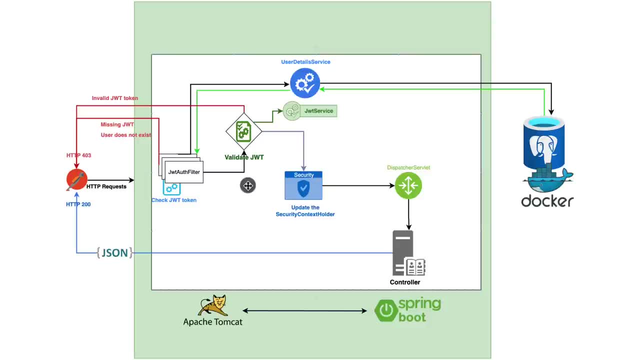 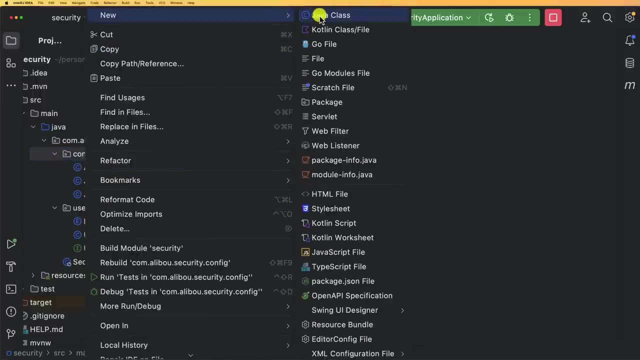 But what we are missing is the binding. We need to bind because we created a filter, but this filter is not yet used, So we need to use it, And in order to do that, we need to create a new configuration class. I will call it security configuration. 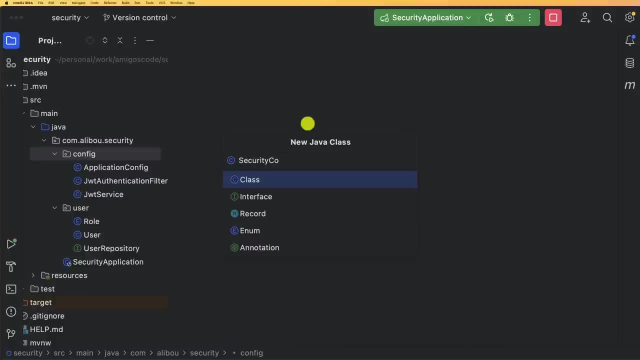 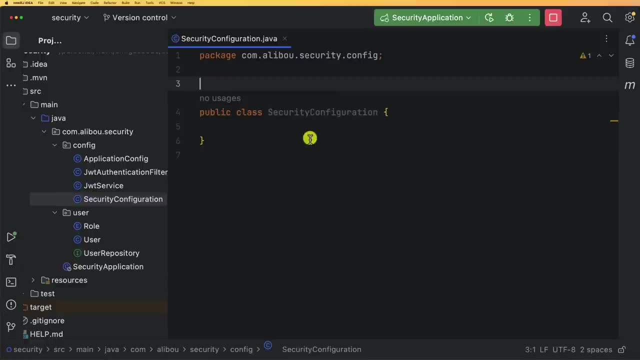 OK, So I will call this class security, config or configuration, And this is going to be our security configuration And this is going to be our configuration class. And, as always, to make a configuration class become a configuration, We need to add this configuration annotation from spring. 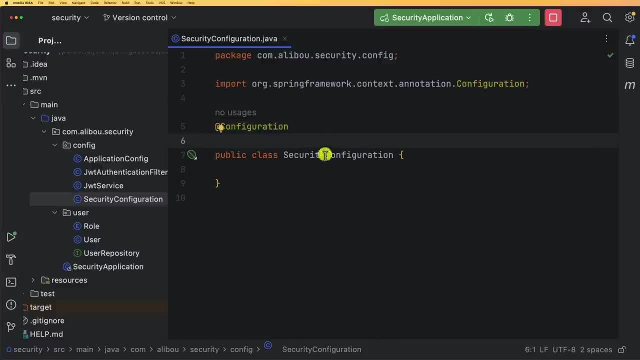 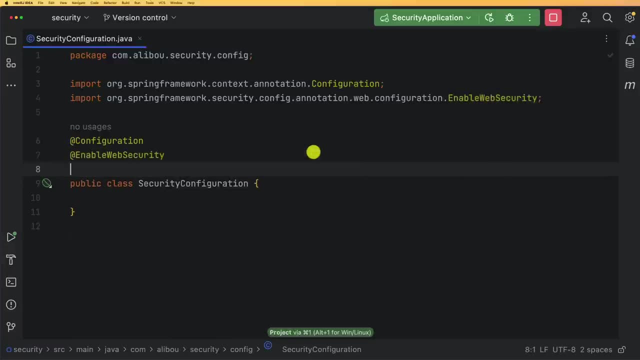 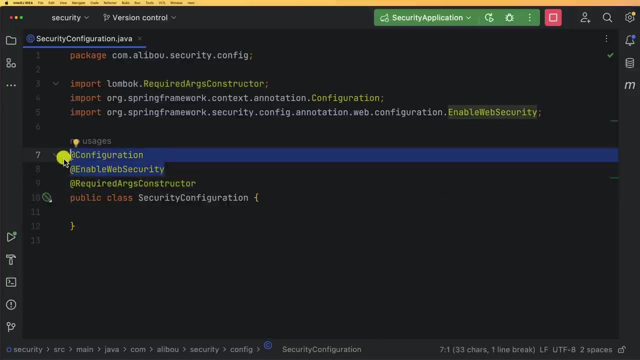 Also, because we talk about security right here, We need to enable web security- Let me make it full screen- And again, we will need the required args constructor. So these two annotations they need to, they need to be together When we, when we work with spring boot 3.0. 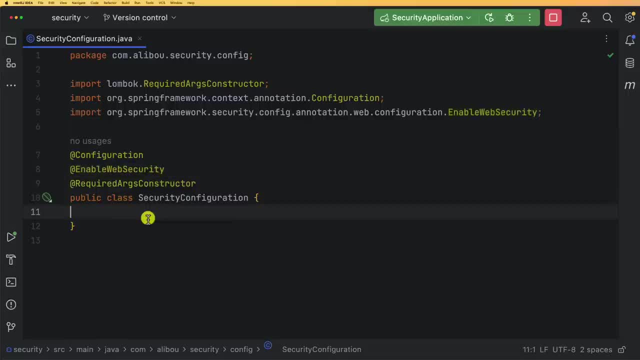 OK, So next, what I, what I will need to do, because, as at the startup or at the application startup, spring security will try to look for for being of type security filter chain, And this security filter chain is the bean responsible of configuring all the HTTP security of our application. 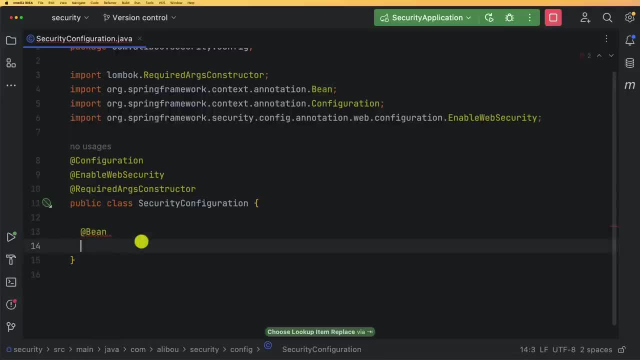 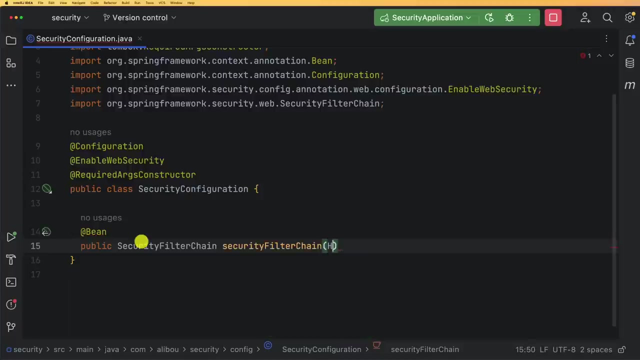 So I will create A bean- Public security filter chain, I will call it security filter chain. And within this method, of this bean, I will pass a parameter of type HTTP security. I will call it just HTTP, just for a short variable name. 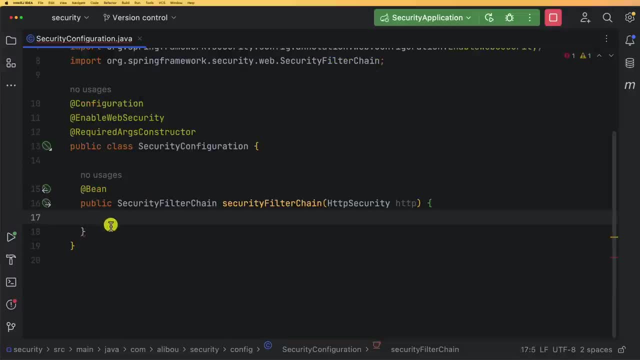 OK, Now let's start configuring our HTTP security. So here, as you can see, it's type, it's of type security filter chain, And to do that let's first return HTTP dot build, And here we need to add also the exception to the method signature, because this build might throw an exception. 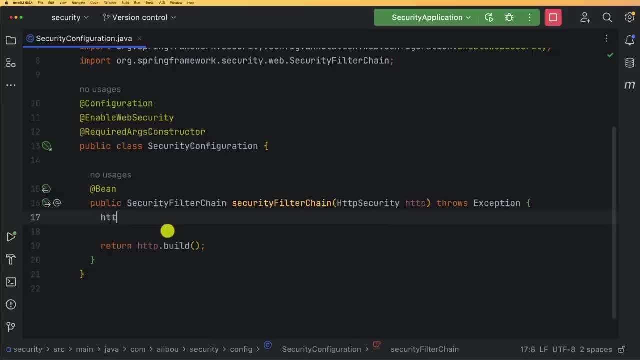 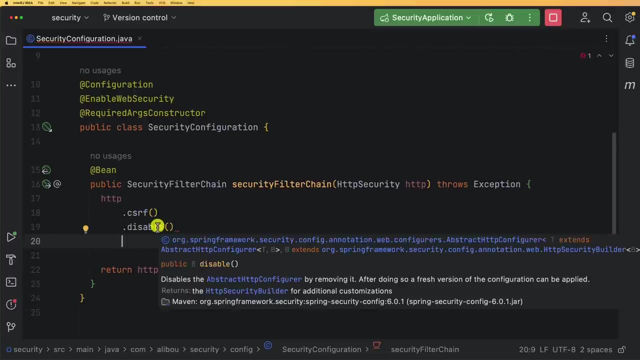 All right, So now to do the configuration. I will start by HTTP dot. I will first disable the CSRF Verification, and we made, we made we might talk about this in the different, in a different video. So here now, once we disable this one. and now let's move on, or we will implement the configuration, the real configuration. 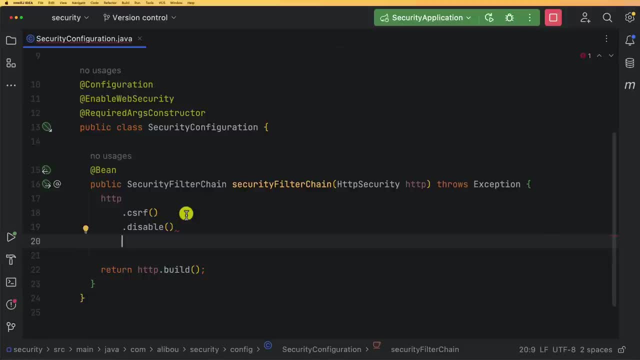 So, within the security, we can choose and decide what are the URLs And the path is that we want to secure. but of course, within every application we have always a white list. white list means that we have some endpoints that they do not require any authentication or any tokens, that which are open, for example. 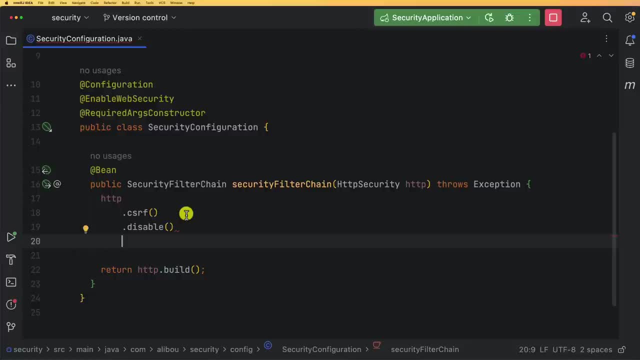 When we talk about creating an account and logging. So in this case, to create an account, we don't need a JWT token, Because at that time we will create a user account and we will require or will ask for a token after that. Also, the same when we want to log in: we don't need to pass the token as parameter because we don't have one yet. 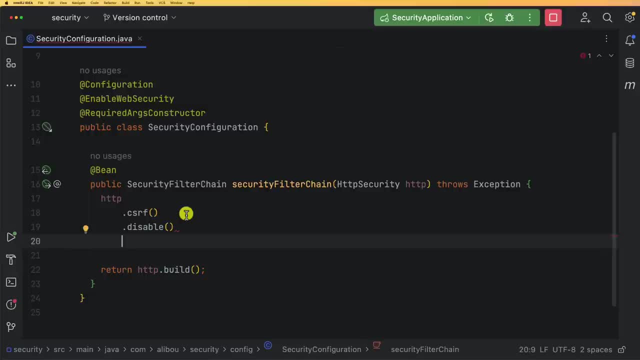 So in this case, this is when we talk about white listing, And here is how we can implement white listing. So, after disabling the CSRF, I want to authorize HTTP requests And after authorizing, after using or calling: this authorizes CP request. 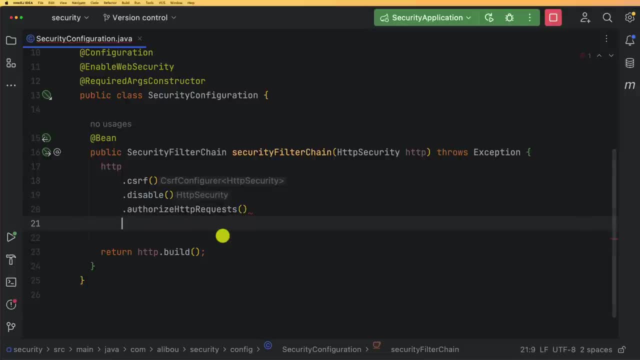 Here we can call a request matcher, Request matchers And for this request matchers we can pass a list of strings and a list of patterns. This will represent the application or our application patterns. We will go back to this later on And for this list I want to permit all. 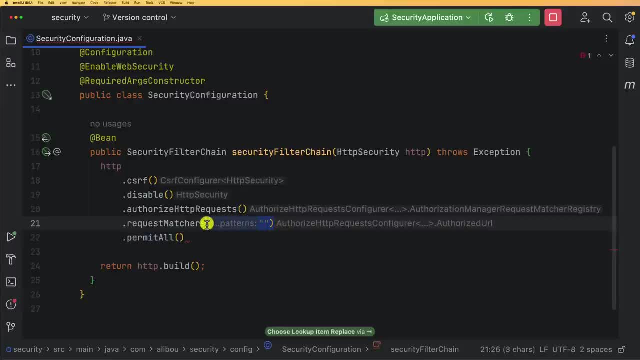 I want all the requests in here, All this list. I want to permit all And then any requests. All the other requests, I want them to be authenticated. So this means I want to white list this list and authorize all the requests within this list. 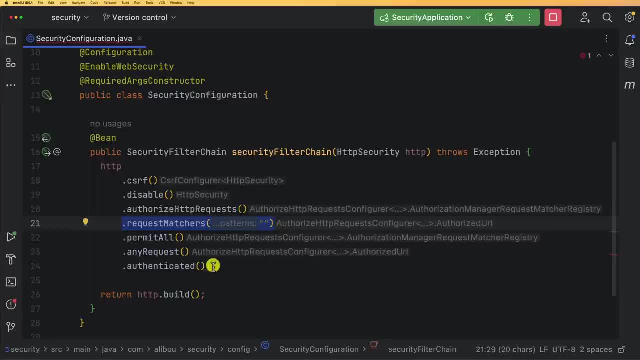 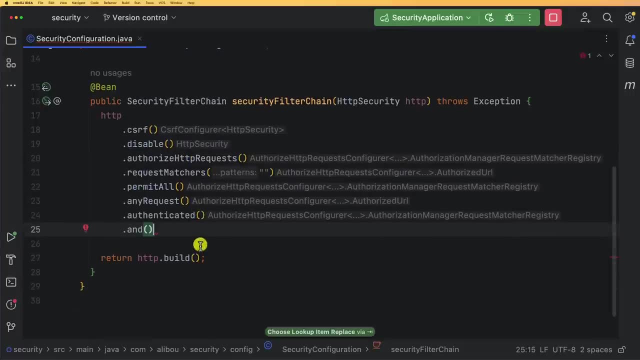 But any other request should be authenticated. Ok, Now Let's talk about and let's see how we can configure our session management. The session management means what We said, that when we implemented the filter, We want a once per request filter. 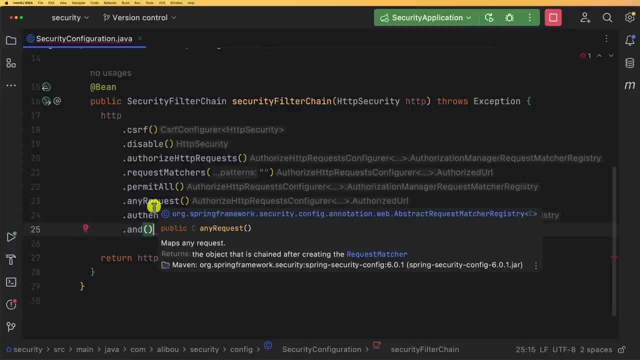 Means. every request should be authenticated. This means that we should not store the authentication state, Or the session state should not be stored, So the session should be stateless, And this will help us ensure that each request should be authenticated. Ok, So now we use the and to add a new configuration. 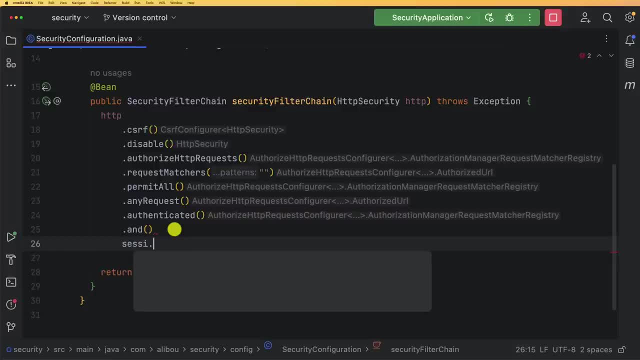 And here let's add Session management. And here I want to talk about the session creation policy, How we want to create our session. So, as I mentioned our session, We want it to be stateless session. Ok, So I will use session creation policy dot stateless. 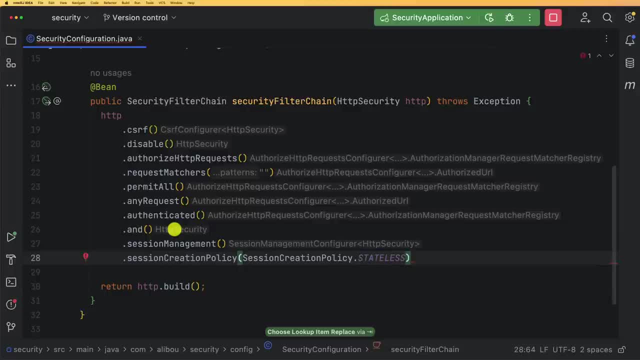 And, like this, spring will create a new session for each request And then- and Here I need to tell spring which authentication provider that I want to use, The authentication provider. I will explain it in just a few seconds. Ok, So I will just add it. 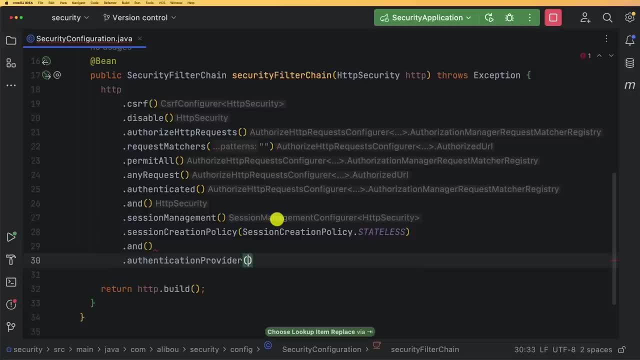 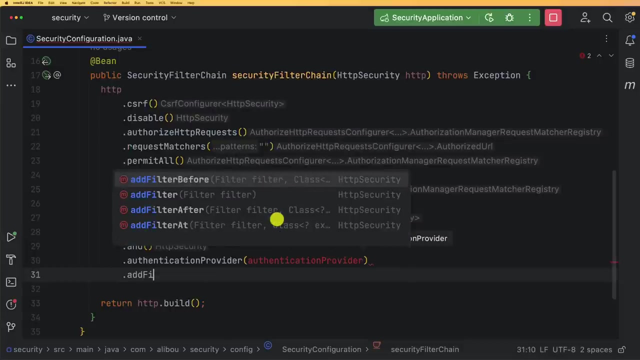 Authentication provider And I will create an object of type authentication provider And then I will go back and create it later on. And then, after the authentication provider, I want now to use the JWT filter that we just created. Ok, So to do that, I will use the method add filter before. 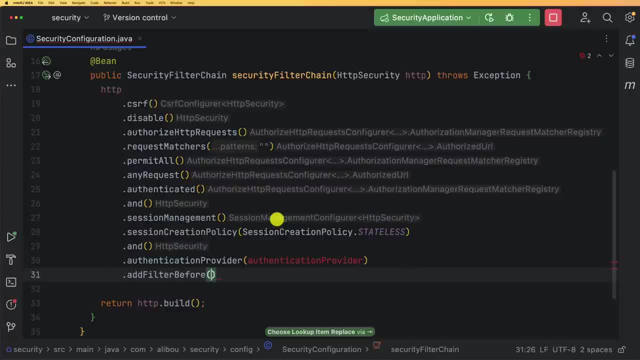 Because I want to execute this filter before the filter called username password authentication filter. Because, as you remember, when we implemented the JWT authentication filter, We check everything and then we set the security context, We update the security context holder And after that we will be calling the username password authentication filter. 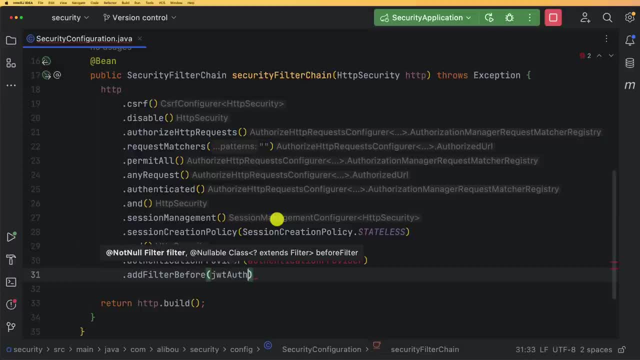 Ok, So here I will use JWT auth filter. I will call it like that And I want it before the username: password: authentication filter dot class. Ok, Now let me create this object. So I will use the not local variable But create a field. 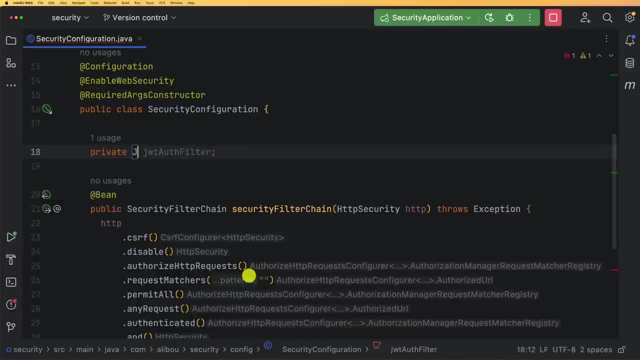 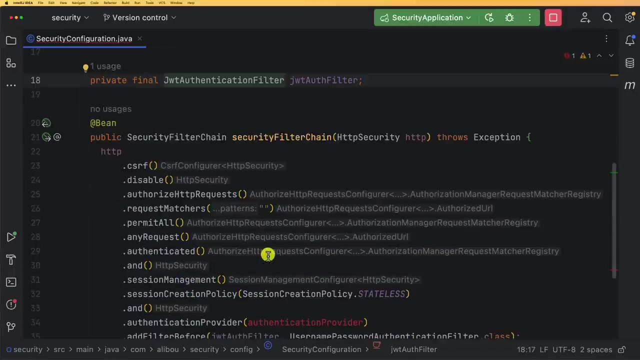 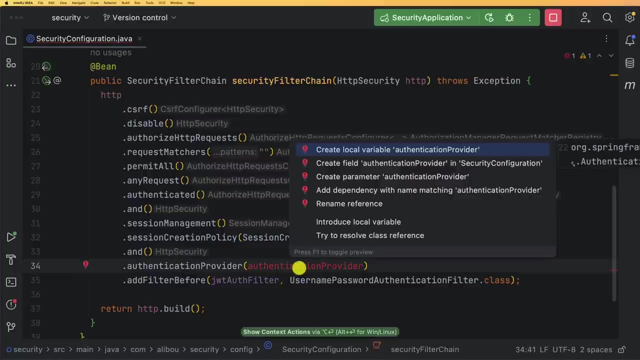 And this one. I want it to be of type JWT authentication filter. Ok, So this is the first one And I need it to be final, So it will be automatically injected by spring, And the next one is the authentication provider. So let's create a field of type authentication provider. 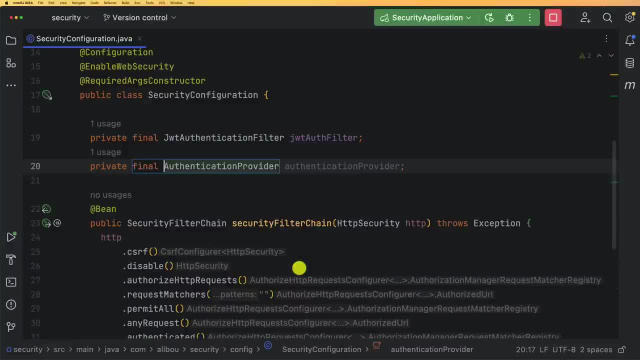 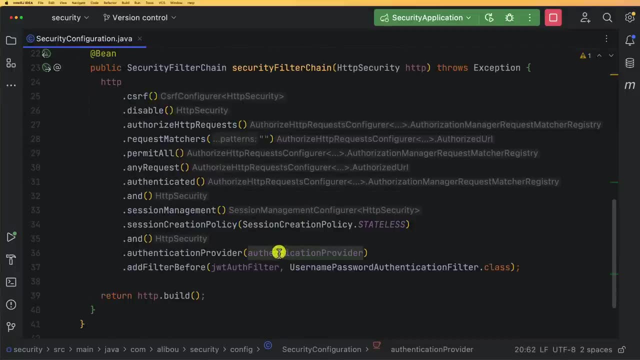 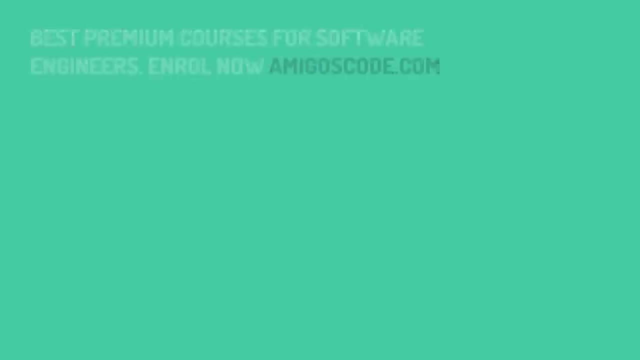 And let's make it final too. Alright, So now I have my configuration ready. All I need to do, or I need to implement now is this authentication provider, And let's do it right now. Now we need to provide this authentication provider bin. 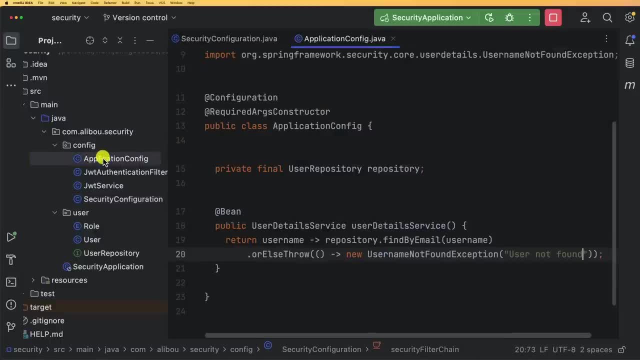 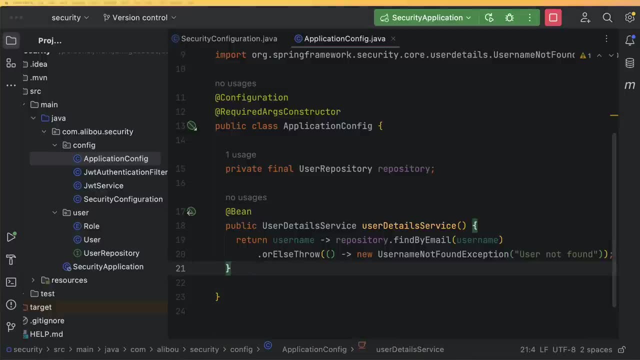 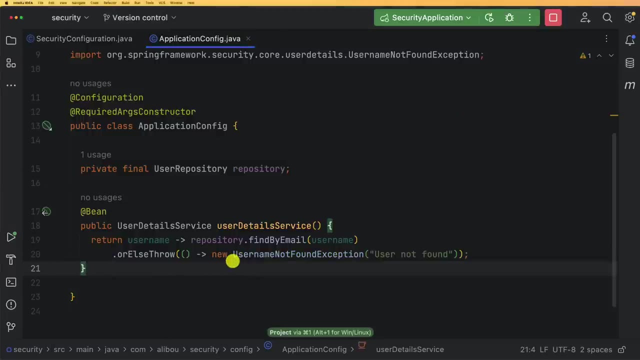 So let's go to our application config class And let's create a new bin, of type authentication provider. Ok, So for this authentication provider, Let me make this full screen. So I want to create a bin, And always public, and the bin: type authentication provider. 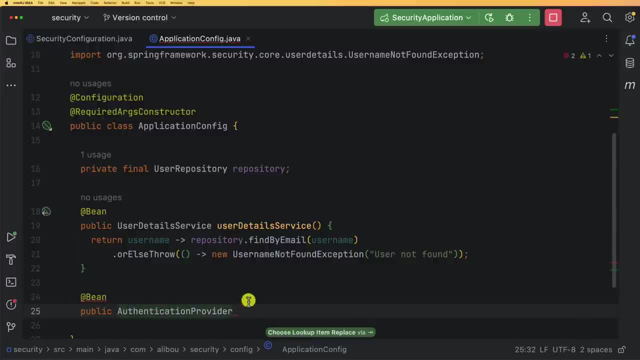 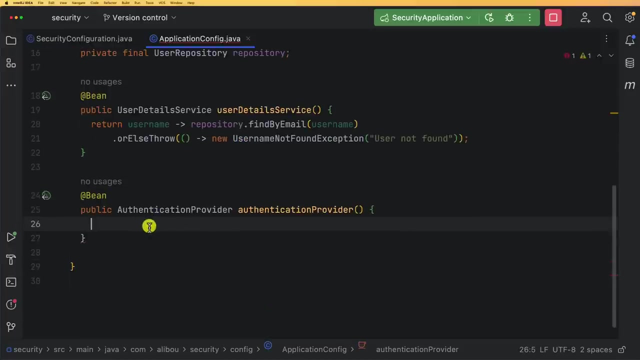 Authentication provider, always from the spring framework package, And I will call it authentication provider And let's start implementing this bin right now. So this authentication provider is the data access object Which is responsible to fetch the user details And also encode password and so on and so forth. 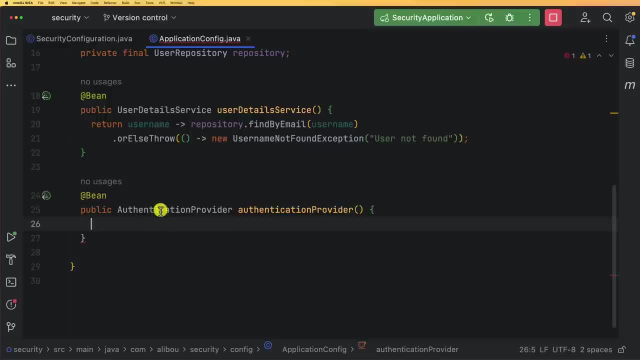 So for this we have, for this authentication provider, We have many implementations And one of them is the DAO authentication provider. So data access object authentication provider- I will call it auth provider- equals new DAO authentication provider. Ok, So within this authentication provider, we need to specify few properties. 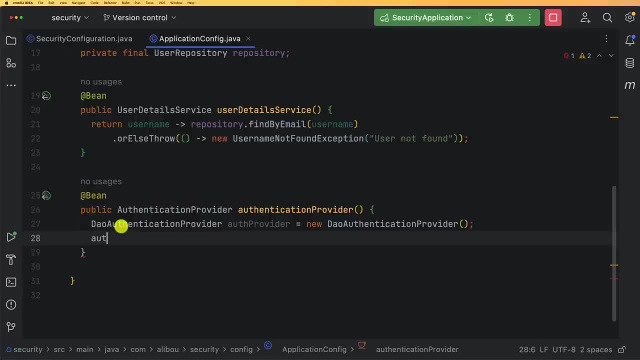 Or like not few, but just two of them, And the first one is the user details service. So we need to tell this authentication provider which user details service to use In order to fetch information about our user, Because we might have multiple implementations of the user details. 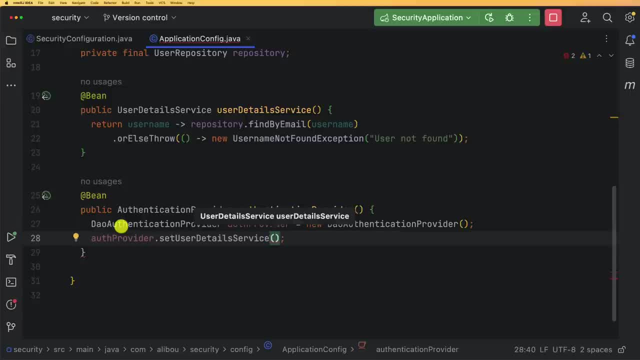 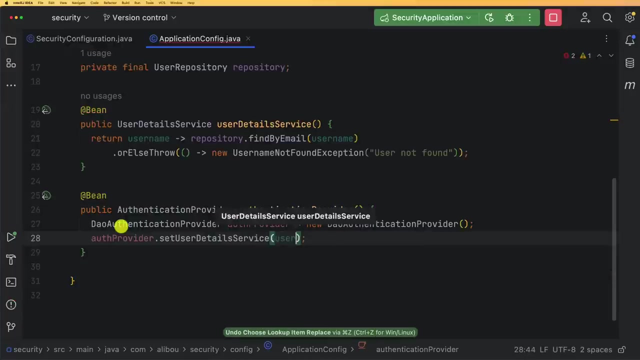 One, for example, getting the information from the database, Another one based on a different profile, Fetching the users from internet In memory database, From LDAP, and so on and so forth. Ok, So for this one we already have our user details service right here. 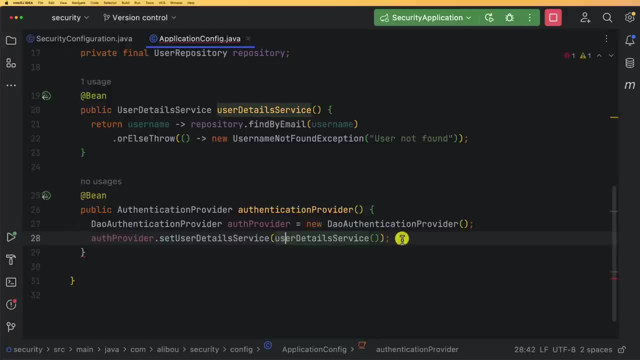 So this one is referencing this method. Next, we need to provide a password encoder. So which password encoder we are using within our application? So if you have a specific one, Or if you are using specific one, We need also to precise this one. 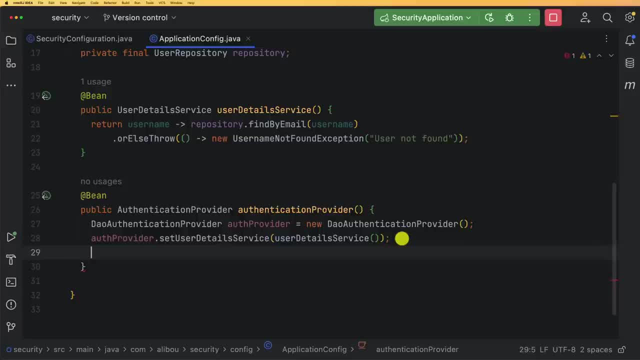 Because when we want to try or we want to authenticate a user, We need to know which password encoder In order to be able to decode the password using the correct algorithm. Ok, So auth provider dot set password encoder And here I will create a method. 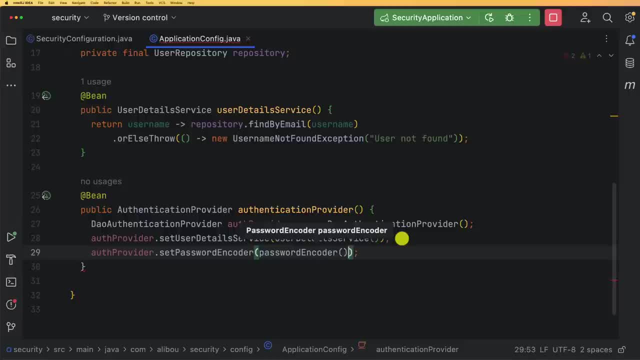 I will call it password encoder, Ok, And I will create a bin out of it later on. So this is the minimum required information that we need to provide, And then all I need to do is returning this auth provider right here. Now I will just go ahead and create this password encoder. 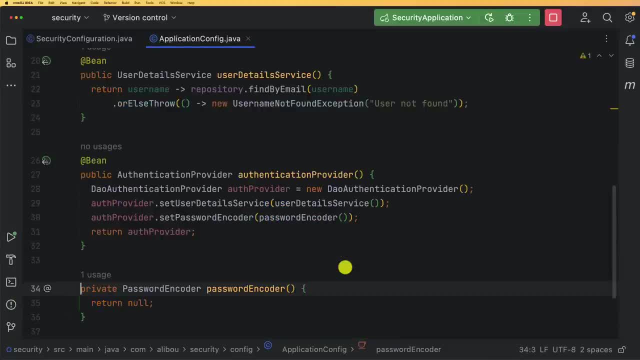 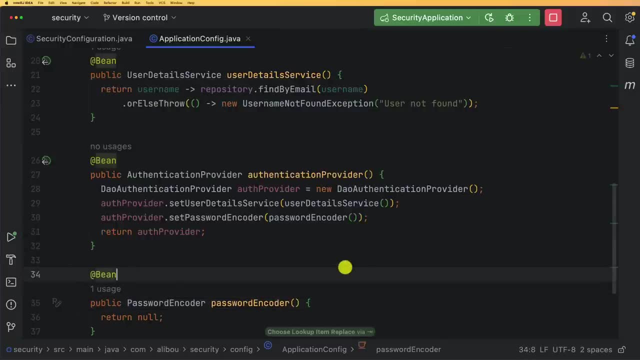 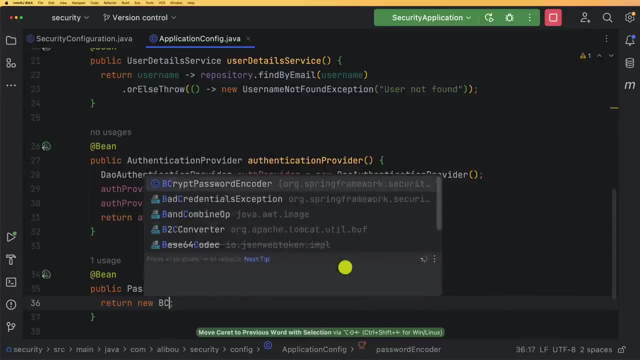 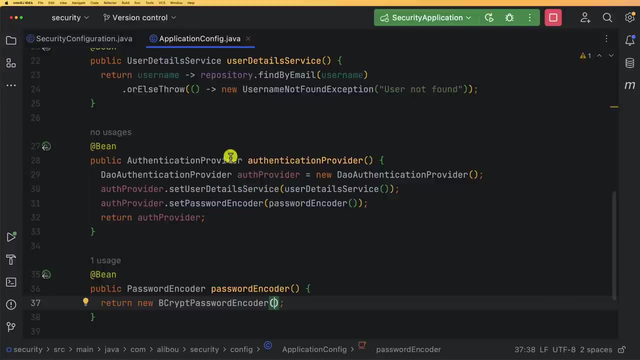 So this password encoder is also- should be also- a bin, So it will be public And I will give it The bin annotation, And for this I just need to return a new Bcrypt password encoder And that's it. So now I have my authentication provider. 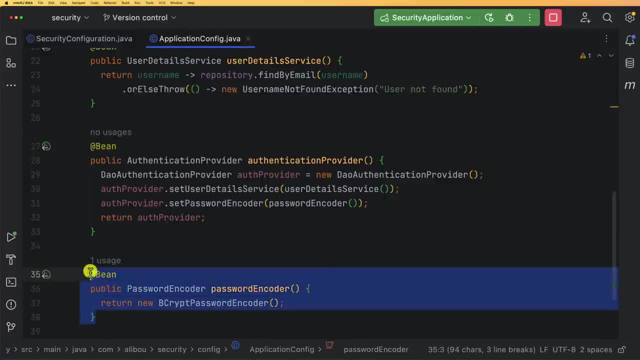 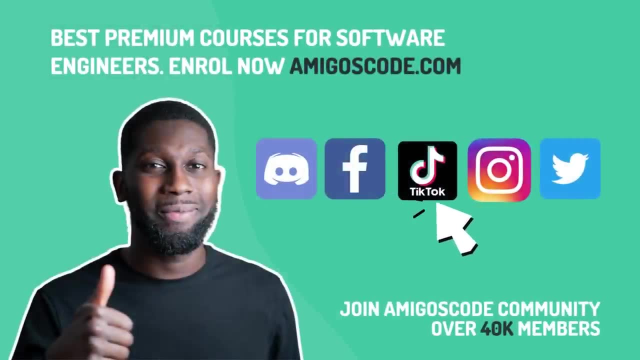 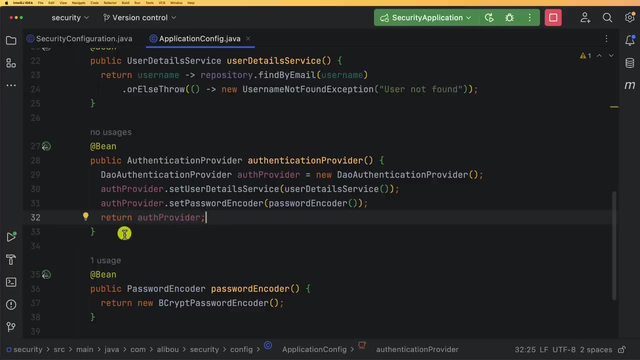 And also I created the password encoder bin. One more step is needed to finish this application: config class, Which is the authentication manager, And the authentication manager, as the name indicates, is the one responsible to manage the authentication. So the authentication manager have, or has, a bunch of methods. 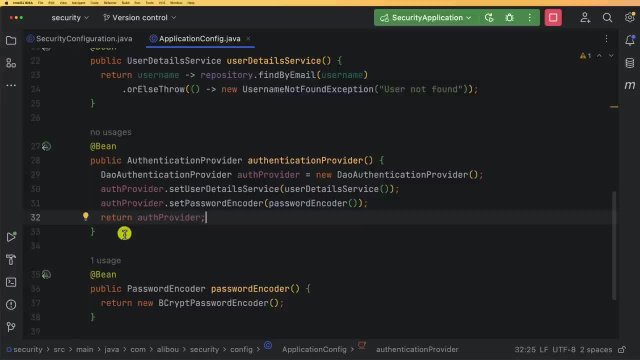 And one of them. there is a method that allow us or help us to authenticate a user based or using just the user name And password, And for that we need also to create a bin, or to provide the bin to be able to use it later on. 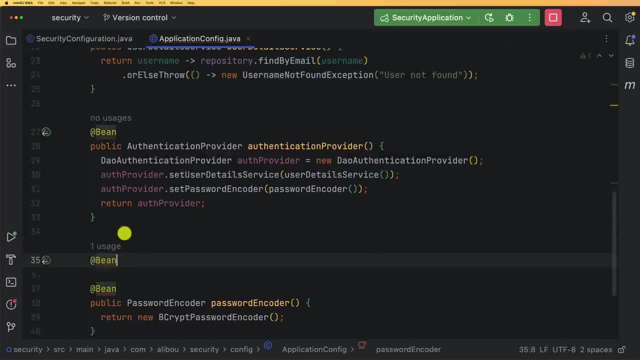 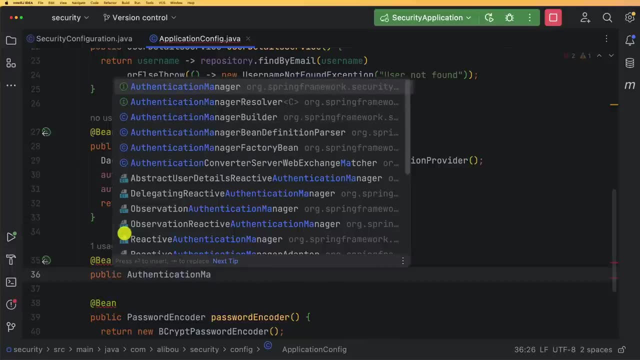 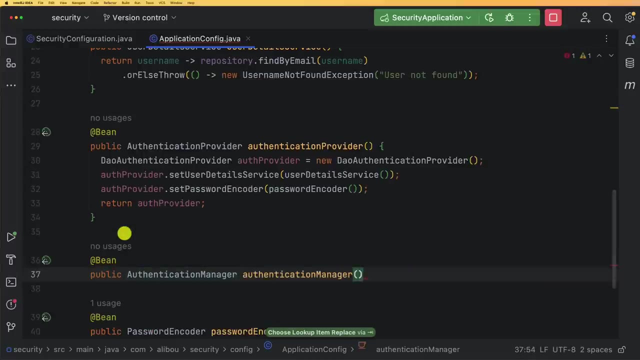 Okay, So I will create a bin And public Authentication manager, Because this is the bin that I want to create And I will call it authentication manager- And within this bin I want to inject an object of type authentication configuration. Okay, 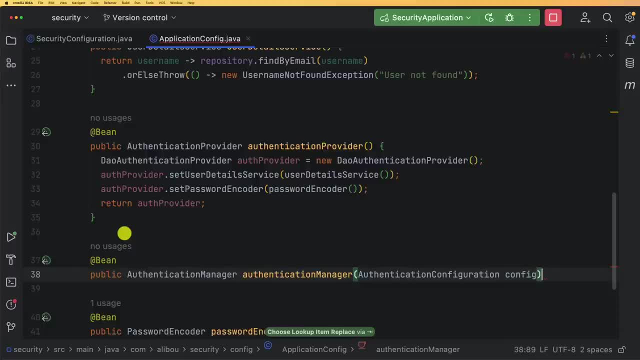 And I will call it config. This authentication configuration hold already the information about the authentication manager, So I will just return configgetAuthenticationManager. Alright, So here we are using the default implementation of Spring Boot, And this is more than sufficient for us. 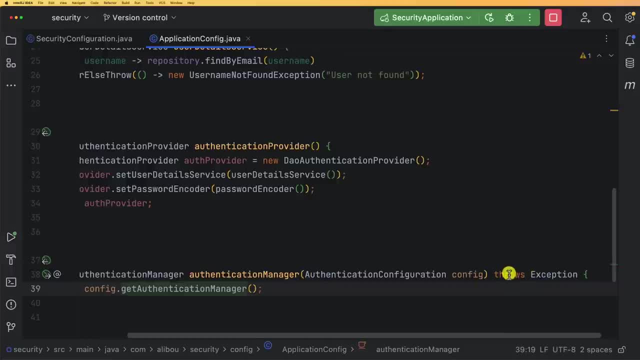 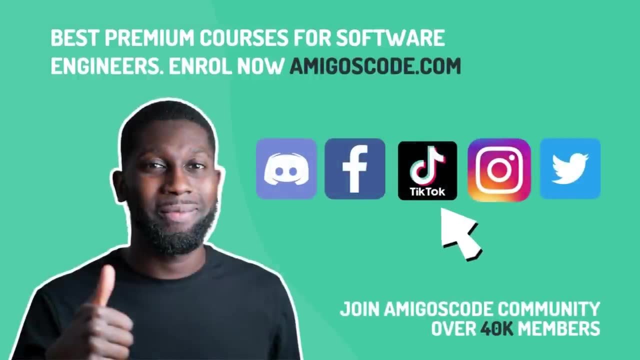 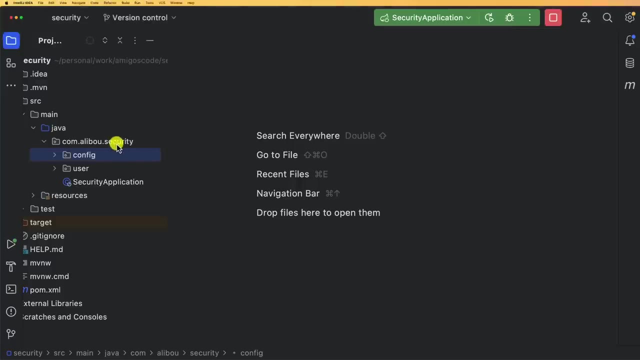 Here. don't forget also to add the exception to the main Method signature. So that's it, Let's move on. and Now we are done with all the security configuration for our application, But we still need to provide at least two endpoints where the user can create an account or also can authenticate. 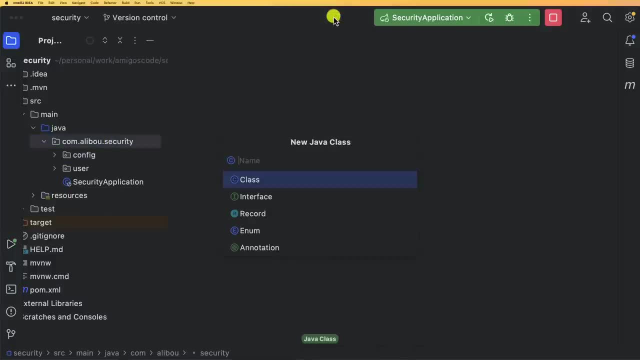 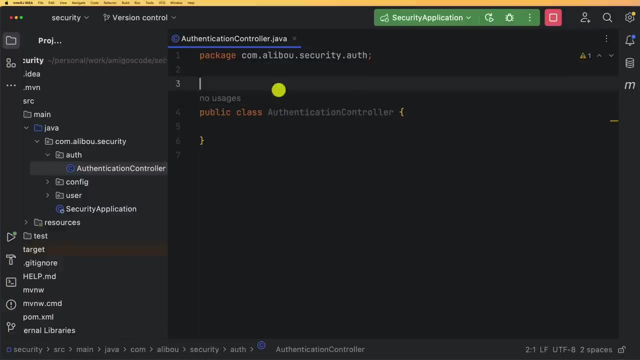 And to do so within the base package. I will create A package, I will call it auth, And within this package I will create a new controller, Authentication Controller. And this authentication controller will have two endpoints that will allow me to create or register a new account and authenticate an existing user. 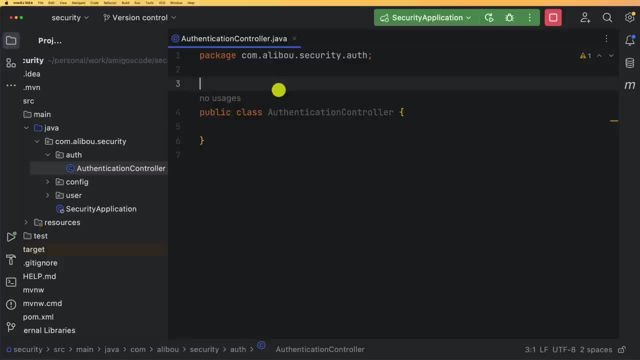 So, in order to call this or to make this class a controller, We need this annotation rest controller And also I will give it a request mapping And for the request mapping it will be slash API, slash V1, slash auth. And also I will need 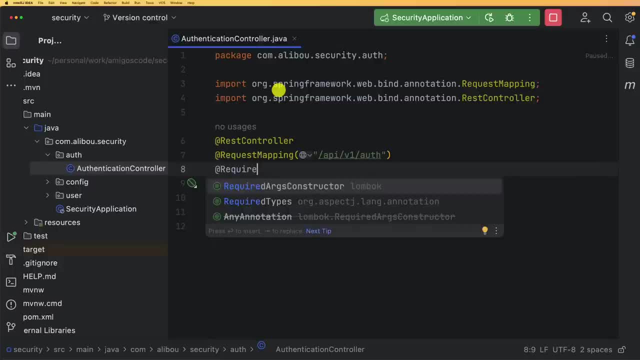 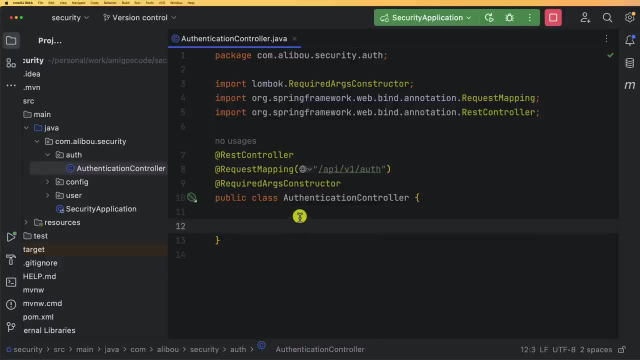 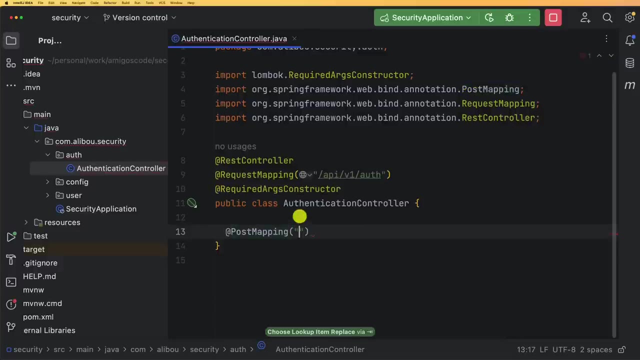 The required arcs constructor. Okay, Now, within this authentication controller, I will create two endpoints, One for register and the other one for the authenticate. So the first one, it will be a post mapping, And I will give it a register For the name. 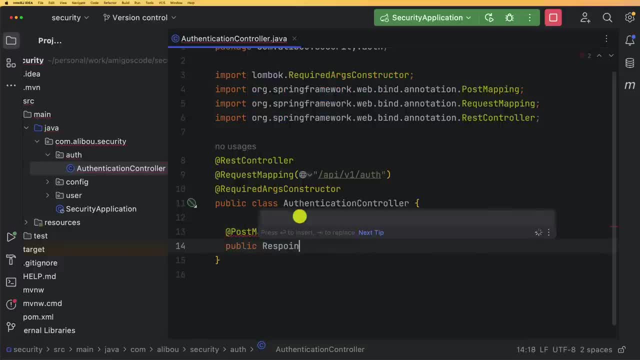 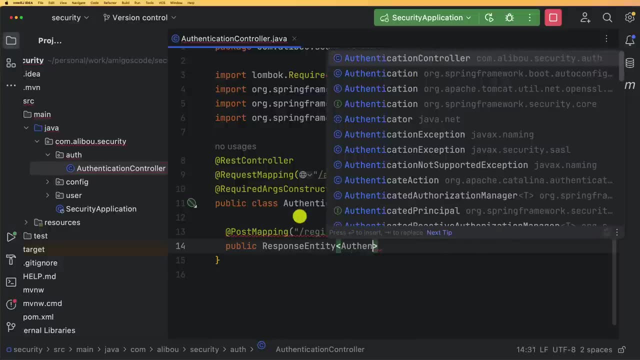 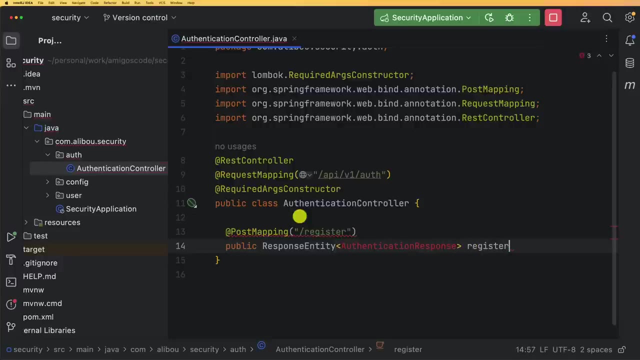 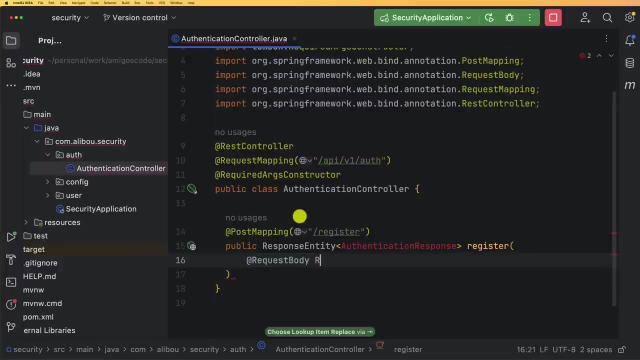 And here it will be a public Response Entity, And now the type will be authentication response. I will create an object later on for that. We will call this method register, And this register will need a request body And this request body I will create an object called. 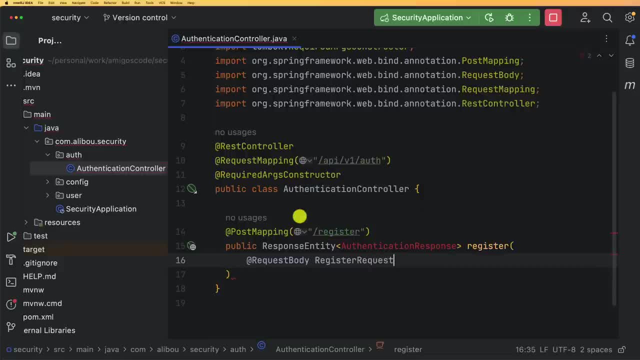 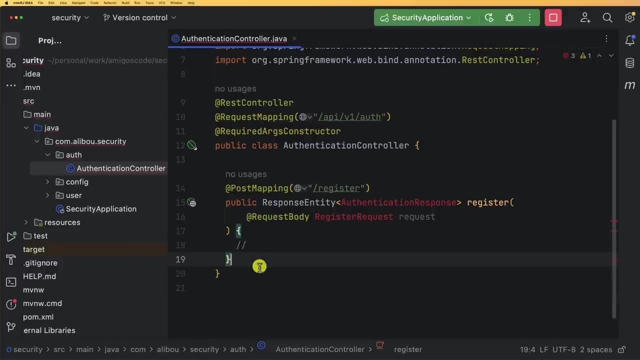 Register request, Which will hold All the requests or the registration information, like first name, last name, email and password. Okay, So I will leave it empty for now. We will implement it later on. I will do the same. I will just copy paste this one. 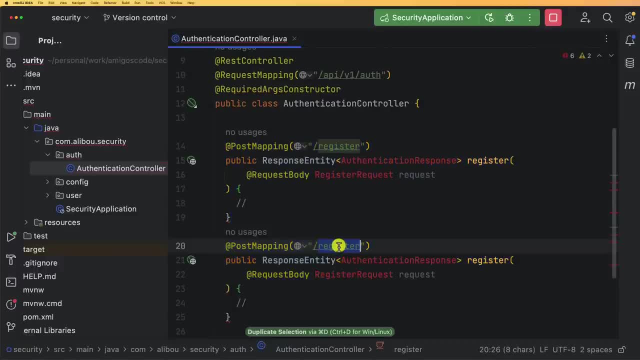 And I will create another map And I will create another method, But this one we call it Authenticate, And it will also return an authentication response, But instead of register request, We will need an authentication request. Okay, So it's an authentication request. 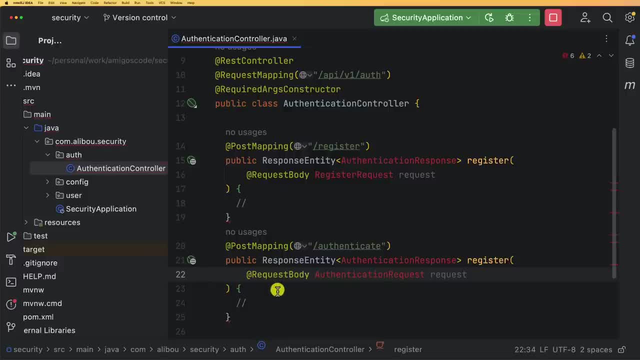 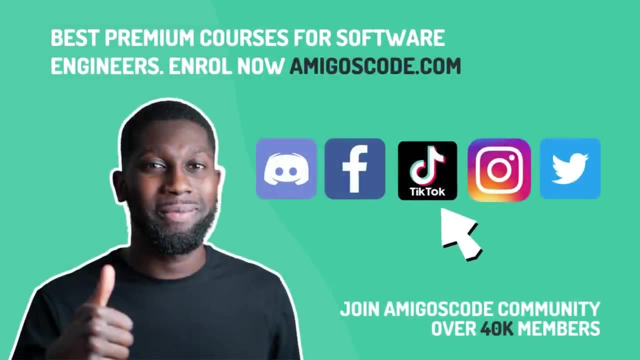 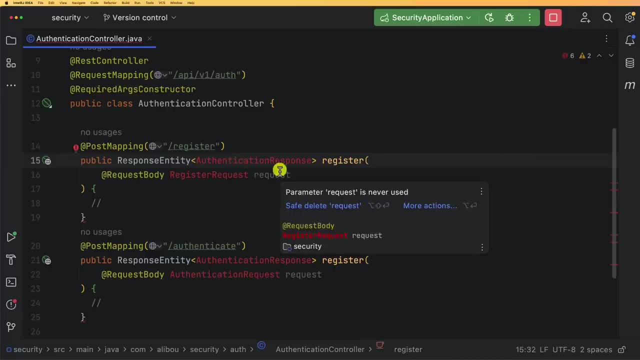 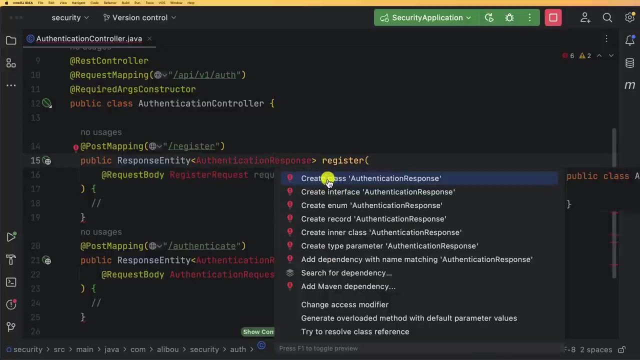 Yeah, That's it. So we have our controller ready. now Let's move on and start implementing things. Let's now create our authentication response. So now, just, I will use IntelliJ to create this class authentication response And I will create it within the same package. 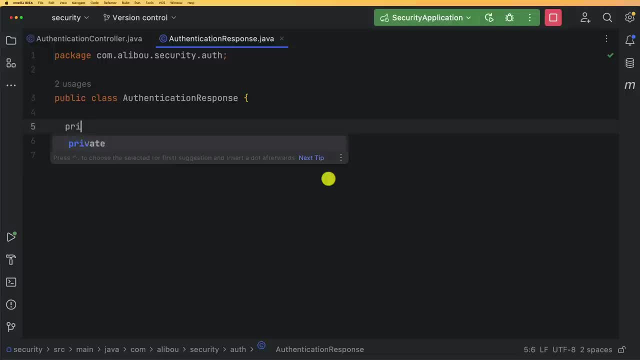 So this response is a simple class That will have only a string token. So this is the token that would be sent back to the customer or to the user, And to do that we will need this data annotation. We will need the builder. 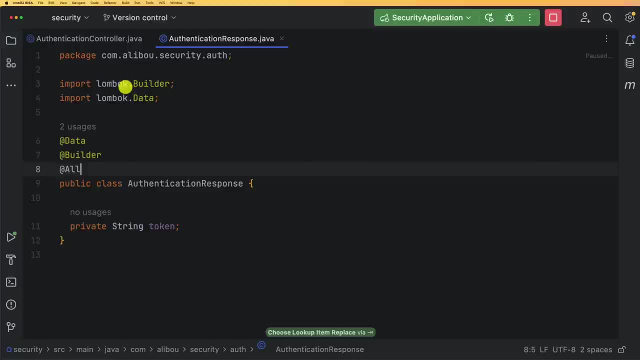 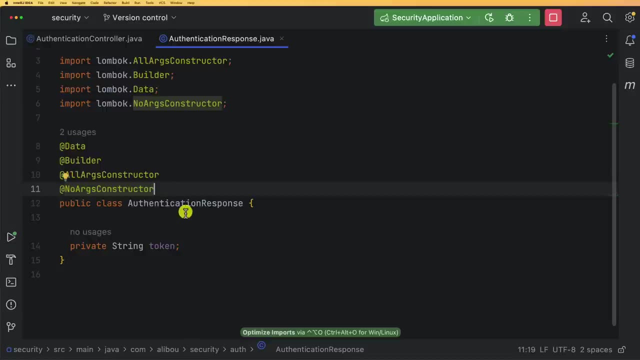 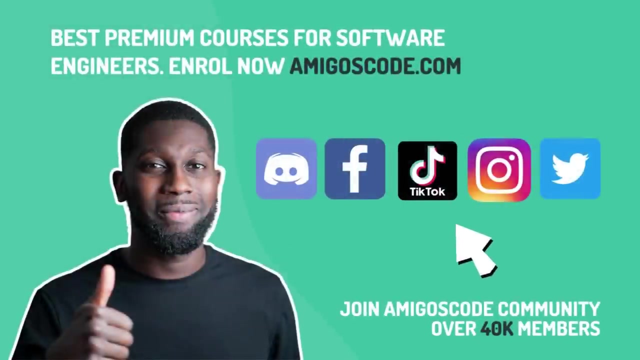 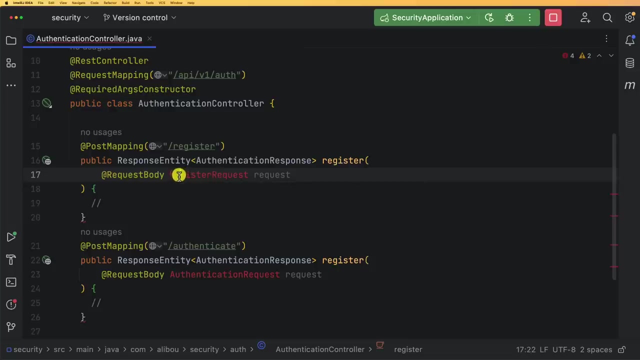 And, of course, the all args constructor And the no args constructor. So that's it. So our authentication response is ready. Let's move on and create the register request. Now let's create this register request class. So create a class right here. 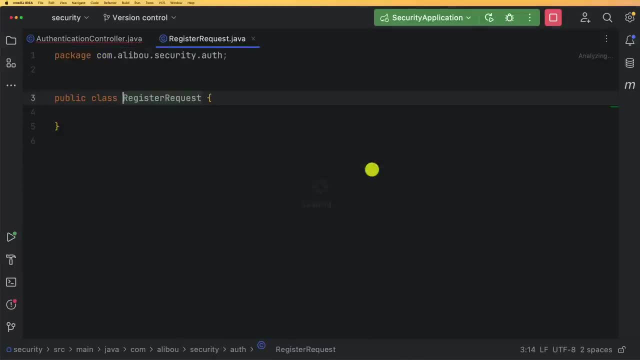 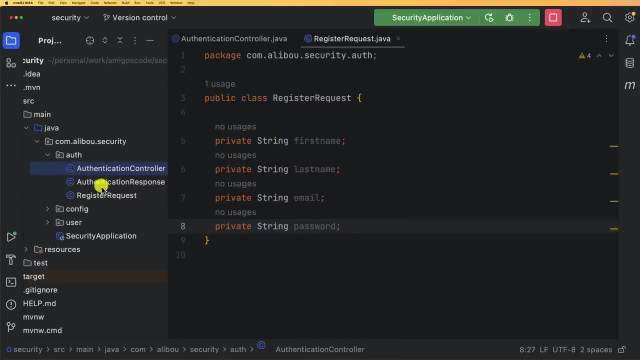 And we will create it within the same package. So this register request. It will also have few attributes, Like private string, first name, Private string, first name, Private string, Last name And also an email and password. So we will also need the same annotations as we used within this authentication response. 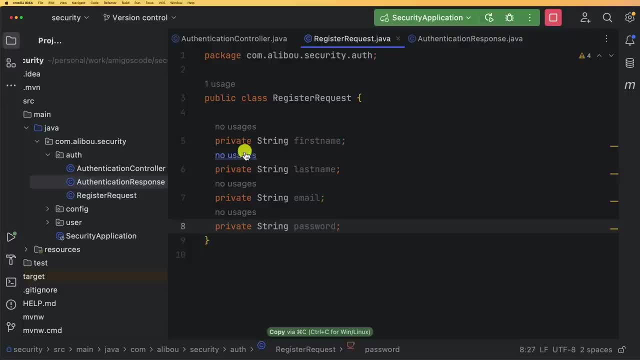 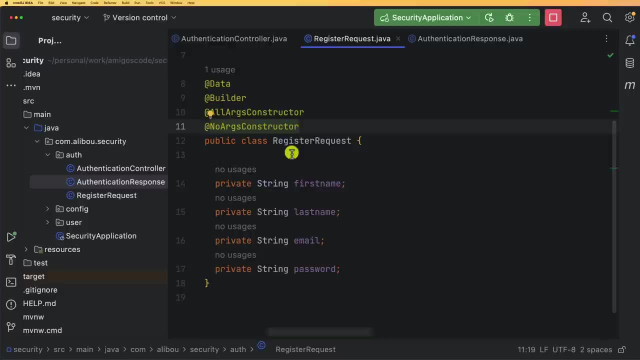 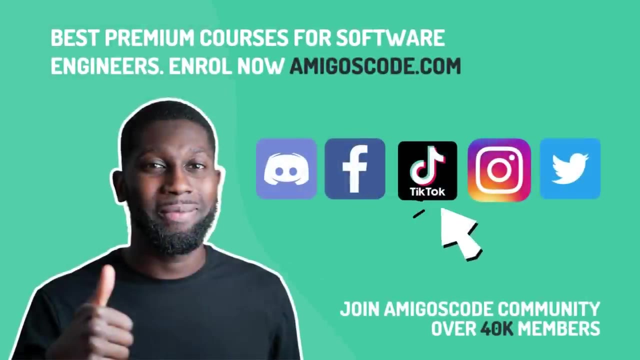 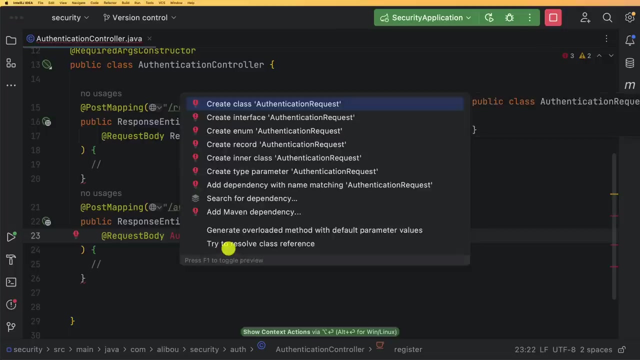 So just go ahead and copy them And put them within this register request. Okay, So we have also our object register request ready. I will create, as a next step, the authentication request object. Finally, we need to create this authentication request within the same package. 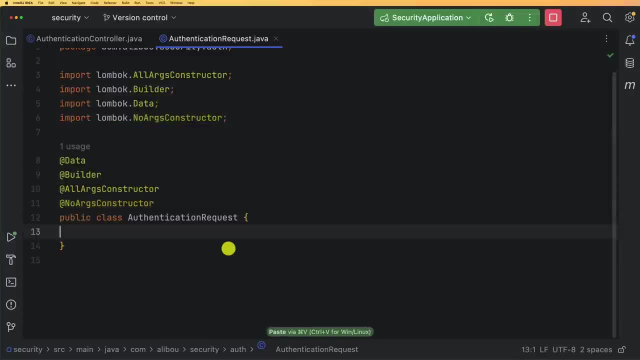 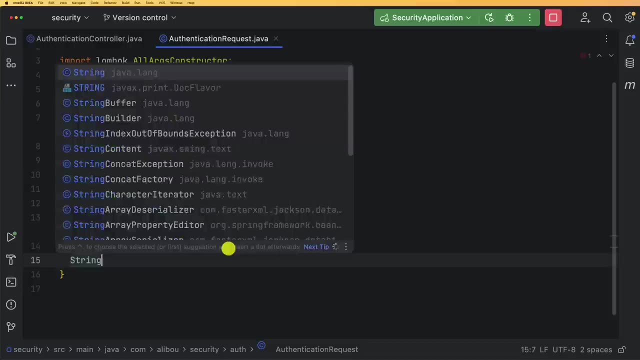 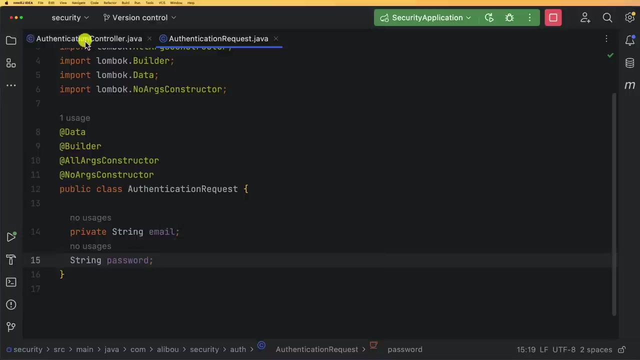 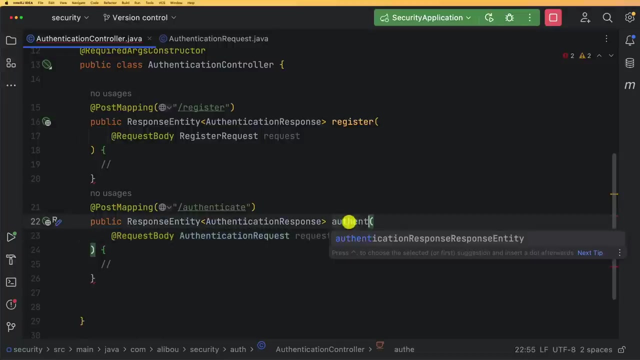 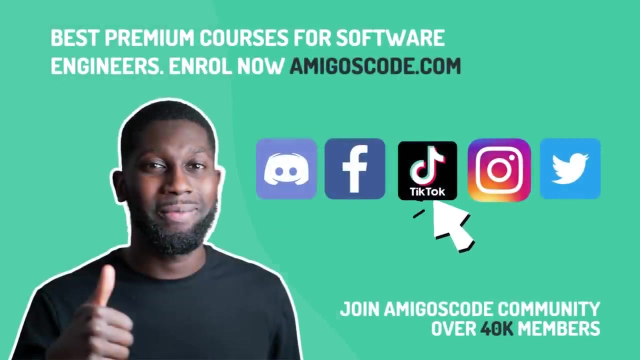 So I will just paste the same annotations, And here this object will hold only two information, Which is the string email And string password. Okay, So that's it. Our object now ready, Let's move on and start implementing this. author register and authenticate request. 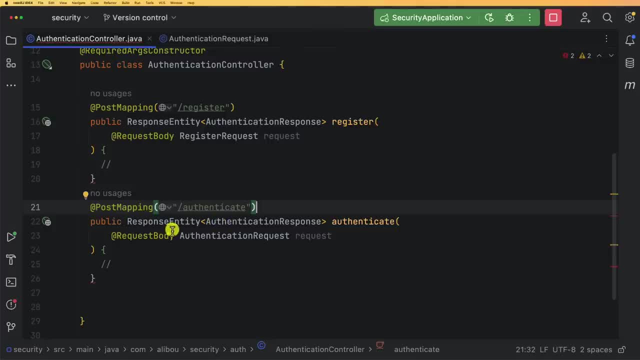 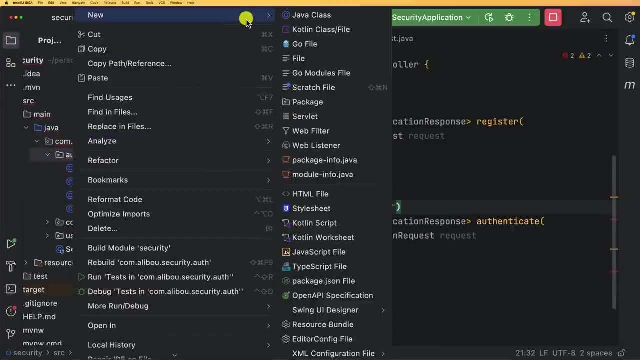 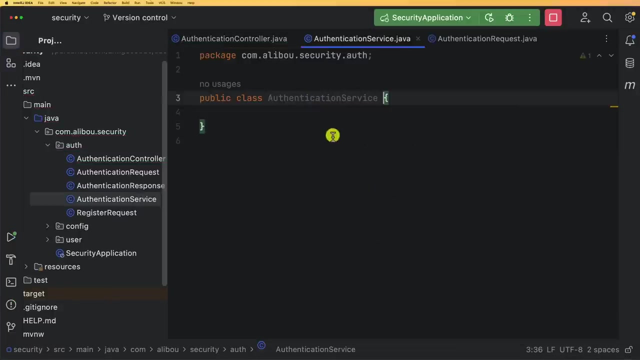 So for the registration and authentication implementation, I will delegate this to a service. So within this auth package, I will create a new class And I will call it authentication service. All right, This is the place or the class where I will implement these two methods. 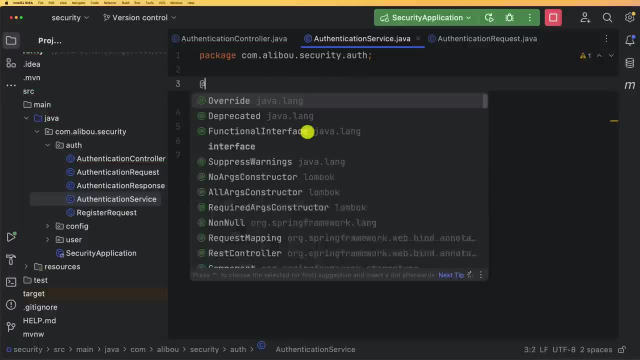 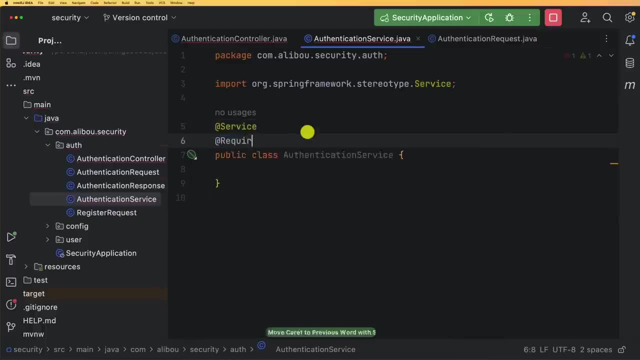 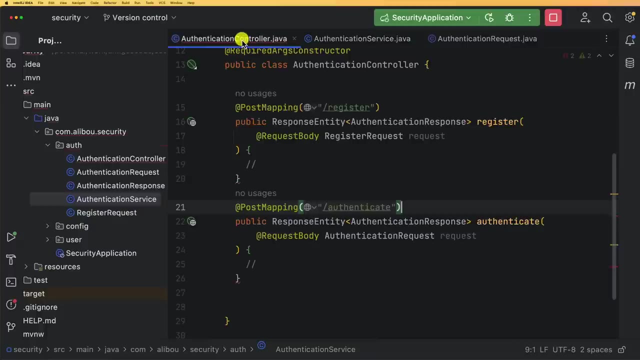 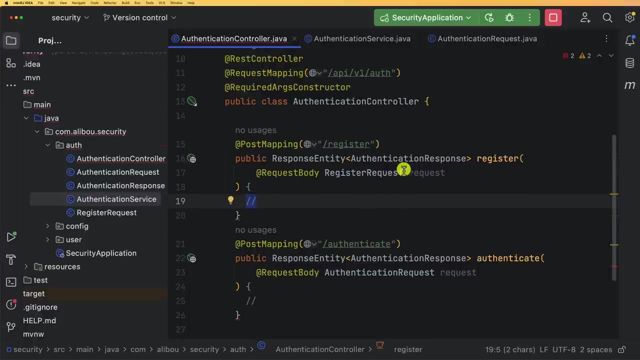 Register and authenticate. So here I will just give it the service annotation And of course the required args constructor. All right, So here we have these two methods. I will just move on And here just make a simple call for this service methods. 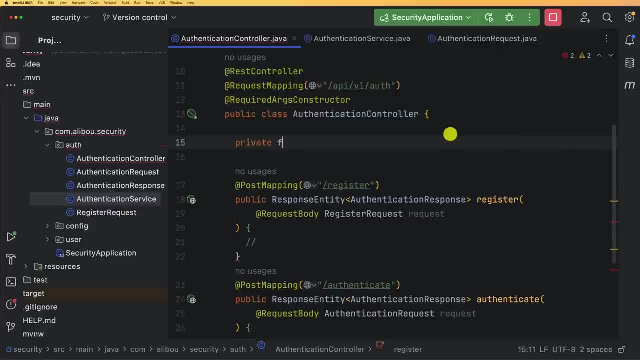 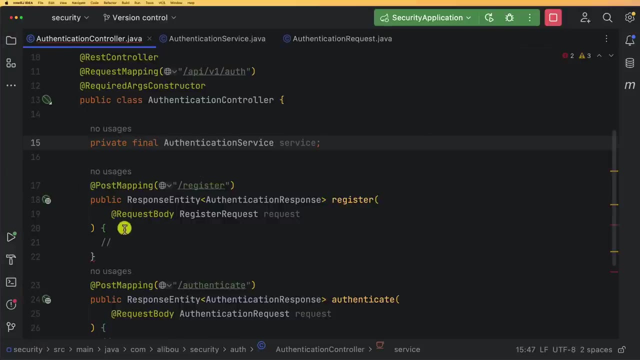 But first let's inject it. Okay, So I will need private final authentication service. I will call it just service right here And within this authentication service. Let me make this full screen Now I will just make the return statements for these two methods. 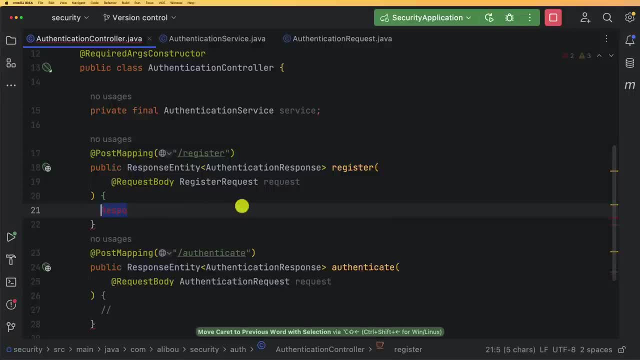 All right. So here I will return a response. entity Dot: Okay, And I will call my service dot register And I will pass this request as parameter. Okay, And I will copy paste this And paste it right here And instead of register, it will be authenticate. 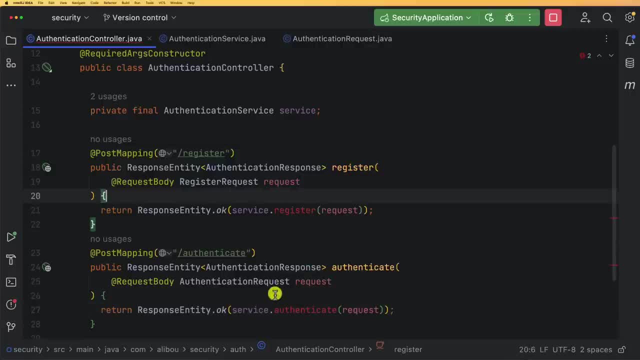 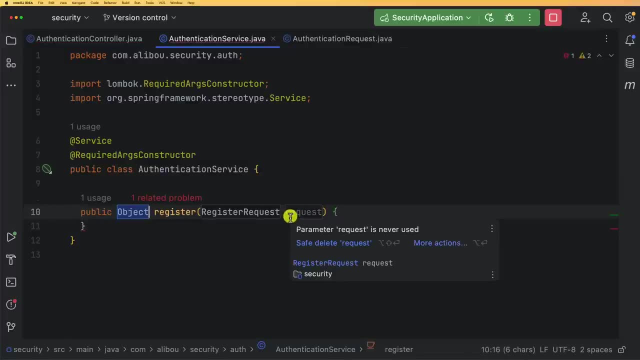 So here we don't have yet our register and authenticate method, So let's go ahead and create them. So create method, register And this one will return the authentication response. So this is what we want to return, And now we can also create this authentication response. 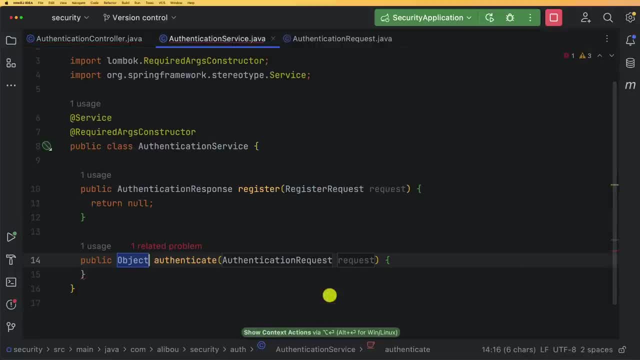 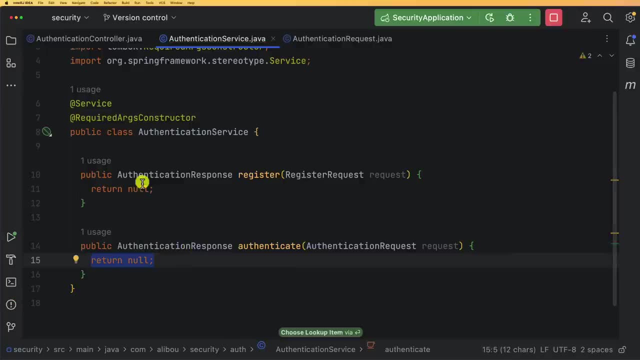 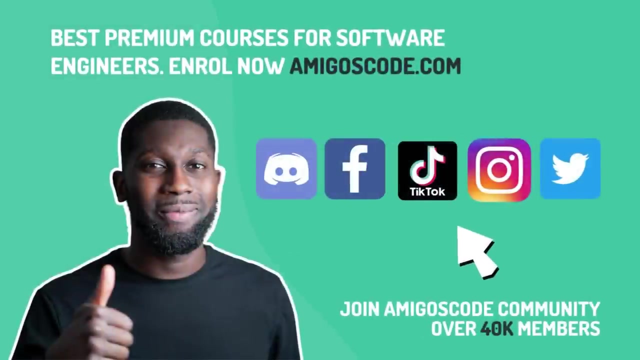 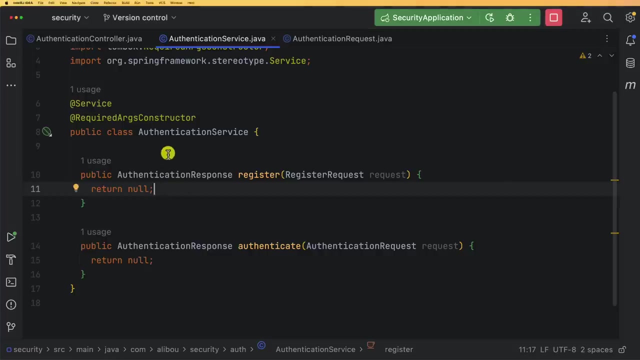 So let's create this authenticate method And the same it should return an authentication response. All right, So now I will start implementing these methods. So now let's implement this register method. So this register will allow us to create a user, save it to the database and return the generated token out of it. 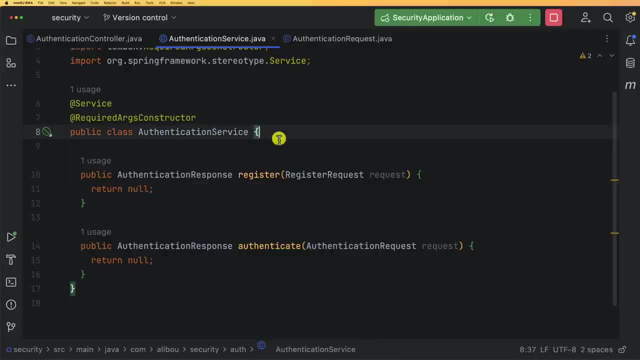 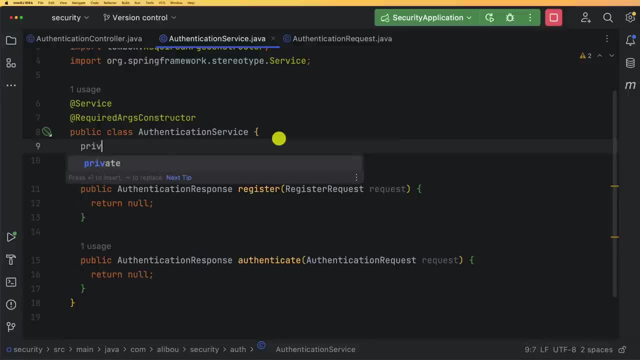 Okay, So for that, because we need or we want to interact with the database and save the user. So the first thing that we need is to inject our repository- Let's call it repository, right here. And then what we need to do: 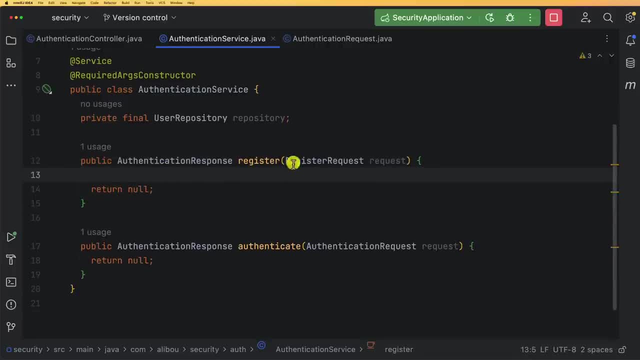 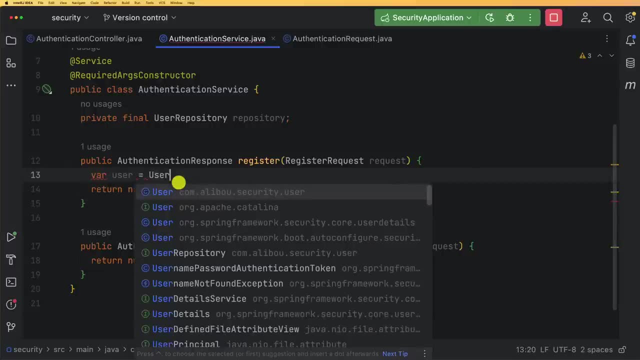 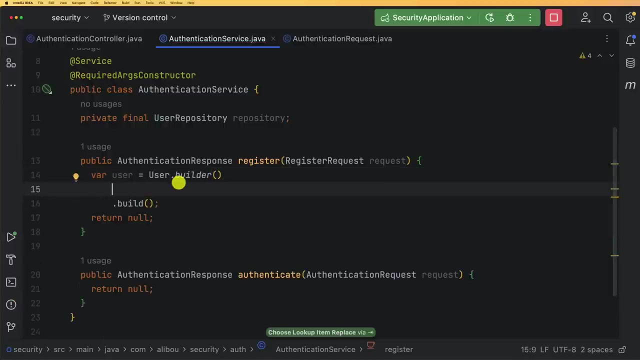 I want to create a user object out of this register request. So I will create a var user equals user, dot builder, And here dot build. So to build this user out of this register request. So I will have the first name, which is request, dot get first name. 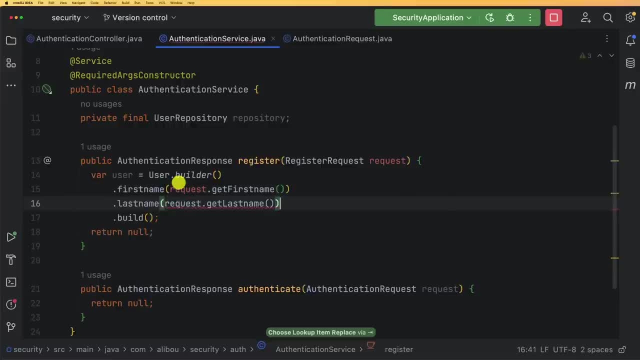 Same for the last name And same for email, So it's email And then the value will be the request dot get email. Now for the password. As you remember, we created our bean of type password encoder, So for this we need to encode our password before saving it to the database. 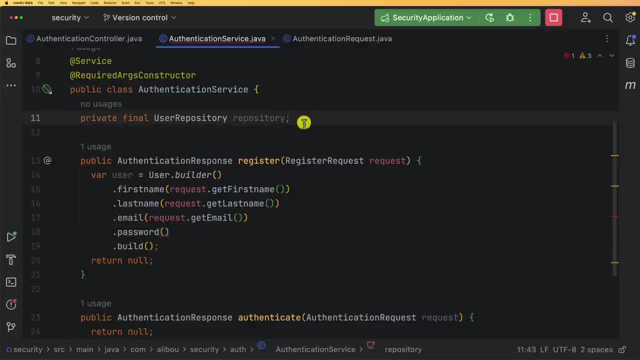 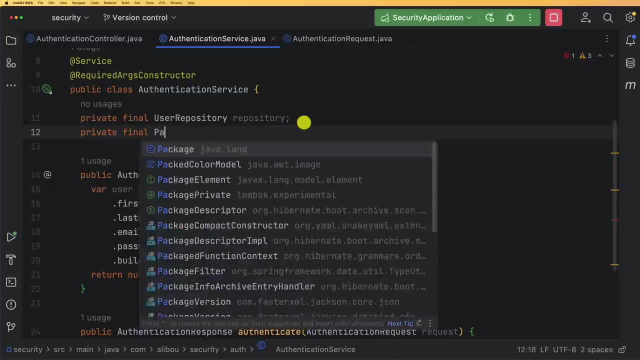 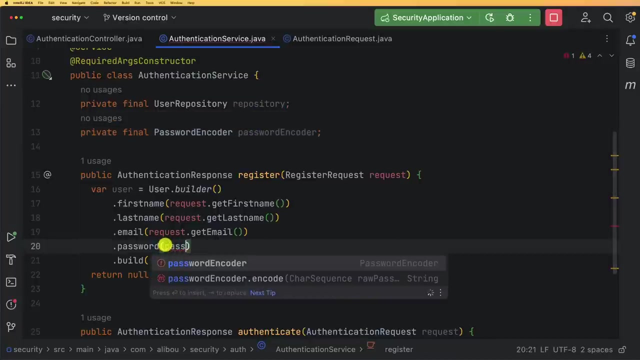 Okay, So in order to encode the password, We need All to inject our password encoder service. So I will do that: Password encoder, password encoder, And this- I will use it right here- Password encoder, dot encode. And here I have the get password or the request dot- get password that we will receive within the registration request. 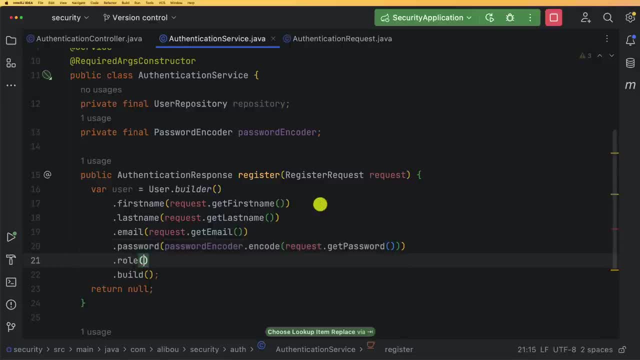 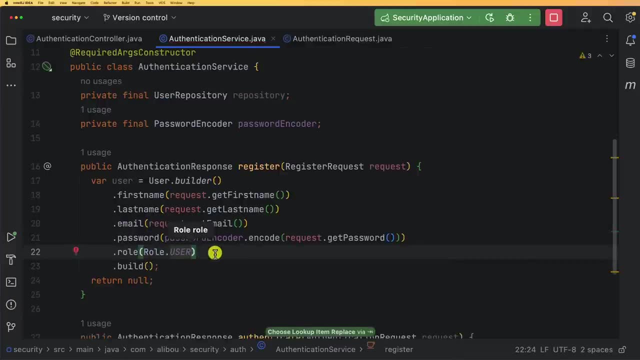 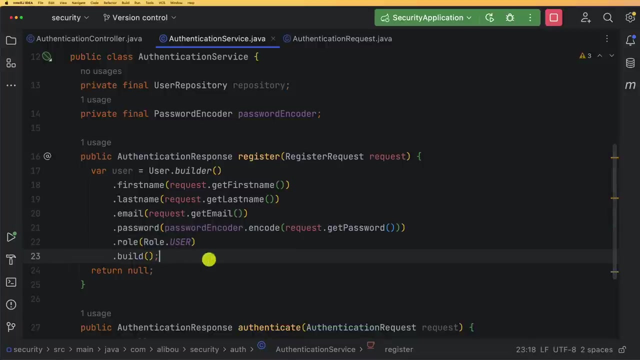 Okay, So Here I will just make a static role always, So I will use a user role, And then we call the build method: All right. So once we build our user object, The next step we need to do is our repository dot save. 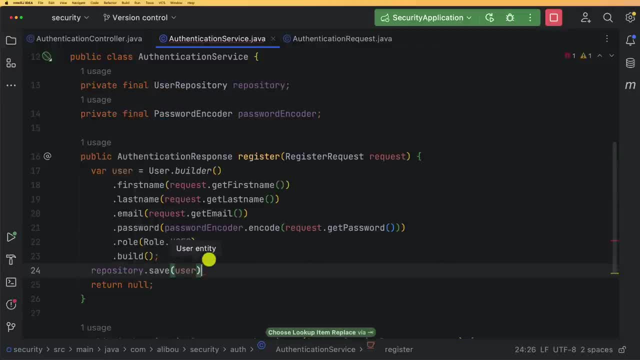 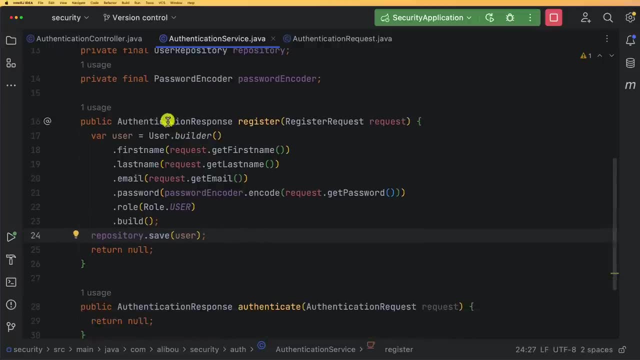 And we want to save the user that we just created, All right, And finally To be To return this authentication response That contains the token. I will create a new variable. I will call it JWT token equals. Now I will need my JWT service to generate that token. 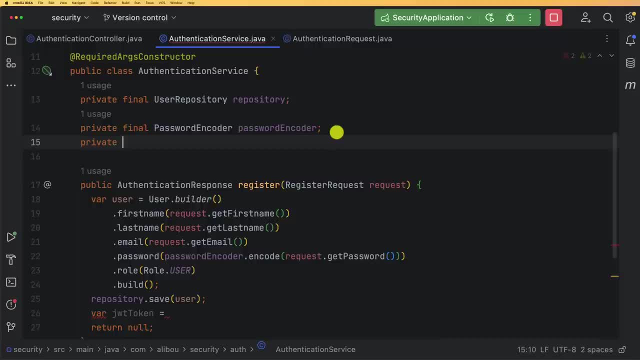 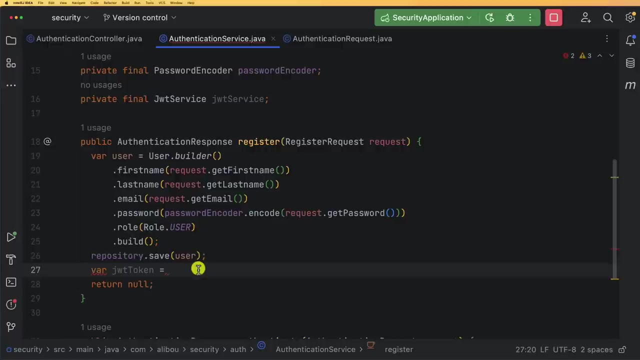 So I will. I will inject also the private final JWT service And I will use it to create or to generate the token using this user object right here. So JWT service dot, generate token The one only using user details. for the moment I don't need to set any extra claims. 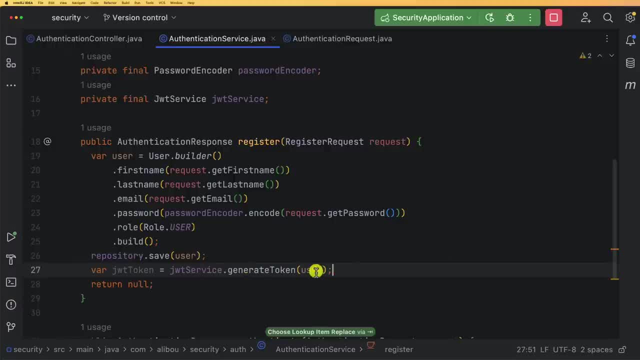 So I will use this user object to create or to generate the token And, finally, I will return an object of type authentication response, dot builder, dot build And I need to pass dot token or I need to pass the token that I just generated. Okay, 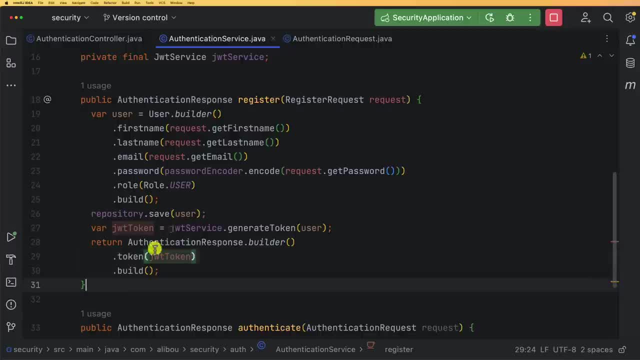 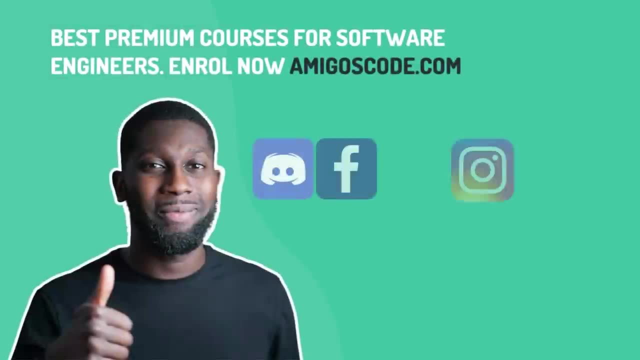 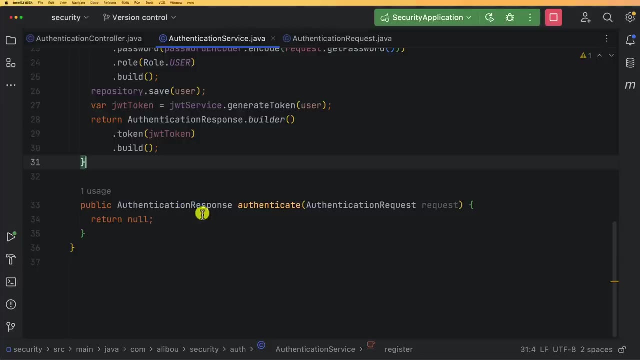 So this is the register method And now everything is implemented. Let's move on and implement this authenticate For the authentication. It's, it's an easy peasy. So you remember, We spoke before about the authentication manager bean And we said that this authentication, authentication manager bean has a method called authenticate. 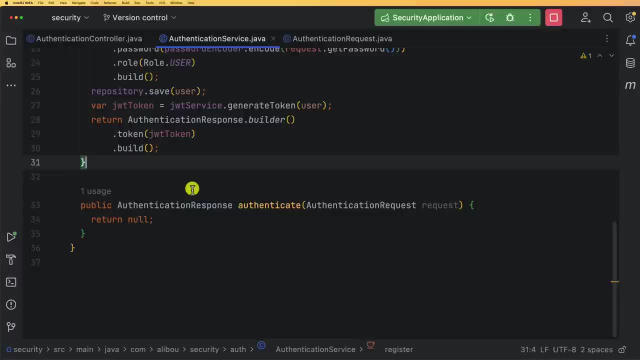 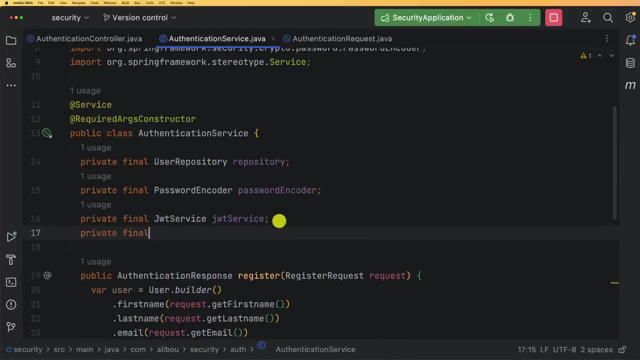 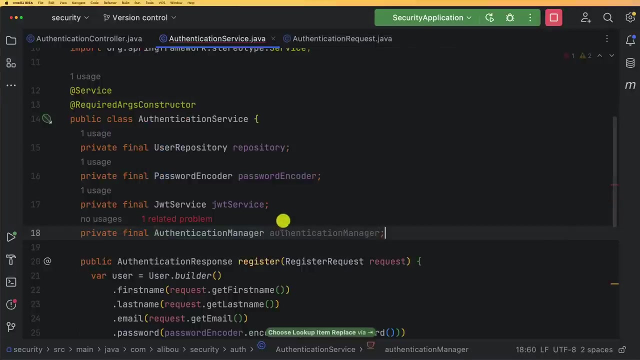 Which allow us to authenticate a user based on the username and password. So for that I will inject first of all my private final authentication manager. Bean, I will call it authentication manager, All right, So I will go back here to this authenticate method. 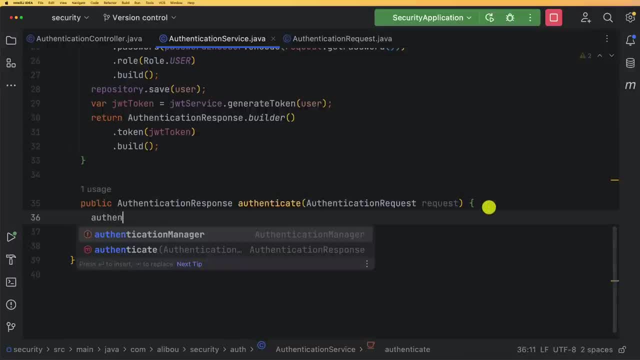 And to authenticate the user. All I need to do is to call the authentication manager, dot authenticate, And this authentication manager takes an object of type username password authentication token. So I will pass a new username password authentication token And within this I need to pass the email. 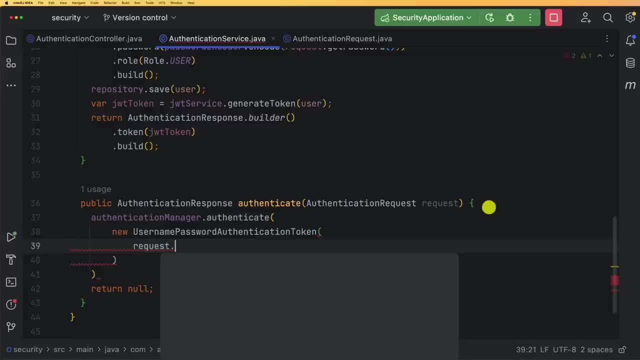 So request dot get email And also the password. Request dot get password, And this authentication manager will do all the job for me. And in case the user is not, the username or the password are not correct, So an exception would be thrown. 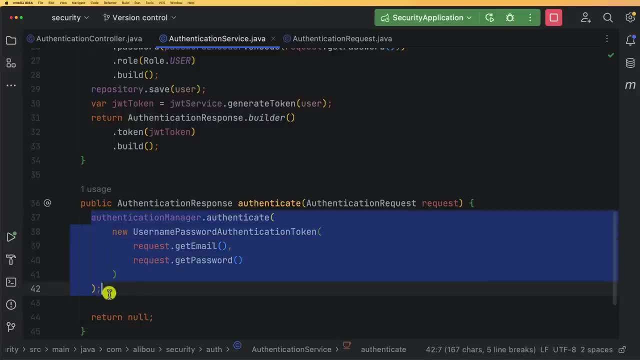 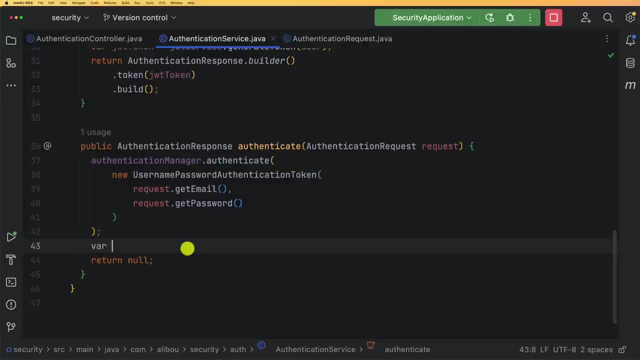 All right. So I'm totally secure when I just call this method. Otherwise what I need to do, I need to create a user And if the user asks me, So if I first of all, if I get to this point right here, means the user is authenticated. 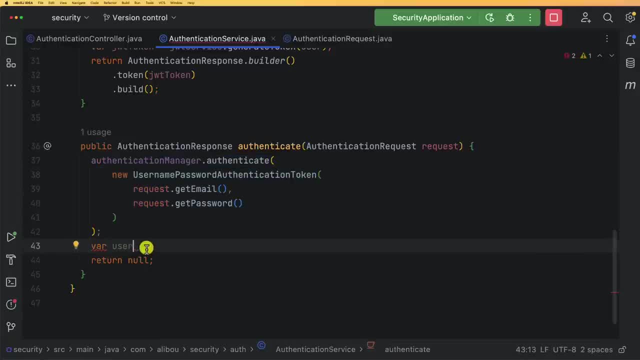 So means the username and password are correct, If both of them are correct, So I will just need to generate a token and send it back. Okay, So I will first of all find, try to get the user And find by email, And I will use the request dot get email. 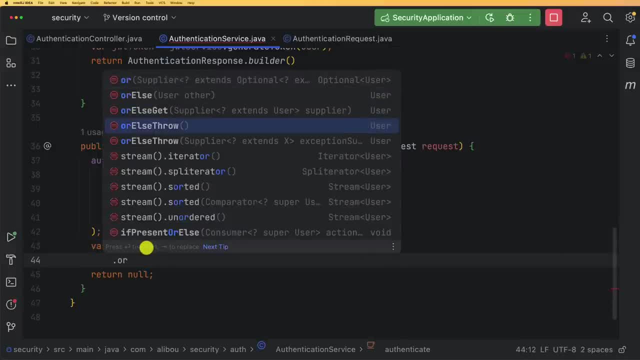 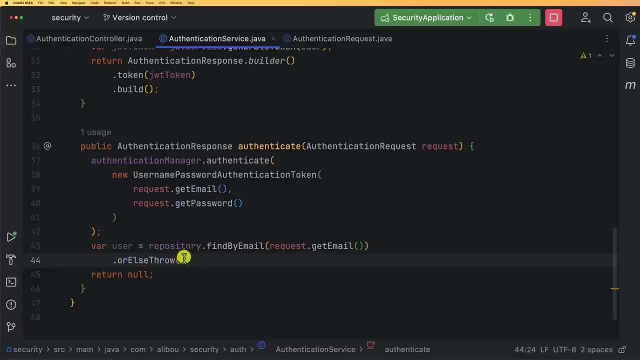 And here, or else I will just throw Okay, Or just throw any exception, Like it's not so important at this level, But for you you might want to throw the correct exception And you need to catch it, handle the exceptions and so on and so forth. 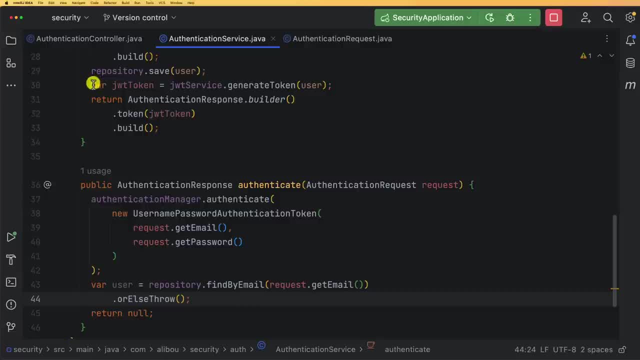 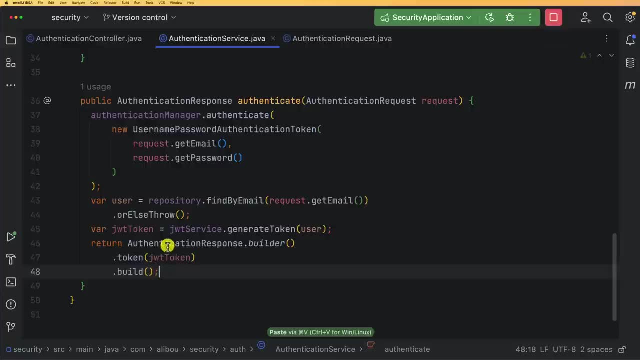 All right. So now I will just go ahead and copy this code, because it would be the same, And put it right here. So once I get the user, I will generate a token using this user object And then return this authentication response. So now we have this authenticate method and the register method ready to use. 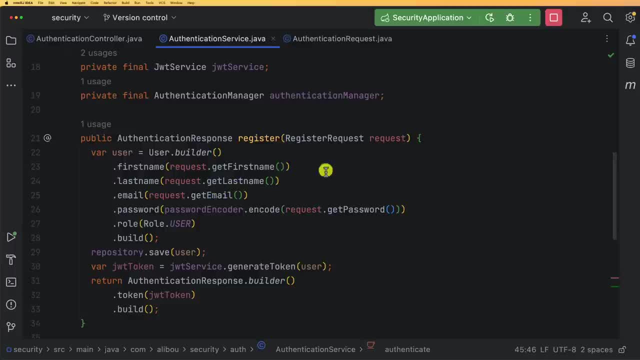 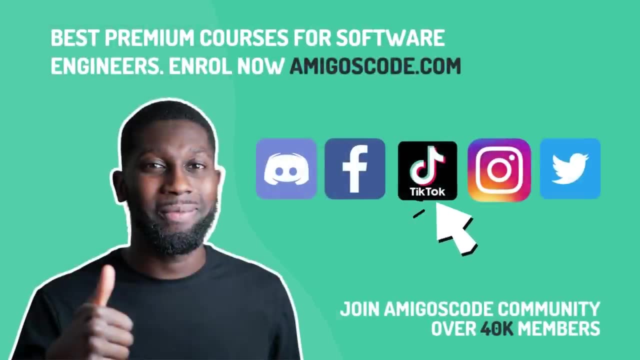 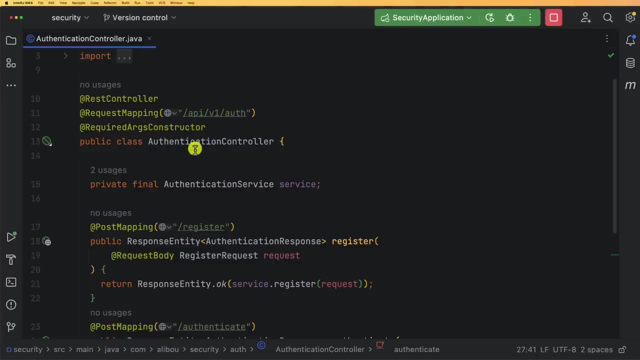 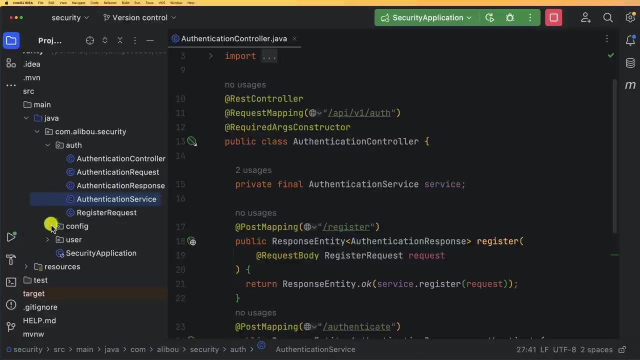 Let's move on and see what is the next step. Now we have our authentication controller ready to use, But there is one extra step, One extra step that we need to do. Do you remember when we first implemented the security configuration and we spoke about? 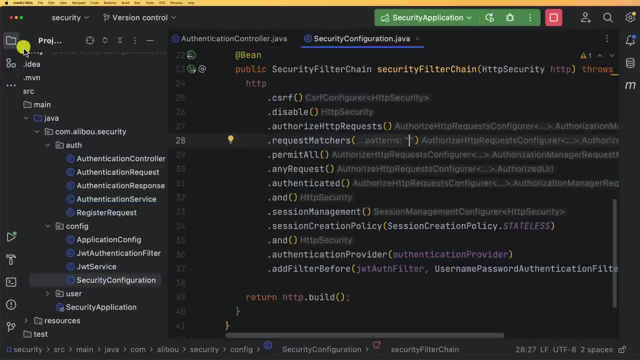 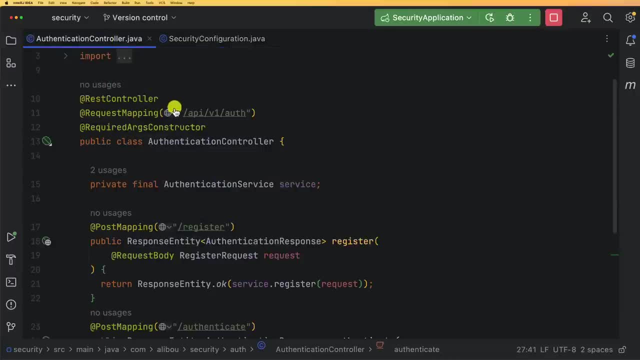 this white list right here. So what we need to provide now within this request matches that we want to permit all. We need to provide or authorize all the URLs or all the methods that we have within this authentication controller. So go ahead, Copy the request mapping that you created. 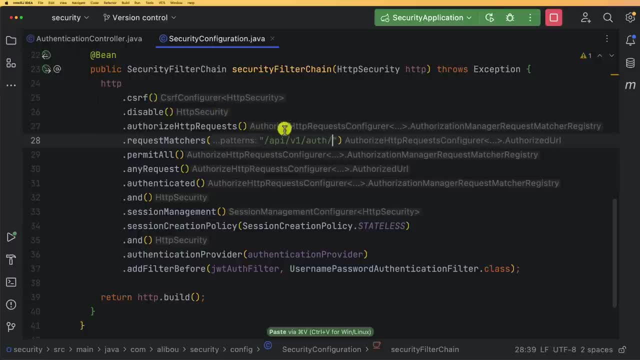 And, for example, here I want to authorize all the methods that I have within this authentication controller. Why? Because, based on my design, everything that I have in here only authentication related methods, So I don't have any business logic methods or endpoints within this authentication controller. 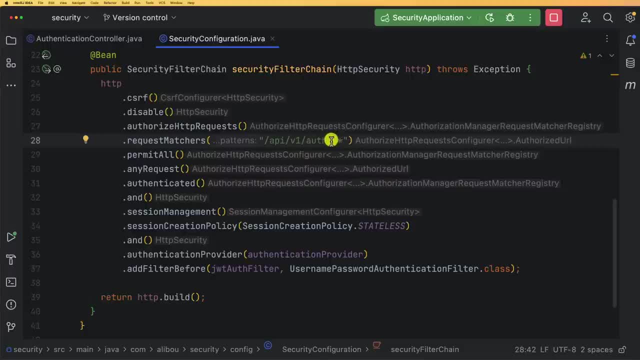 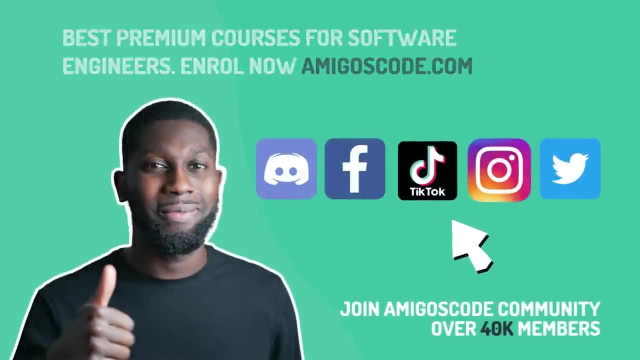 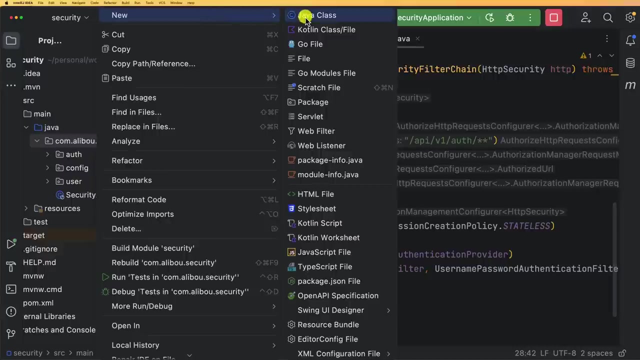 So that's why I'm allowing- I'm allowing All the methods within this controller. So that's it. Now let's create a demo controller for that. I will create a new controller within a new package. So right click here, new class, and I will call the package demo, and I will call it demo controller. 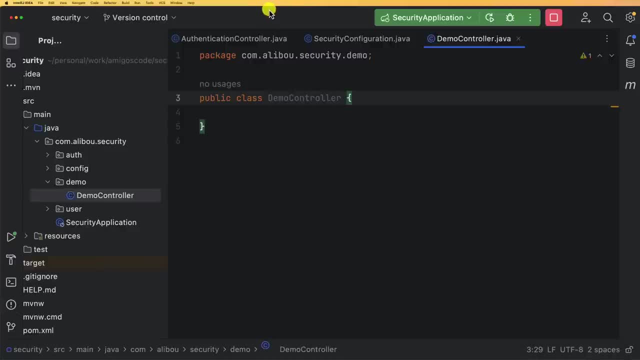 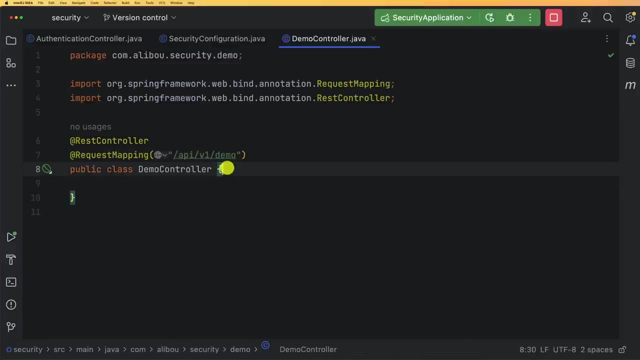 So this demo controller will be also secured. So I want this endpoint to be secured. I will copy this, this annotations right here, Paste it here, And so this one will be demo And let's call it demo controller. And now I will create just a get mapping, a simple method that 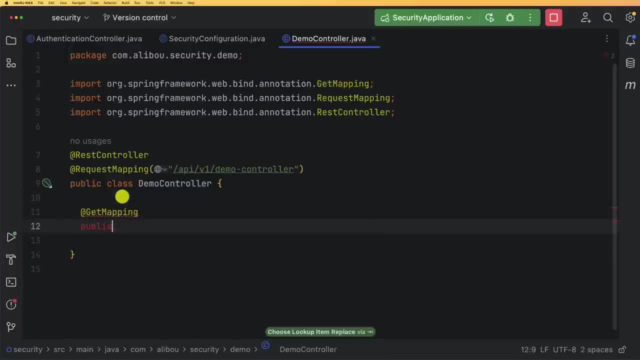 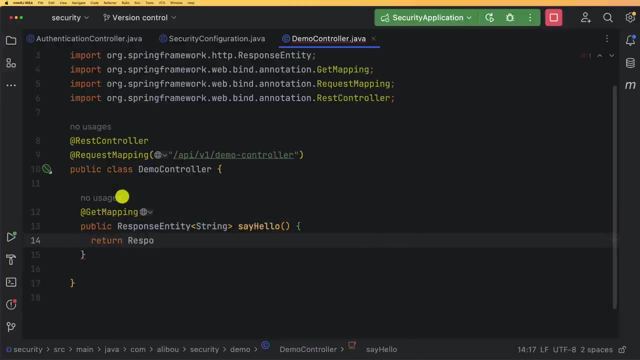 Public. that will return a simple string: Okay, Response entity of type string Say hello, for example, and then I will just return a response entity Okay, And with a body: Hello from secured, Hello from secured endpoint, And that's it. 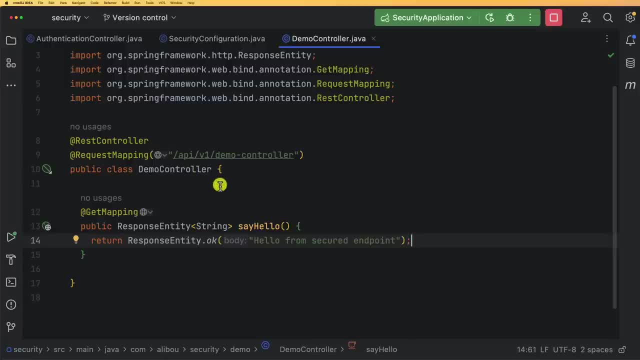 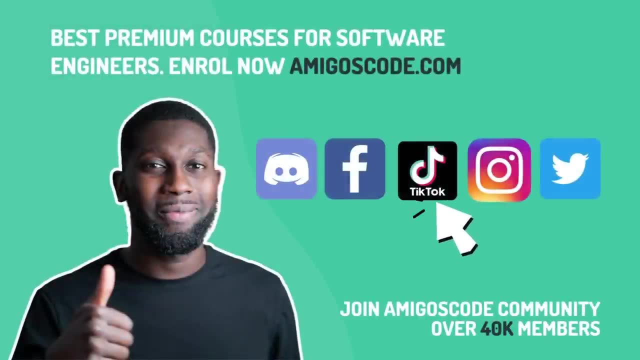 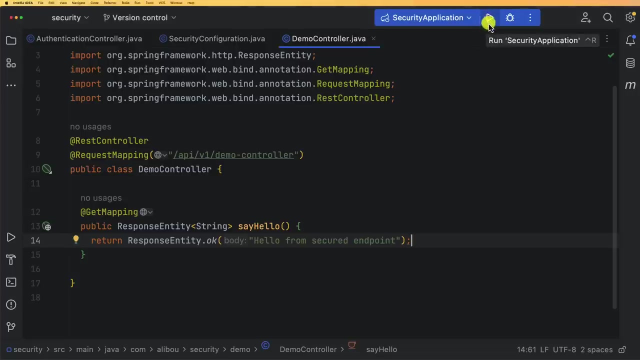 Now let's go ahead, Start our application and test these changes. Let's start the application and make sure that all the code that we wrote together is working fine. So go ahead, Click on start and let's see what we will have in the console. 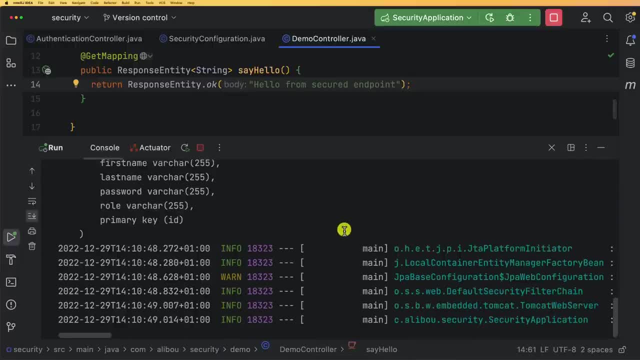 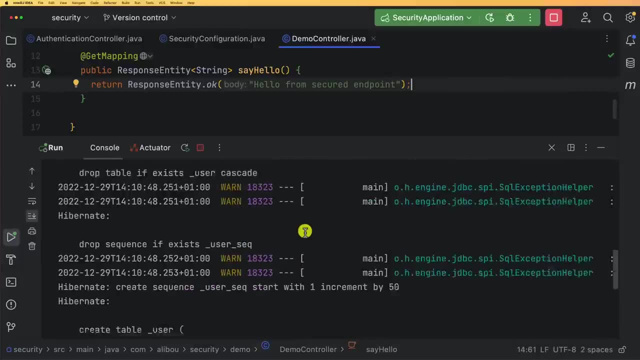 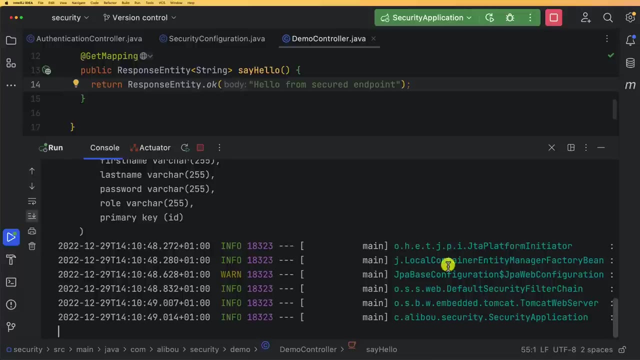 So let's make sure that everything is fine. So, as you can see here from the logs, we no longer have this auto generated password by spring security And we have here that you are creating the sequence and we have the table, user gets created and the application is running correctly. 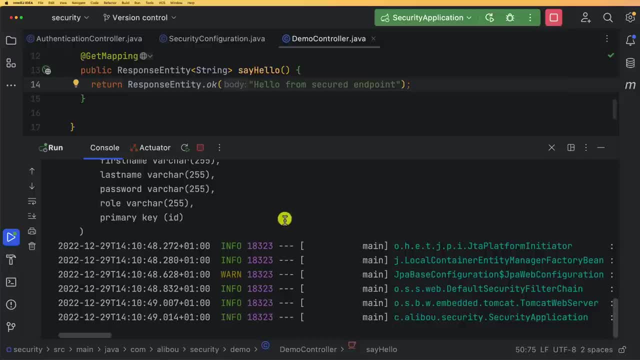 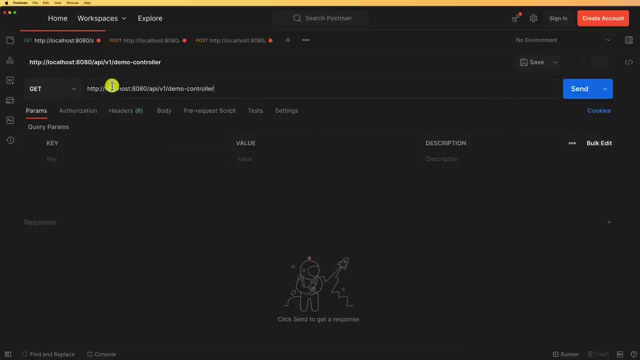 Okay, So now let's start our postman and test this endpoint. So I have my postman started right now, So I will use this endpoint Within a get request. So the endpoint is localhost and my port is 8080. slash API. slash V1. slash demo controller is the same one that I have right here within my code. 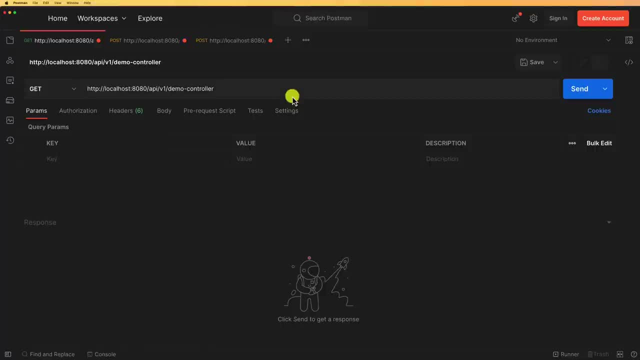 It's demo controller And now I will click on send. We see that we have no authorization, We have nothing in here, So I will just go ahead and click on send And normally, like the expected behavior, is this endpoint Should be secured. 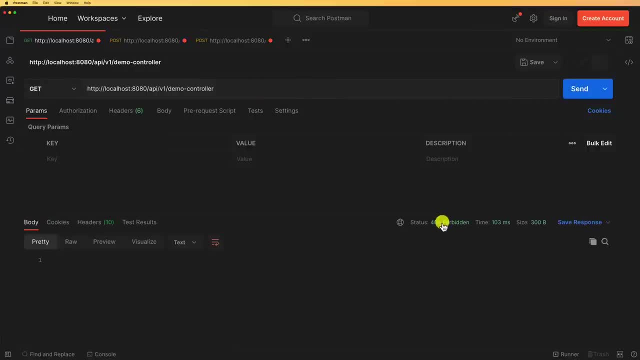 Okay. So when I click on send, we exactly can see that we have a 403. forbidden means that we are not allowed to access this endpoint. Okay, Next, we have our two endpoints, the authenticate and the register. So let's first start with this register endpoint. 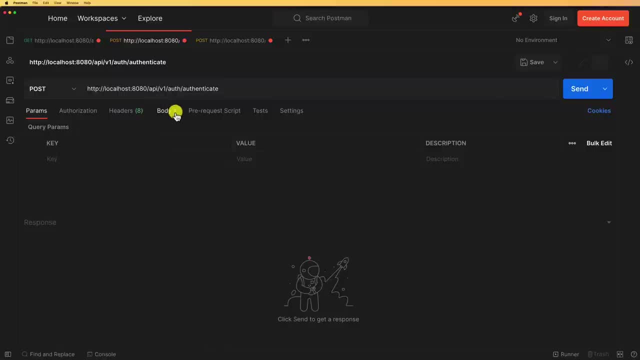 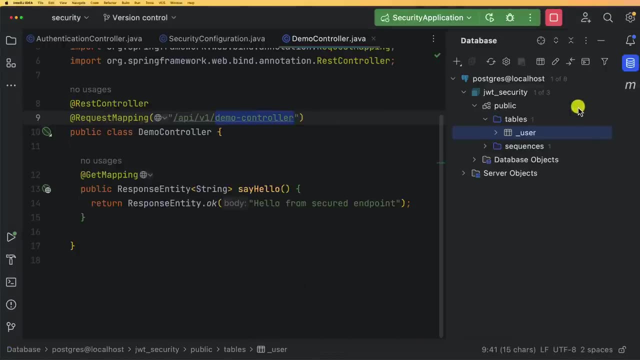 Or let's before that. let's start with the authenticate And for the authenticate. Now we know that we have No user within our database. We can also double check that. So if I open, let me close The other tabs. 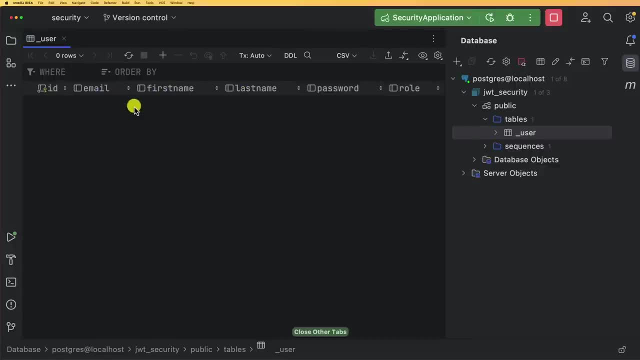 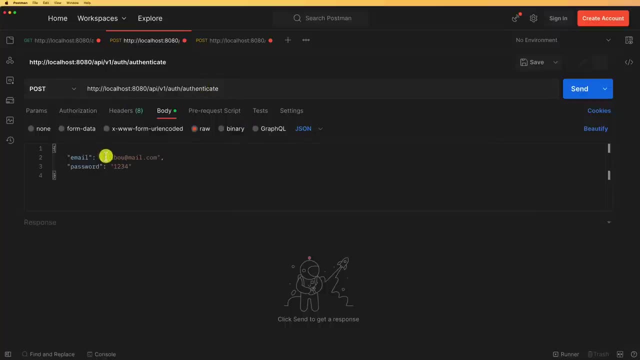 So here I don't have any user registered within my database. Okay, But now if I try to connect to or to authenticate a non-existing user, I also expect to have a 403 as a response. And this is what we see, right here. 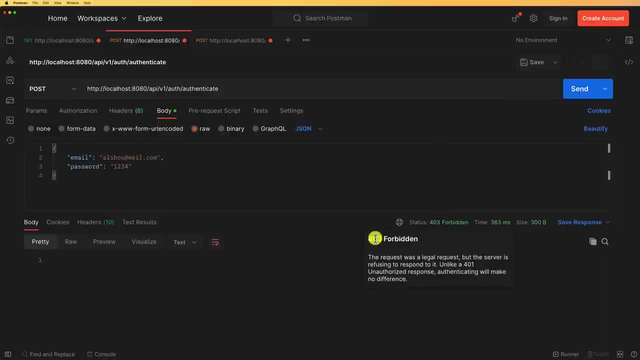 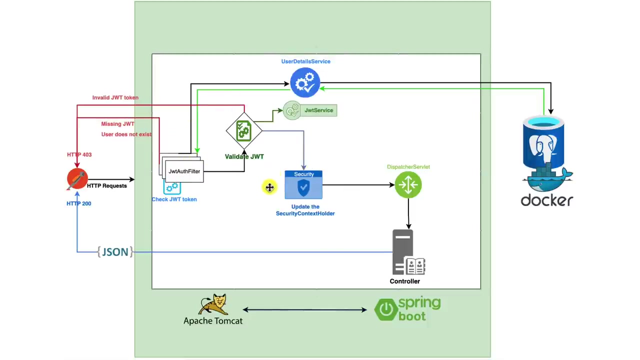 So it's 403 forbidden And the user is not allowed to access this endpoint. And this why? Because we have here within our schema, So we try to check and validate everything, even if the endpoint, Even if the endpoint is secured. 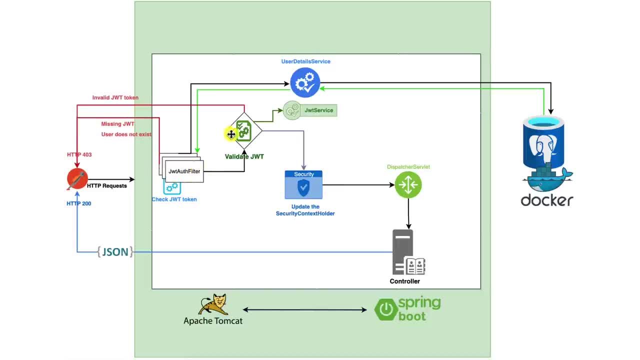 So we get into this authentication filter, We validate everything, But once we get to the user details we don't have the user in the database. So in that case we will see. In that case we will send back a 403 to our customer. 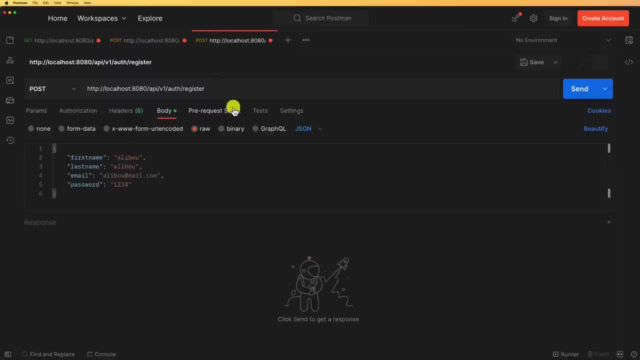 Okay, So now let's create a new user. So I will register a new user. So I give it Alibu as a first name, Alibu last name And Alibu at maycom and 1234 as a password. So now when I click the send button, I should get generated token or a JWT token as a response. 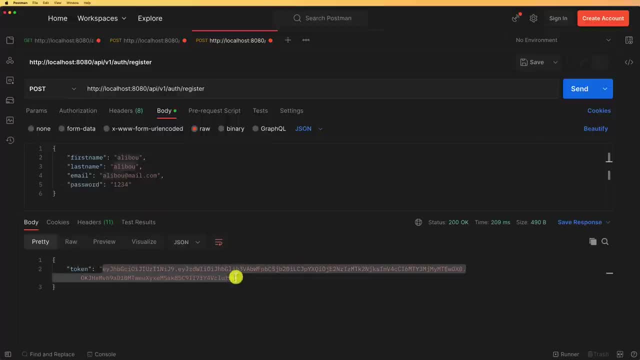 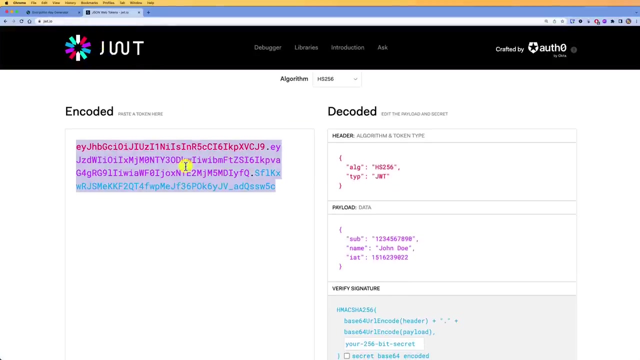 So This is what we see right here. So I will just copy this token and I want to decode it And let's see what we have within this token. So let's go back to the JWTio website and paste the generated token in here. 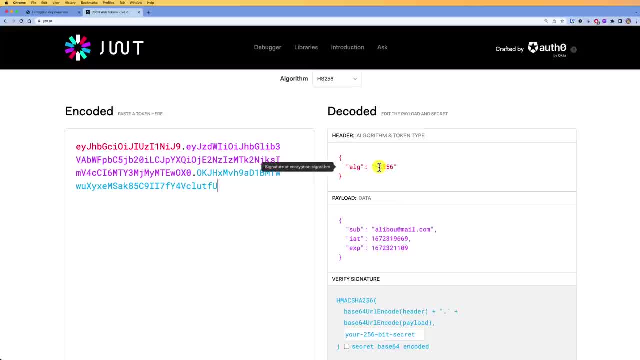 So we see that we have the algorithm here, which is the HS256, the one we use to generate this token, And we have our payload. So we set already the subject to the to the user email and we have the issued at. So the creation date: 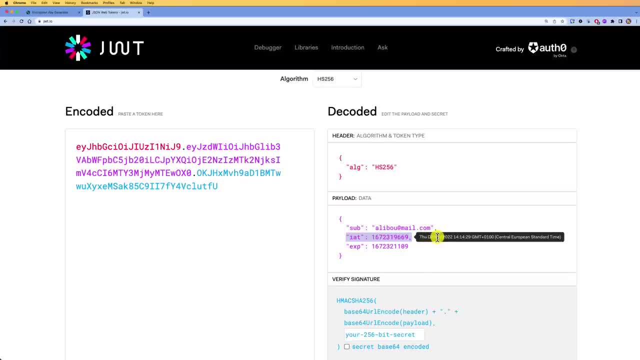 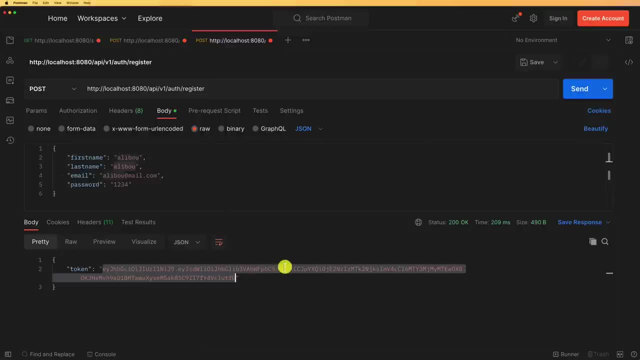 And, as you can see in here, it was created December 29 and 1414. And this one will expire at in 24 hours. Okay, So this is our generated token. Let's go back and test the authentication right now. So we see that the register is working. 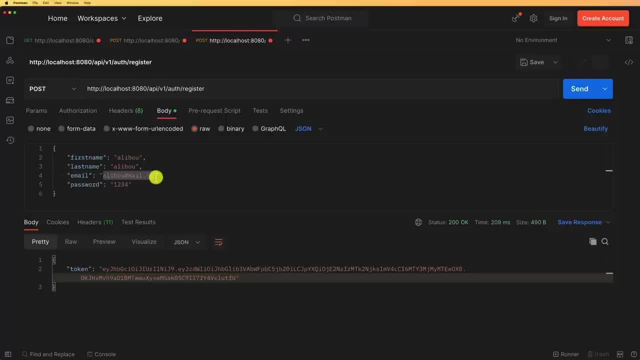 But let's ensure that Within this same username and password, we are also able to get a token or to generate a token. So this is the same email and the password that we have And if I click on send, I should get the token. 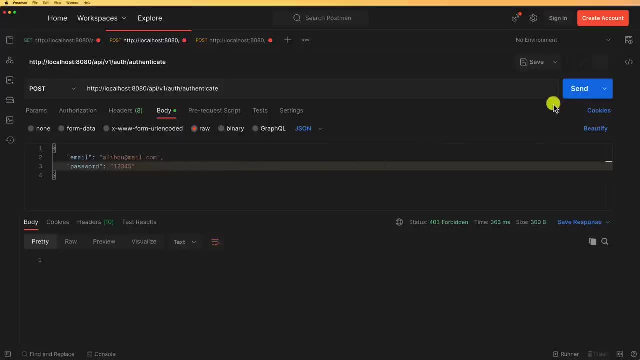 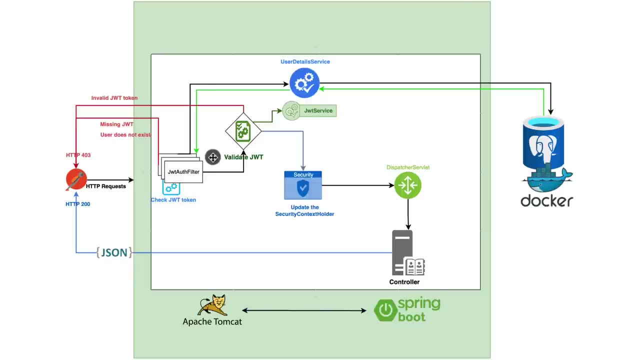 But let's first try with a wrong password. So when I click on send, So here we have our 403 and here it's because of this process, So we have the token and then we start the validation process, So we extract the username and password. 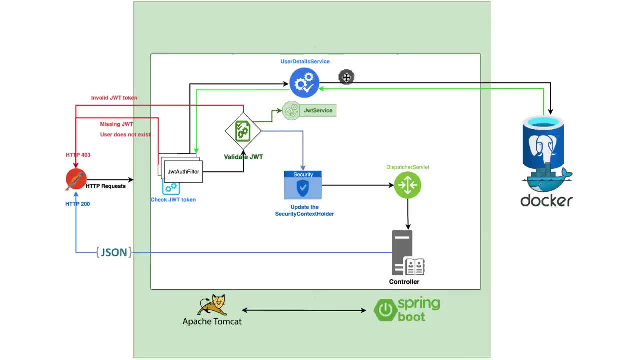 And then we are calling the user details service to try to fetch the user from the database and the user. We got it because the user already exists. But when we move to the security filter chain and to use when we move to security context holder, we will try also to use the authentication manager to authenticate that user using the password and the user mail. 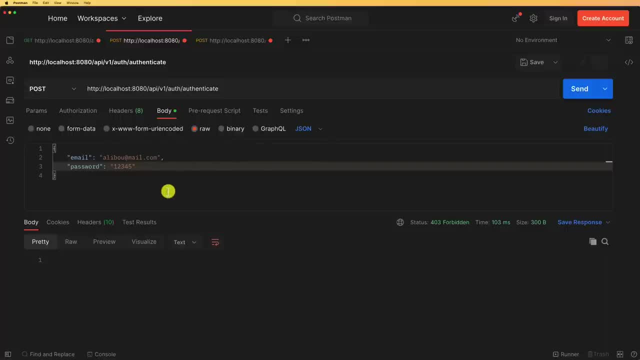 That were provided within the request, But this password is wrong, So that's why we are also throwing a 403 as a response. Okay, So now let's test with a correct password. So if I click on send, I see that I have my JWT token. 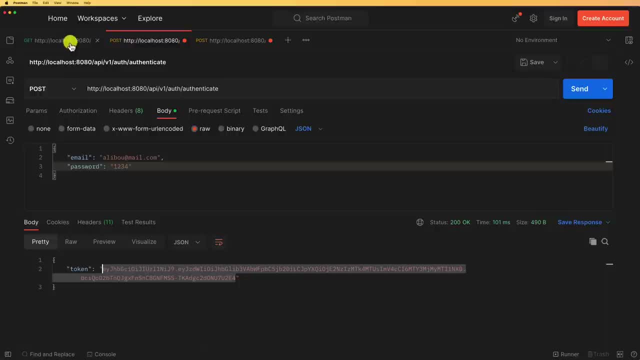 I will copy this one And then I will go back to this get method. I will click again and make sure that it's always 403.. And how we can authorize this request right now. So, within the authorization here, within the type, click and choose beer token.